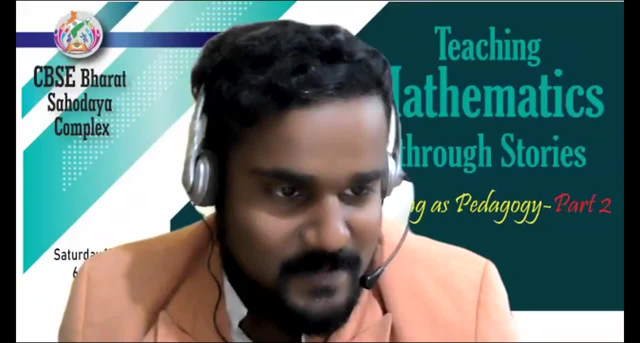 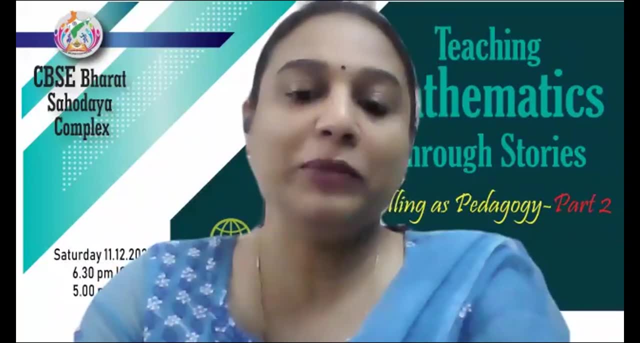 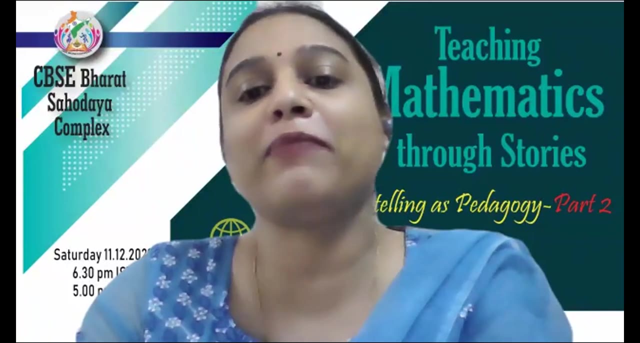 Please, Ma'am over to you, Thank you. Thank you, Mr Arun Mohan. it couldn't have been a better beginning. Thank you so much. Good evening to one and all. Yes, Tell me your story, Tell me your yarn, Tell me your skill. 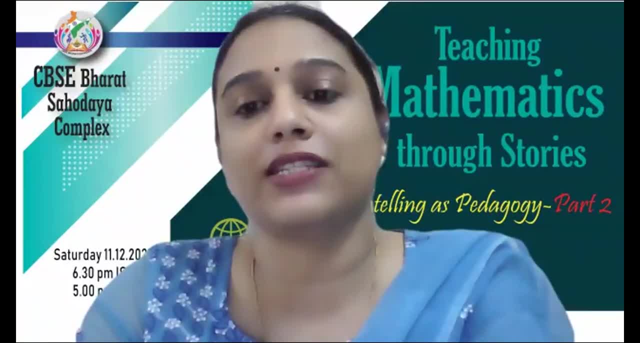 Take me on a sighting journey of magic carpets and graceful swans. I want to study, I want to learn. Can you help me address this little concern? I am a child with a vivid imagination who loves stories of every kind. They help me indulge my natural curiosity and enlighten my fertile mind. 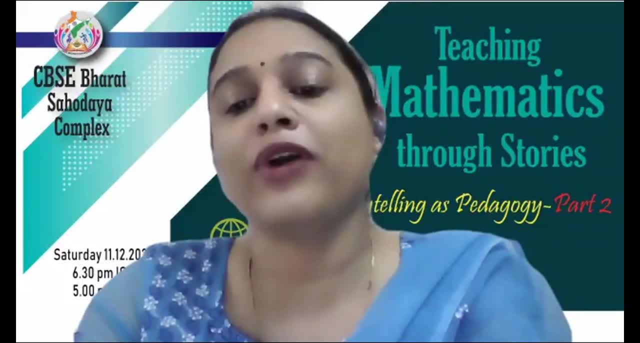 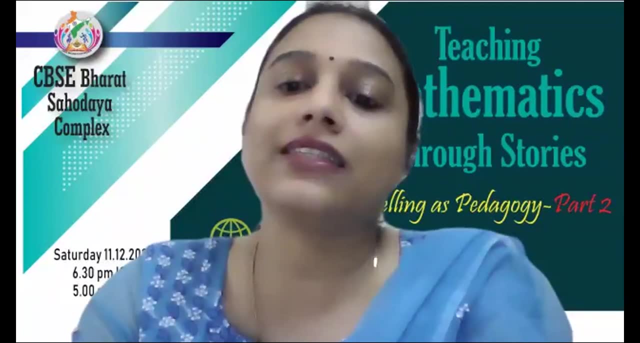 When you tell a story I love to learn. Can you help me address This little concern? Good evening to one and all present here. Doesn't this little poem remind us all of our students? Each of us who has ever been to a class has experienced the eagerness and bristling energy in our kids when they hear the word story. 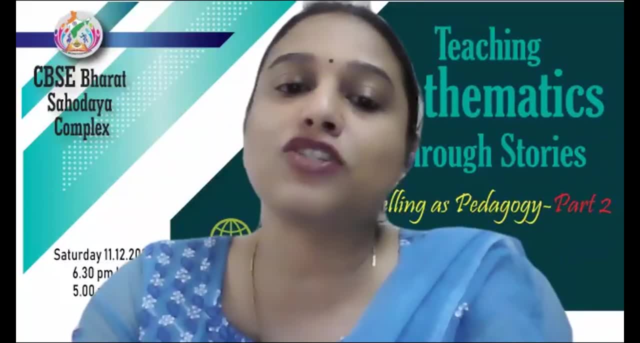 Right from the tiny thoughts to our 12th graders. there is no child who cannot be charmed with a story. Today, we have all gathered. We are here for the 102nd web training series conducted under the aegis of CBSE Bharat Sahodhya Conference. 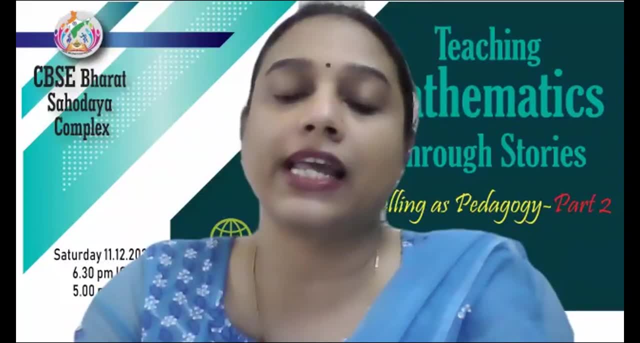 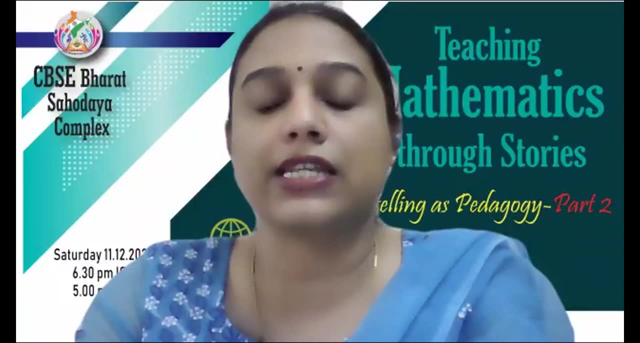 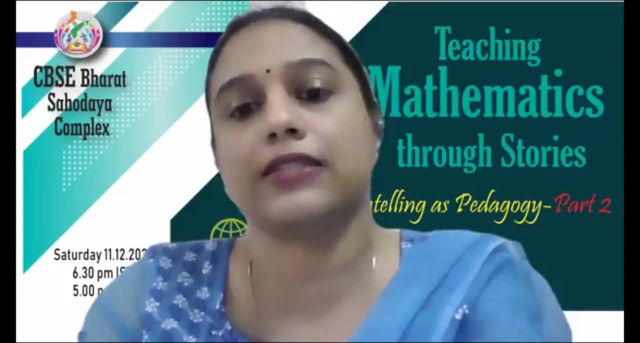 This session is part two of the Storytelling as Pedagogy series of the CBSE Bharat Sahodhya training sessions, And today we will be dealing with the ways in which mathematics can be taught to storytelling. Humans are storytellers. 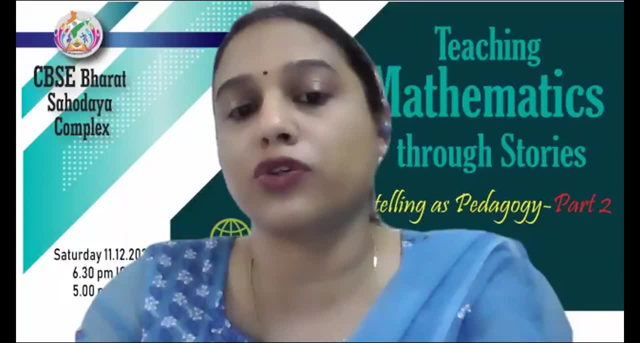 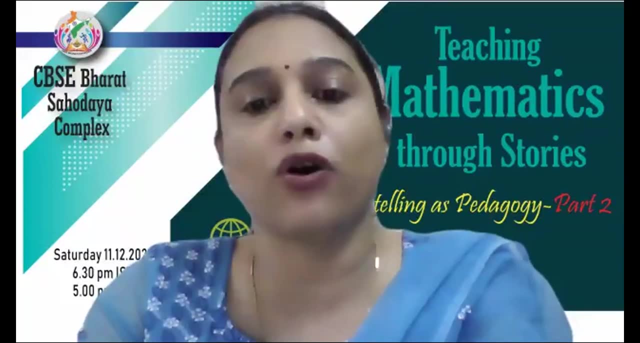 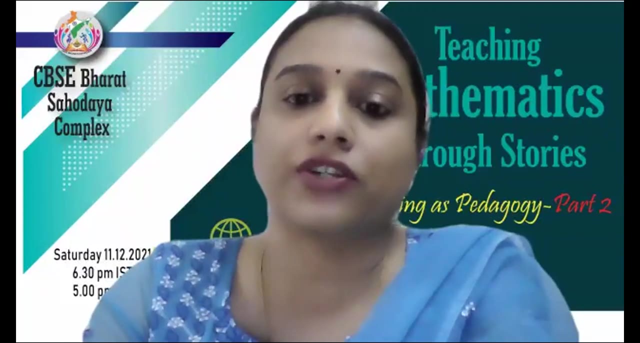 We have virtually forever used stories to communicate, To pass on wisdom And to spur imagination. As long as people have spoken to each other, well before the advent of the written language, storytelling serves to pass down cultural, ethical and other information from generation to generation. 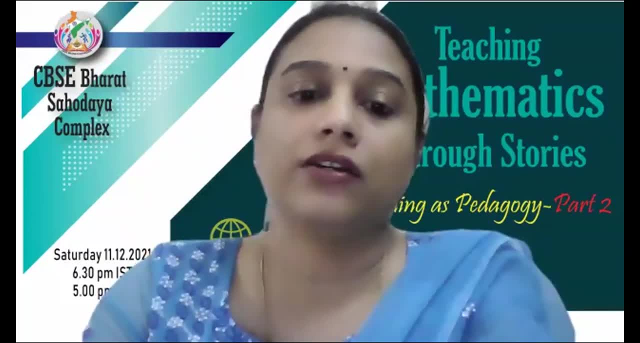 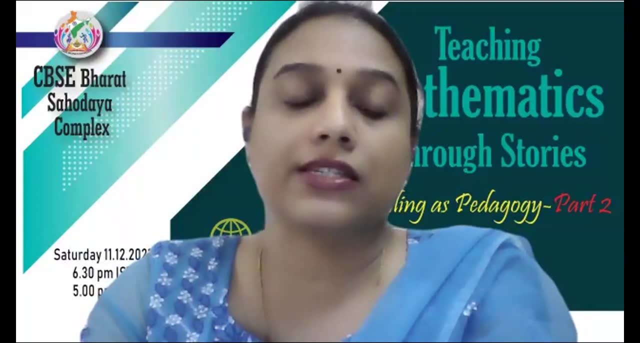 Even today, in a modern, largely literate era, oral communication is still arguably more important than written communication. There is evidence that humans may even learn better than written communication. There is evidence that humans may even learn better than written communication. There is evidence that humans may even learn better than written 반응 pouvoir. 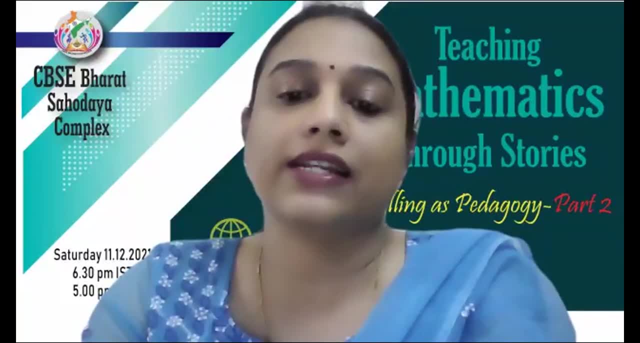 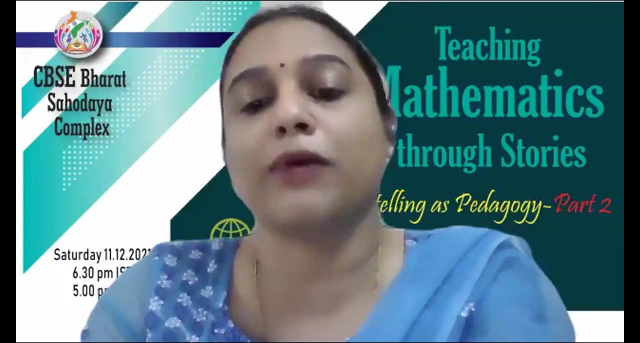 when some content is presented as a story rather than a lecture. While the powers of storytelling have been tried and tested in the languages ​​and the social sciences, I guess it is still relatively new in the field of mathematics, And that's exactly what Usha Mandel threw light on in today's session. 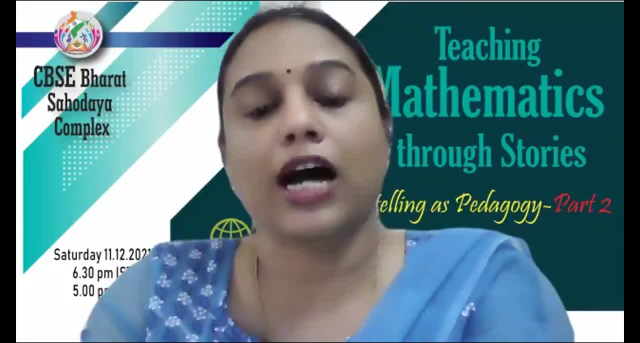 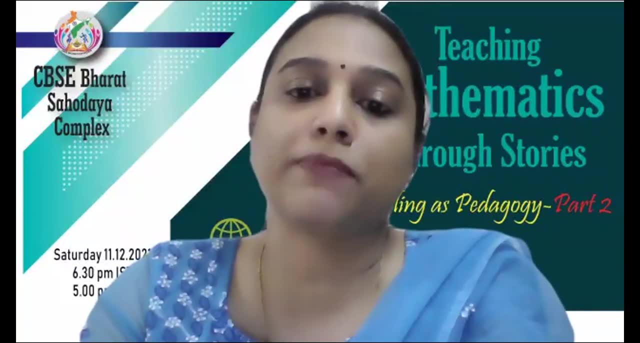 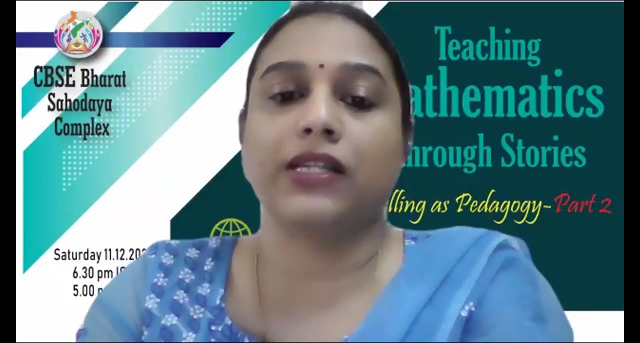 I'm sure all the educators gathered here today are looking forward to an exciting and enriching session. Before we commence, I request the participants to please note a few points for the smooth conduct of the session today. Kindly be visible and keep your mics on mute. 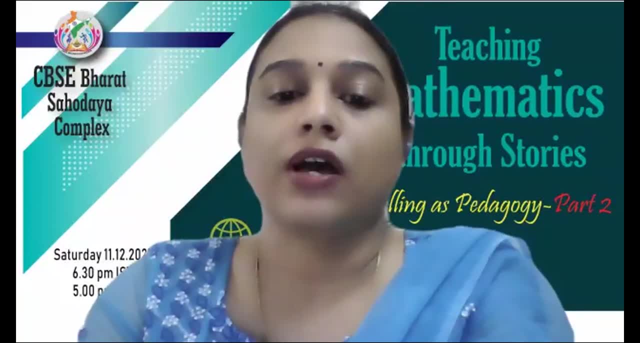 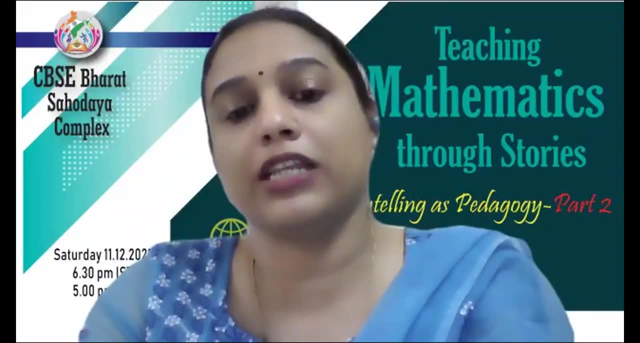 We have tried to incorporate the questions that most of you have asked during the registration. Pusha ma'am will be addressing those. If there are more, you may post them on the chat box. There is a dedicated question and answer session at the end in case you wish for more clarification. 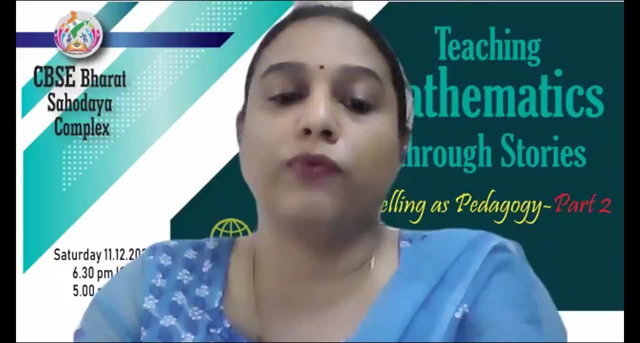 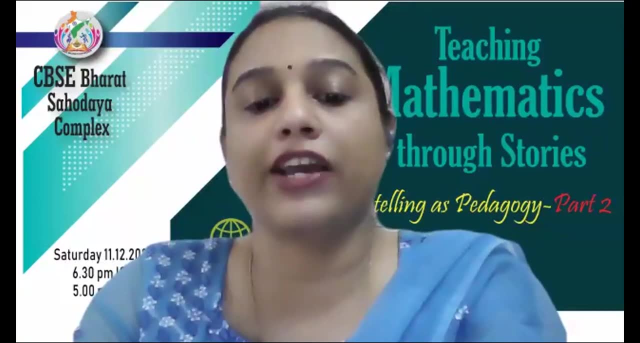 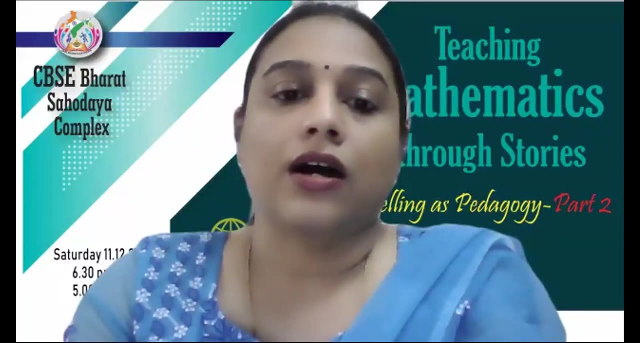 Kindly note that the feedback and certificate link will be shared towards the end of the session. Please note that this is a permanent link for all our sessions And a humble request to all of you to stay connected till the end. I now take the opportunity to welcome our Program Director, Dr Abdul Salam. 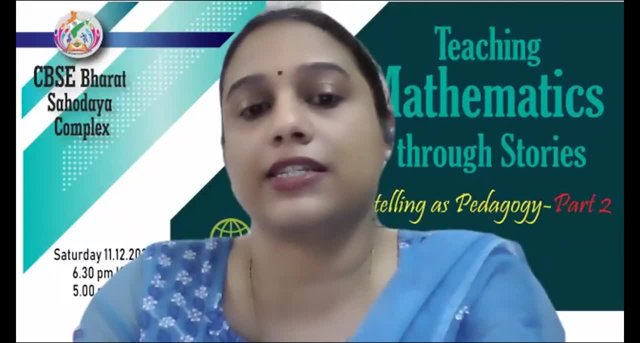 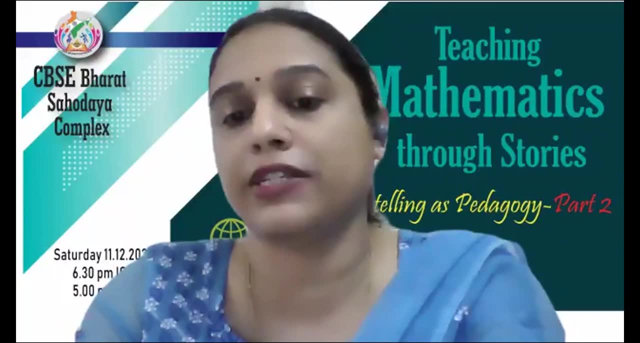 He is the captain of this ship of transformers, who works tirelessly towards empowering educators across the country. His relentless efforts have brought so many of us educators on a single platform, thus enabling us to share resources, material and ideas to not only help our students, but also to empower ourselves professionally. 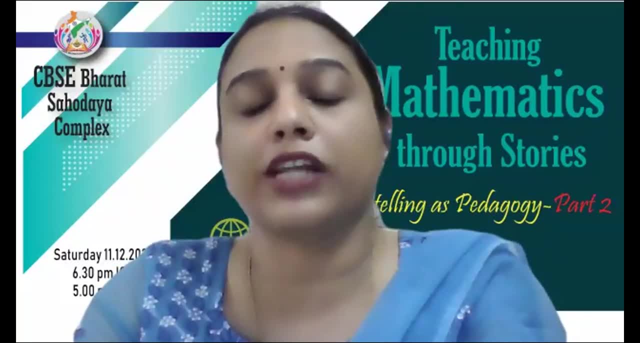 A humble thanks, sir, to you to all the support and provide and help and support that you provide us with. May I request you to welcome. deliver the welcome address, sir, Over to you. Salam, sir, Thank you. 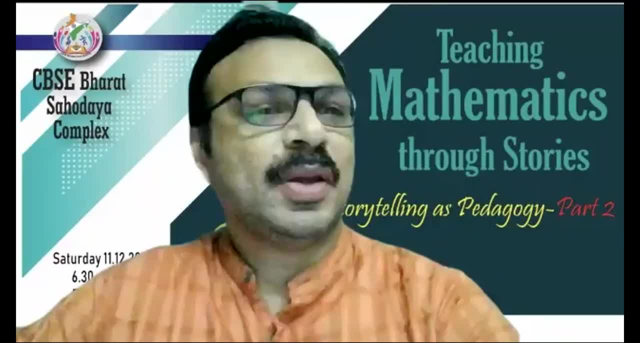 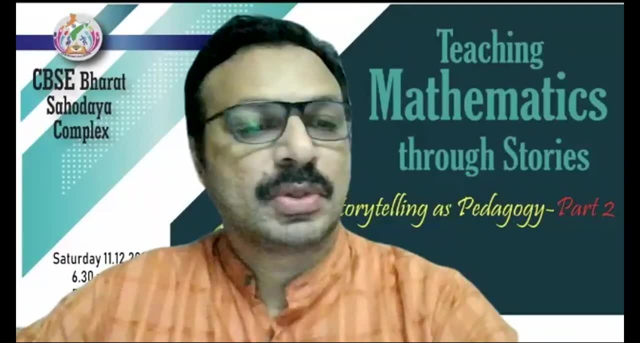 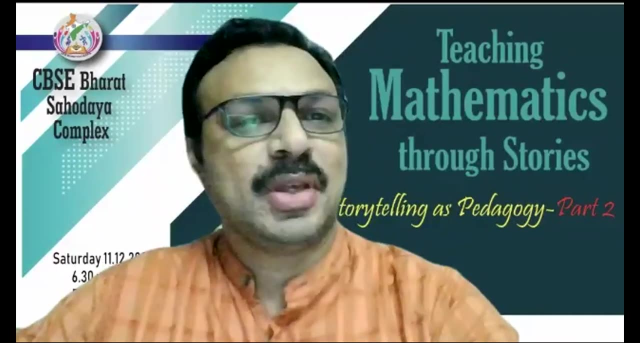 Good evening and a hearty welcome to each and everyone: respected resource person of the day, Ushah Chhabra, ma'am and moderator Saritha ma'am, Mr Arun and each and everyone. We are back after the celebration of the 100th episode. 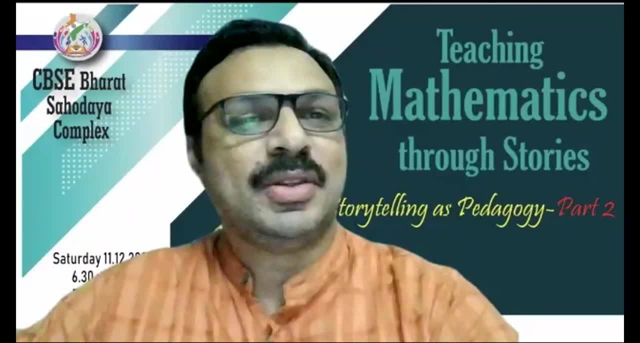 We cannot, you know, take rest, as there are many things waiting for all the educators to know. And we cannot, you know, take rest, as there are many things waiting for all the educators to know. We cannot, you know, take rest, as there are many things waiting for all the educators to know. 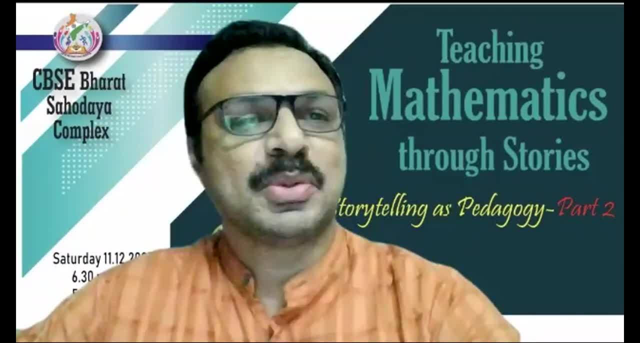 And we cannot, you know, take rest, as there are many things waiting for all the educators to know. And we cannot, you know, take rest, as there are many things waiting for all the educators to know, And Ms Saritha has given a detailed introduction. 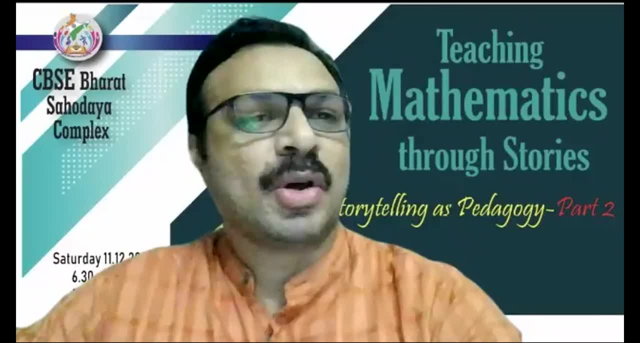 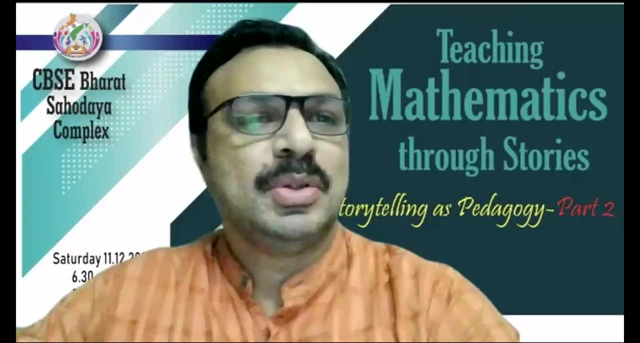 There's no need to say it's not a topic for debate as well. Everybody likes stories And of course you can. you know, use stories in different ways. Definitely, you can also invent stories. When we were children, you know, grandparents used to invent stories. 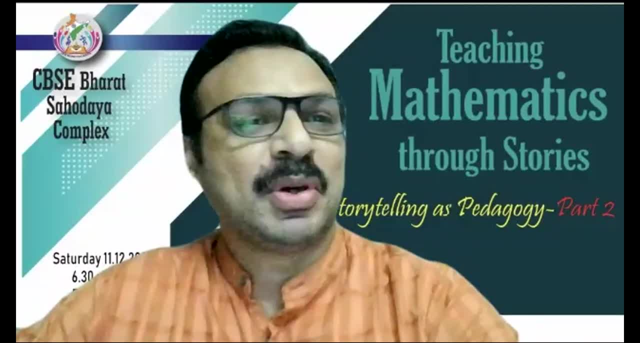 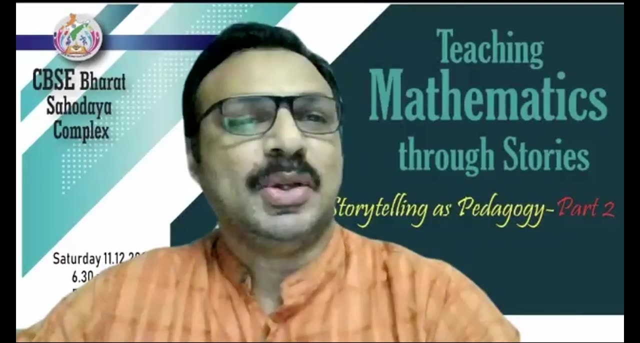 and you know, in order to make us, you know, keep quiet and listen, to also eat food or learn a study, i mean so, uh, these are different, you know? uh, what do you call ways? there are different ways in which you can use stories, uh, to get into the heart and minds of children. when i say this, i 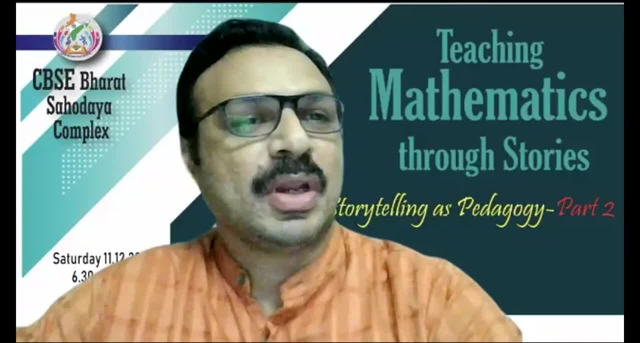 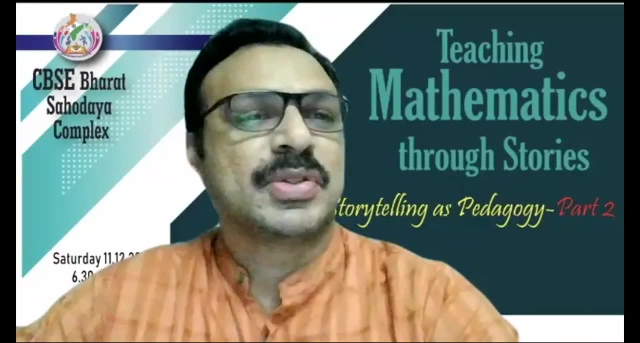 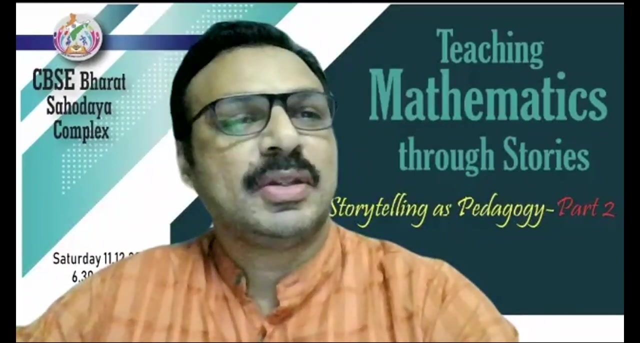 remember a story which i was talking, you know telling this to my school children, when a teacher wanted to teach the importance of making efforts, hard work, and all she made a story and, you know, told the students. dear children, i'm going to tell you a story there are. there was a farmer who had 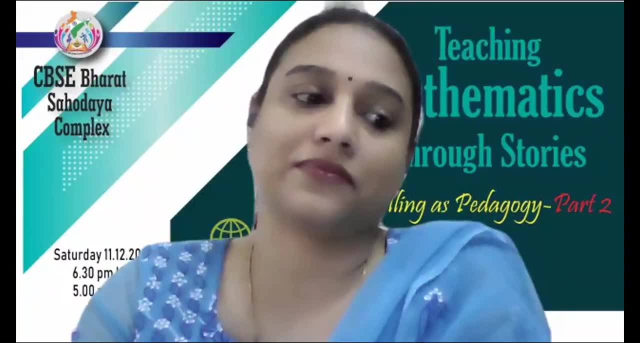 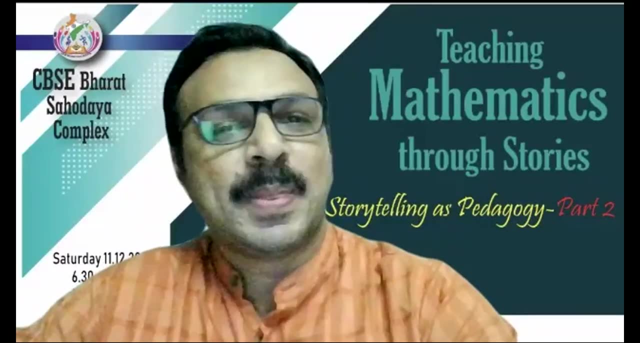 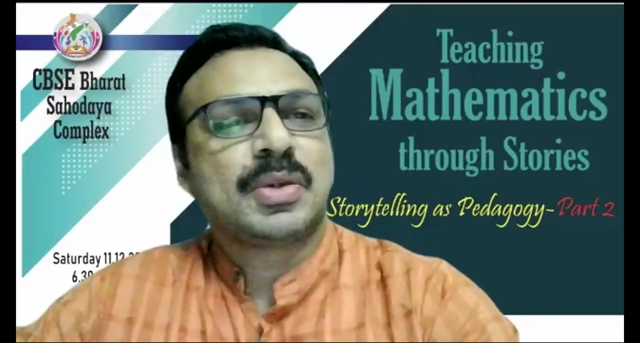 three sons, and these sons were not, you know, so active. you know they were not so active and they were not so active. and they were not so active, uh, and was they were, they were not helping, uh, their father. so, uh, father, the farmer one day called his sons and told: there is something you know, you must, must, you must know in life. 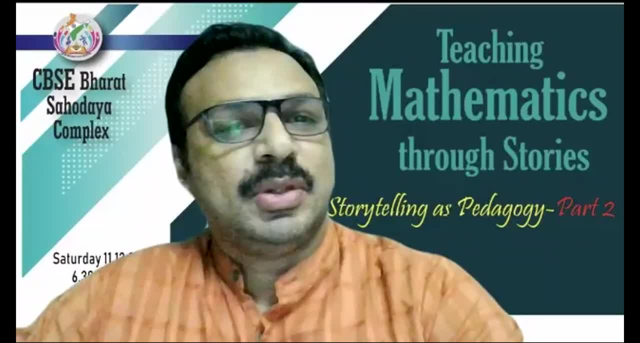 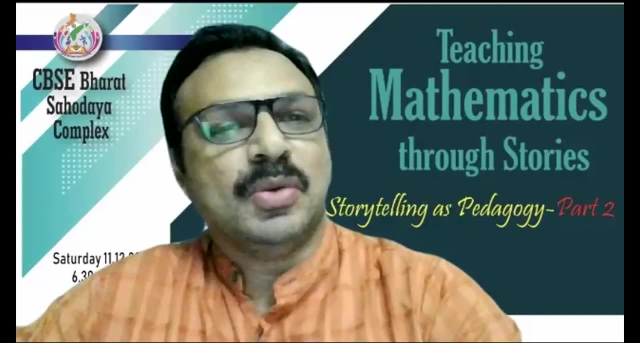 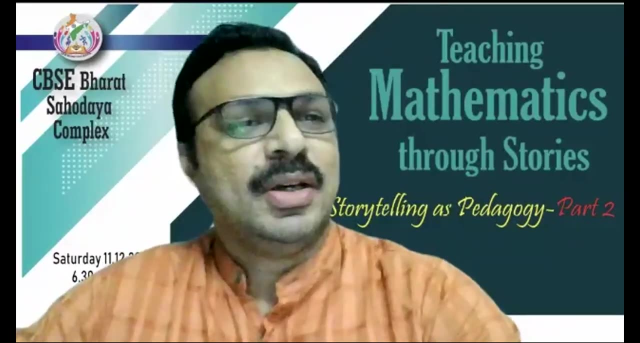 there is a secret of life. children asked: what is the secret of life? they want to know. they became very curious. all right, when you become 12, i will tell you the secret of life. days passed on and the eldest son became 12 years. he went and approached his 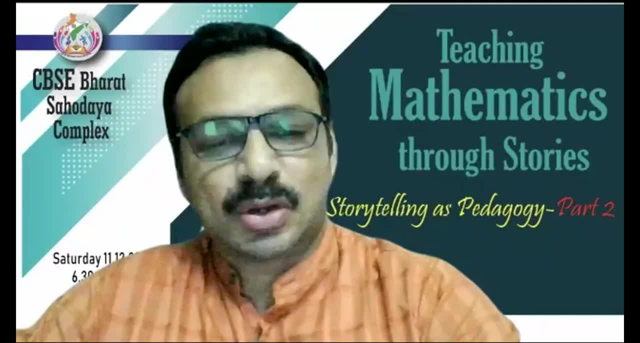 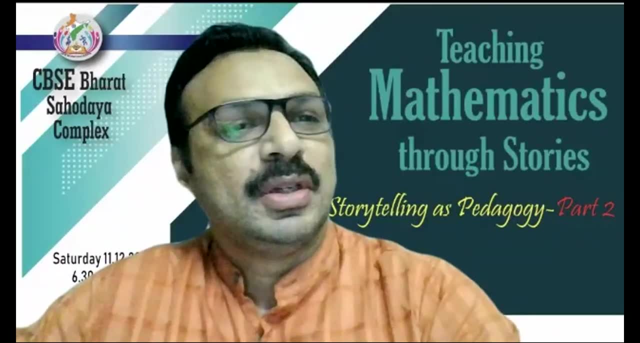 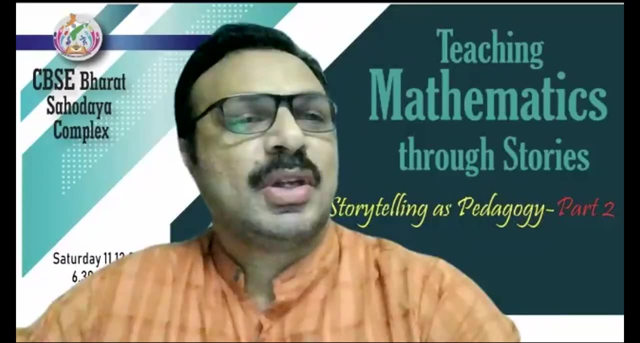 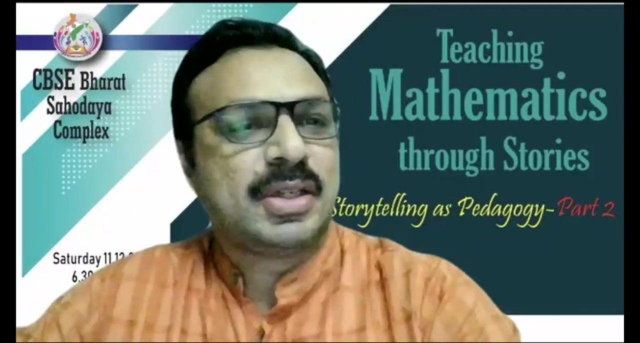 father and asked: father, what is that secret of life? the farmer said: all right, my son, i wanted to tell you that cow does not give you milk. he said. he repeatedly said i have a. he said he repeatedly said i have a. and his son, you know, went on asking: cow does not give us milk. he went on, you know, arguing as well. 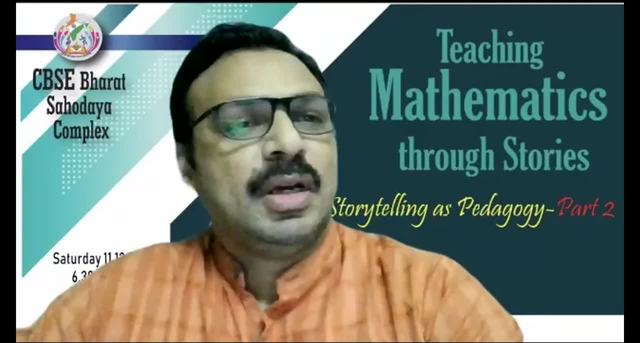 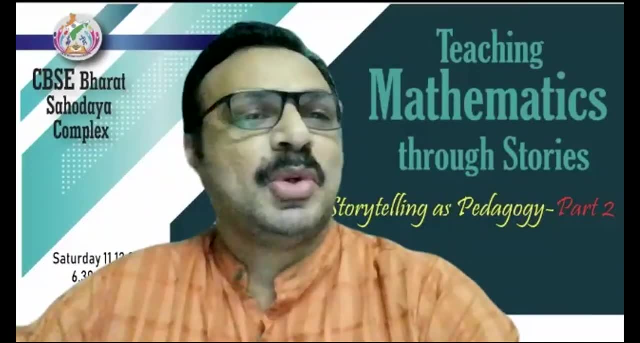 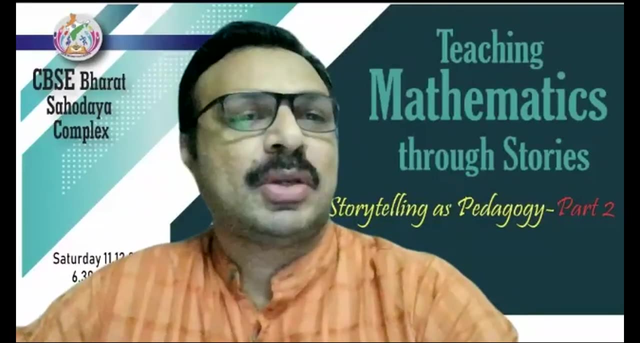 then the farmer said: you see, you have to milk the cow. the cow does not give you milk. you have to milk the cow. you have to feed the cow. you have to bring the cow up. you have to then make all arrangements. you have to milk the cow. it all depends upon how you milk and how you. 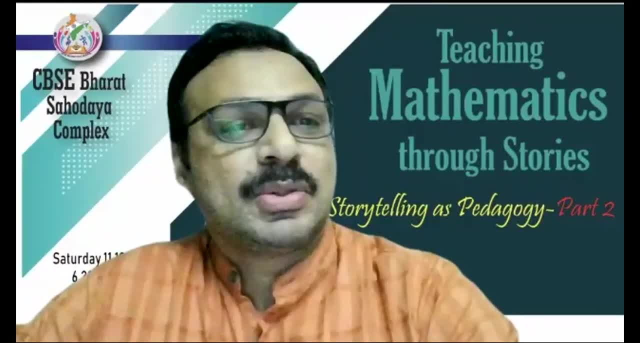 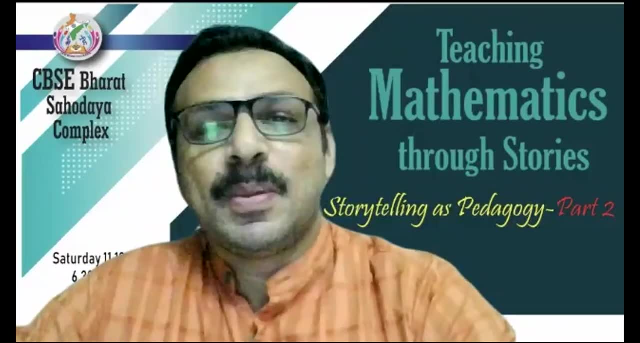 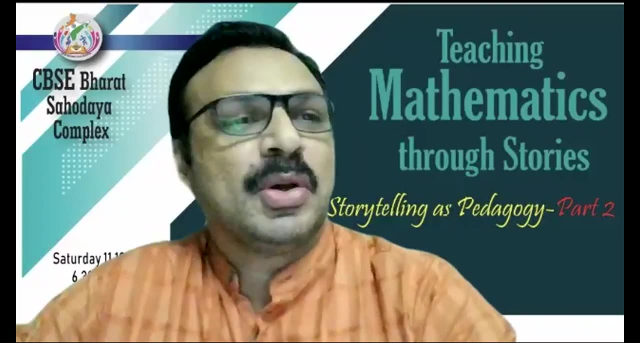 do it, how hard you work. so the success of life is hard work. the children understood what you know their father was doing and uh, they started, you know, helping him the next day because you know the way in which the father told the success of life is for something different. 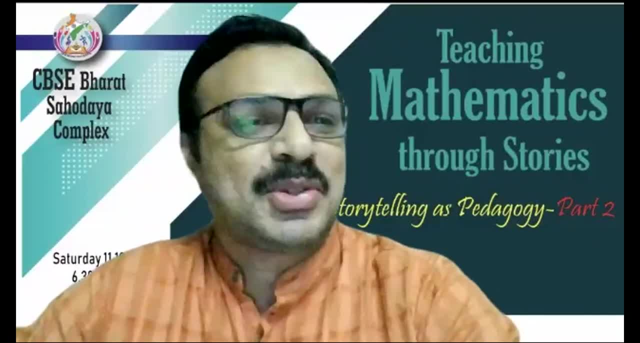 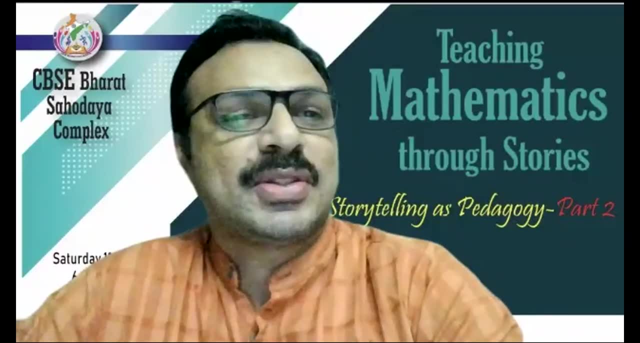 this is how we can use stories. you know, we have to invent stories. we can use stories in different ways for different subjects. so let's uh listen to usha chabra ma'am, who has come for the second time, after the brilliant program we have had with her sometime back. 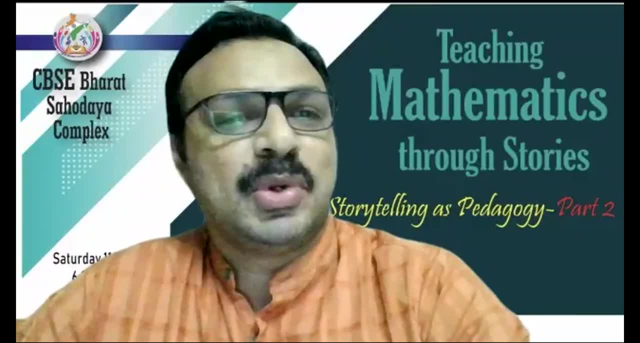 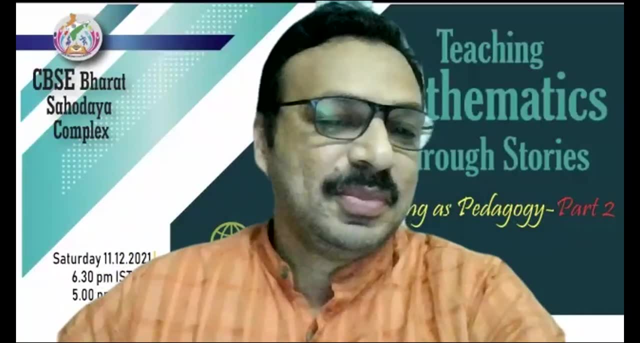 we uh on behalf of each and everyone. we welcome usha, chabra, ma'am and each and everyone to this uh program. thank you so much. over to saridam, thank you. thank you very much. our next dignity for today is our program collaborator, mr shibu. 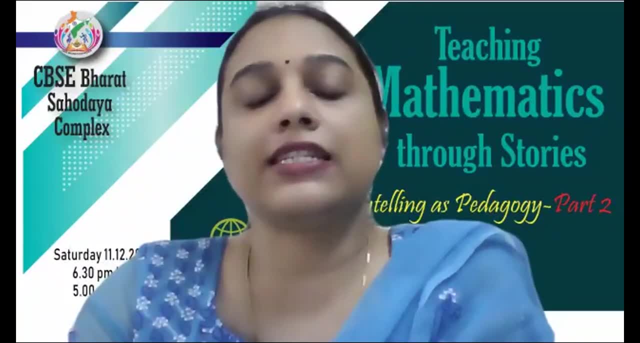 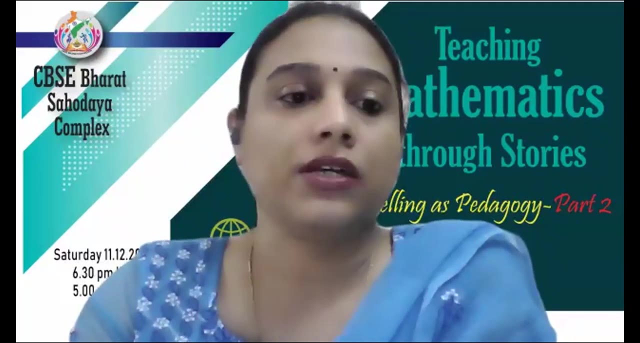 mrs shibu is the honorable president of bharat sahodia. he is a veteran principal who has many years of experience in the education scenario. he has served in many capacities during his long and illustrious career. at present, he is the principal of hk and residential schools, column. 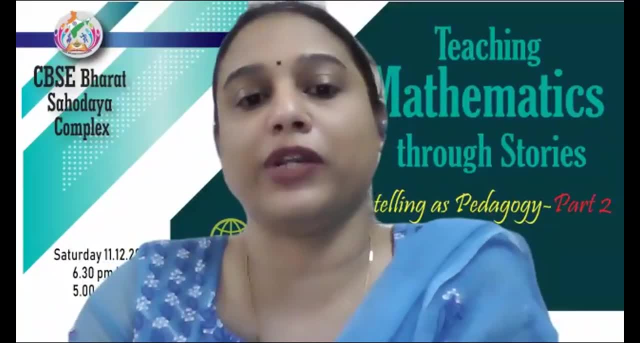 i take the privilege of welcoming, as a first person for today, usha chabra. good evening, ma'am. this usha chabra is a red scum awardee, an educator, an author and a passionate storyteller. usha lan has been teaching hindi for 24 years at delhi public school, rohini. 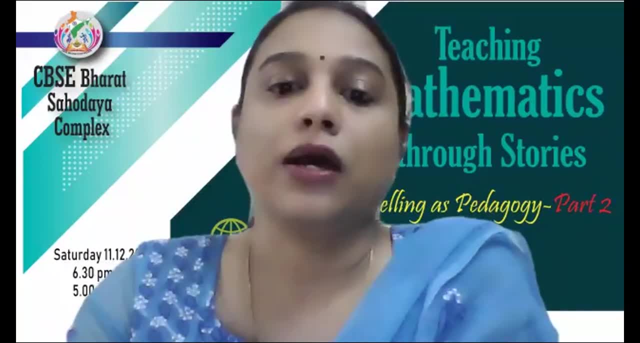 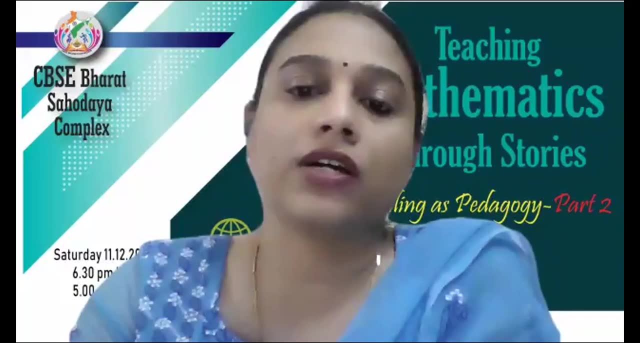 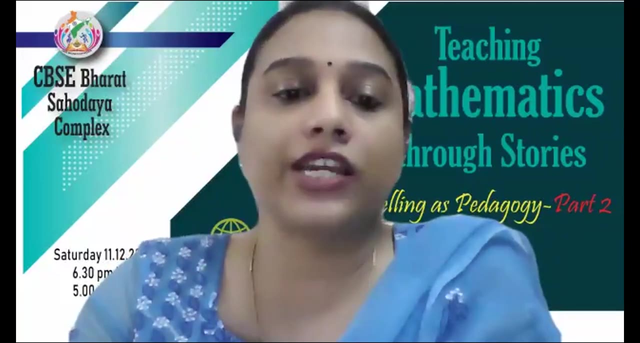 her mission is to ease the challenge of states in hindi by both the teacher and the toss as part of making hindi accessible to all. she has authored three separate series of textbooks in hindi, as well as published a couple of poetry books. she has reached out beyond the confines of her school. 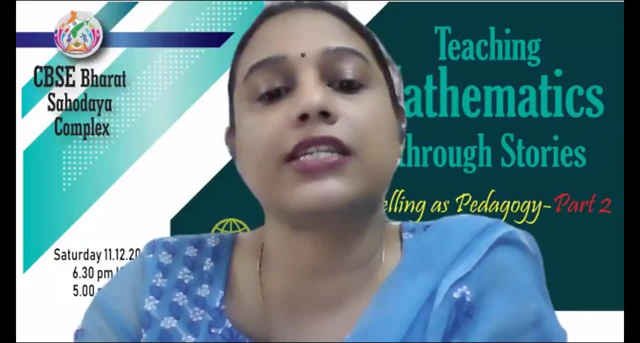 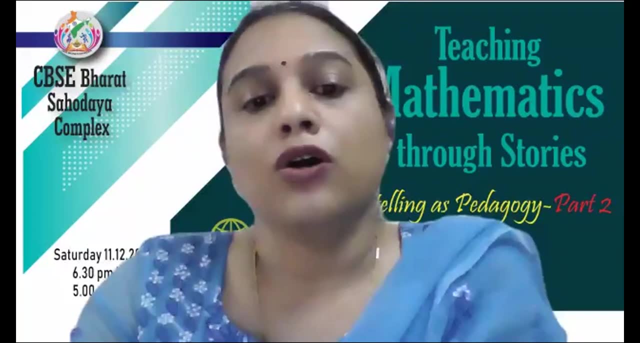 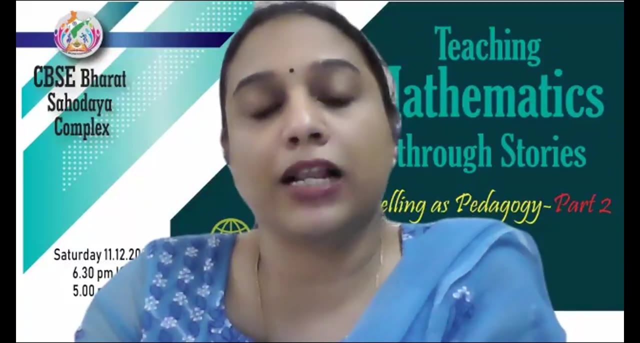 and ventured into conducting storytelling sessions, teachers and parents orientation programs and workshops for children on creative writing and dramatics across india. usha ma'am has taken sessions at the world book fair, nehru memorial museum and library, national baal bhavan, rajiv gandhi foundation and many more. she was also a part of the prestigious jaipur literature. 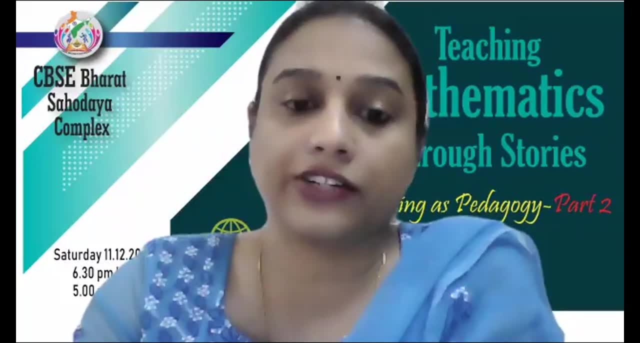 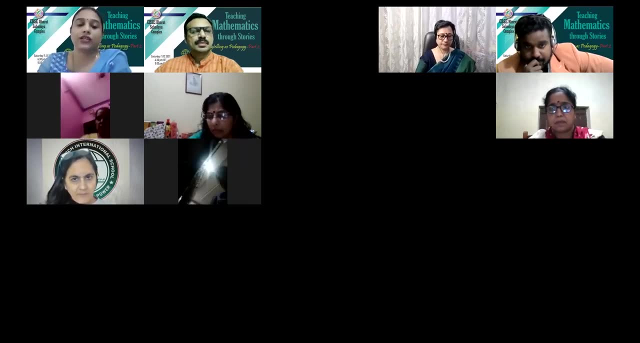 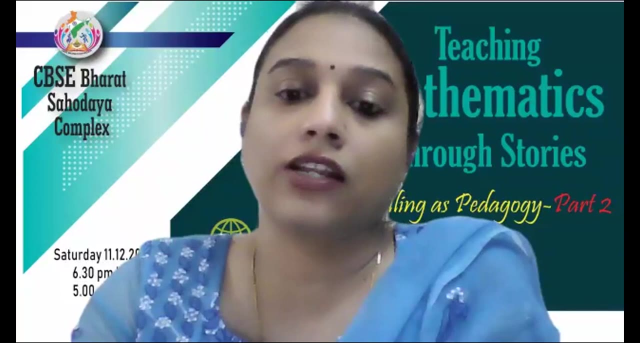 festival outreach program, divani children's literature festivals, kampu literature festivals, to name a few. to keep up in this digital age, and especially in current times, madame has conducted numerous online sessions and updated her challenge channel on youtube, which is a repository for teachers, parents and kids facing challenges in learning hindi, be it grammar book chapters. 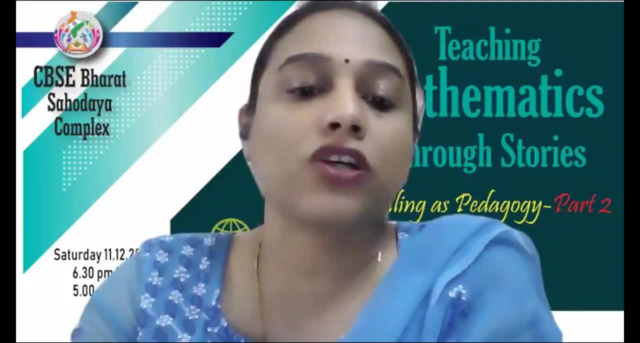 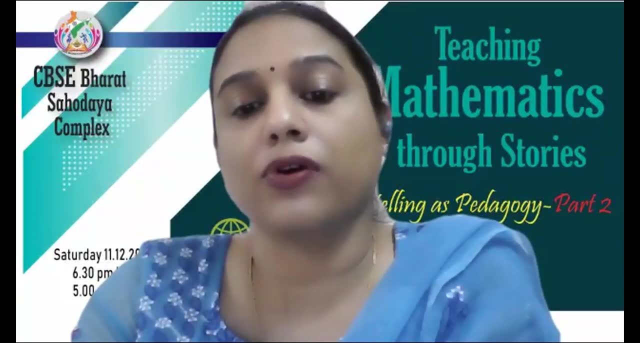 storytelling or poetry recitation. she has also designed capsule courses for teaching hindi to non-hindi speakers for students of indian origin in singapore, the uk and the us. in addition, she has scripted stage shows for nakya ballet center and ntpc. it's a privilege and honor to welcome you, dear usha ma'am, we are all waiting. 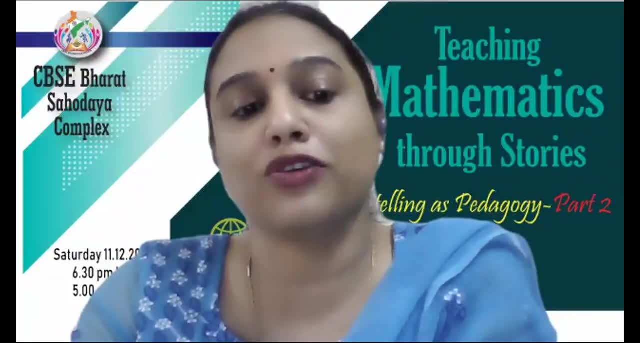 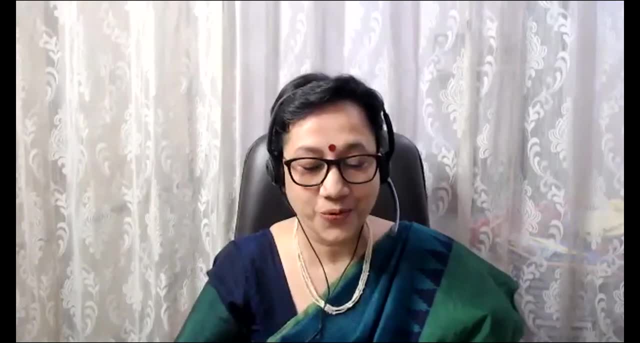 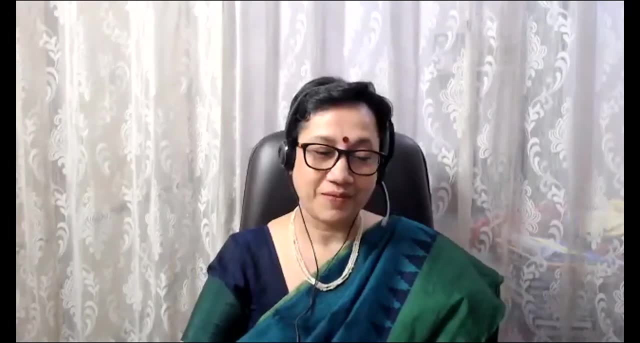 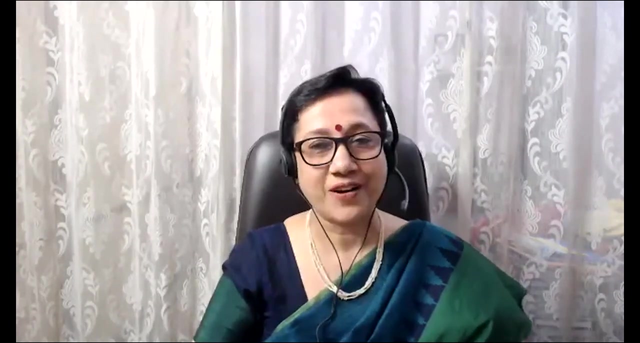 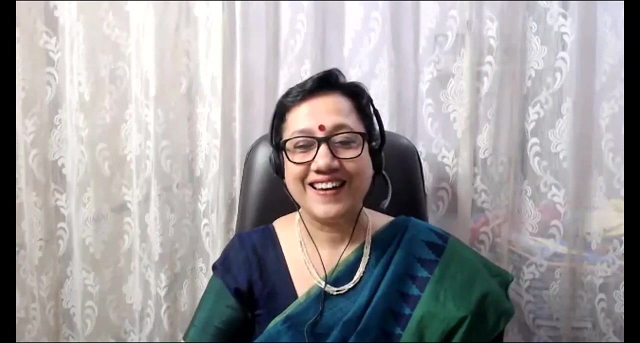 thank you, ma'am. dr abdul salam, sir, cbsc bharata, their complex team, mr shibu and sarita ji, thank you so much for the beautiful introduction and i am really honored to come here and speaking in front of you all. thank you so much, sir, once again. so, uh, let me start by talking about 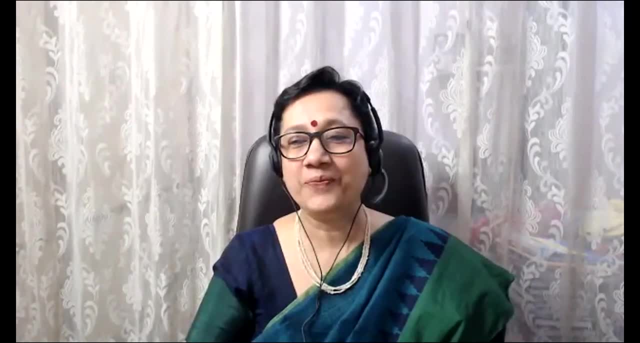 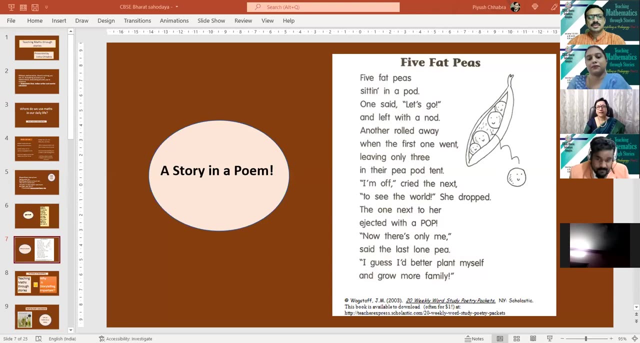 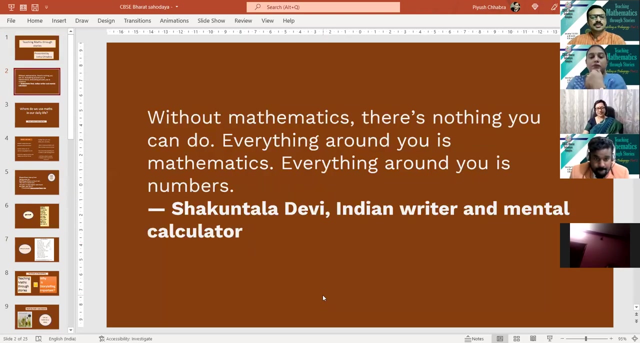 mathematics. you are able to see my screen, sir. sorry, Taji, you are able to see my screen, okay, okay, okay, okay. so first of all, let us listen to what Shakuntala Devi, Indian writer and mental calculator, the maths genius, we say: without mathematics, there's nothing you can do. 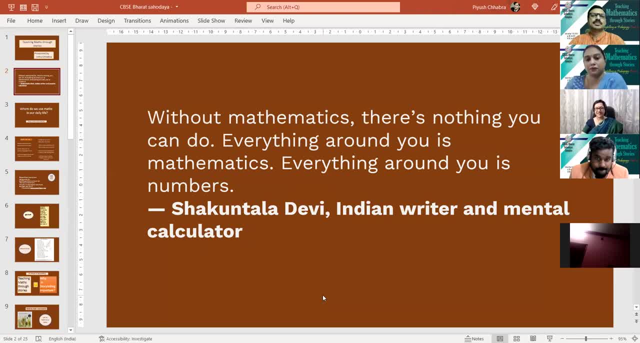 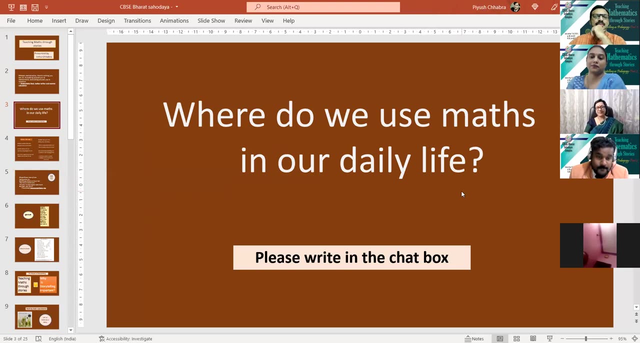 everything around you is mathematics, everything around you is numbers beautiful, so mathematics is everywhere. so I just want to know from my audience- my teachers sitting over here to just write down in the chat: where do we use daily life? please write down in the chat, let me see. where do you find maths? 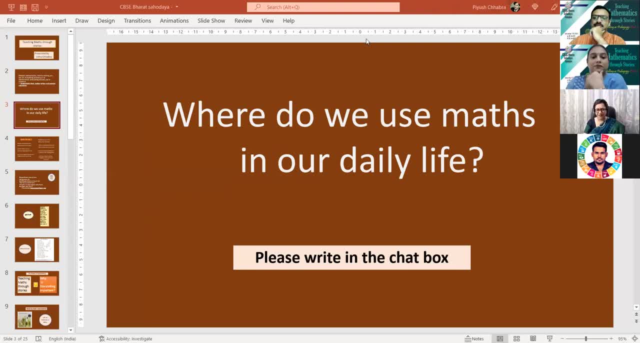 please use the chat. okay, grocery shopping everywhere. time evaluation: okay. marks market shop cooking: okay, driving cutting fruits, kitchen right, yes, yes, yes, yes, yes. making bills travel: yes. shopping traveling. making card: okay. utensils report card: dawn to dusk: yes, maths is everywhere. making tea cooking: yes. science lab: yes. celebrating birthday: wow, great. 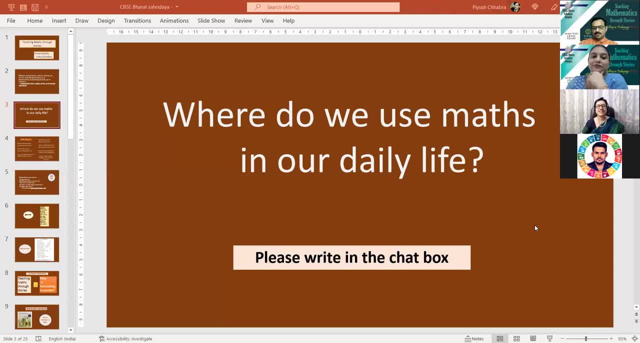 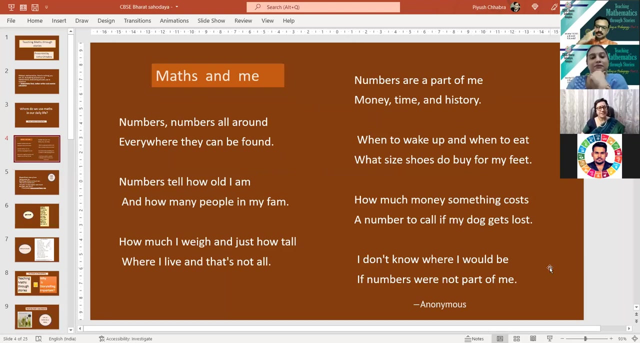 yeah, patterns, yes, budget, yes, yes, you are right. okay, clock, yes, time, even going to school, we are just going with by our watch. yes, yes, yes, yes, great. and now let us read this poem. what does it say? whatever you have written, it's in a nutshell over here: maths and me, numbers, numbers all around, everywhere they can be found. 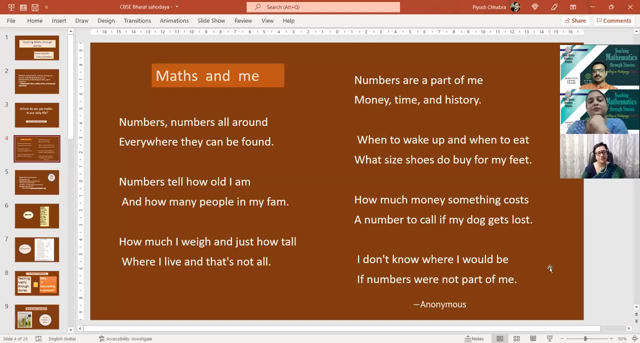 numbers tell how old I am and how many people in my fan, how much away and just how tall where I live. and that's not all. numbers are a part of me: money, time and history, when to wake up and when to eat, what size shoes do buy for my feet, how much money something costs, a number to call if my dog gets. 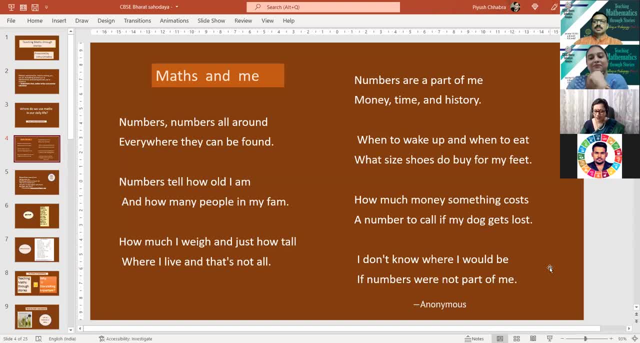 lost, I don't know where I would be when I would be young for numbers. I'm not broke from love. my mom's I would be if numbers were not part of me. yes, the poem also tells us the same thing, that, throughout the day, what not is there which we are not using? where we are having mathematics? 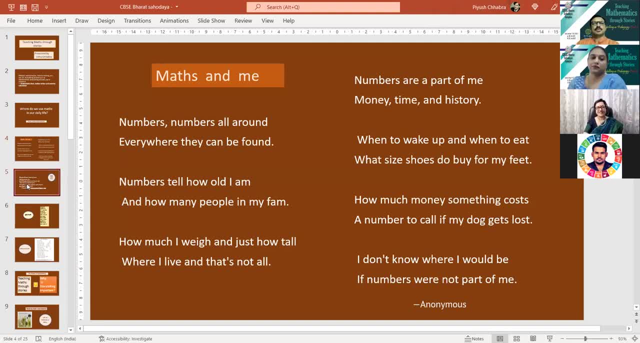 so mathematics is so so important that I can't tell you now. I just want again teachers to just write in your chat box how many children out of 40 in your class love maths. please write and genuine number. I just want out of 40: 15, 20, 10, 20, 10, 30, 21, okay, hardly 10, hardly 7 and 8. 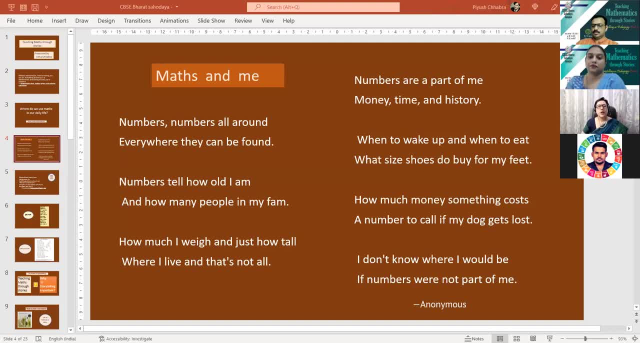 they are liking maths. okay, 20. someone said 40 out of 40. I'm very happy. then someone said only 5, 20, 50 percent, 20, oh, 15, lower primary 100 percent, fine, okay. 25, 100, 30, 18 out of 25, 83, 33, okay, okay. 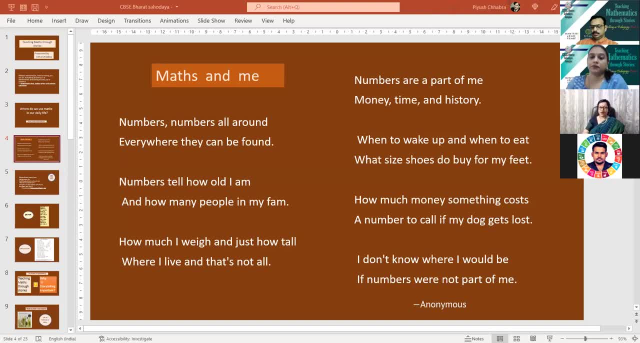 see it's very good that all of them are liking it, but if we are writing 15 percent, we are writing 7 or 8 children out of 40. it means it requires some more attention towards this. what is it what is happening? yeah, when they go higher classes, not like that. okay, depends on the 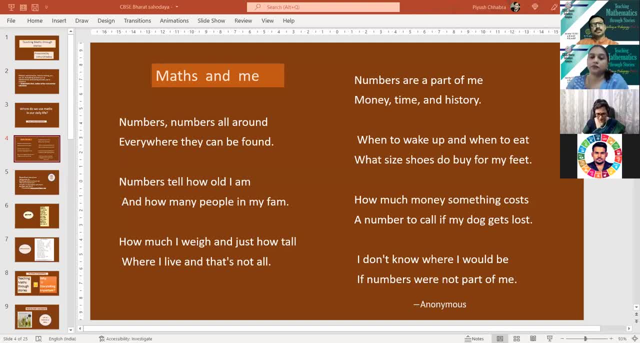 teacher. this is very good that you have written that. Alice George, yes, depends on the teacher, yeah, so here we go. here we have just assembled to understand how I can make my subject interesting, how I can make maths interesting. so it's a big challenge because so many times what I have seen, that 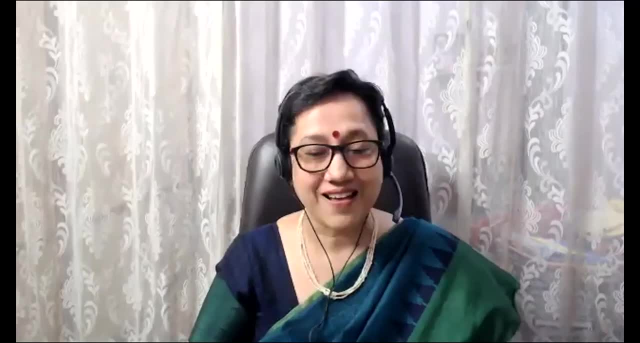 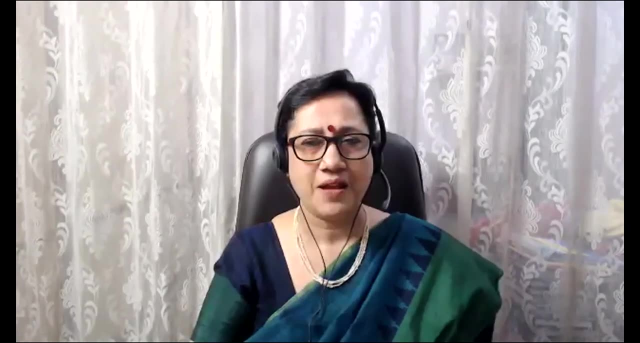 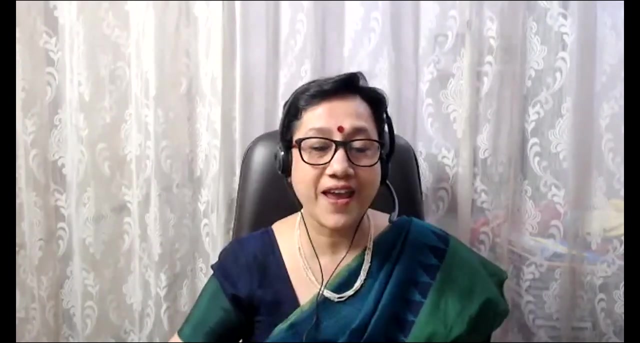 parents. when they come to the class and for the PTM, they always say: ma'am, I don't know what has happened to my child. he does not want to do maths. many of the parents have complained, and so you know, and so you know. unfortunately, even though they say math is good for children, it's still very 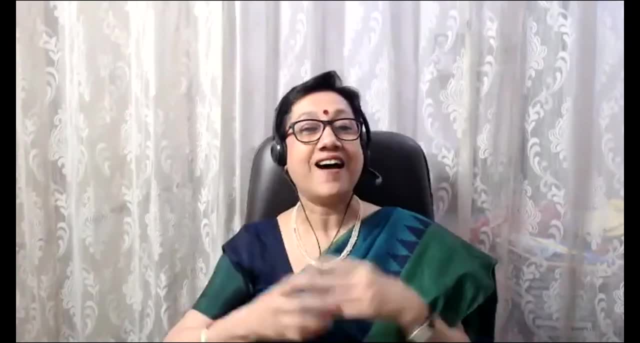 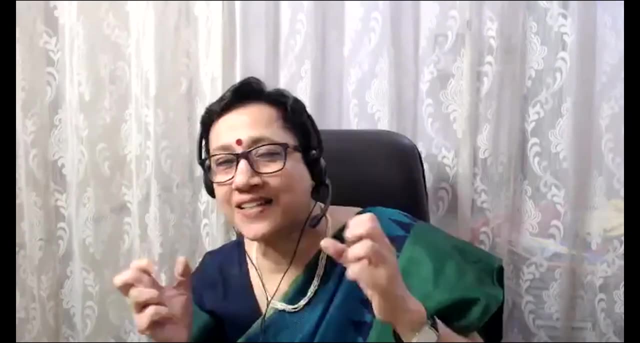 important that you start doing maths, because no one will just pay me the same amount for a year. this is my life. this is where i talk about the nature of this activity of admin. this is what my, my love is. this is the advantage of thisция. so at least that end of the year. 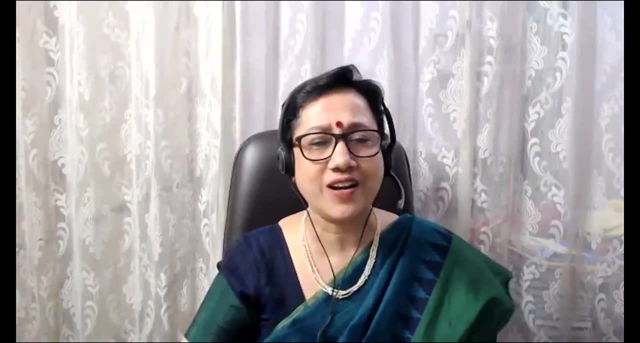 is this to technology working, but at the same time, unless it isiana picking the topic, is pursuing a particular subject. then after the club is out of cad À ceca, I'm just compliant like this long I'm gonna do what we want to model in our classroom, because not only you. 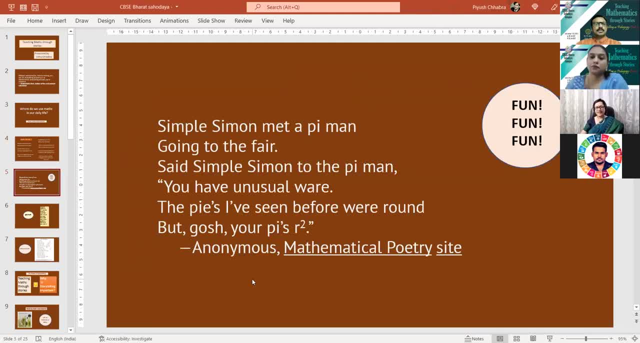 can understand. so that's all if we can do it for ourselves. so today I'm going to talk a about math, math, weirdity. math is the stage: laatulu math. this is that our subject is there when the time table is. Let's see here a small thing: Simple Simon met a pie man going to the fair, Said simple Simon to 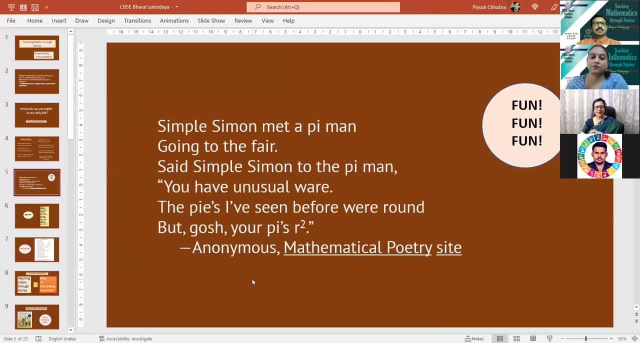 the pie man, you have unusual wear. The pies I have seen before were round, but gosh, your pies are square. So here see, this is also a type of story where two people are meeting and then they are talking. Okay, so children make all this type of poetry, So we can also have poetry in a. 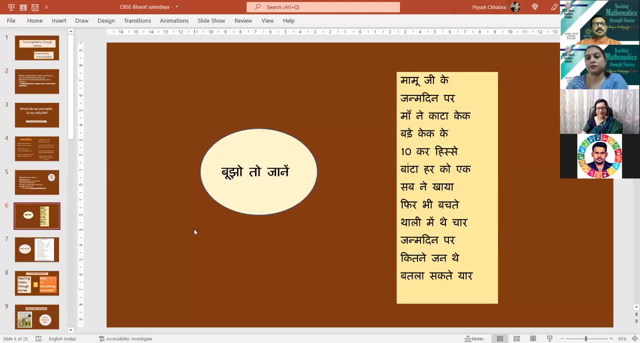 form of story or story in a form of poetry. Either, if someone is there, in Hindi also I can have. mamuji ke janm din par maa ne kata kek bade, kek ke das hisse kar bata har ko ek sab ne khaya. 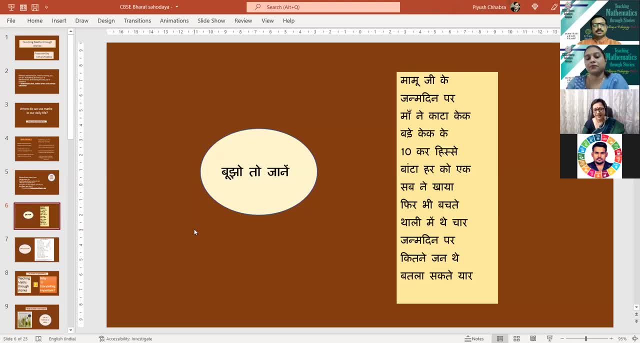 fir bhi bachte thali me the char janm din par kitne jante batla sakte yaar. Now, here again they are asking in a form of: actually it's a story. they have made a simple, small story in a form of a poem, And then 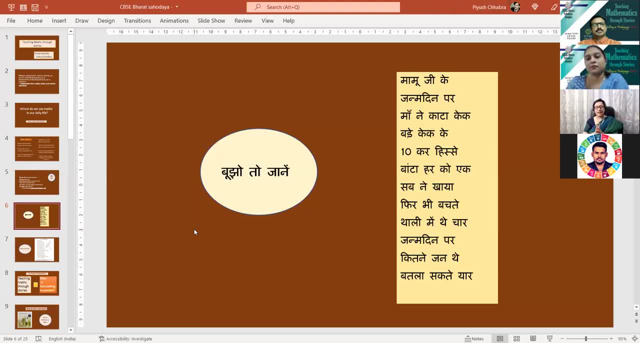 they are celebrating birthday, So- and these topics are always near to the children- So birthday parties, eating pizza or cake, So we can have some of the questions based on this which children like The environment. we have to take into account And whenever we are doing maths with them. 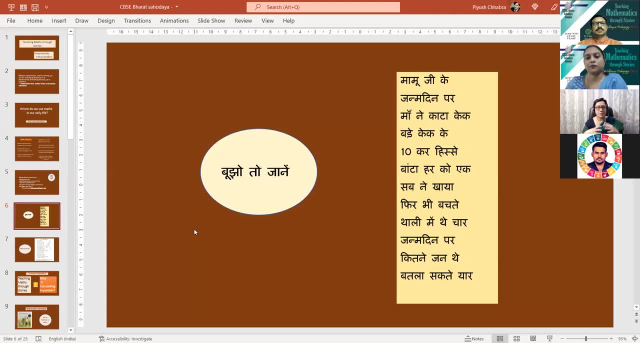 we can just call them: tell me, what do you want? Space, Okay, space And shapes. Then we can just take all these examples so that children are hooked to whatever they actually like. Let us make all these things into poems and stories. Now these are. this is: 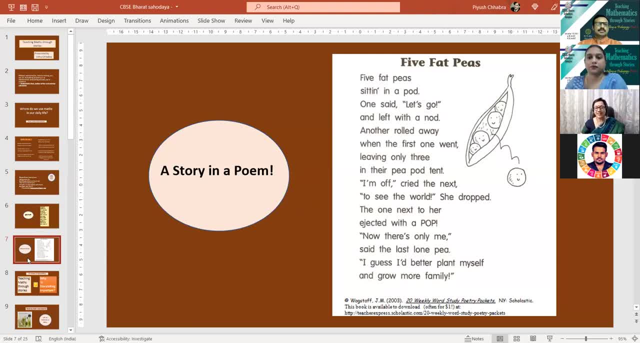 also a poem. Children love to make poems and telling you. So tell them to make a story and then put it in a form of a poem also. So I'm just giving few examples before I start my own storytelling. So five fat peas sitting in a pod. One said let's go. 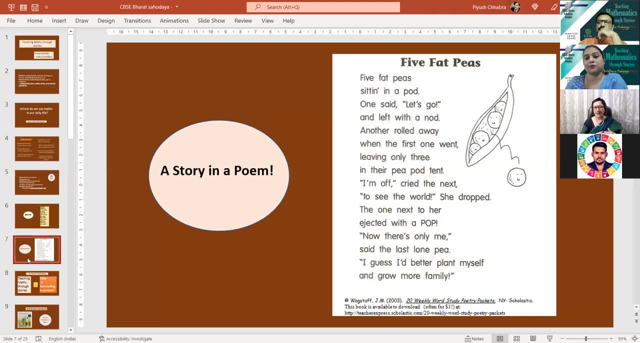 and left with a nod. Another rolled away when the first one went, leaving only three in their pea pod tent. I'm off, cried the next. To see the world she dropped The one next to her, ejected with a pop. Now there's only me, said the last lone pea. I guess I would better plant. 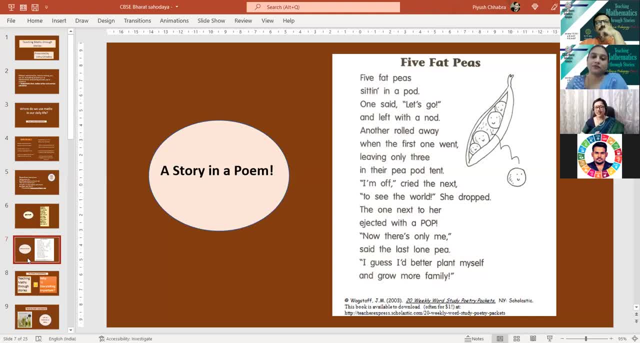 myself and grow more family. So this is a simple story of five fat peas story form. and then they have used one after the other. who is going? how much is left? We can always do this type of storytelling also with a small poem. Start your class with a small poem where there's a small 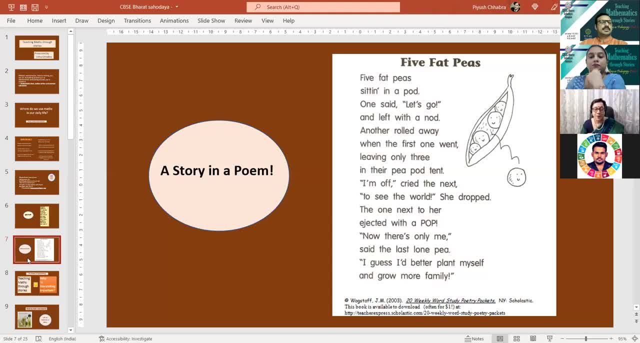 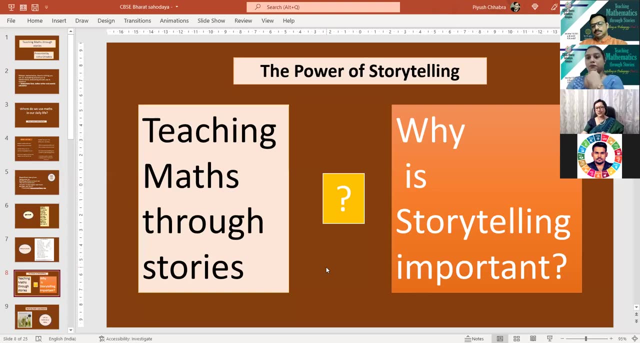 story in that, And then children will just think, okay, we can also write a story from our own textbook. What we will do? we'll make a poem out of the story. So this can also be done. Now the question over here: why is storytelling important? Why are we talking about teaching? 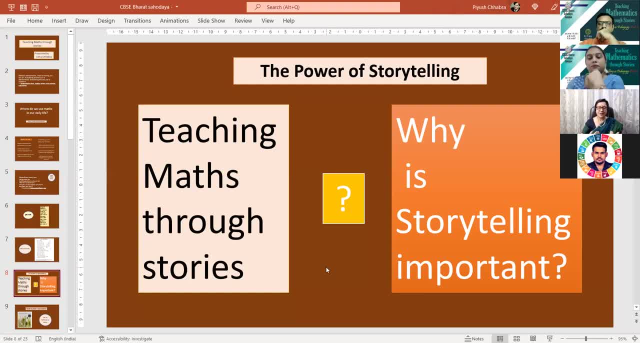 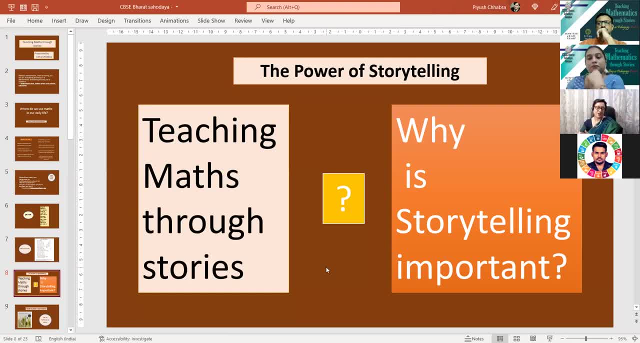 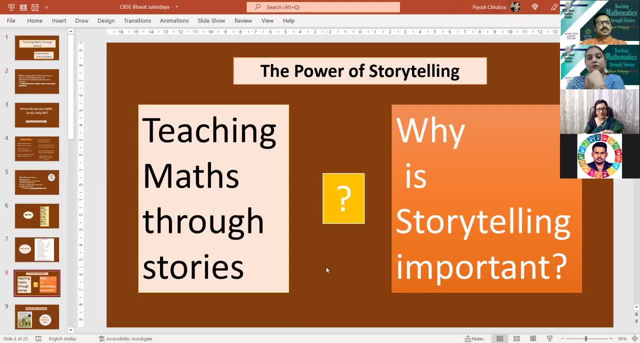 problem. So stories are already there, But, yes, the story should be very much interesting. The problems which we just have in front of children. they are not in a form of a story. That's why children don't take it easily. They find the language difficult for them. So what is it that I? 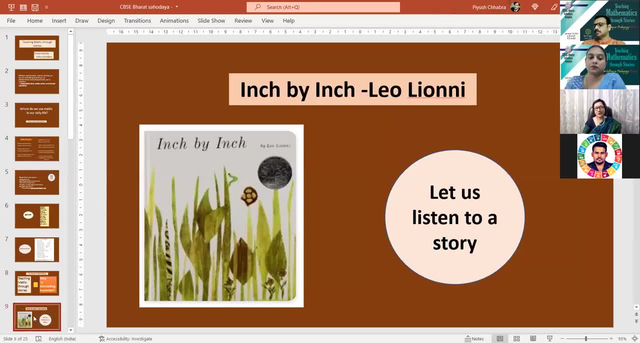 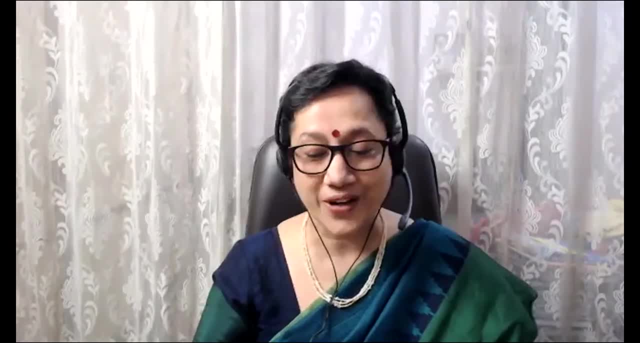 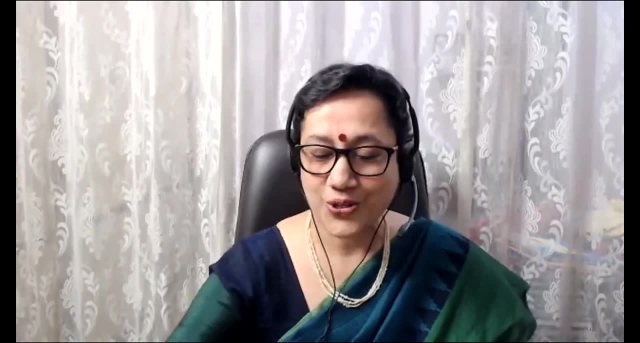 can do to make the story more interesting. What is it that I can do to make the story more interesting, So that children are very much there in my class? So I'm going to tell you a story, a small story. we will see that name is inch by inch. So there was a garden And there was this warm, a small. 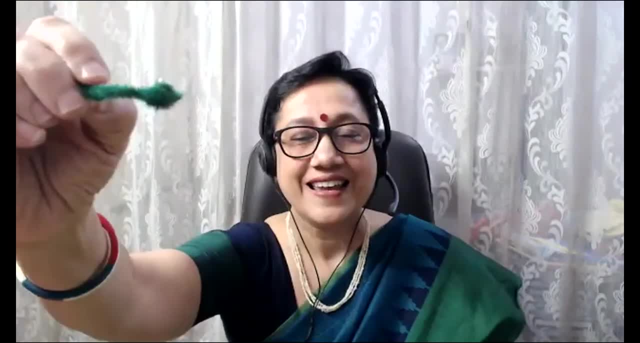 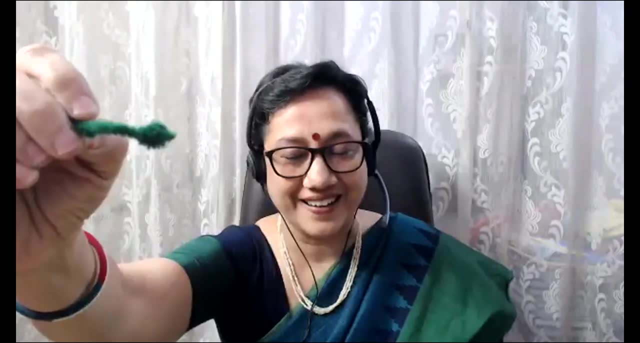 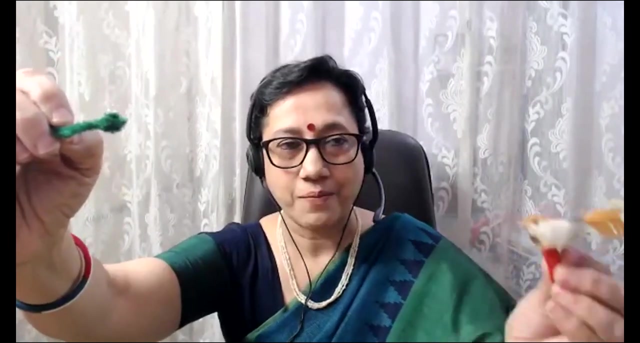 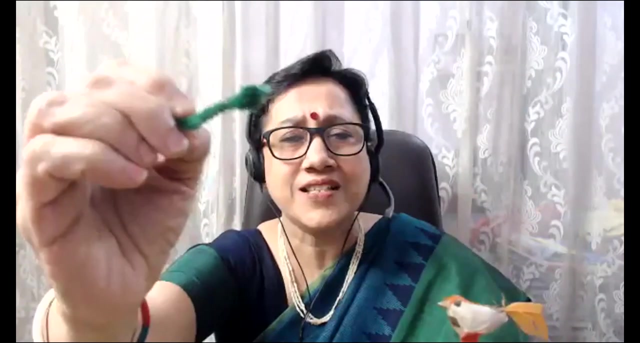 warm and it was very much busy eating leaves. Ah, it's so juicy, It's so nice. I am really oh so happy. and he was busy eating the leaf and suddenly there comes a robin, I'm going to eat you, I'm just going to eat you. No, no, no, no, no, Please, please don't. 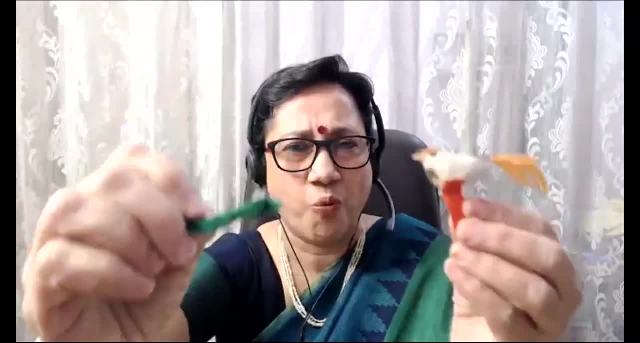 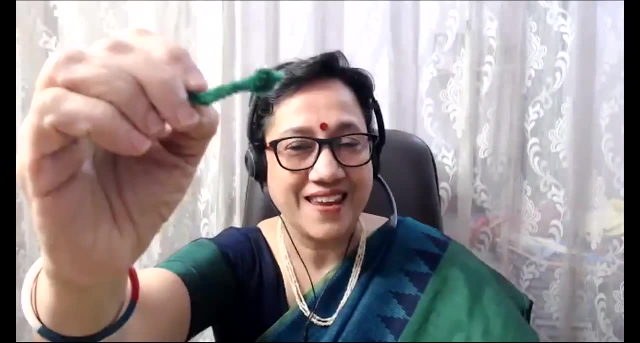 eat me. Please don't do that. I'm so important. What important you are. How? How are you important? I don't see any importance. Don't you know me? I am an inch Inch. What is this inch? I don't know. 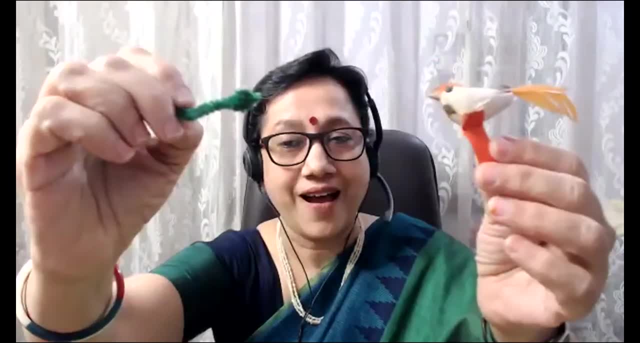 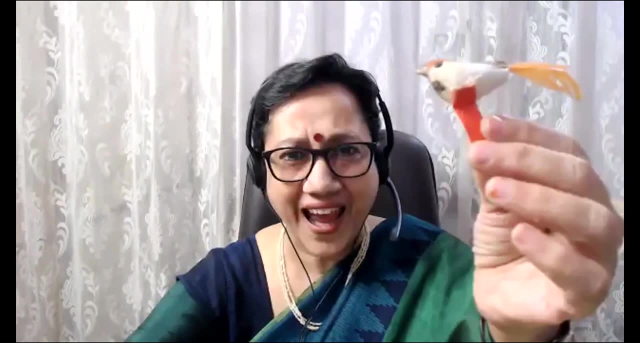 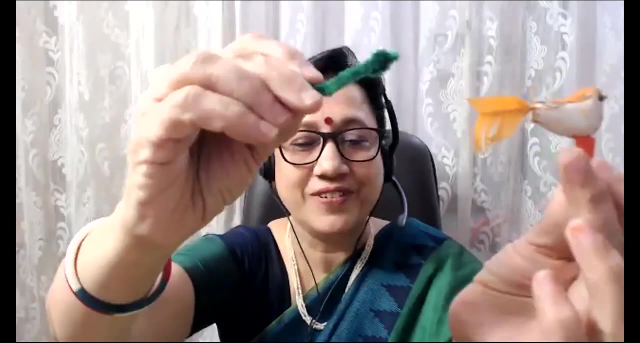 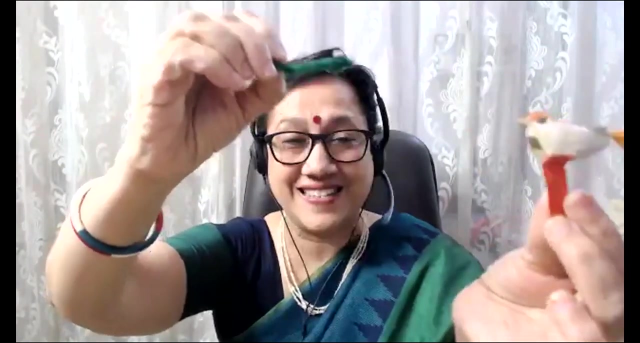 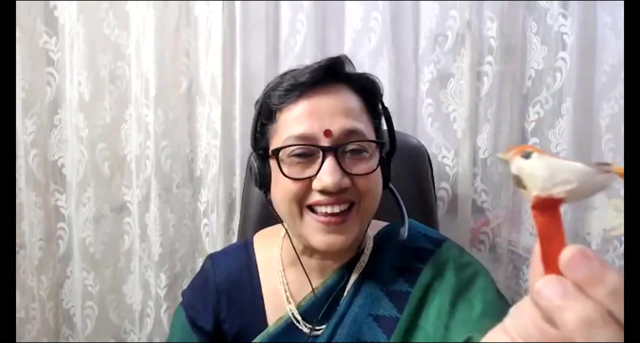 you? Oh, I'll tell you. I can help you to tell you how long is your tail. Is it? Can you do that? Yes, Let me come to you. and then this inch worm comes and measures: Wow, You are just like your tail, is just like me. One inch, Is it true? Really, My tail you have. 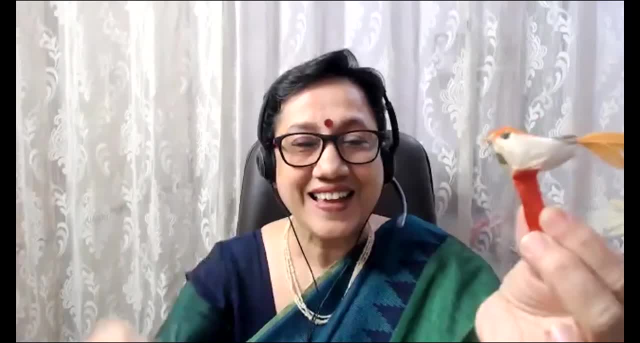 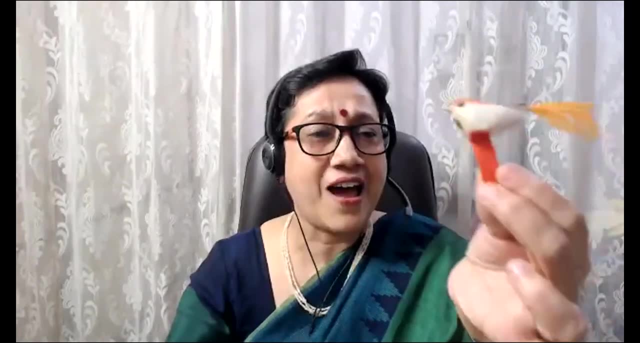 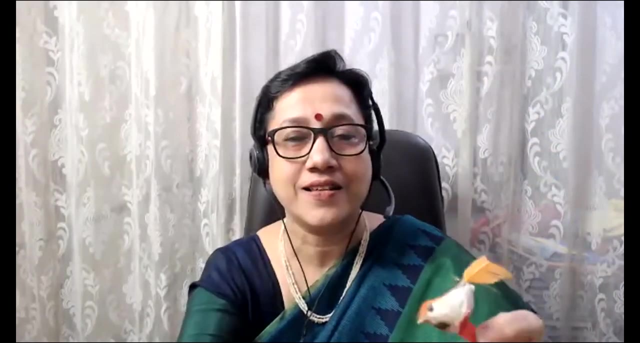 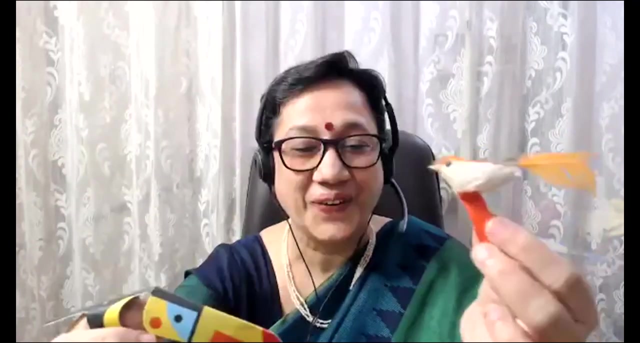 told me that it is one inch long. Yes, I'm telling the truth. Oh my God, I'm so happy. I have a tail of one inch, One inch. And as she was just happily saying this and this toucan came and asked: why are you so happy, Don't you know? You know what My tail is? 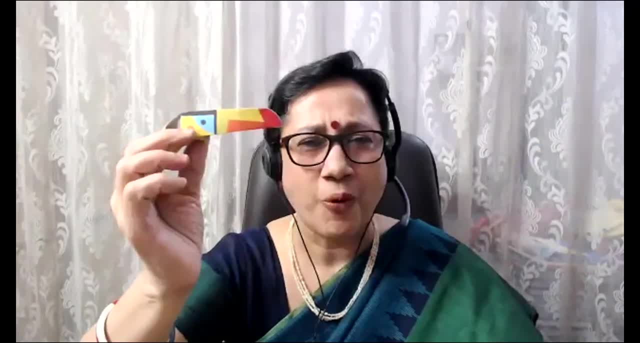 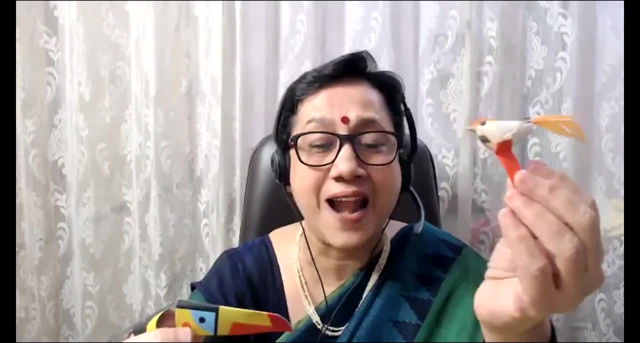 of one inch long. What? How did you come to know? Tell me that There's a worm, I was going to eat it and they said: no, no, no, I can help you, Is it? I will also go to him and ask Worm. 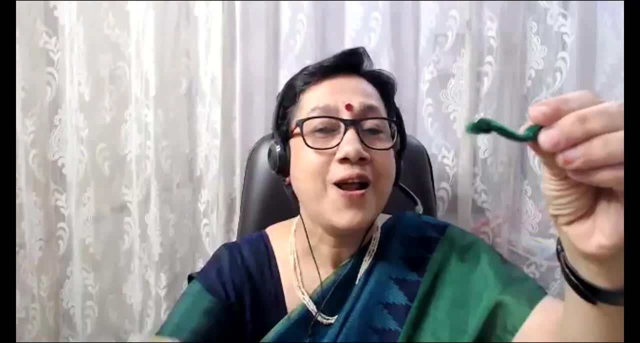 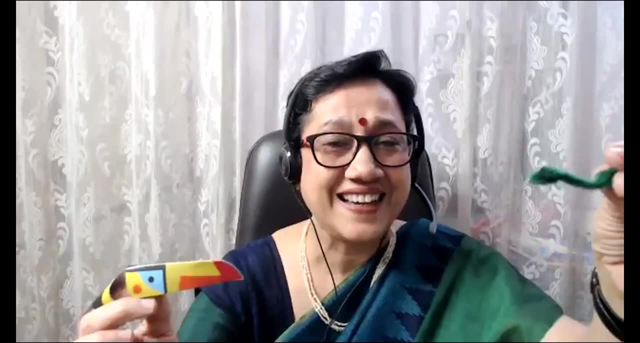 if you don't tell me, then I'll eat you up. No, no, no, no, no. Don't eat me, please. I will help you to measure the size of your beak, Is it? Yes, Yes, yes And. 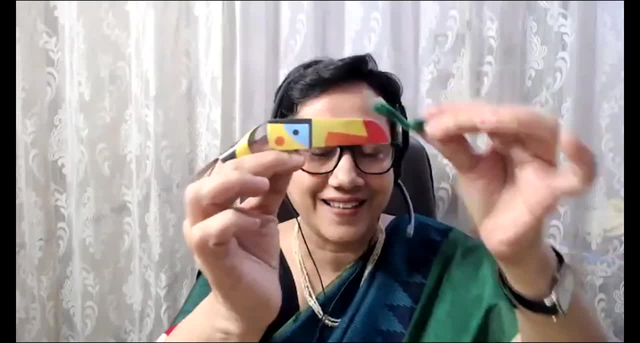 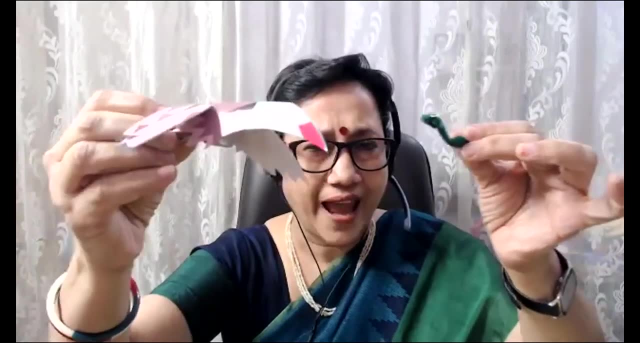 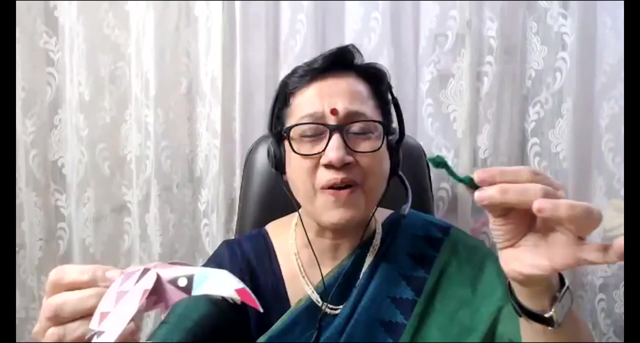 then it started counting one, two, three, like this, And then he was also very happy. And then came an eagle and then said: hey, can you just measure my wings? Yes, yes, But don't eat me, No, no, no, no, I'm not going to eat, you Just measure. 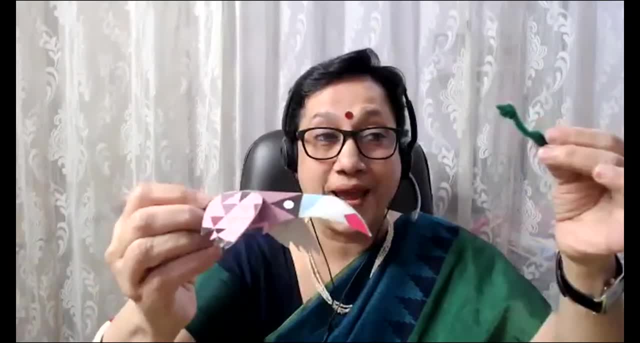 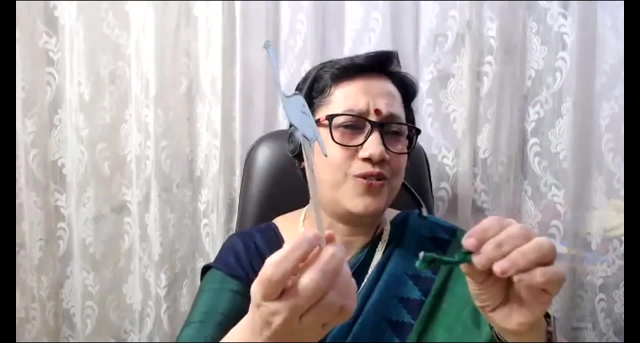 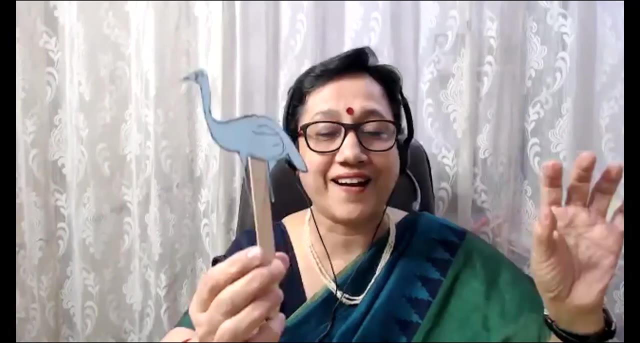 And then one, two, three, four, like this. It measured the wings also. And then came this grain, My legs. they are also too long, Please let me just help me. And then it started measuring this also, And, slowly and gradually, all the words over there. they were so happy that yes. 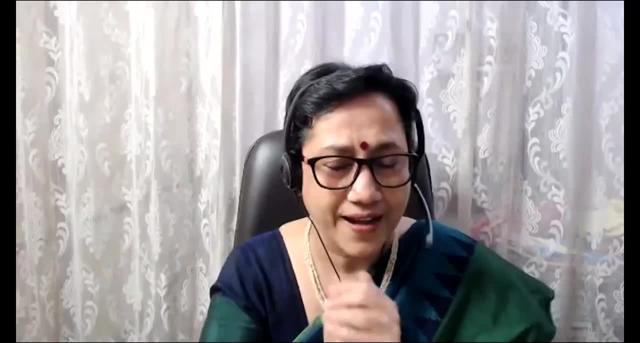 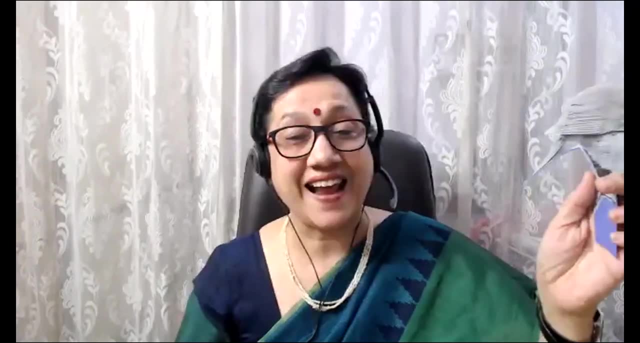 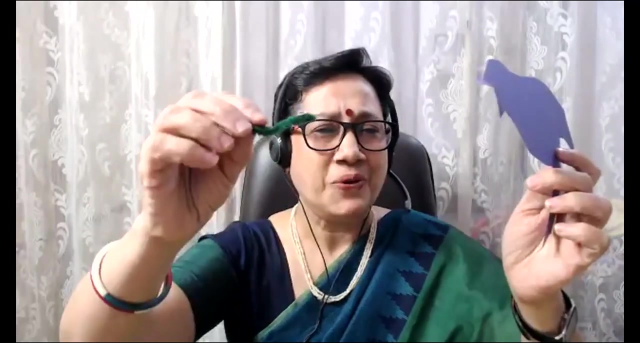 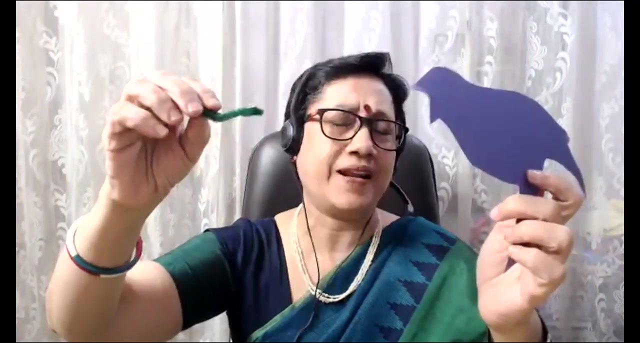 we know how much are each thing measures. And then came a robin. It said this: this came as nightingale and said: I can understand that you can measure all these, But do you know how far my song will be? Just tell me how far people can listen to my song. 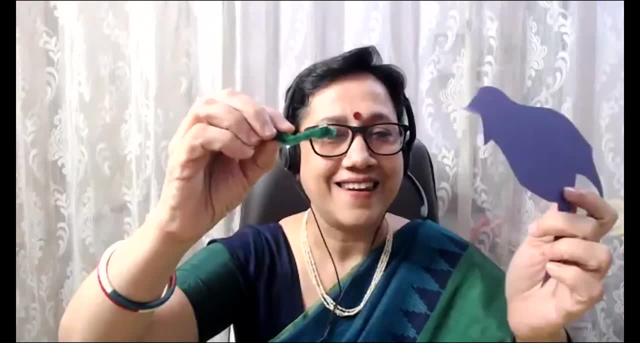 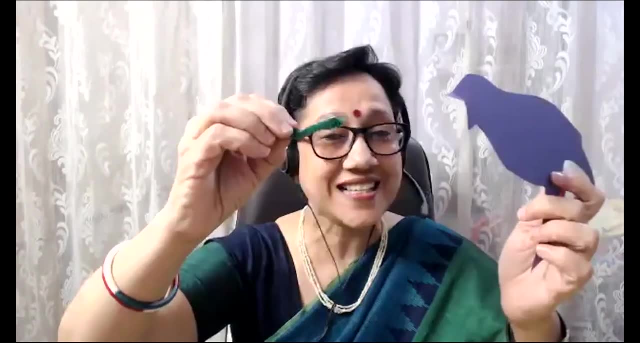 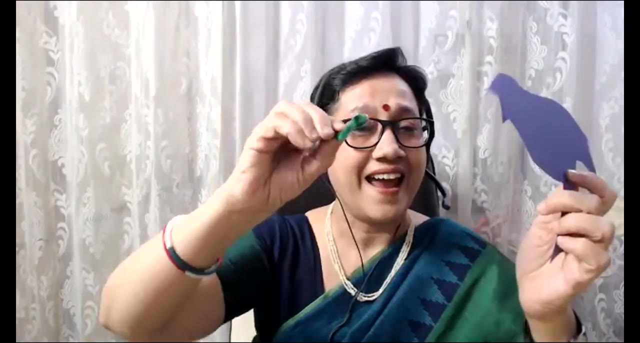 Otherwise I will eat you. And then this inch thought for a moment and then said: don't eat me, I will just let you know. Just please sing, I will just measure it. And the nightingale started singing And inch by inch, 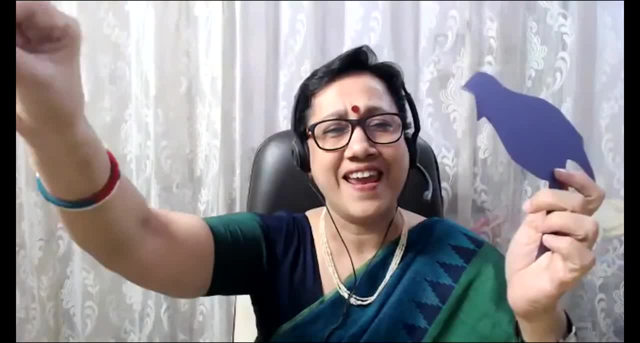 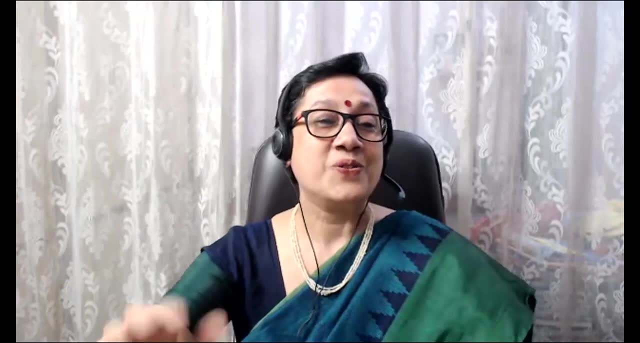 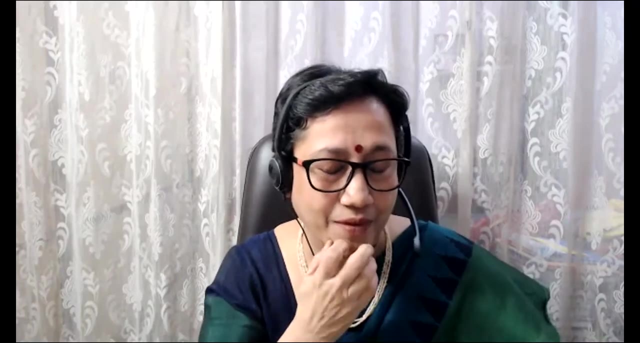 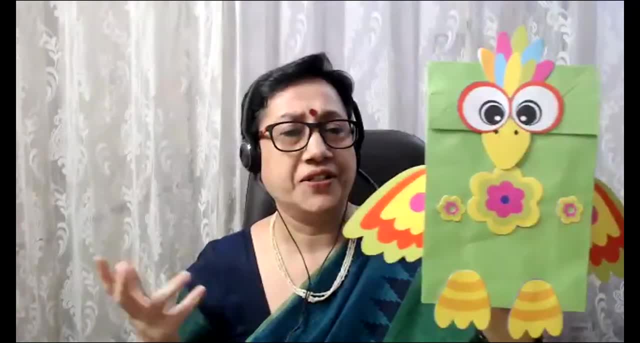 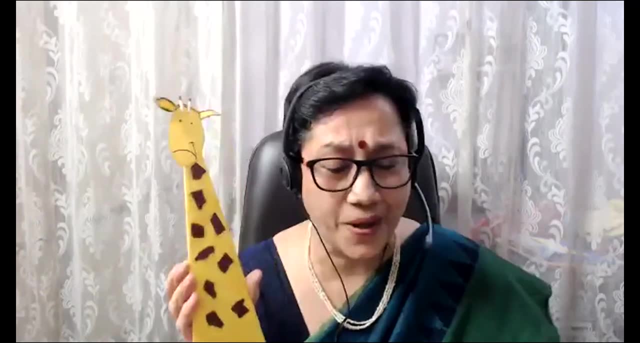 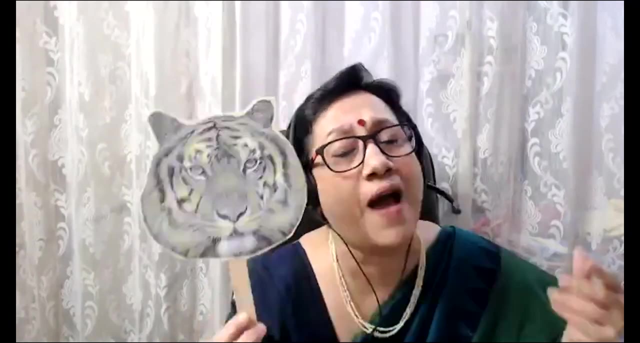 So there and said: now, what about me? Where will I search that From the interval? and then the giraffe also came. What about me? Who will tell this? And then came the tiger and said: yes, what about my tails? And then came this: so many animals, they all. 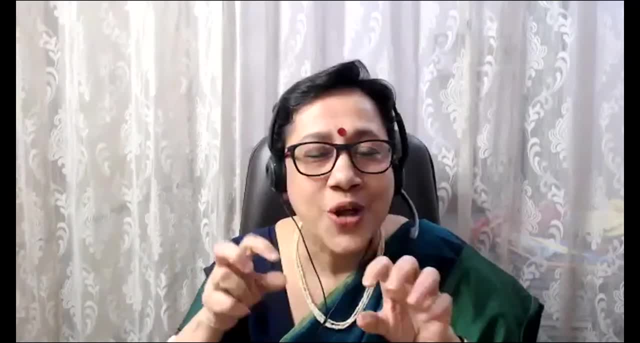 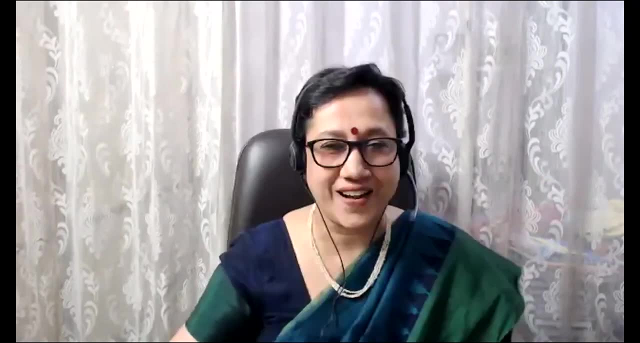 gathered around and they are now trying to find out where the inch has gone. What can I do? Okay, so now I'm being asked if I'm asking you to let me know the answer. Is that what you think? Yeah, Yes. 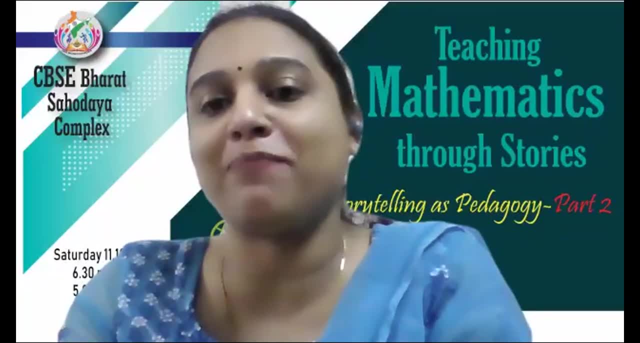 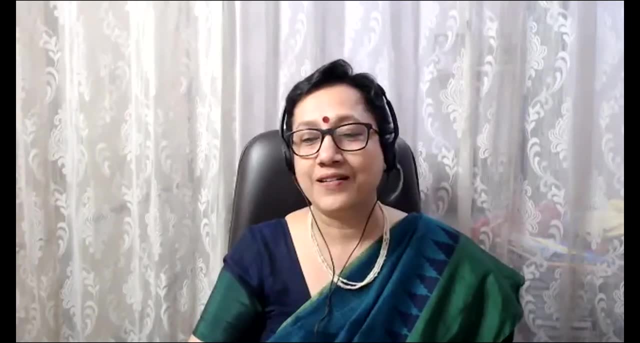 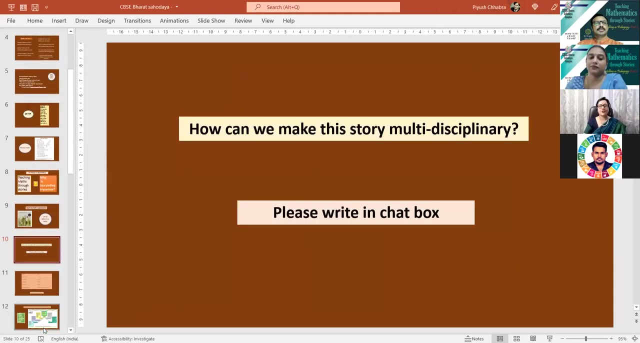 That's not my big scrum of the simmer us on. Oh no, Okay, Thanks so much. You're welcome About that, All right, So yeah, Thank you, そうですね. Today we'll get everything. 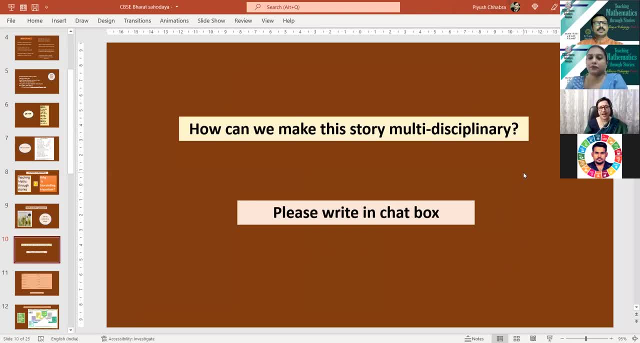 So that's all Um video. I think, Yeah, multidisciplinary. please write in the chat box. i just want to know how. but how will you use it? where will you use it in the classroom situation? for what measurement? food chain character- okay, pre-mass teaching measurements- addition. 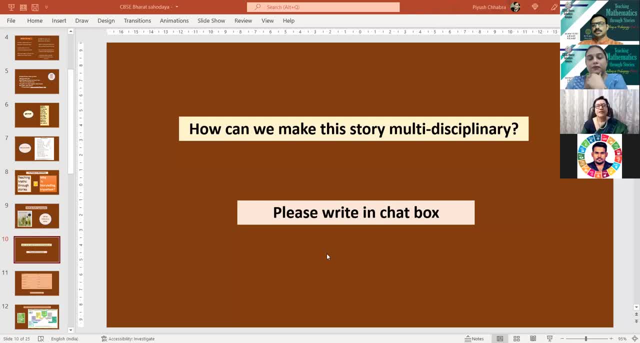 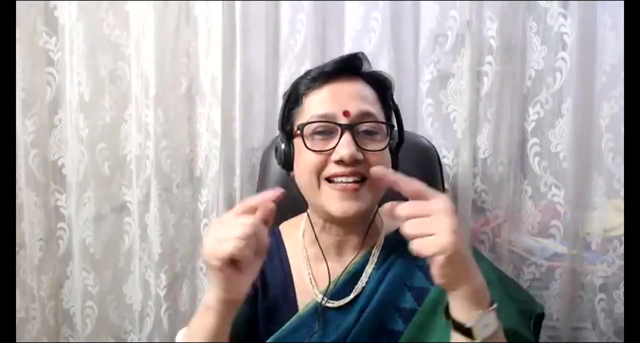 grouping: okay, okay. okay, measurement and multidisciplinary how we can do it: yes, counting word problems: okay. value education: okay, how we will discuss now. yes, measurements, okay. okay, just let me know how we are going to make it multidisciplinary. comparison. biology: okay, anyone can unmute and speak. 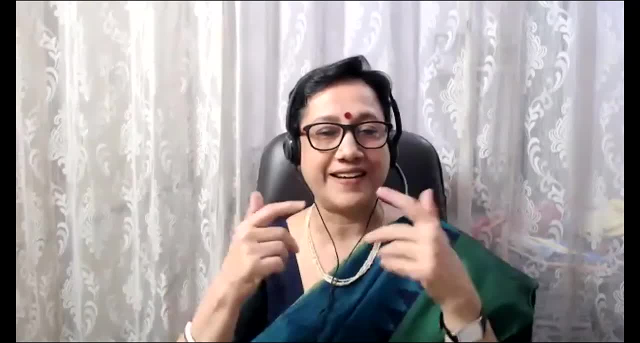 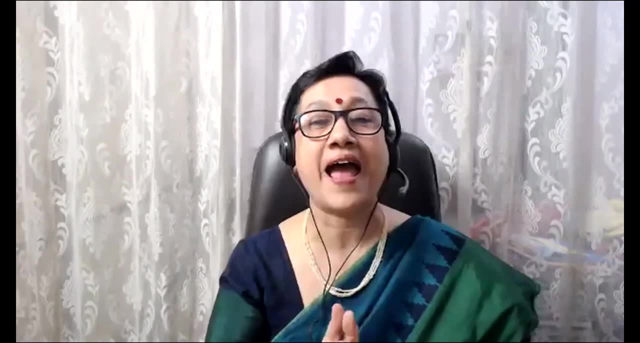 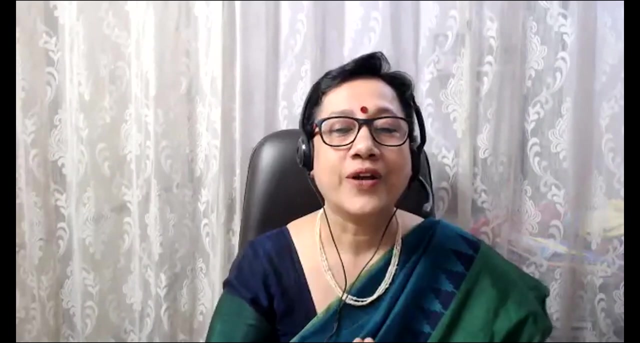 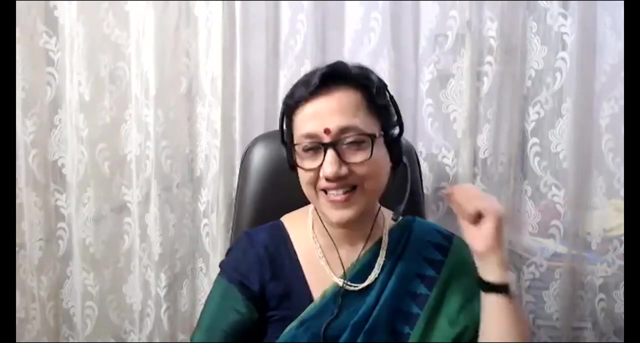 i will like to know from you how you can do it. multi-disciplinary: okay, you are writing. i understand someone who can write with biology sequencing. english ssc map: yes. english story: yes. yes, anyone who would like to say something? okay, environment science- okay. science with feather: yes, feathers and birds. so so many things. so this is the main thing where 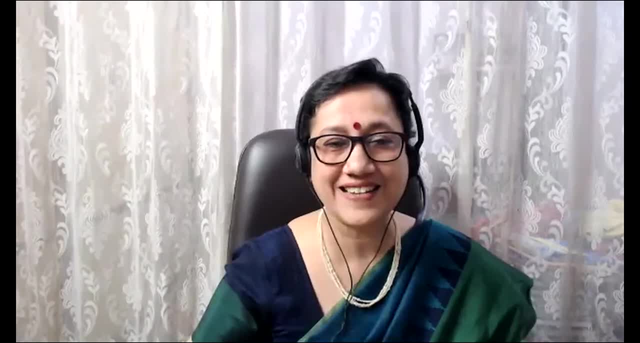 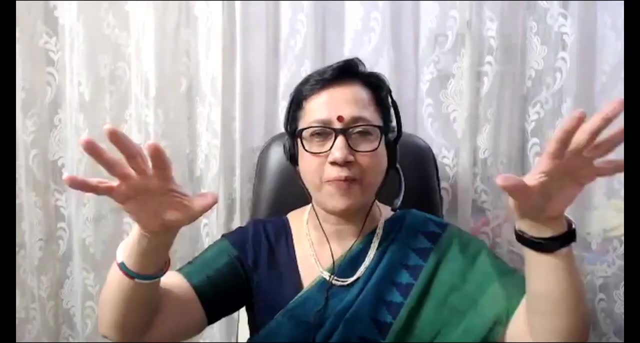 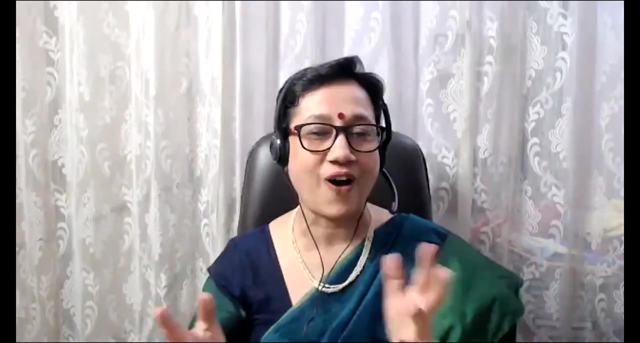 the nep 2020 also says the thing right. so we have to understand, with such a simple story, multi-pronged- are you getting my point with some one simple story? if we do it in class two or class even class five also, if you are doing ecology over there also you can do this and then you can connect with. so 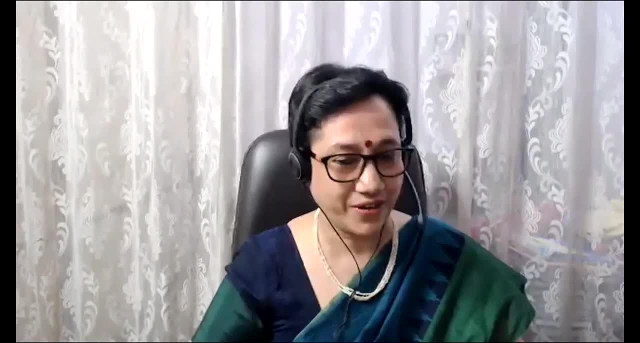 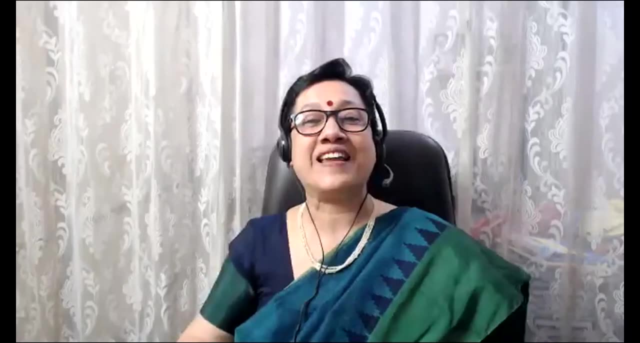 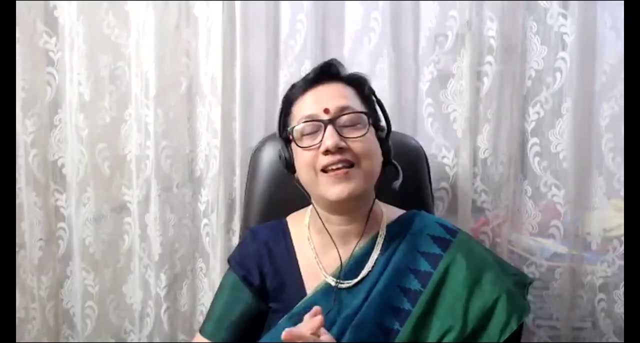 many things, even comparison measurements. whatever you are saying, you are all correct. english science, yes, so many words, yes, yeah. yeah, this is good for being clever. the worm is clever and he knew that. what if i go away from there? then it's better, because he is getting tired by just measuring people, right, okay, cross. 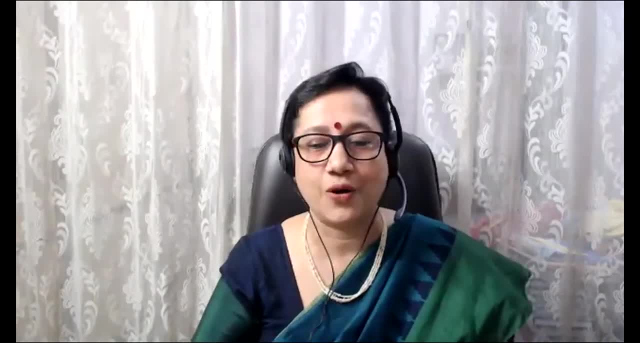 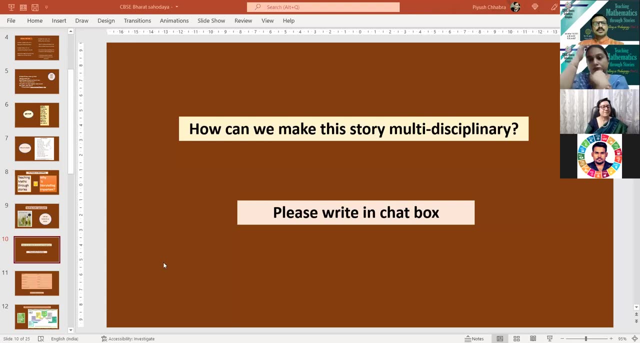 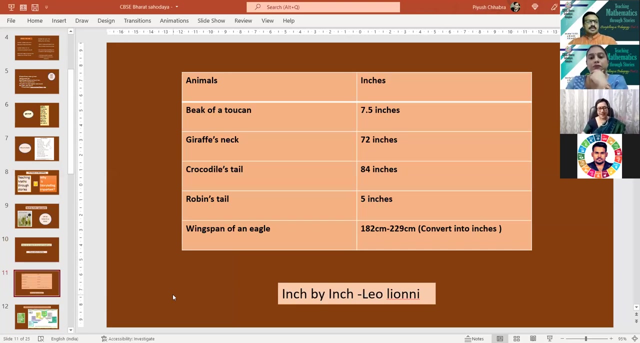 links with science. okay, you can't unmute, no problem, so i will now move ahead. okay, so you have already understood. see what i have done. this is also very good exercise that you can do like: what is the beak of a toucan, then giraffe, snake, crocodile. 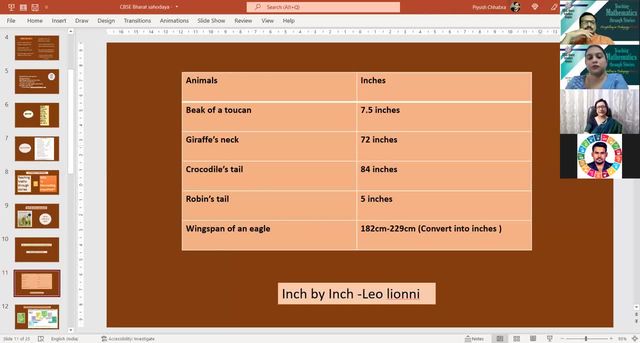 see robin's tail wingspan of an eagle. now what i did? i went to the encyclopedia and try to find out this so you can ask them to find out from of different animals. whatever animals you are doing in the class, you can do that way also, so here we can use and even converting into inches. 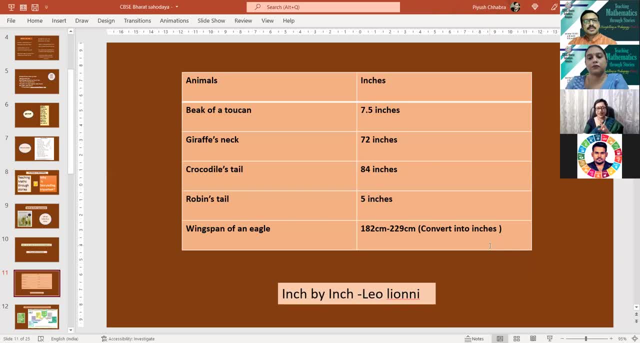 we're gonna learn disciples in texas. sometimes they're getting into centimeters, sometimes they're getting into centimetres, so you can tell them how much types of animals in each class can you answer, So you can tell them what is the relationship and how inches and centimeters are connected. 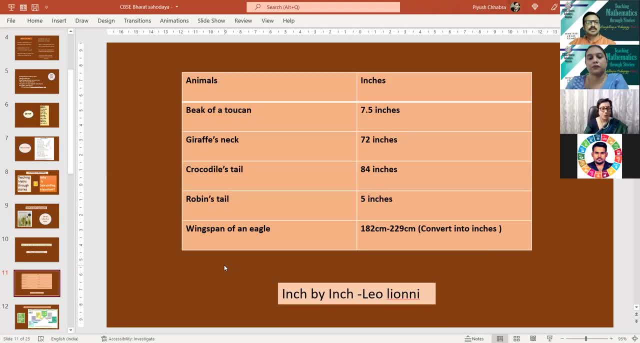 So this is also there. Even then, when they know about inch, now how many inches the table is there now, chair and the blackboard, or your copy, a book, anything that you can relate to. So it's a beautiful story, multi-pronged, and it's so interesting. 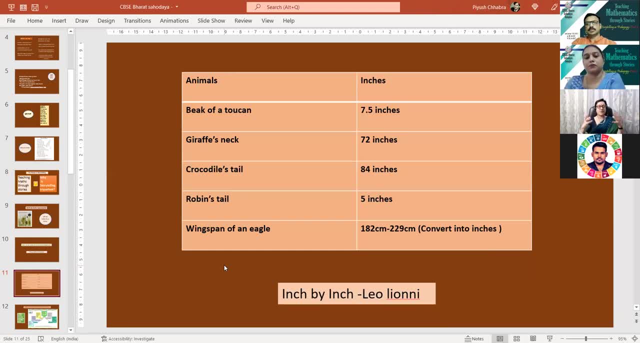 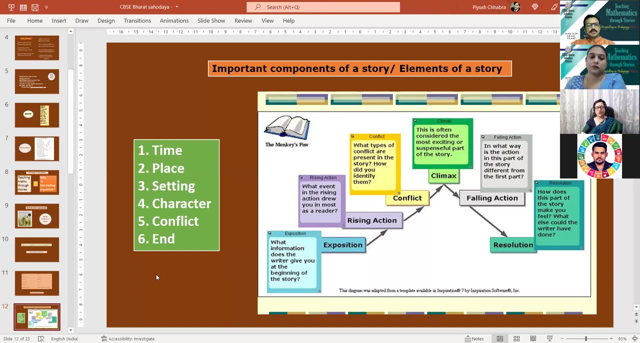 The cleverness of a worm also. So all these things, when we take into account the classroom, becomes interesting. Now you can also tell children to make their own story, So I'll just first come to you with this Now important components of a story. as I told you that you have to just give, see whatever problems you are getting in the book. that is only a bone. 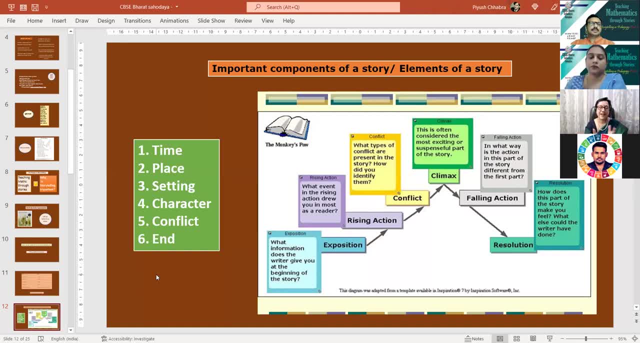 So you have to add some flesh, as I have added. What did I do? I changed my speech. I just, like you, can say: posture is there, Then voice modulation is there. How I'm starting, What is the time, What is the place setting character? 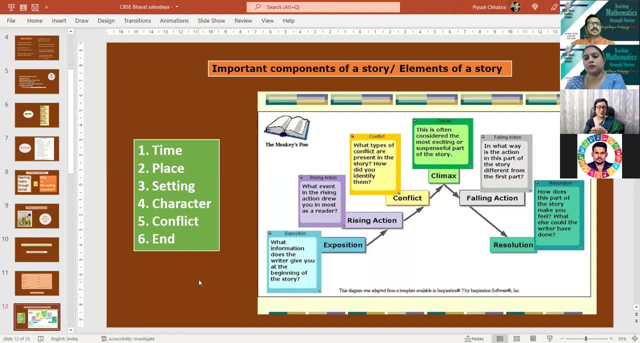 Then there was a conflict that everyone wanted. Now he also wants to go away, He's getting tired, This is also there and everyone wants to eat it up. So this is a conflict and how it is now helping them out, And then the end is there. 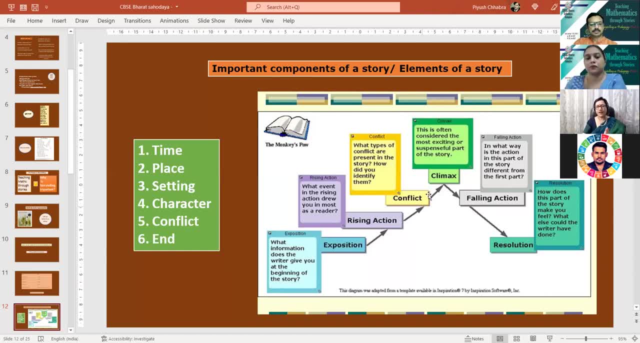 So there is an exposition, Rising action, conflict climax, falling action, resolution. So when you are making the story, just remember these things: that this, it goes like this and then ends. So this is very, very important for making the story interesting. 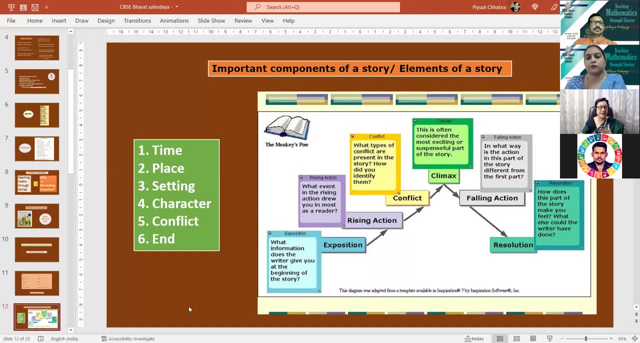 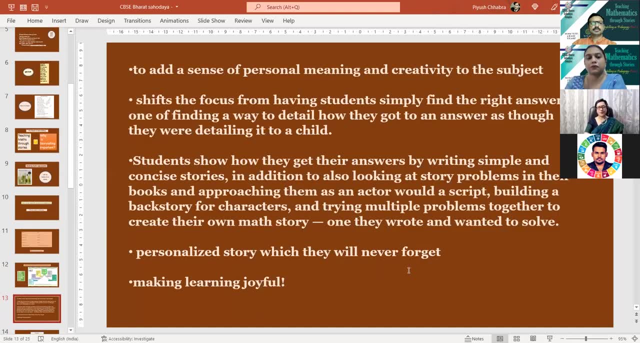 If there's no struggle, then the story is not very like liked by children. You can see that way also. And now let us see this. So what it did? to add a sense of personal meaning And creativity to the subject. So what did the story do? 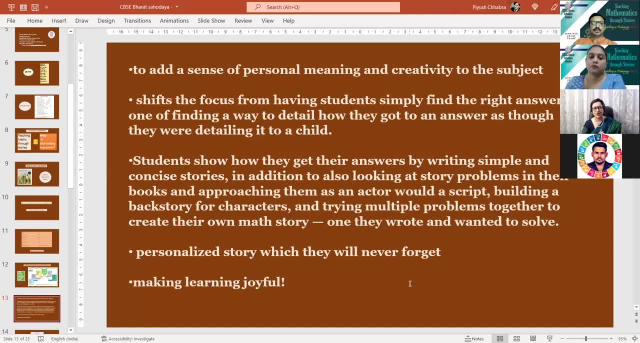 It shifts the focus from having students simply find the right answer to one of finding a way to detail. They're adding the detail How they got to an answer as though they were detailing to a child. Students show how they get their answers by writing simple and concise stories. 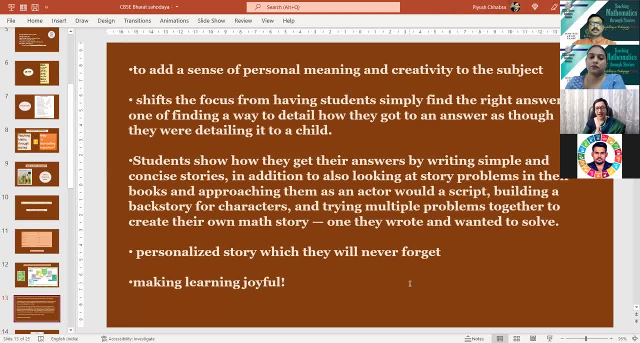 In addition to also looking at story problems in their books and approaching them as an actor, would like us to write a script building a backstory for characters Trying To create their own math story, one they wrote and wanted to solve personalized story with. they will never forget. 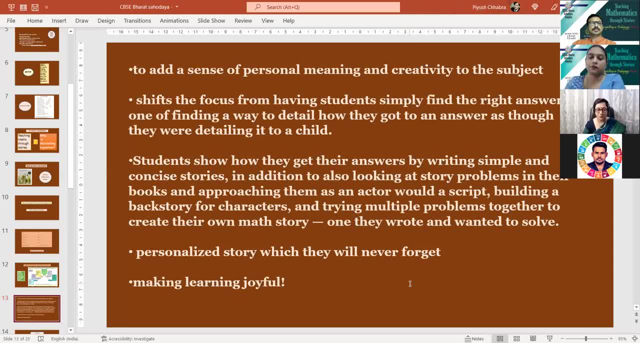 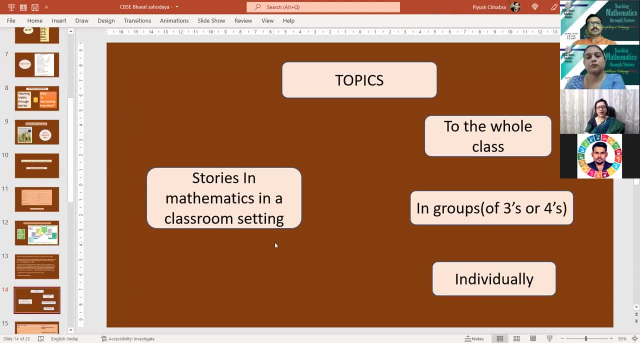 Now, if you give them some of the topics and you ask them to make their own stories, they will never forget, So making learning joyful. So how we can do that in the class Like stories, how to do it like topics, you have to get whichever topic you have done in the class. Maybe you have shown it to the whole class. So how we can do that in the class Like stories, How to do it like topics: You have to get whichever topic you have done in the class. maybe you have shown it to the whole class. 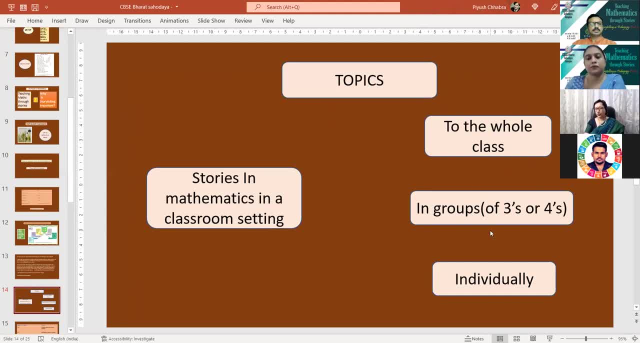 once. okay, now you can divide them in groups of threes or fours and you can say: now this is the same topic. now you have to make your own digits, make your own story and you will see how they are doing. then you can also give them individually. each and every child will do their own story. 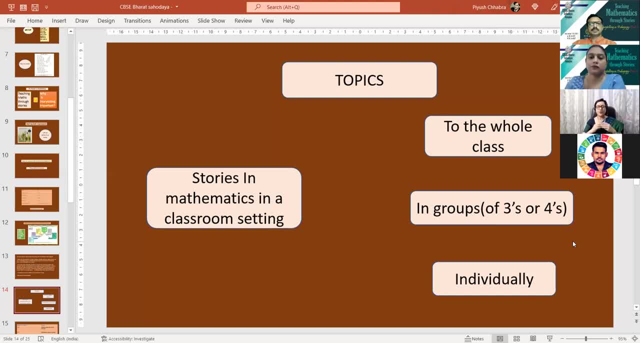 but here i suggest that in lower classes mostly we give in groups so that children come out, and there are some children who are not very good at doing it, so when they are sitting in group they feel secured and then at that time they can write in groups and beautiful stories they can. 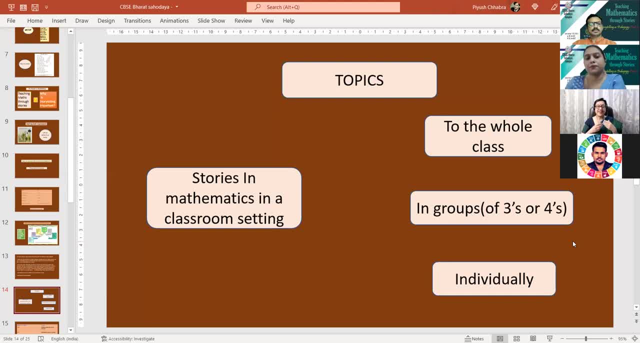 come up with and they can enact. also, they can enact and give voice modulation to it and expressive it will be and they will never forget. so the process of learning is important, rather than getting the answer in the primary classes. so once they are used to making their own stories, they can write in groups and beautiful stories they can come up with and 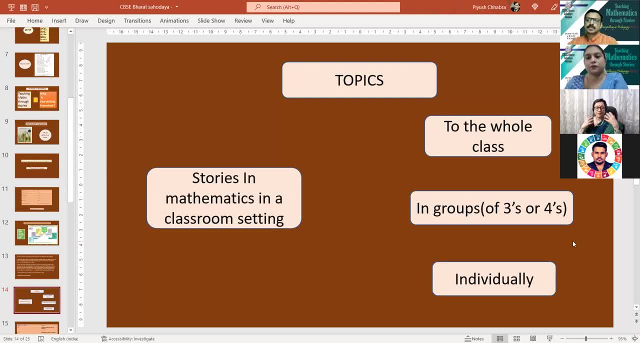 if they are making questions on their own, the problems are making on their own in the form of a story. they will just enjoy your classes. ma'am is coming, she is going to give us this time and we are making a good, nice story. so if they are peeping out of the classroom of the door, that 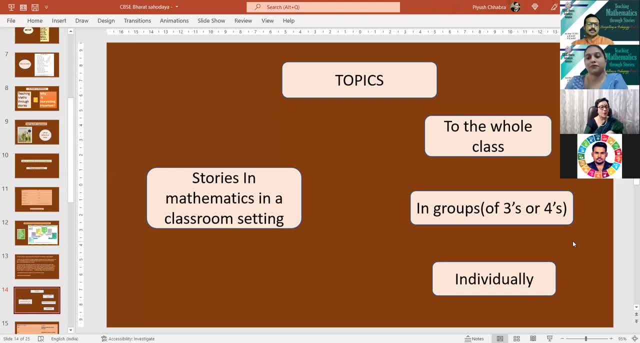 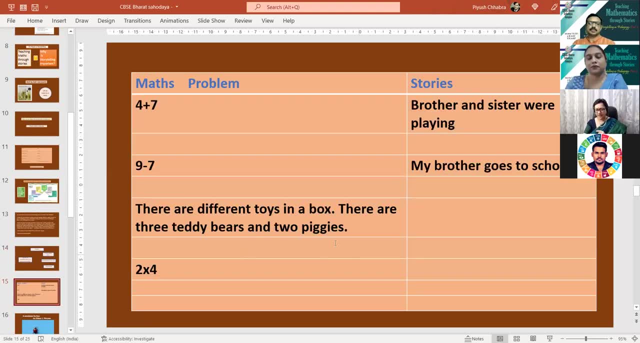 yes, ma'am is coming and they are happy. it means you are going in the right direction. so here also we can have like see, i have given one example. that math problem is there four plus seven? and here if we are asking them, just write down what is it equal to, so it's better. what if i ask them: four plus seven is equal to something, it's better? 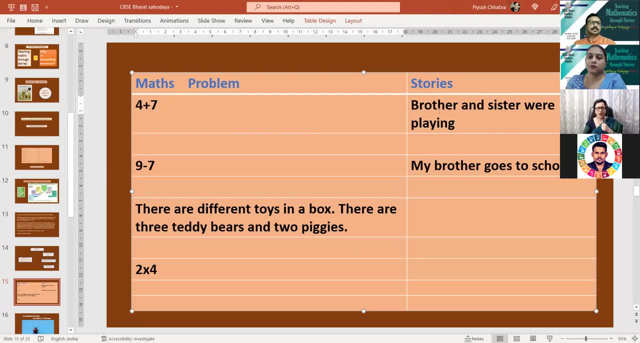 than we ask them to make a story. anyone over here can just tell me, brother and sister, they were playing together and then something happened. i don't know you have to make a story here- word problem, but you have to make it nicely. four plus seven: how can you do this addition with the help of a story? who will tell me? anyone can write in the. 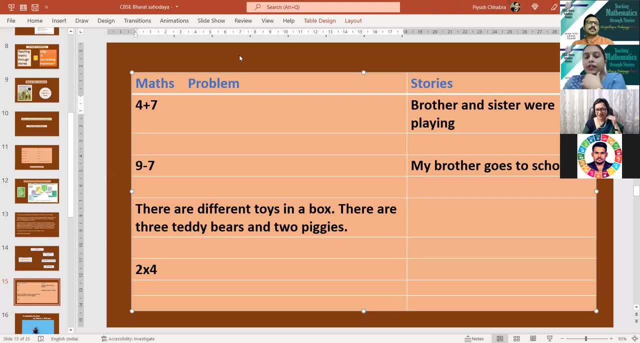 chat. participants can write in the chat. i can give it out for you or for ushama. yeah, yeah, just write two, three lines so that i know. okay, but, brothers and sisters, even not only this, you can also have your own story four plus seven. but it should be interesting. 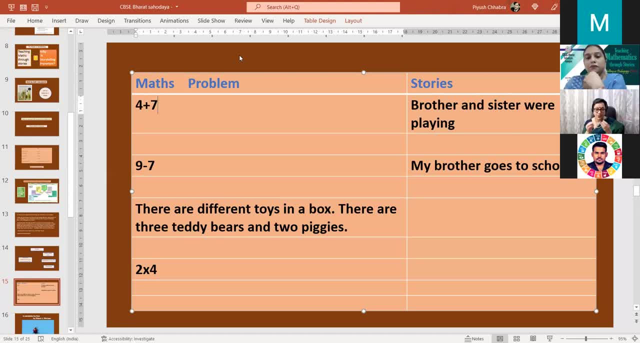 whatever the uh children like, use those things, like children like birds and in this, in this way, you can use your own examples. uh, four cars, okay, four cars, four cars plus seven, yeah, yeah, yeah, i can read. yeah, yeah, yeah, brother has four toys, sister has seven toys, uh, and if we add four, 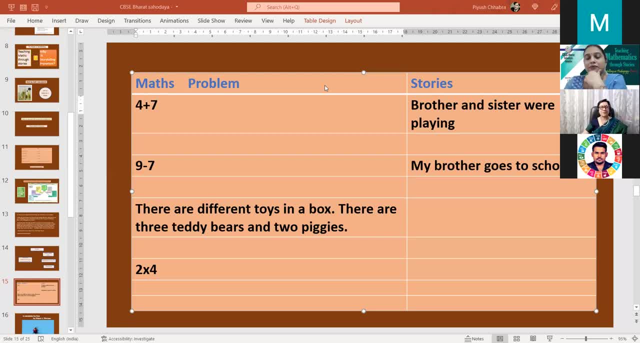 more to it, like the uh, once a brother was playing with his own toys and he had maybe four- yeah beats four- shells. so we have to improvise upon our story also, not like this, that they have four bats and three bats. it is very simple, in the the same way they write it, but we have to add some more thing. 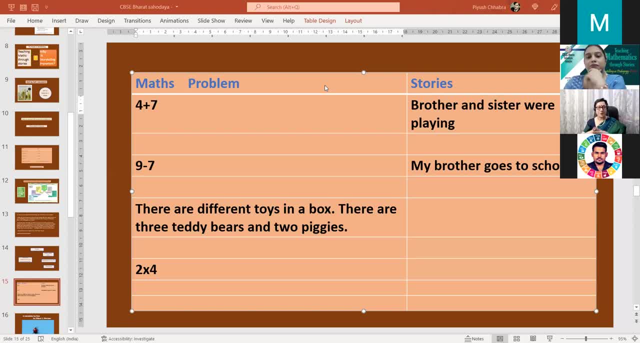 something more like four toffee, seven dollars. no, but you have to add, maybe there was a birthday party and then they got the prize so that children get interested in that. i mean to say see, simply, if you write have birthday event, then if you are writing, uh. 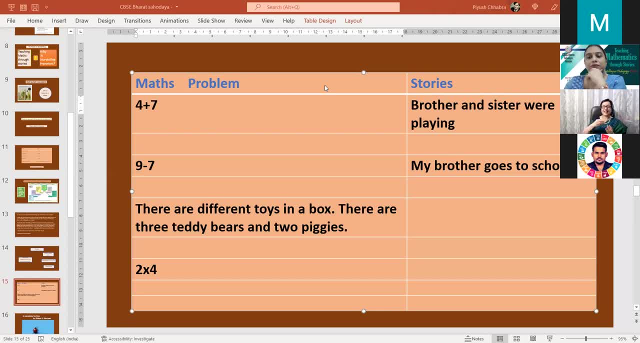 pranali, you are writing birthday event, so you have to describe the birthday. even so, it was a birthday party, it was so good, everyone was there with the gift and all this. so please add yes, yes, rakhi festival. everyone was happy, so many rakhis in the house. 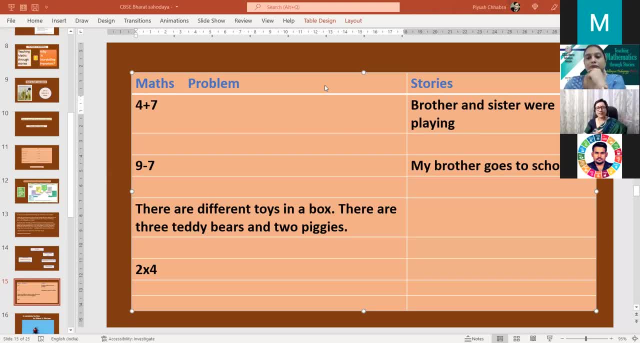 unboxing the gifts. okay, yeah, mother cooked for diwali, yes, so what did she cook, cook? and then you are adding some flavor to it by adding, maybe idli dosa vada and this: so many dosa, so many vadas like this, similarly, for multiplication, similarly, but if what, i 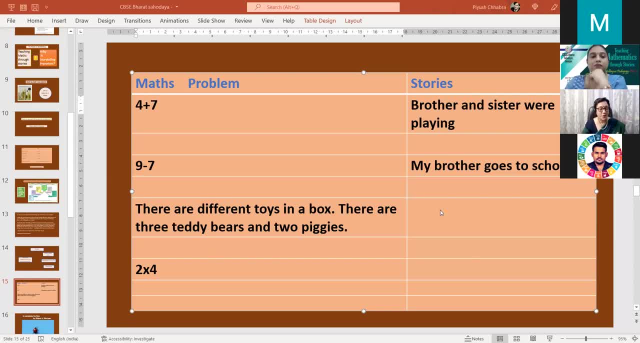 mean to say you have to understand that the stories, yes, laddu, as you said, laddu, children- it is a favorite of children. but your story should have some more flesh, not like simple bone structure, that four toys and seven, maybe balls like this, not like that you have to give. 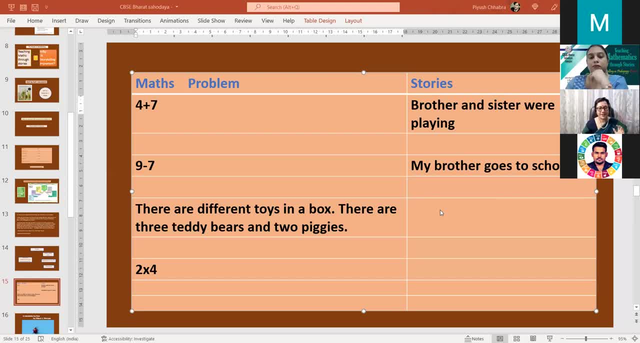 some atmosphere, some environment. you have to put it there so that they there are different toys. in a box there are three teddy bears and two piggies. now maybe we can say that later on. then, what they did, what they did, they gave it to someone who was in need, maybe some child who was there and who was 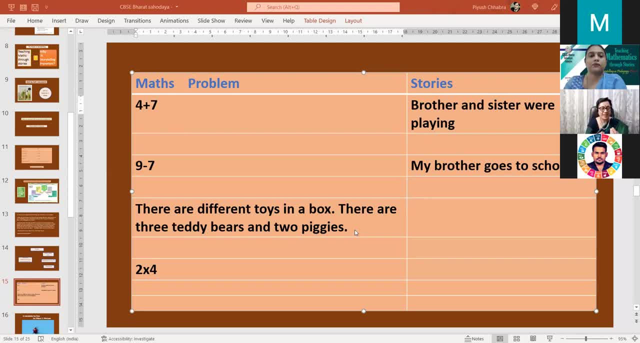 just looking for some kind of a but because there was no product in that box. so maybe you have to look at that and you have to give it to the people who are getting them the table. what he did they gave it looking at the toys. he never had played with a toy, so at that time they gave away their one, teddy. 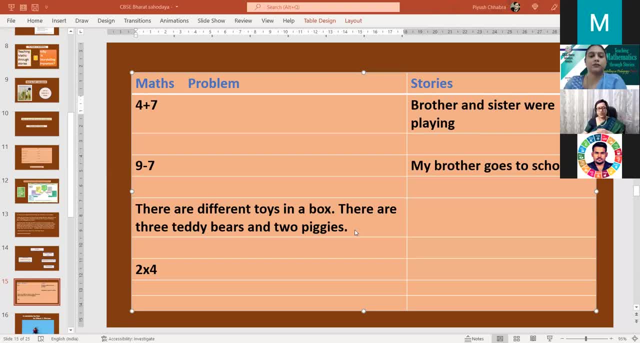 bear and one piggy they gave. so like this. so i mean to say your story should have some more interesting thing, not simply writing that four chocolates were there and how many now sweets they have not like this. it should be a bit more enhanced. okay, see, i'll tell you a nice story now. 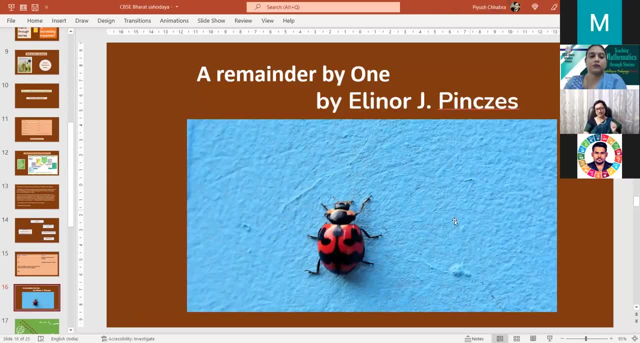 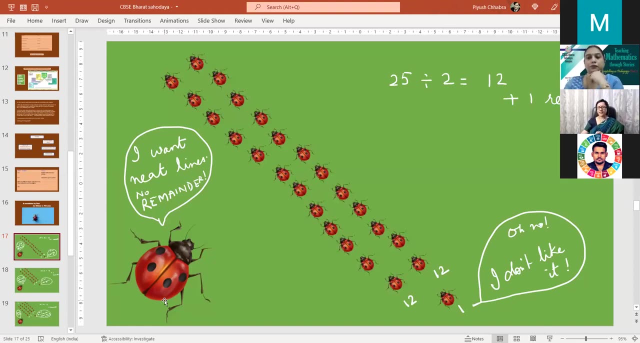 just see this one, a remainder by one. this is also a very sweet story, you will see. so this is a little bug, a little bug, and so there were so many bugs and there was a queen bug and she said that just do march pass in a better way, i just want you to move nicely. and they all: one, two, one, two, one, two. 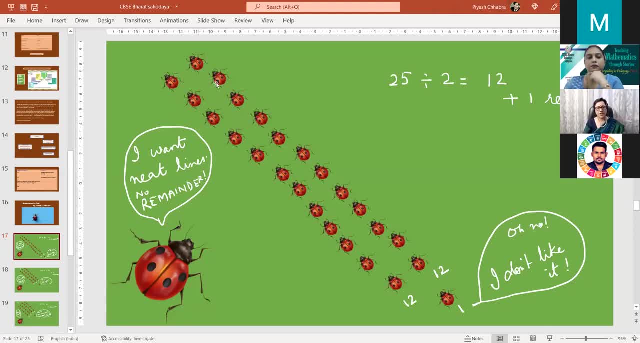 so they what? what they did? they were 25 and they just lined up like this. so they divided themselves into two parts and then, like this, there were 24 and one was left and it said: oh no, i don't like it. and this queen said: i want neat lines, no remainder. 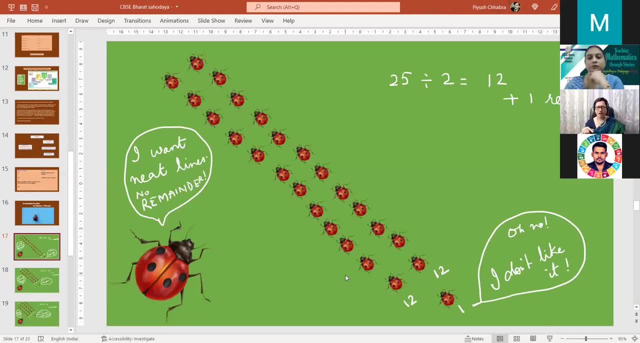 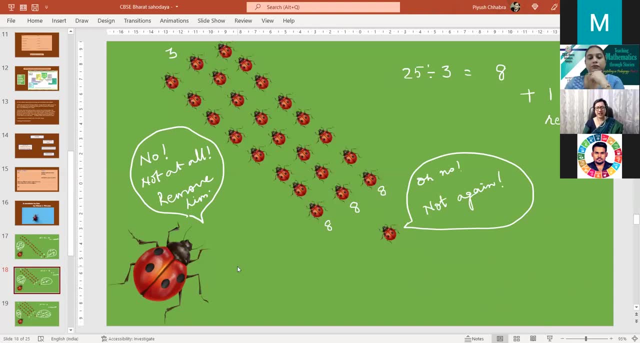 remove this bug. this is left one. no, i don't want that now. this bug was very, very sad. next again, they thought he thought: why can't they become in in in three lines? let me see. and then next day they became into three, so it becomes eight and three. 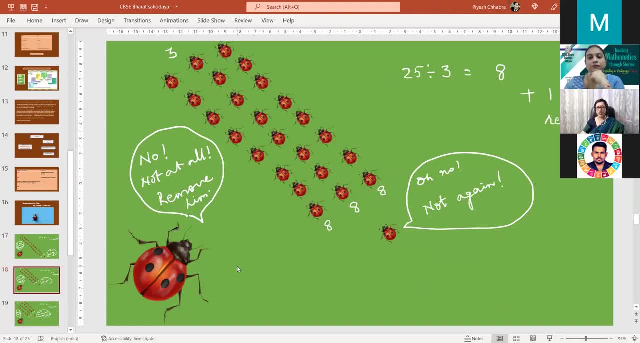 lines, so 25. they divided themselves into three lines and again one remainder. oh, no, not again. and then this queen said: no, not at all, remove him. this bug was really upset. oh, what to do? i don't want to be left alone. no, no, no, no, no. oh, what to do again? he said. 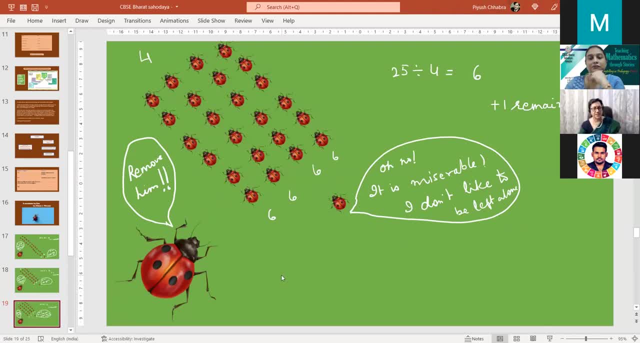 thinking what to do next. and then again next day he says everyone, why not let us please divide into four, please include me? they all said okay, and then again they divided themselves. this time six line, now they were into six, four lines and six in one room. again one, oh no. 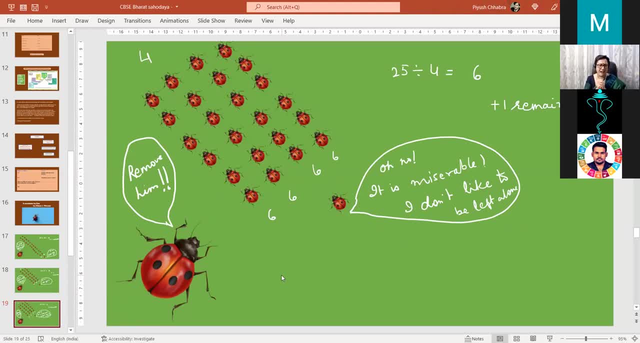 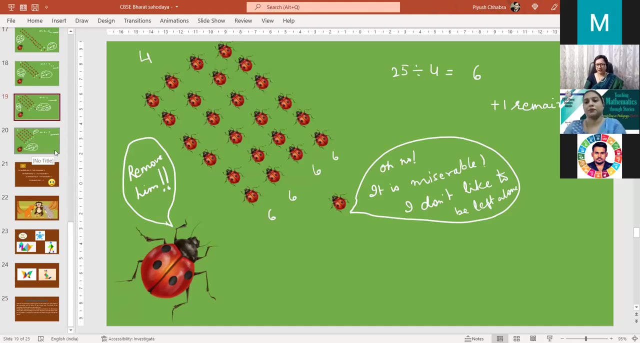 it is miserable. i don't like to be left alone. and this one is saying: i, i don't want to see this single one remove him. oh my god, no, no, no. i'm having sleepless nights. i really don't like it. again, he's thinking and he just asks his friend: please, one more time, please divide yourself into. 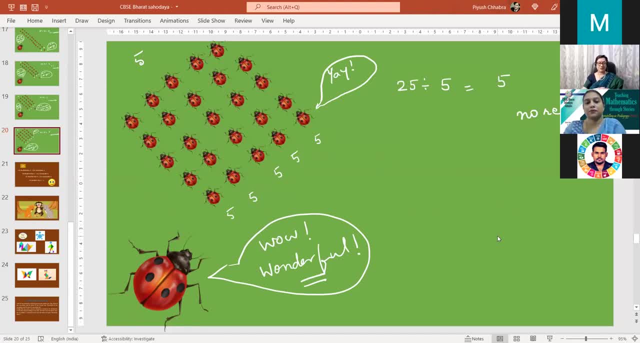 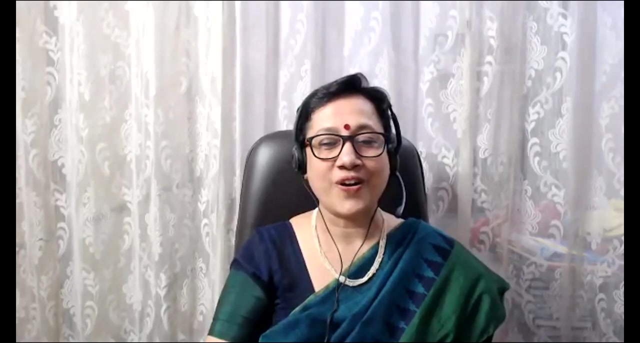 fives. now, when they divided themselves into five, then what happened? no remainder. and he's saying yay, and the queen says yes. now the march past is good, wow, wonderful, and this small little bug is really very happy to be the part of this team. so in this way the story goes, and i just want everyone to please write down what are the various 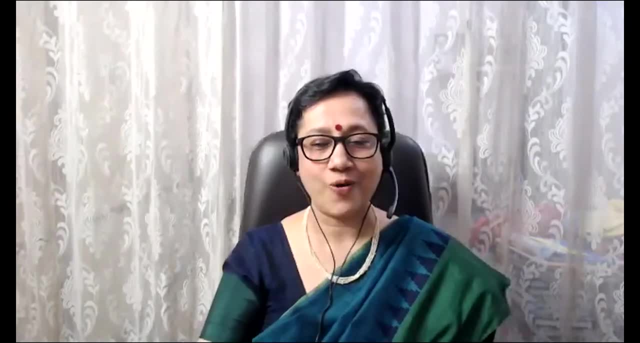 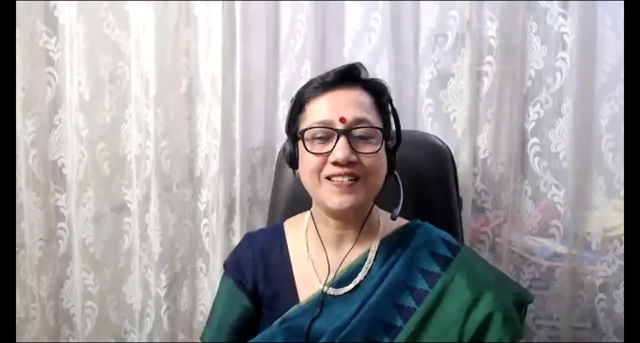 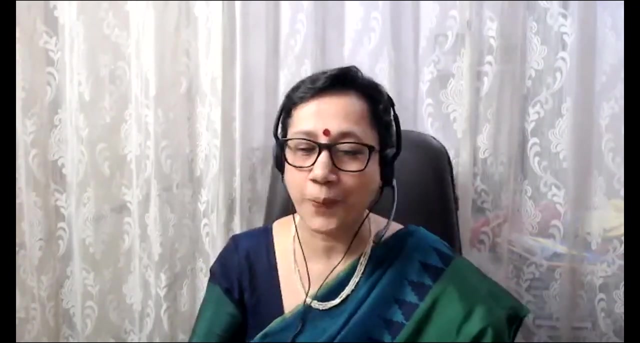 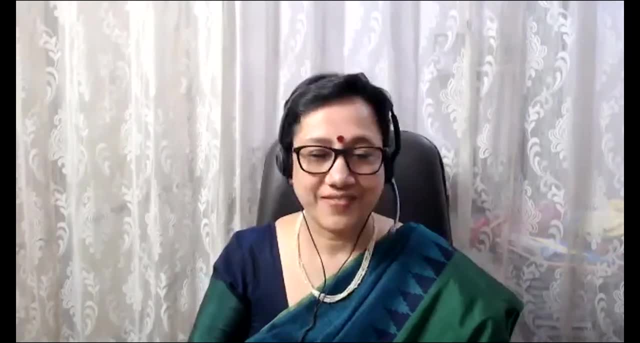 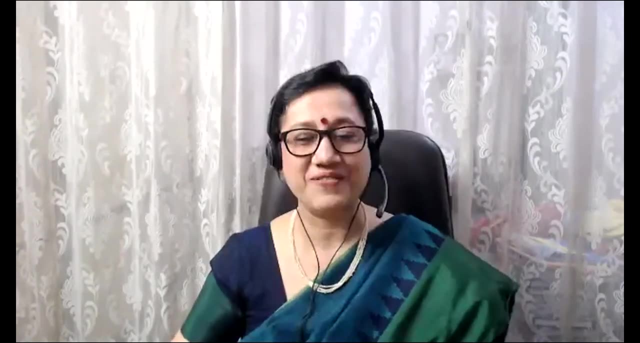 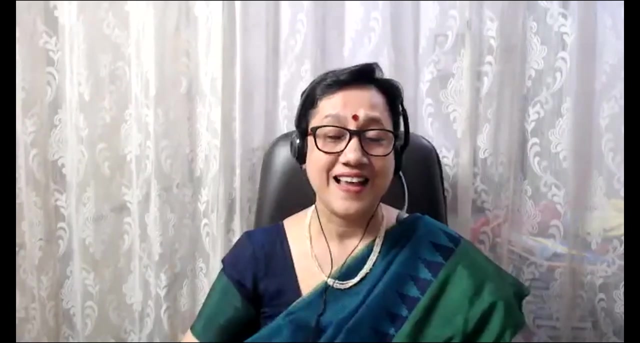 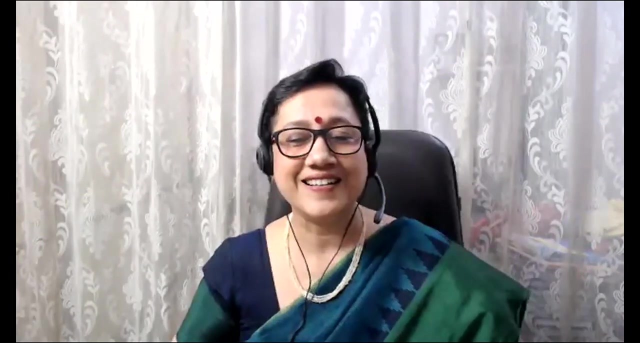 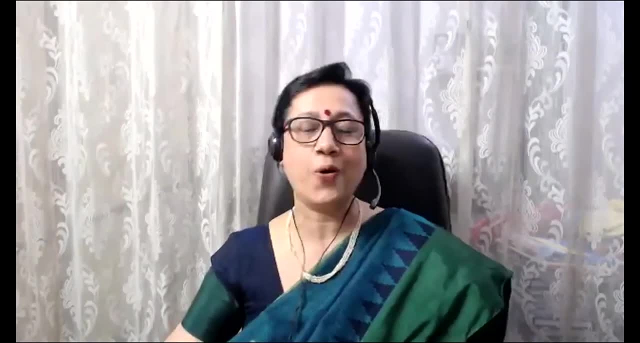 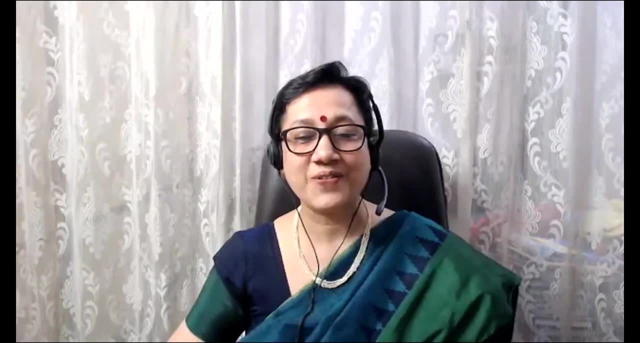 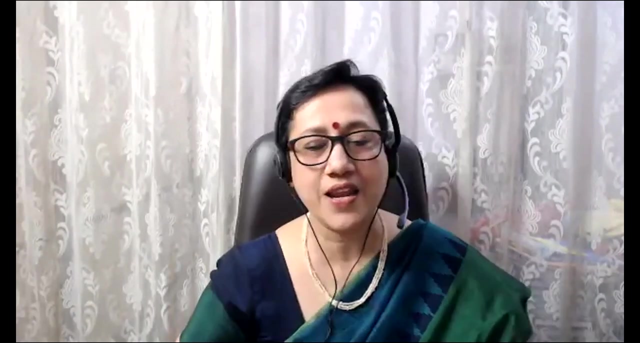 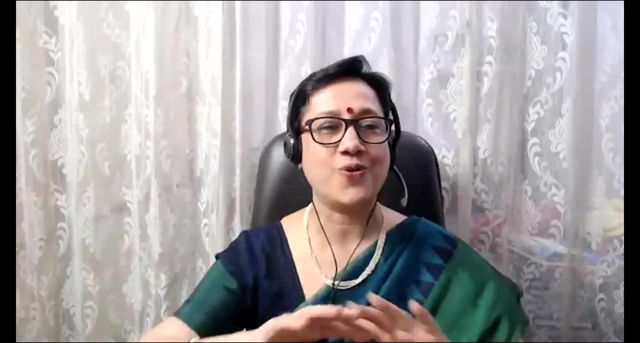 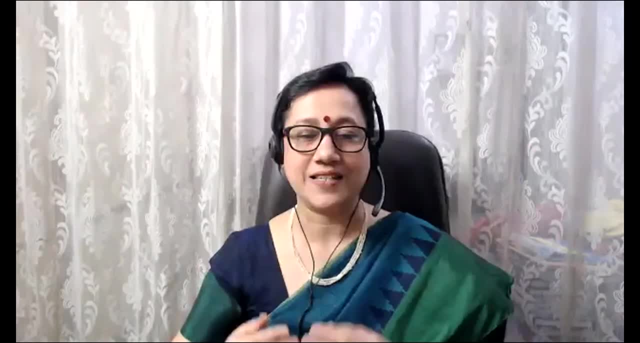 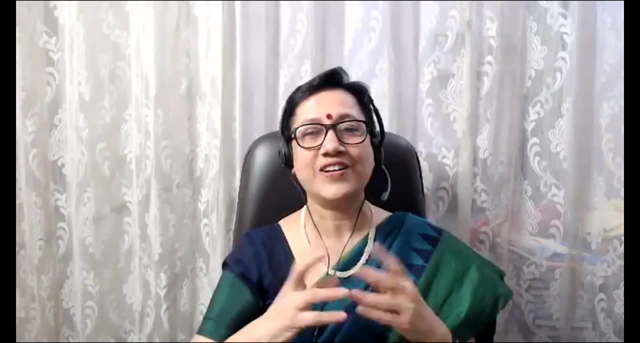 And when I'm doing, even if I'm showing it on the PPT, you must have observed that I'm doing what? Voice modulation Right. So that is very important. Otherwise children will not be able to correlate what and the situation of that bug who's left behind. 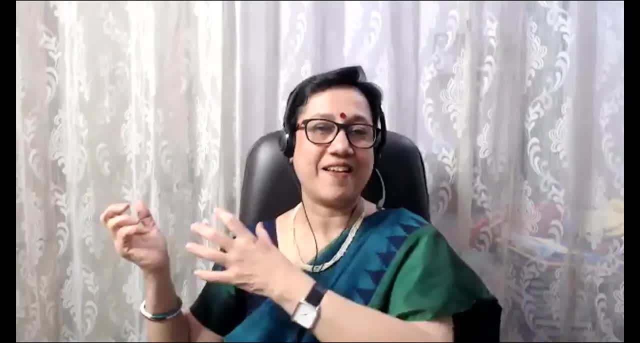 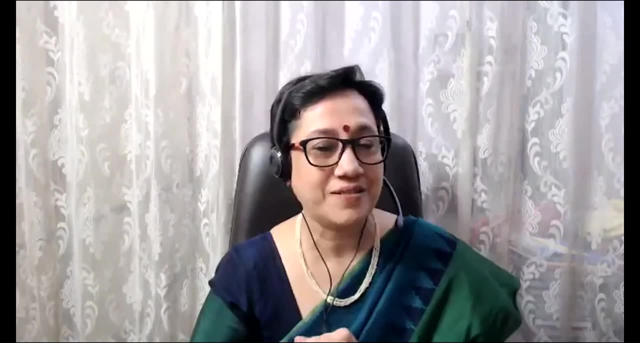 Even the team members. they also don't like that he's left behind. They just want him and they listen to him and then rearrange themselves. So all these things are very, very important, because these values also are to be instilled in children. 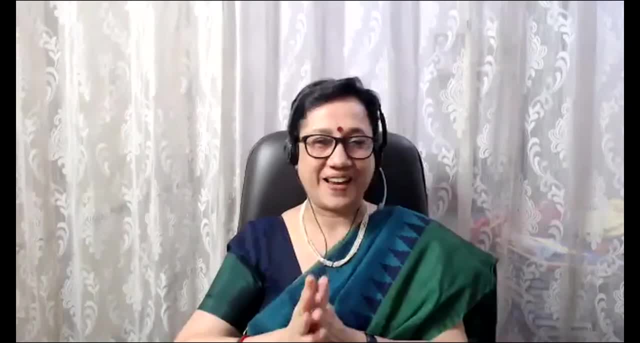 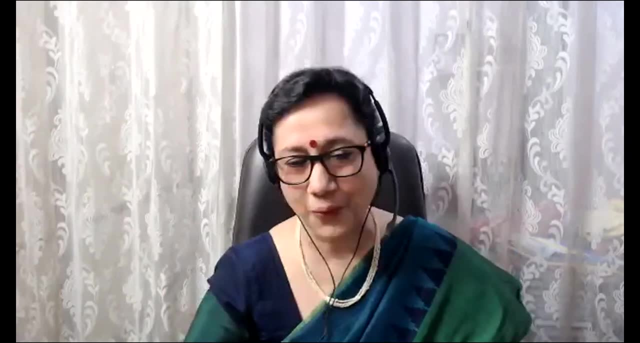 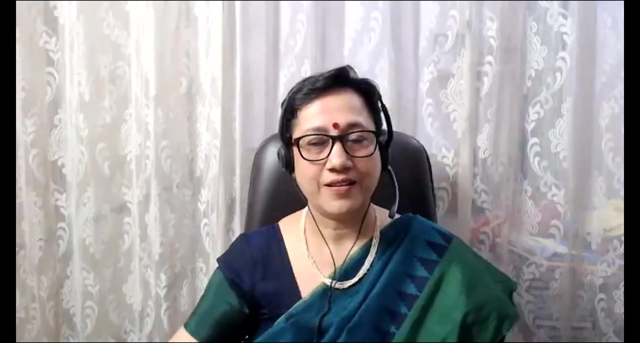 So we have to understand that through maths also we can do- It's not only the job of a value education teacher or any language teacher- that the values to be. No, we can have our stories. We have to select our stories in that way that it is again giving the value also. 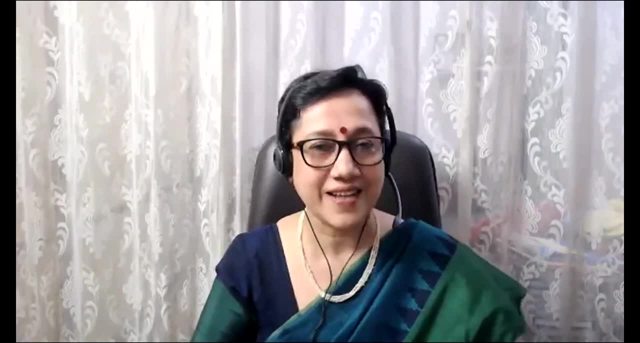 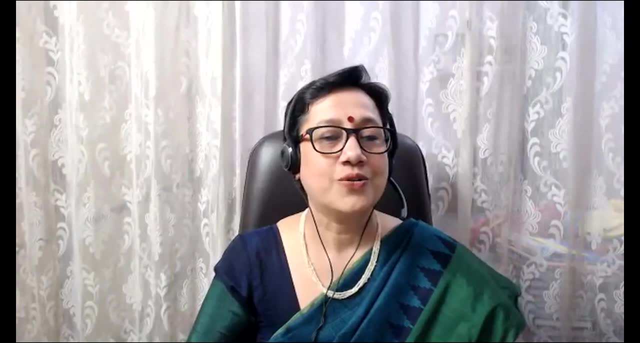 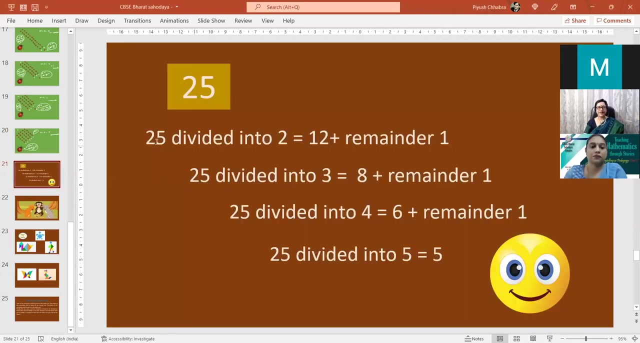 Though we don't say children will only say: what do we understand From me? ma'am, he was very smart, He was very good, He was very hardworking, like this. OK, so Now we move ahead. OK, so here I did like twenty five divided into two, twelve plus remainder one. twenty five went to three, is goes to eight plus remainder one. 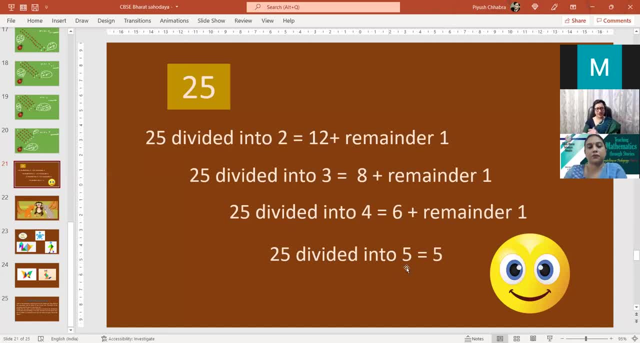 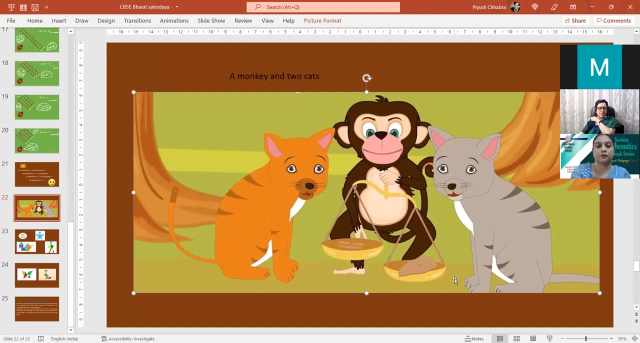 So in this way we have seen: Yes, Five divided into five is goes to five rows and then no remainder. So he was very, very happy, And you all know about this story. who can tell me which concepts can we do with a monkey and to get the punch it under a story? please write in the chat box. 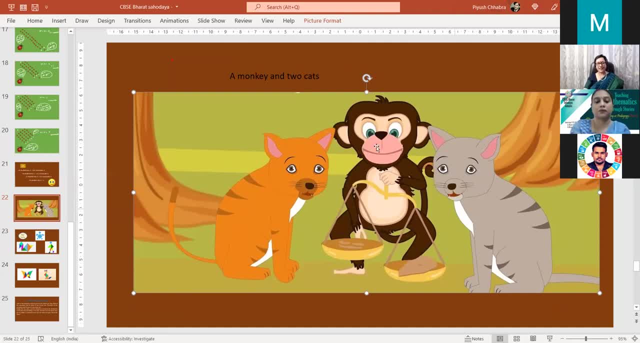 Let me see. This is: there are two cats and there's a monkey, and then there was he's having a balance. I hope you know all the story That there was a fight between two cats and they just what happens? Yes, A monkey comes and says: oh, don't quarrel. 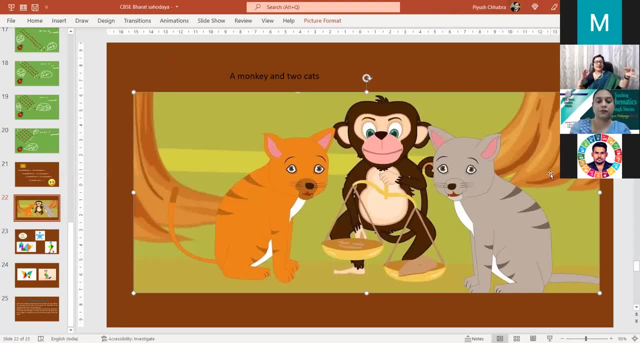 Don't quarrel, I will help you. And then he just cuts into two pieces, but unequal pieces. So which concept can we do with this? Tell me Right in the chat: Yes, yes, yes, yes, yes. Fraction comparison: 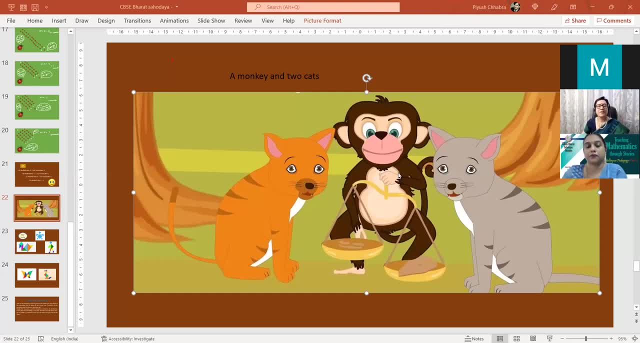 Right Division. OK, OK, Huh, Huh, Yes, Yes. So we have to dig into our punch it under the stories. Also, there are many things hidden into that, So let's find out. what is it? How can I use those stories? because they are beautiful and children know that story. 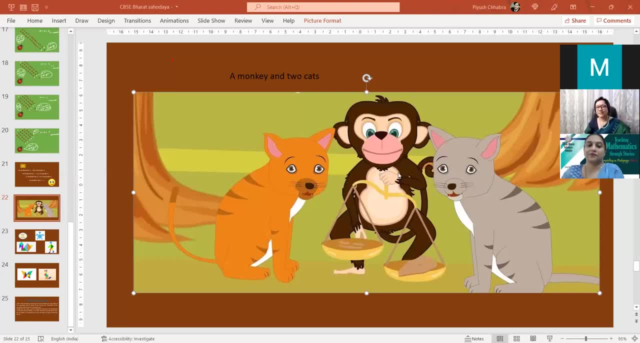 Yes, Yes. Street smart tactics: Yes. Moral value: OK. Fraction OK, Balanced OK. Life skill: Yes. Life skill is very important here, Yes, Yes. Weight fraction OK. Equation: Yes, Equation also, even in chemistry. 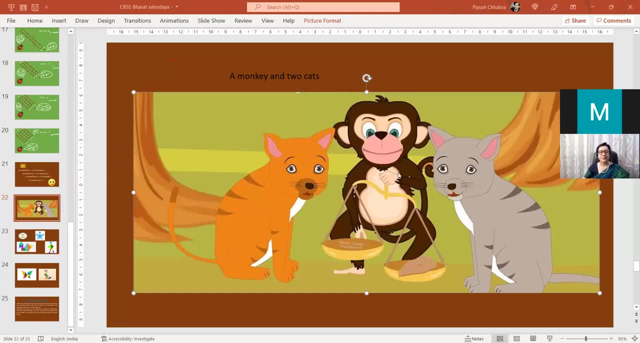 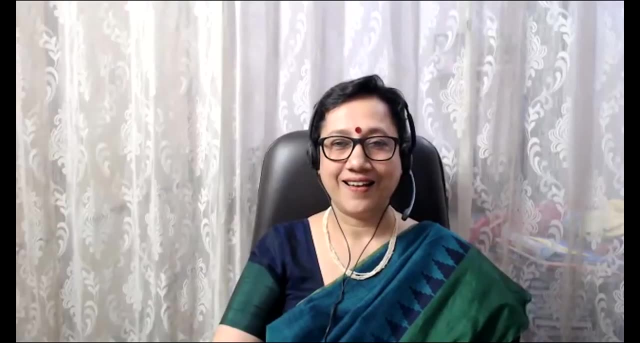 Also, you can use teachers, those who are science teachers, learning by doing sharing, caring, OK, Problem solving, life skills- Money, Yes. Money, Yes, OK, Great, Thank you All of you. you are really participating so well. you are just responding to my questions so that the 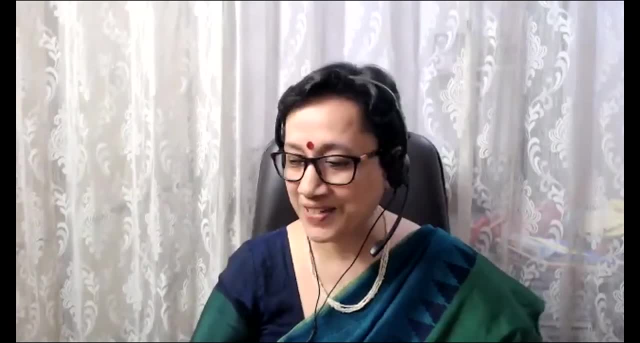 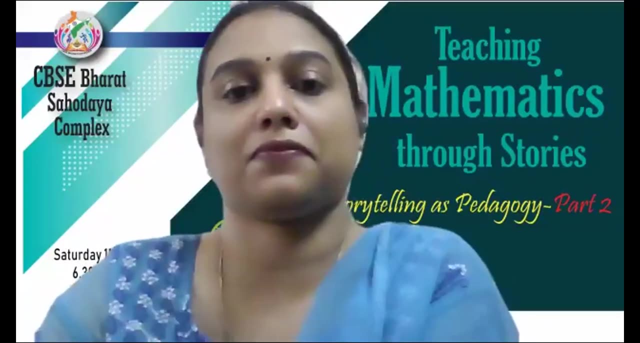 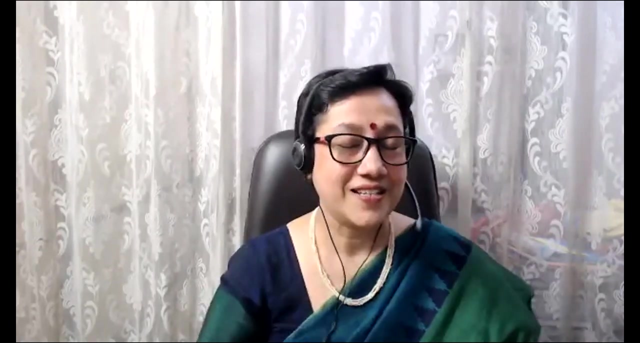 Session becomes interesting. I'm happy about it. So I would like to tell you a nice story Again, a story of a small girl. The girl is Munia- Muni, you can say- And she's in Maharashtra, Anjarli village. 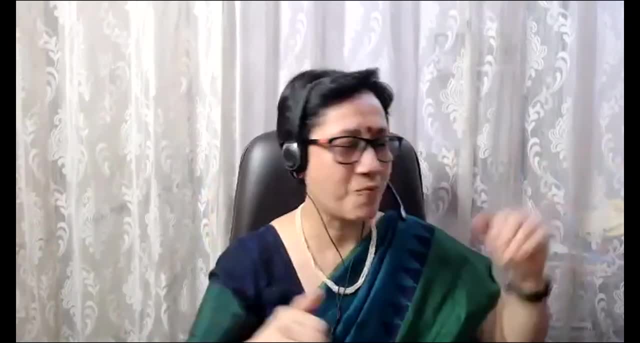 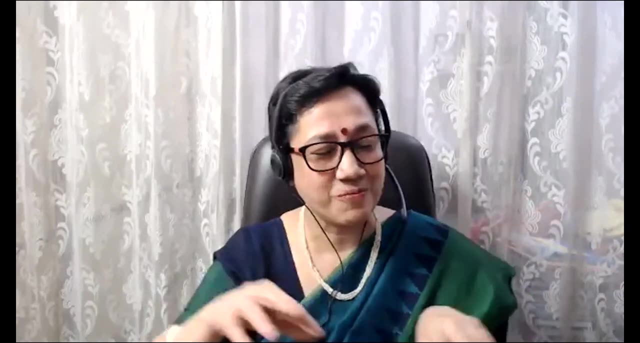 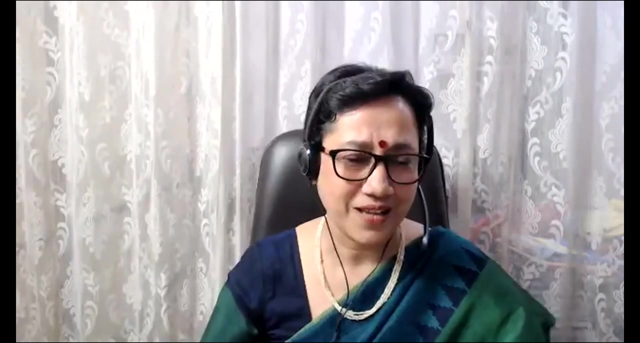 She keeps roaming, here and there. She's small, tiny one, But very sharp, And then she's moving around. She's moving around every day, throughout the day. She's just moving around and she has so many friends, you know, And the cock also comes. 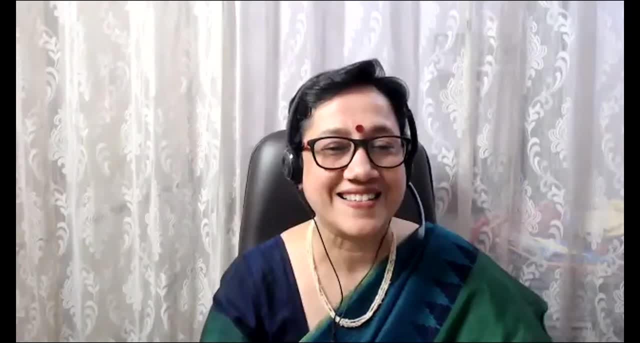 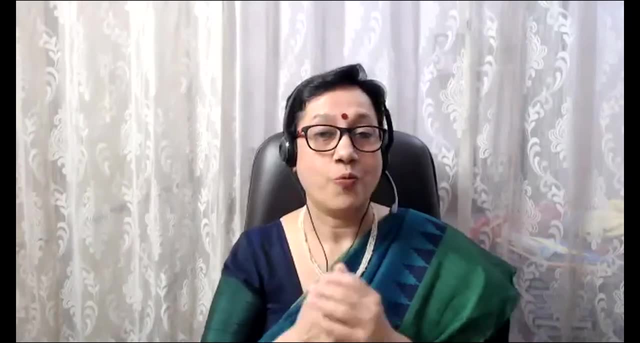 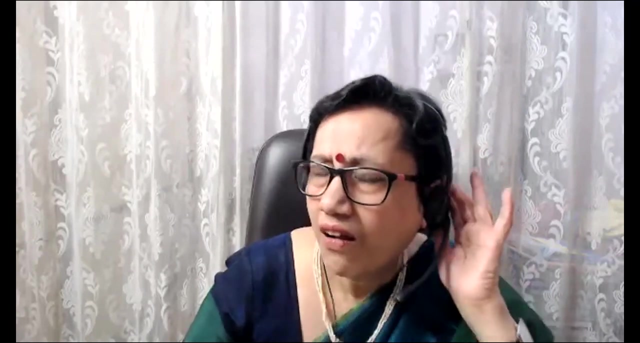 And then a small puppy Like this. So all the animals are the part of his. You can see everyday life Once. when she comes into the house in the evening, she listens to some voice. What is happening? Let me listen. Mama is shouting at Papa. 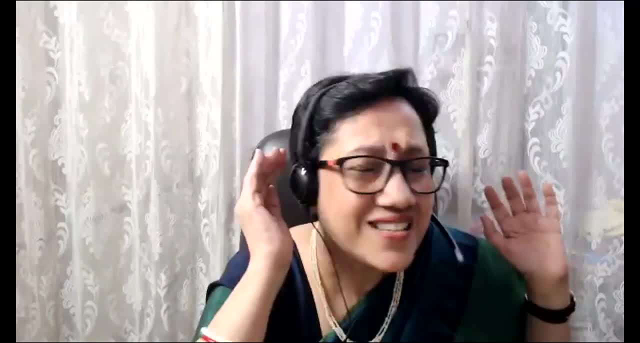 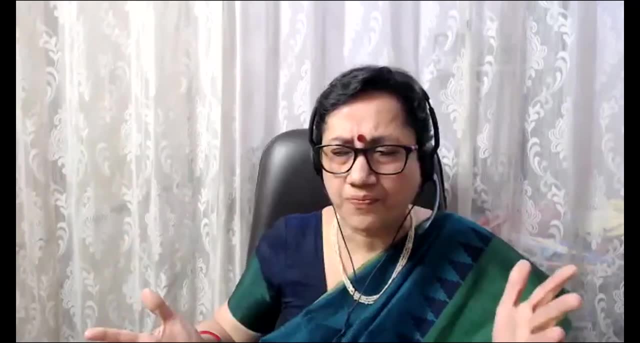 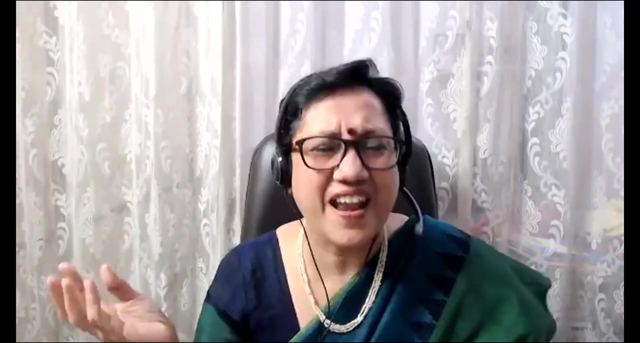 What is it? I don't know. Let me listen. Mama is saying: Why have you brought so much of salt? What are you doing? I could not help it. My friend has given me that gift, This gift. How much salt do you want? 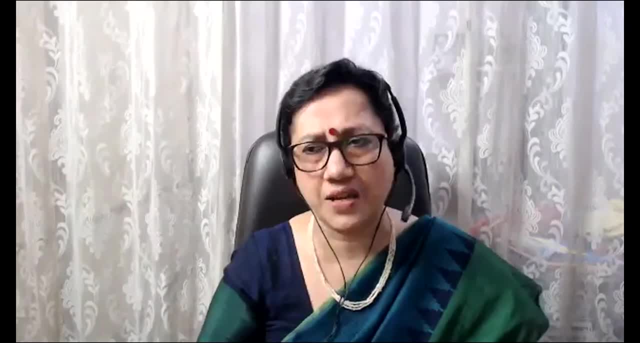 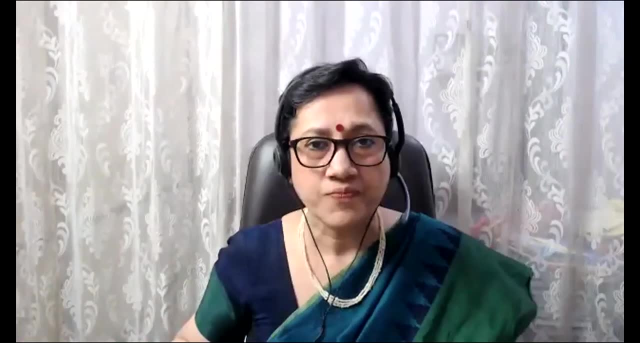 How much salt do we require every day In a vegetable? In a vegetable or dal Pinch of salt, And what have you done? You have brought full sack of salt. We are not even going to use it for a year. And you know there is no space in my home. 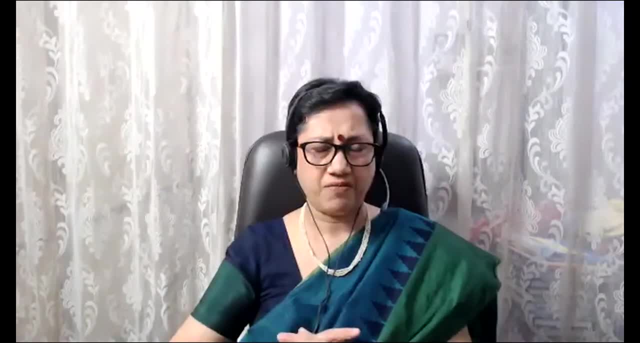 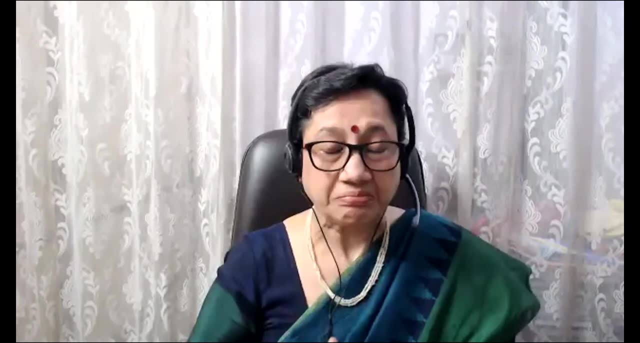 Such a small house you have built. What to do Where to keep? Don't shout, I'll keep it in the backyard. Okay, Keep it in the backyard. And this Munia was What to do. How can I help? 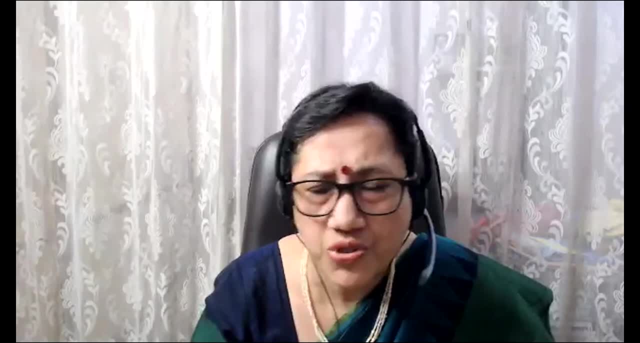 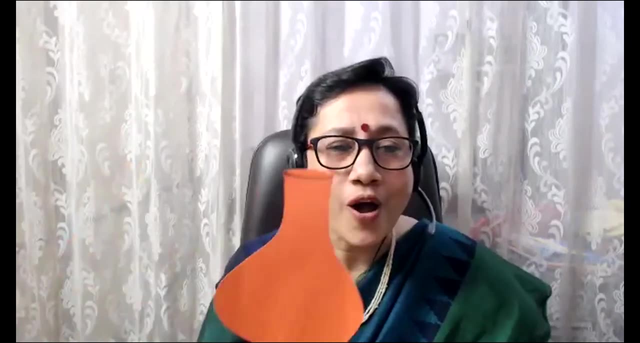 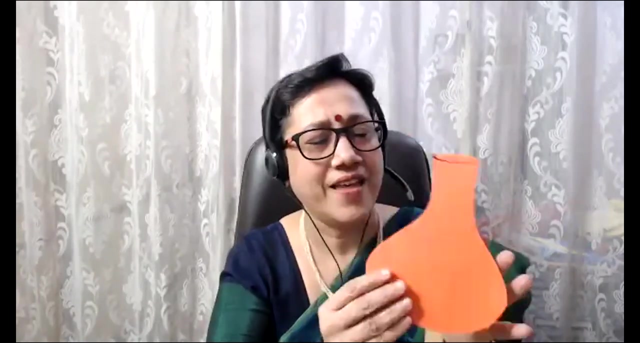 How can I help my parents? Then she goes to the backyard, Looks here and there And then she finds One pot Which she can just pick up. Oh yes, The size is okay, I can pick it up. And then 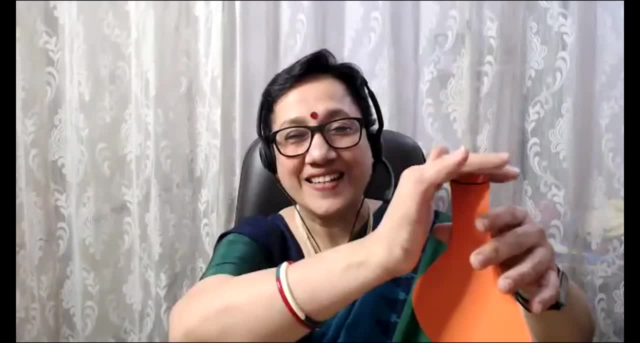 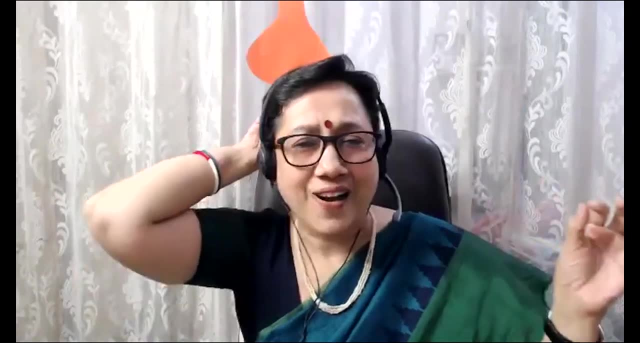 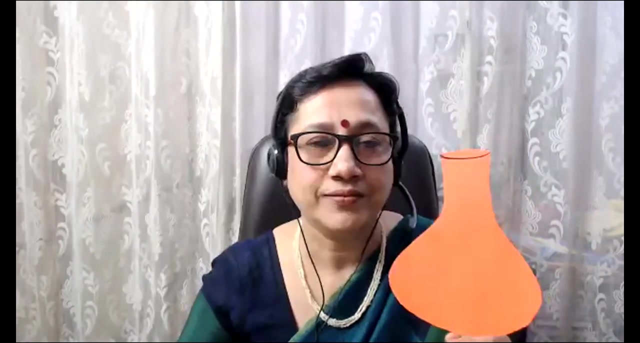 What she does? She pours some salt into it, Mmm. Now she carries on her Bag and just goes: Namak le lo, Namak le lo, Aunty, Salt, Do you want, Mmm? So Munia, You are selling salt. 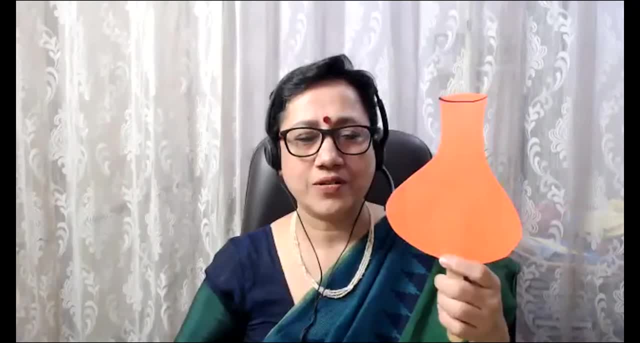 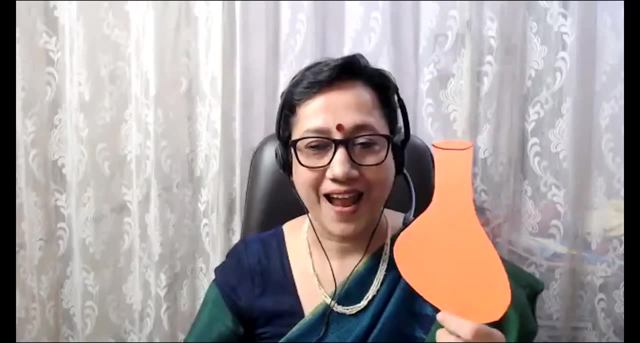 Yes, aunty, Do you require salt? Okay, One pot, Aunty. it costs Five rupees for a pot. Okay, Then give me one, And then Aunty takes the salt And then gives it to her. 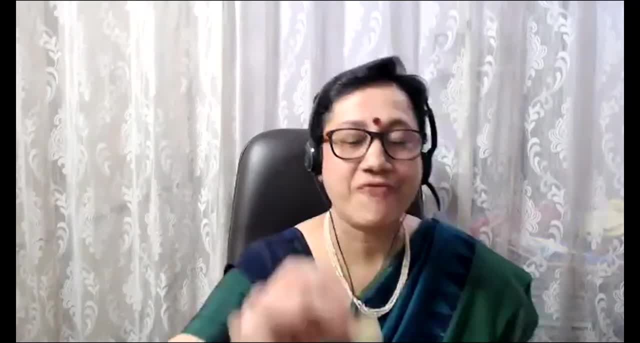 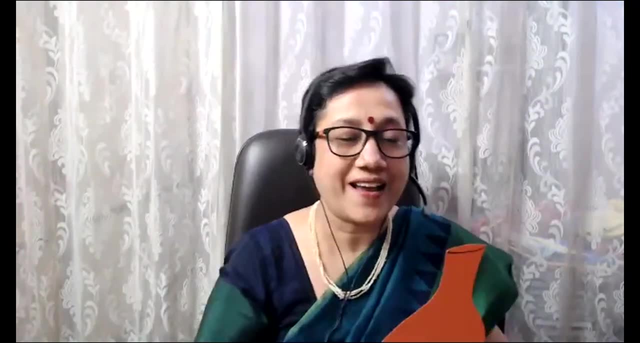 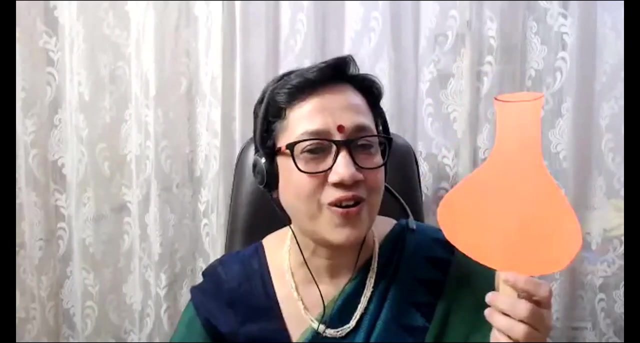 What Five rupees, Yes, And five rupee coin She gets and puts in the This one. Now she goes again, Fills it up Every house. she is Aunty, Aunty Salt, please, Do you require salt? 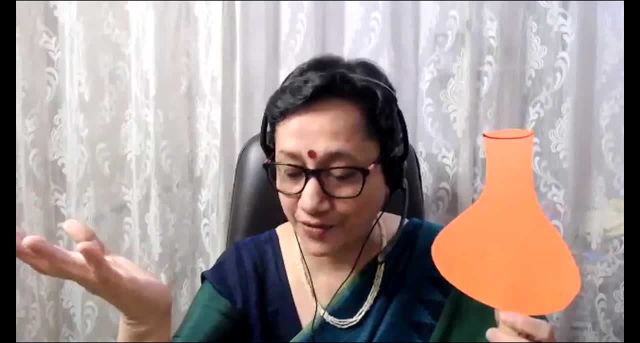 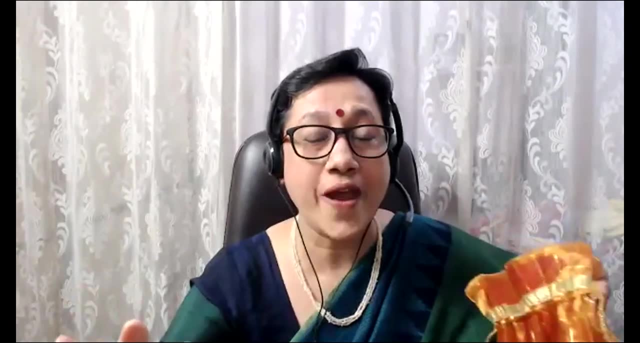 Okay, Give me three. Now how much will she get? Fifteen, Yes, Fifteen rupees. And puts One, Two, Three, Fifteen Now in one house. When she went there She got twenty rupees note. 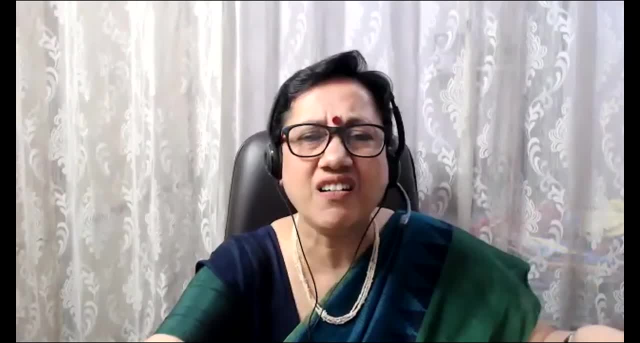 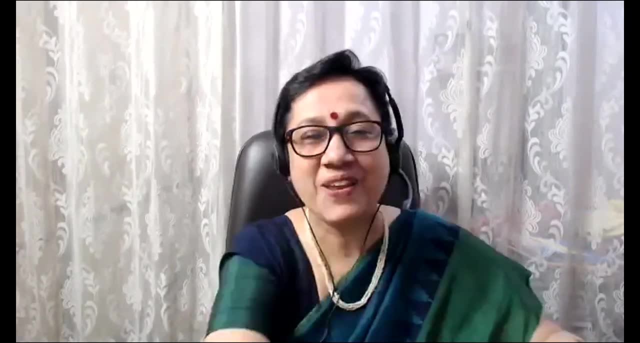 But they wanted only two. How much she should return? I am not understanding. What should I do? How much should she return? Yes, Ten, Ha, Thank you. And now she is Counting: Okay, Ten, And in this way. 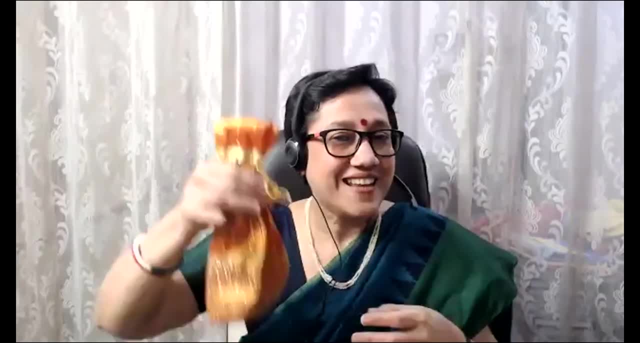 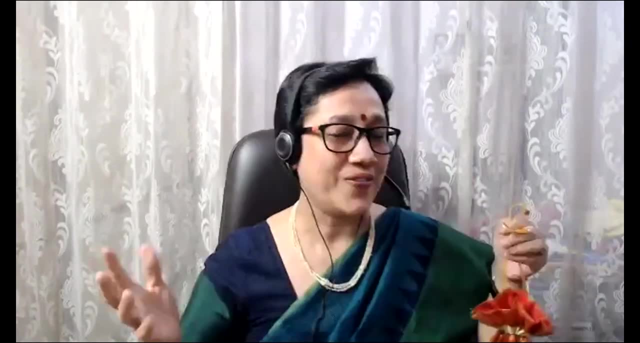 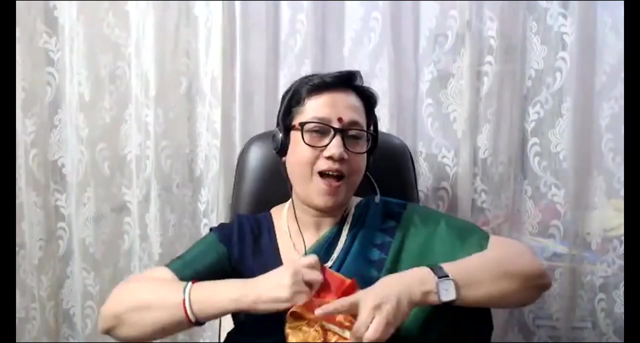 Throughout the day What she did. She had collected So much coins And then, When she came back, She saw the sack is Empty And there This is full. And she started counting. Five, Ten, Twenty, Wow, So much. 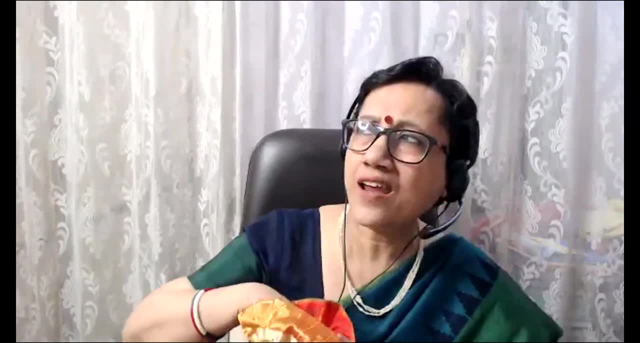 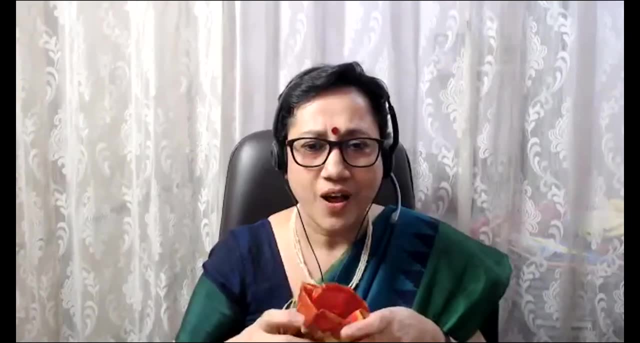 And then suddenly Papa calls: Muni, Muni, Where are you? Papa Come here And the papa comes over there And looks at: What is this? Get this money, Muni. What have you done, Papa, Papa. 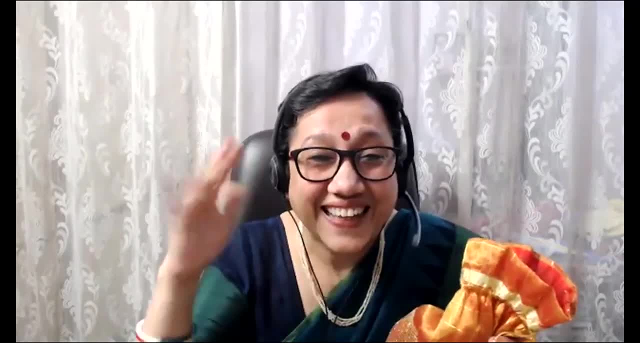 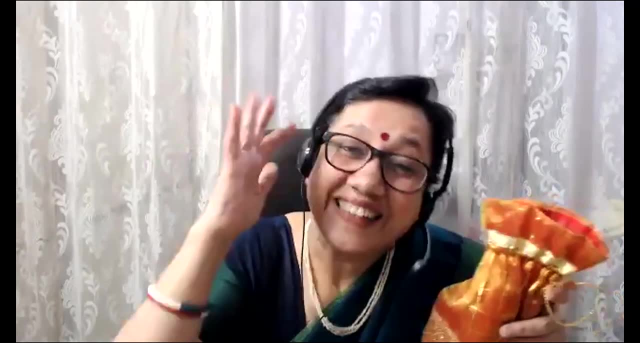 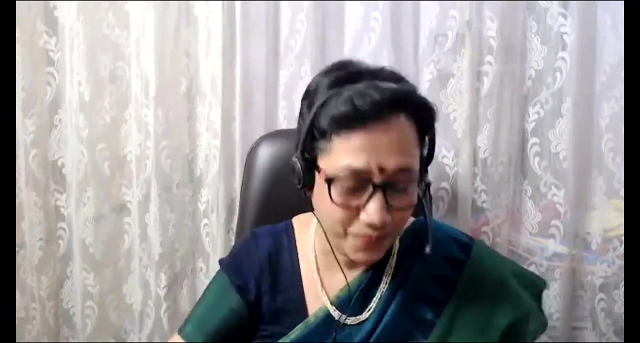 Come, Come, I will show you, Ha, What happened to them: Salt. This sack is empty, Papa Ha, And you have done this. Oh my god, Let's, Let's go to mama. And they all, Both of them, went to mama. 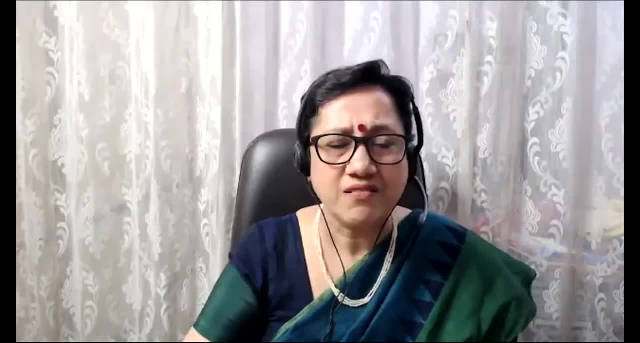 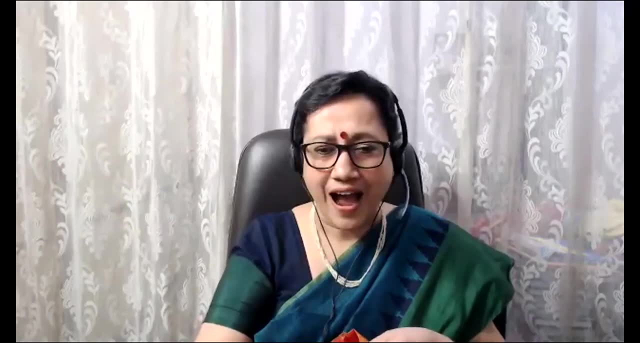 And mama was What happened? Why are you so happy See what your daughter has done? So much of money, Ha Muni, How. And then she said, Mama, I have sold all the salt That was such a big problem for you all. 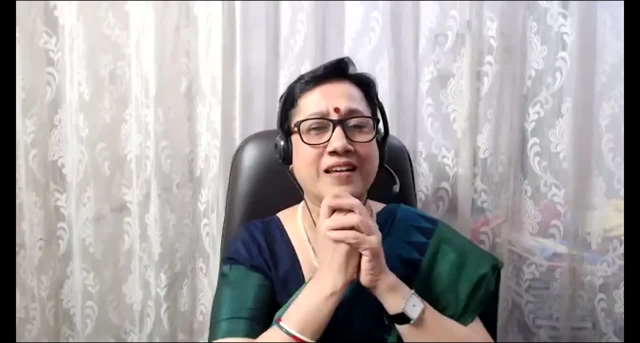 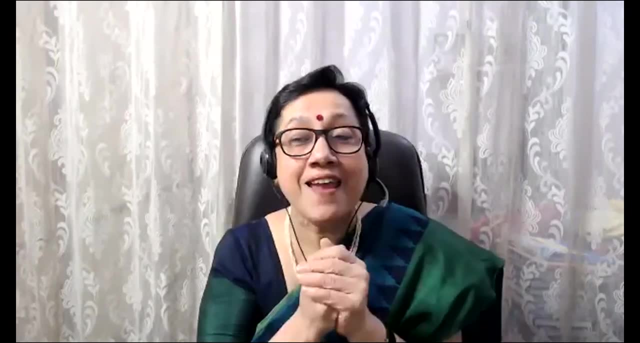 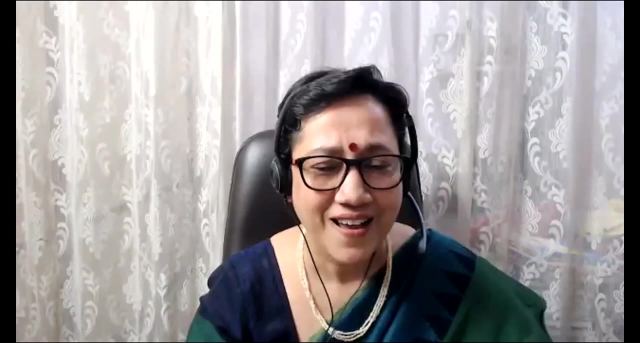 Mama said: Oh, my dear, You have become a small entrepreneur at this age. I am so happy I am going to use this, This money, for your Future. I will send you to study to school now, In a bigger school. 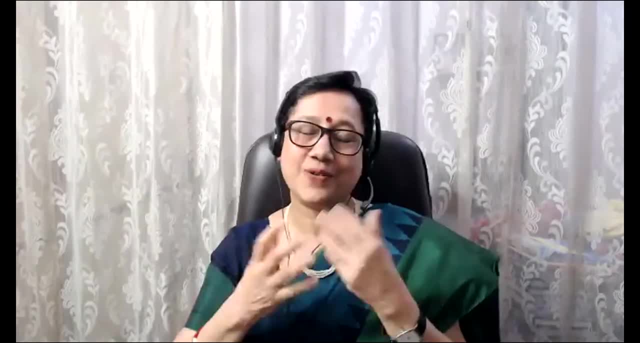 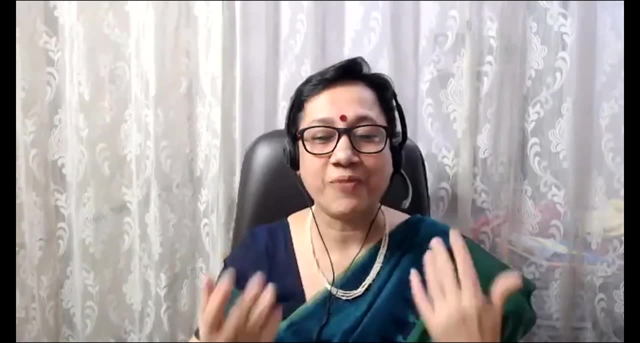 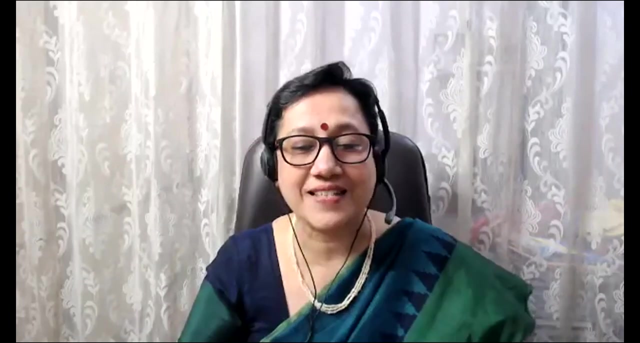 Muni is also happy. The whole family sits together And have food happily And people have already written: Weight measurement, Money Problem solving, Decision making. Now you have started understanding How to use maths in school, How to use stories, 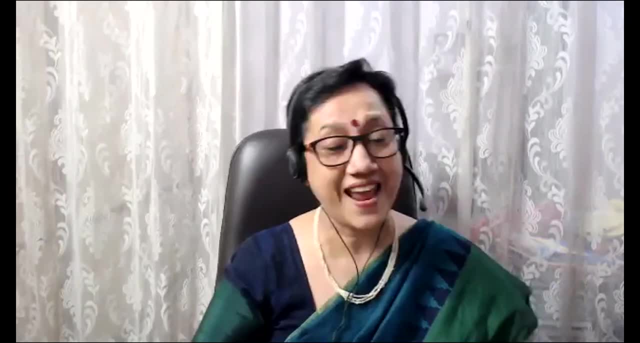 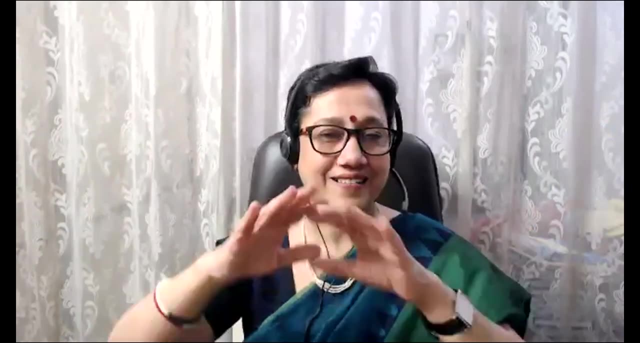 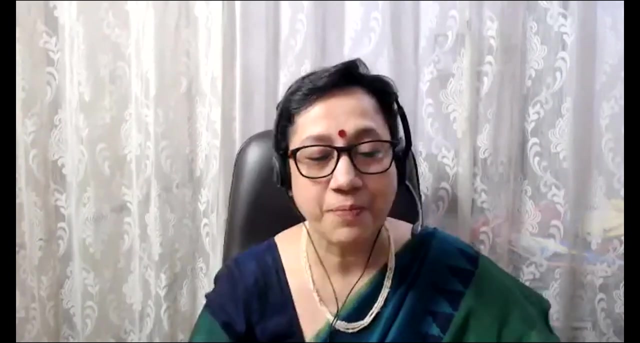 Yes. Disadvantages: Yes. Profit loss: Yes, Yes, Yes. Full and empty: Yes, Yes, Yes. Even you can also add That salty area, Even salt also We can think of later on If you are a science teacher. 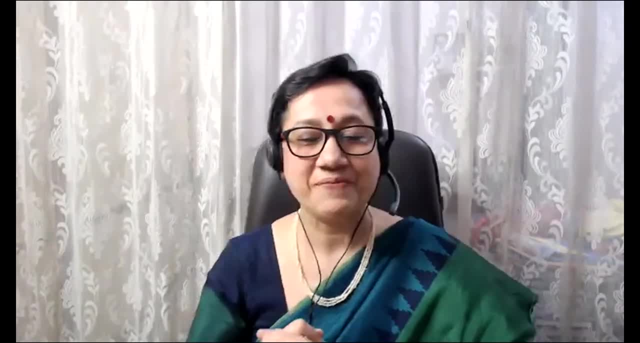 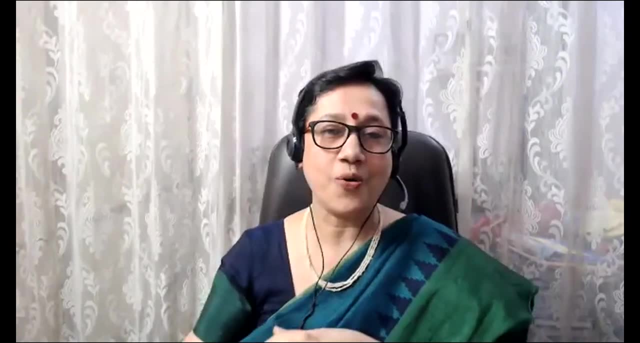 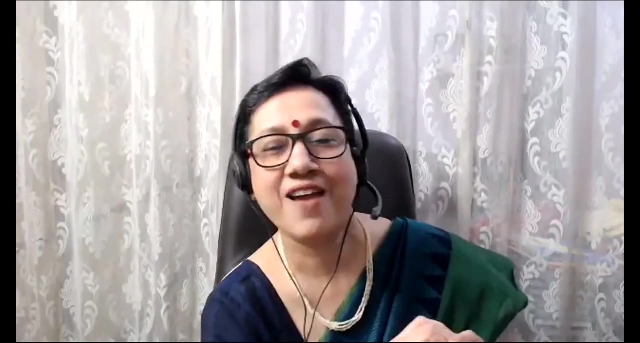 You can also do that, Okay, Yes, Money transaction You can easily do. Yes, Right Division, Helping Money, Great Creative thinking, Mental competition skills. Wow, So many, See, So many With just one simple story. 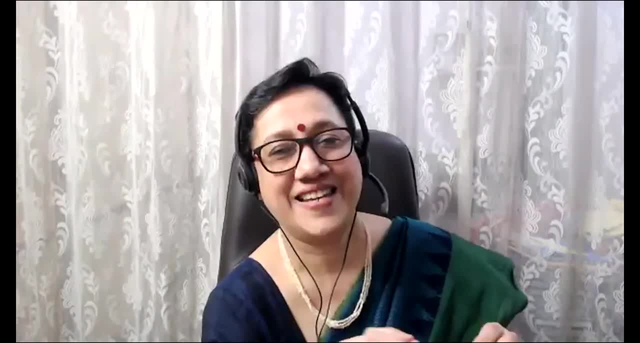 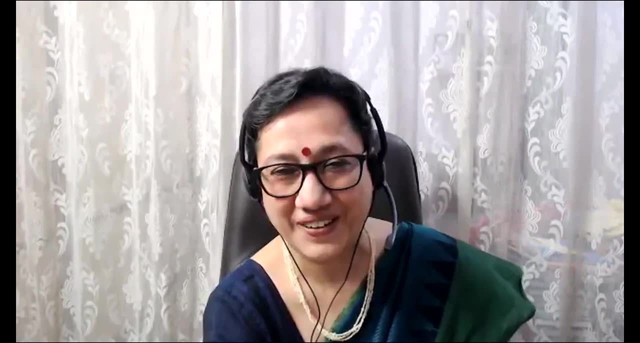 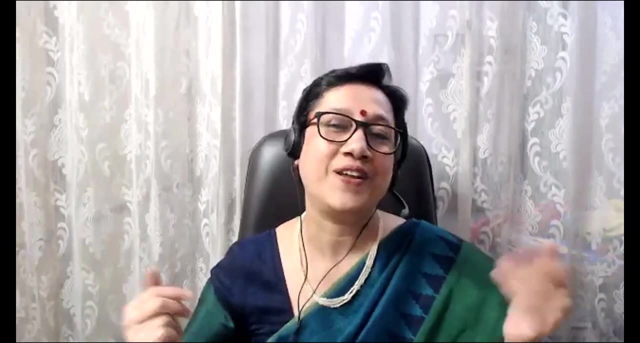 And I must say: But today I have changed that story With a girl, Because I want Girls also to understand That they can also be an entrepreneur. So we can also do that. You can always say That we have to make. 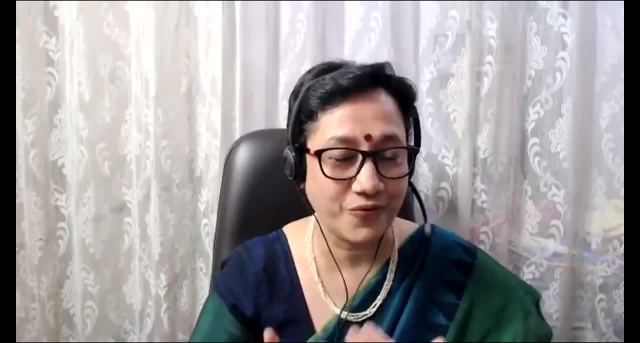 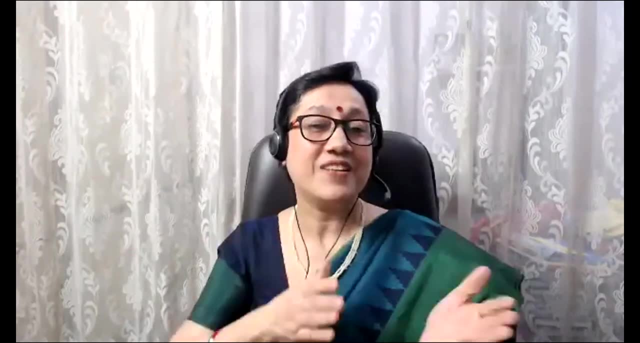 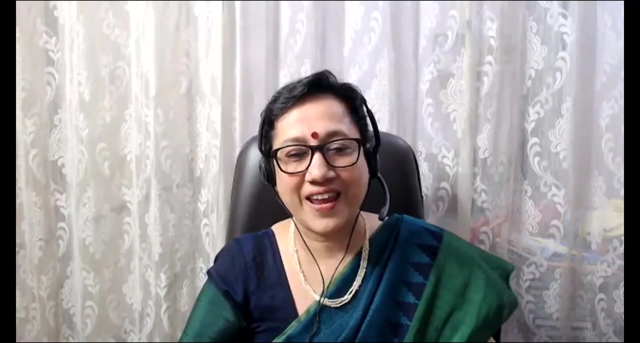 Like gender equality Also. you can do in the class Some stories of boys, Some stories of girls. Otherwise, most of the times What we do Is telling you How I change the story With the girl. There is nothing. No protagonist can be anyone. 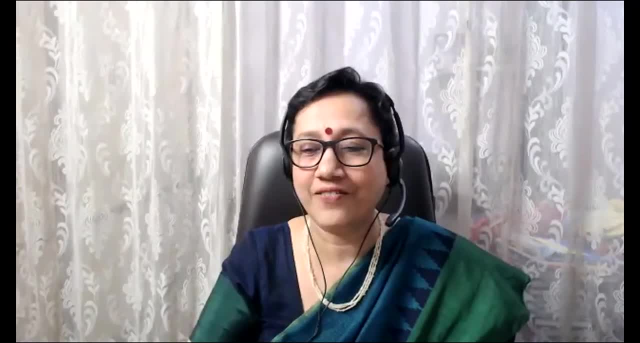 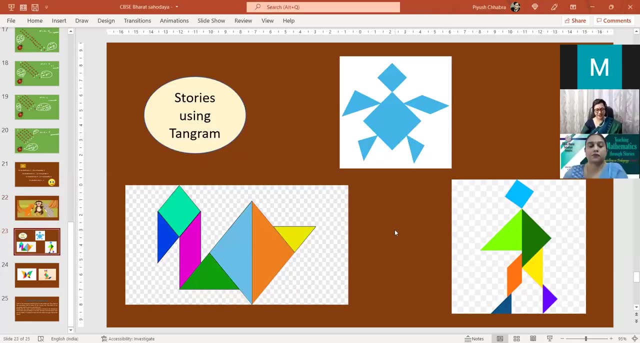 So we can think on those lines also. Okay, So I hope you are understanding How we are doing stories In the classroom. And then see this one. So Tanagram is also a good way To do stories. Give your children. 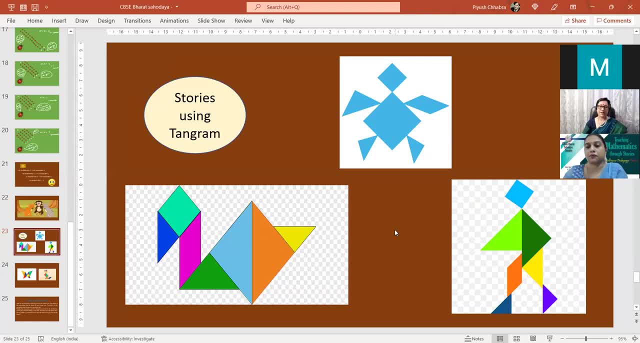 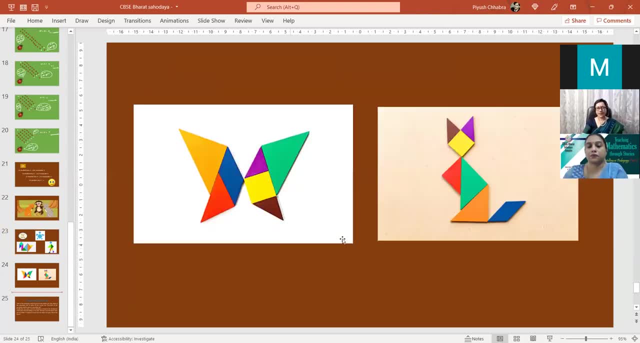 Tell them to bring their Tanagrams. Not only make a story, But yes, with any topic That you want to enhance them with, Okay. Similarly, here also There are two stories. Anyone who would like to tell What story you would make? 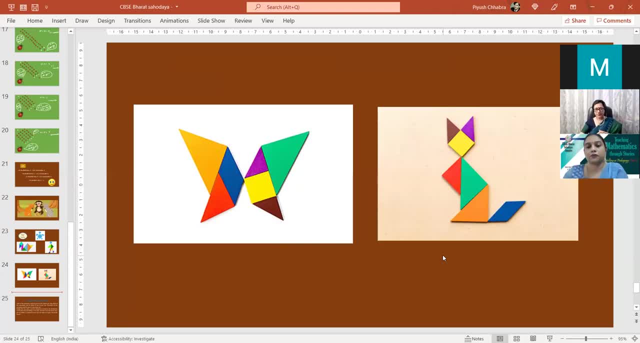 With one single concept With this cat and a butterfly. Anyone who would like to make A one, two line story, Then we can have some topic, Give a topic to it. This topic you would like to deal with: Tanagram, with these two images. 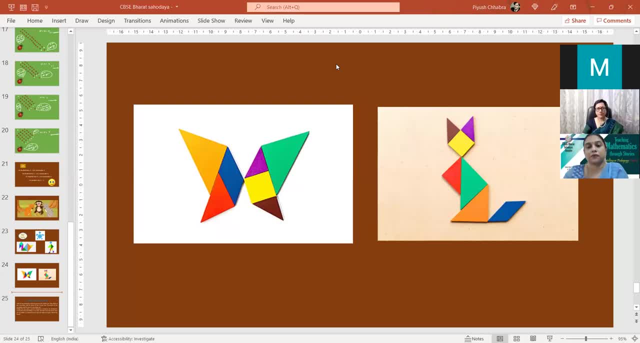 And you make it. Anyone Shapes- Okay. now I want Symmetry with butterfly, Okay. no, I want some story. I believe you want people to make stories. Yeah, Story. I want, with two characters, Make a story, But with some concept in mind. 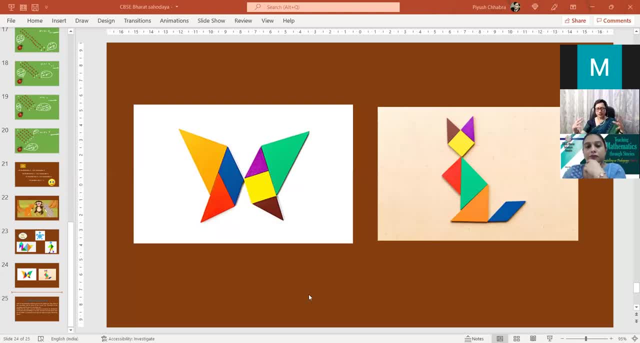 Yeah, colorful cat And shape a butterfly. And then you have to make a story Out of it. Concept of addition: Okay, on a triangle planet With the triangles. Okay, okay With tanagram. I want some story. These two pictures. 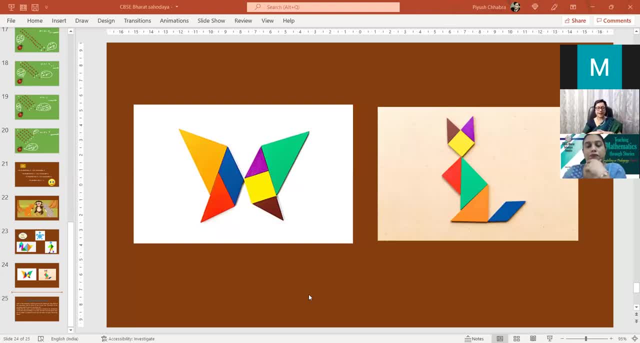 If one of the children have made One of the children have made These two pictures And you are telling them: Okay, use some story. Okay, so, yeah, So, yes, Now you can fly, Then flying part is coming under science. One day, the triangles got together. 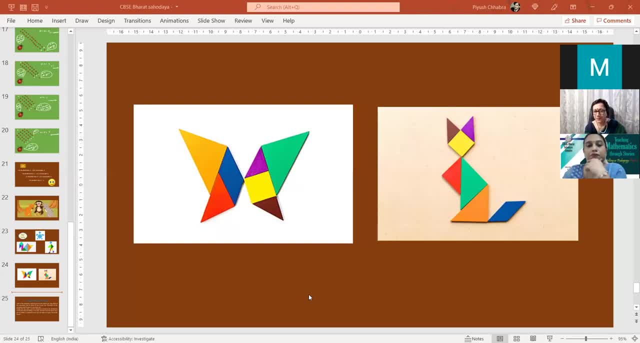 And decided to have fun. Okay, okay, Who is very happy As symmetry? But cats do not understand. Ask her the concept of symmetry. Okay, now great. Okay, Polygons who decided: Okay, cat catching a butterfly With the measurement. 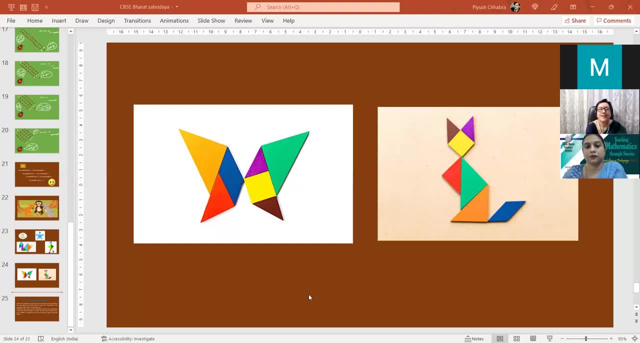 And help of something. Okay, but fighting, who is winning? How high can you reach? Okay, height- good. This is also good. Yes, Their friends are going to flying height, As can be. I can deepen- Good, This is good. 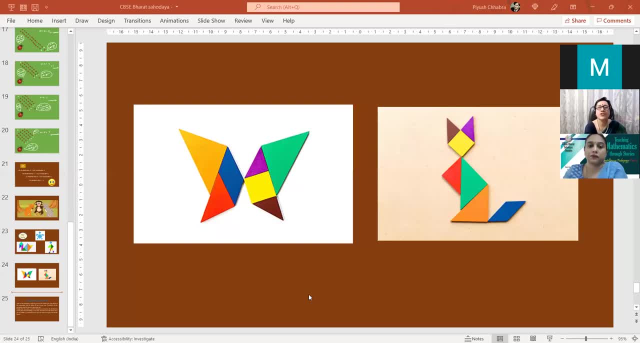 Nice. So concept of height: So you have given- Maybe you have given them Okay, number of legs height: Okay, counting here Can be idea of line of symmetry: Okay, Butterfly collecting honey: Teach measurements, Okay, yeah. So now you have started getting it. 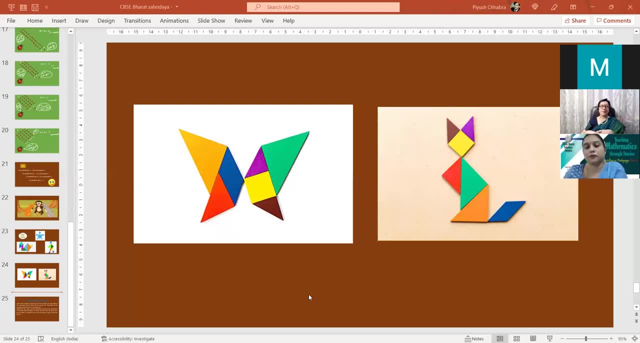 That how we can use To make problems, Problems in a form of a story, And I have already told you That. what you can do, You can have them over there individually, But lower classes maybe in groups And then the whole class. 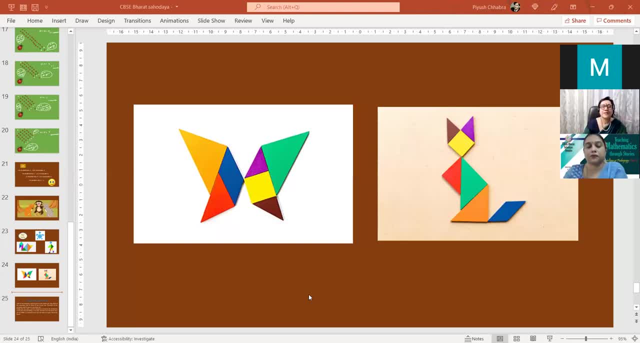 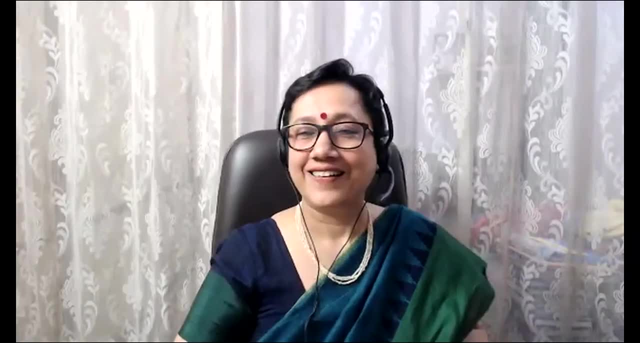 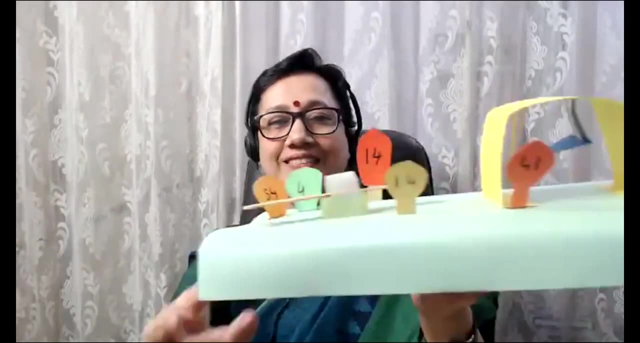 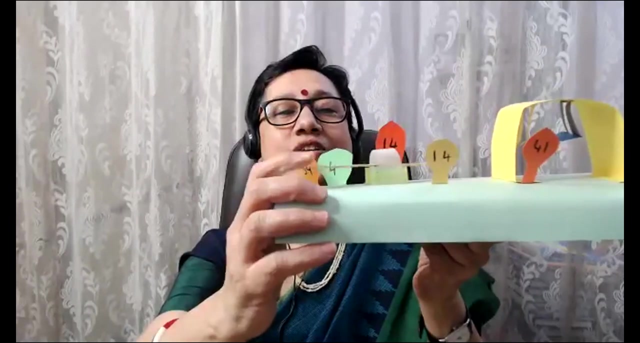 Together also. Yes, Great, Nice, Yes, See. And one more is there Which I had made. this one You can see here. This one is there Where this child, This is number 14. And he wants to sit on this, see, saw. 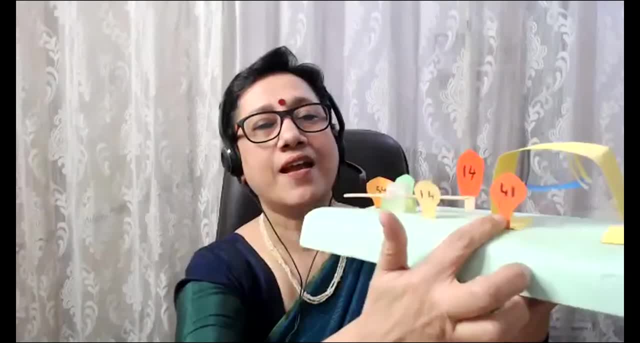 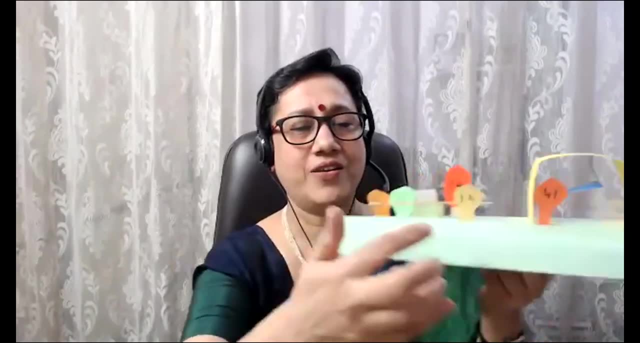 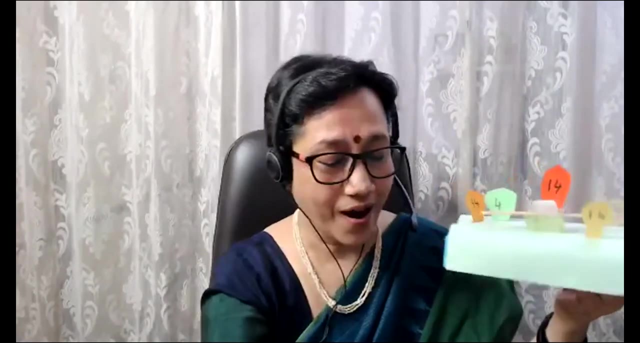 Okay. And then he asks others: Will you be able to play with me? No, no, I can't play with you. This is 40. I am 41. And you are 14.. He says, Oh ho, We look similar. 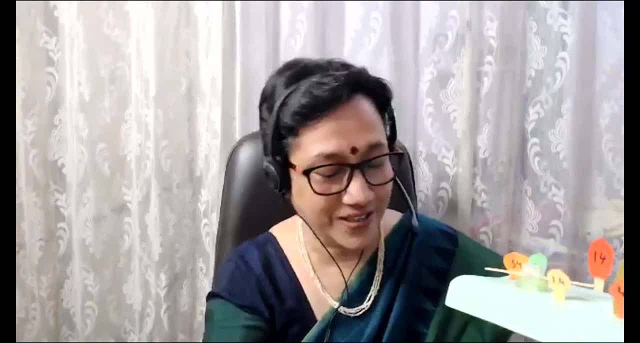 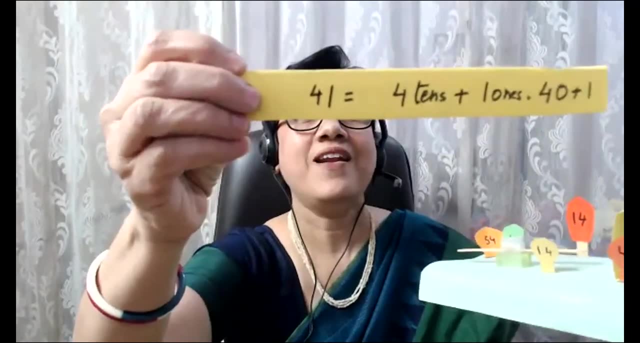 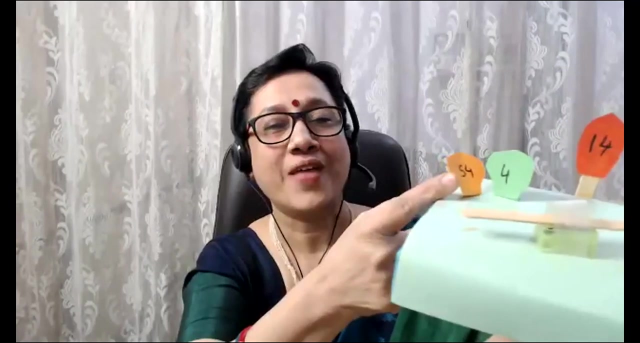 Why can't you play with me? He says no, You are 14.. 14 is 110 plus 4. 14. And I am 41. 41 is Okay. Then he goes to 54. And asks: 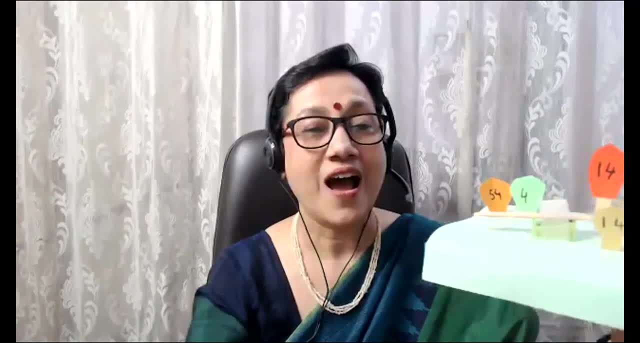 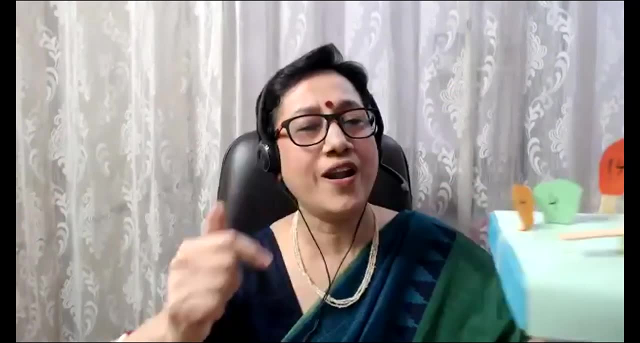 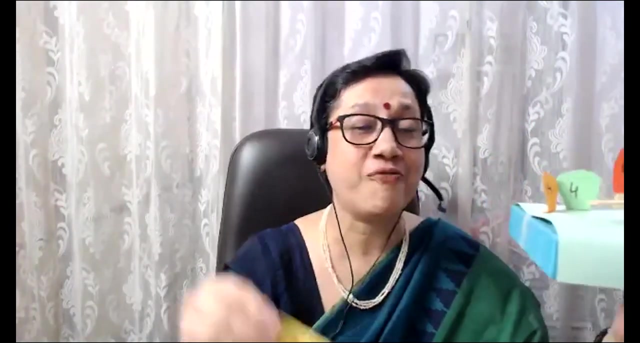 Will you be able to play with me? He says You look like me. He says no, no, I am 54.. 5 tens and 4 ones. Then he asks this person: Only 4.. Will you be able to play with me? 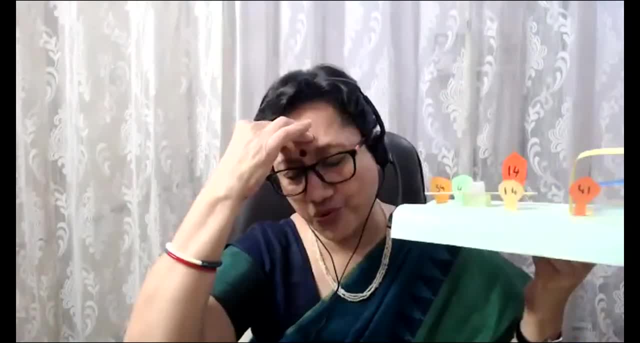 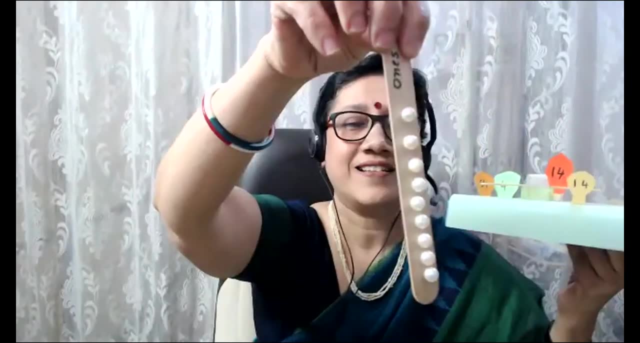 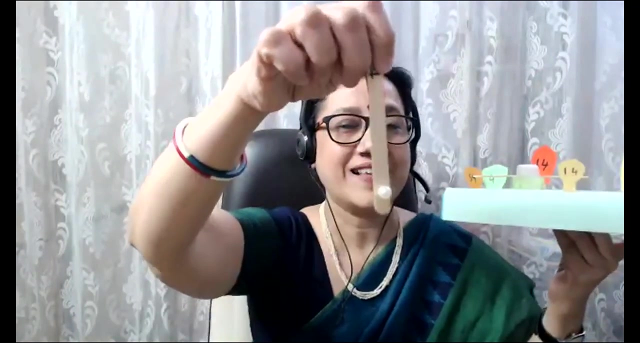 He says: no, I am actually only 4.. What is this tens? What is this ones? Then it is like this: When there are 9. It is in ones, And once you get one more here, Then it becomes a tens. 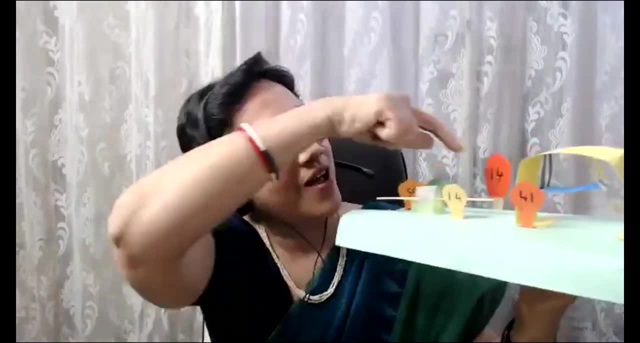 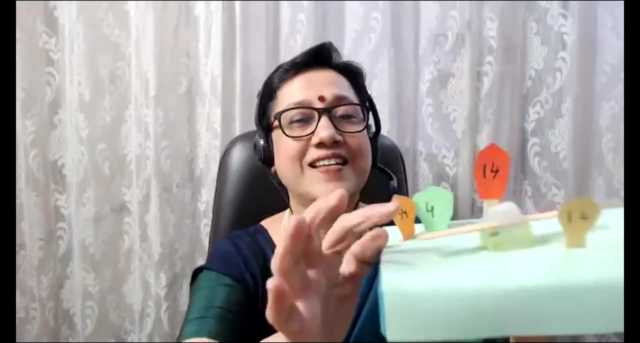 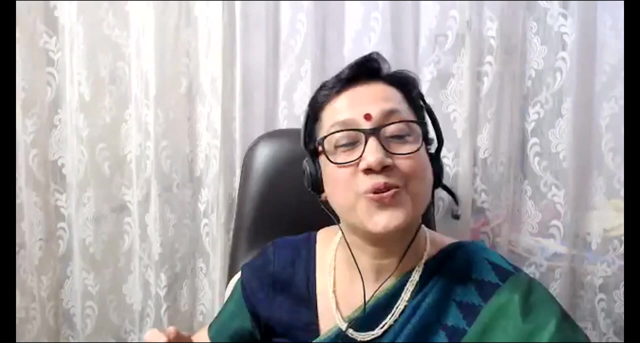 Okay, So this becomes tens, Yes, And then comes 14 at the back. He looks at it And he just runs over there And these two now can sit on this. see, saw, So 40. They sit together to have this. 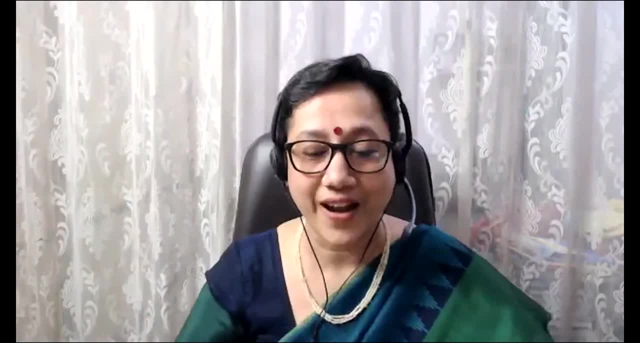 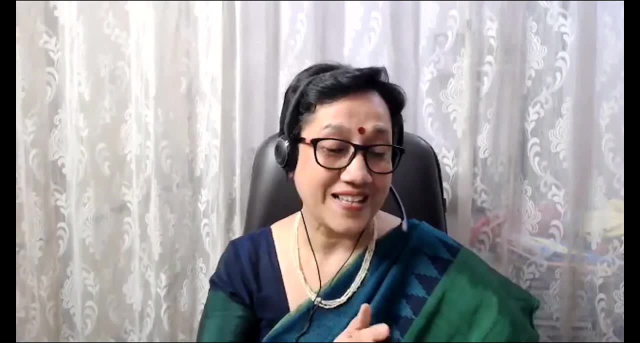 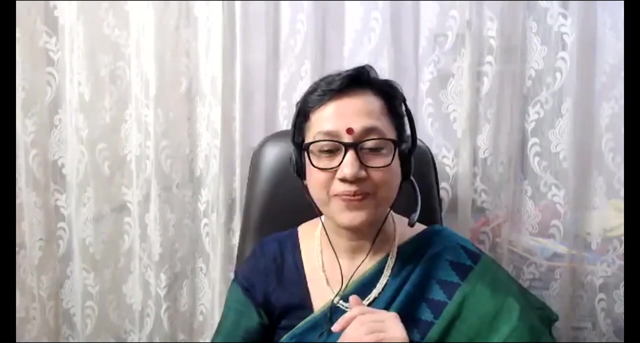 So, in this way, what we can do. Yes, you are all writing now That you are understanding How we can use this Place value, Or you can say Tens and ones, Whatever the concepts you have You can use in this method. 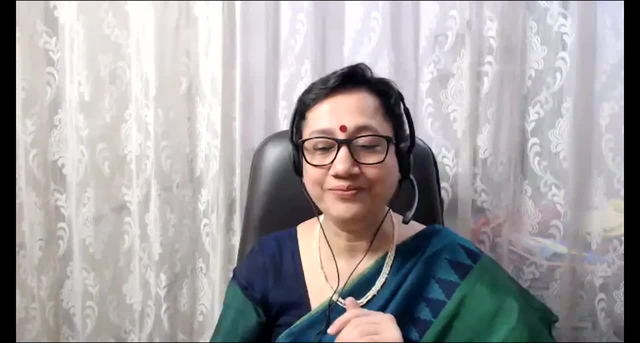 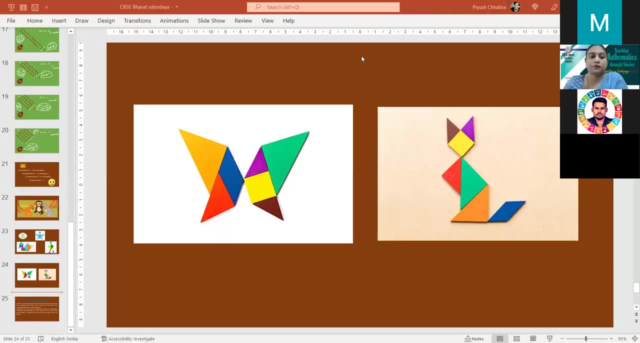 These are simple stories. And Then, Yes, Let me read the chat, Whatever you have written. Okay, Yes, Yes, Thank you Okay, Yes, Yeah, Yes, Face value: Yeah, Yeah, Take care, Okay. 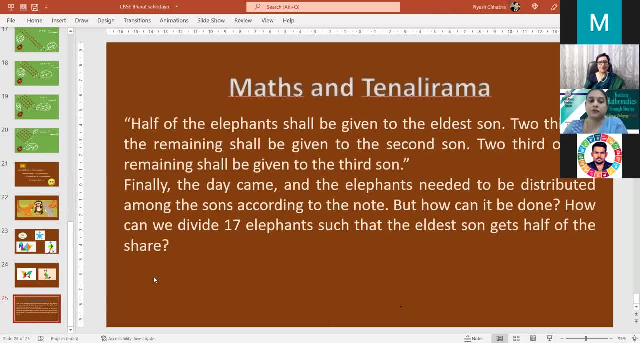 Thank you, Thank you. So now we have come to last story. Very simple story, But, yes, with Tenali Ram, Even Mulla Nasruddin stories are also sometimes Somewhere. you will find some of the things, And here this is once. 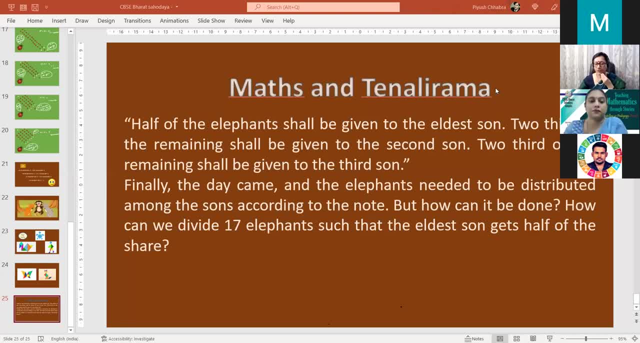 The king says to Tenali Ram: I don't know what to do. I have to give elephants to my children. So I have three sons, So the first one, The eldest son, should get the half, And I have only 17 elephants. 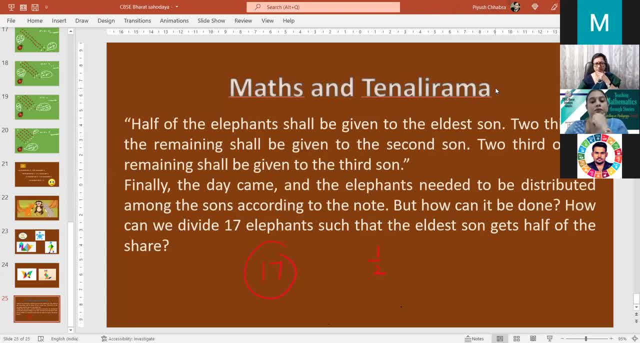 The eldest should get half, And then Whatever is left out of it. Then One third should be given, And then this should be given: two third, Two third will be given What is remaining of that, And again, whatever is remaining. 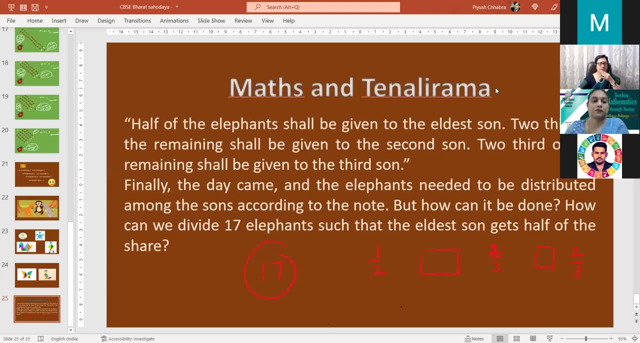 Two third will be given. Now Tenali Ram thinks and thinks What to do, How to do One more elephant. Then only I can do. So what does he do? He gets one elephant And it becomes 18.. Now, with the rule, what he said, 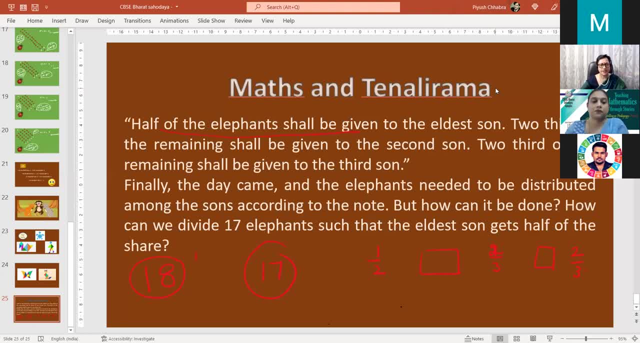 That half of the elephant should go to the eldest son. It means half means 18 by 9 becomes Half. half is equals to This 9.. So 9 is given to the eldest son, This one. Now we are left with only 9.. 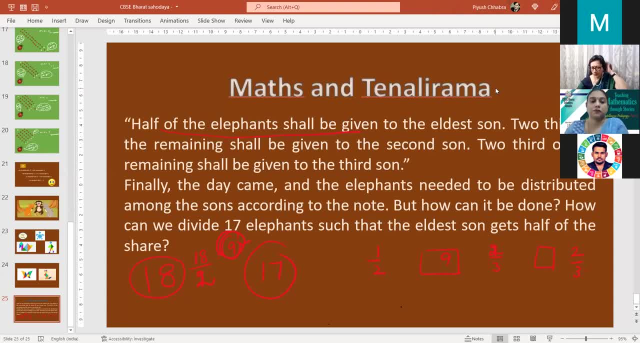 So out of 9.. Two third is to be given to the Youngest, The middle one, So this becomes Six, Six. he gives to the second one, And again, what is remaining out of What is remaining Three, And then out of three. 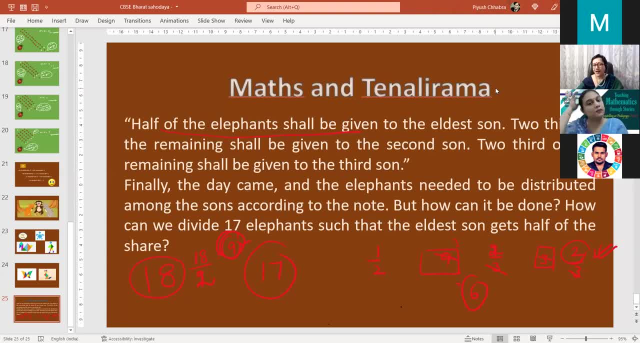 Again, two, third. So what happens? Two he has to give to the youngest. And how much is left now? Two, Six, eight And nine, Nine, eight, seventeen, And then one is left, One left again. he gives back What he had taken from the other person. 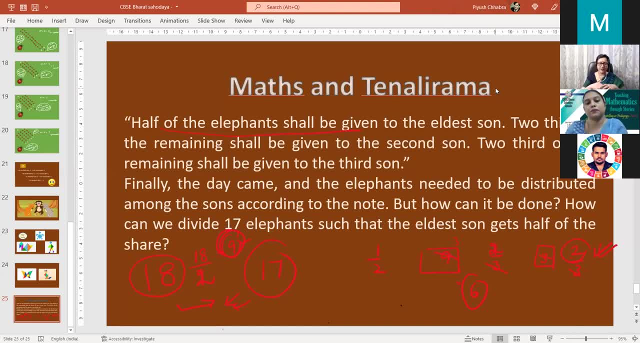 So in this way he solved. So in our stories also Panchatantra, I have told you We can just find out Tenali Raman, Even our, You can say Mulla Nasruddin also. You have to think. 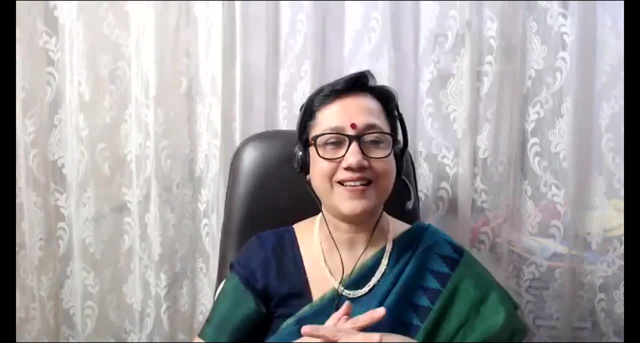 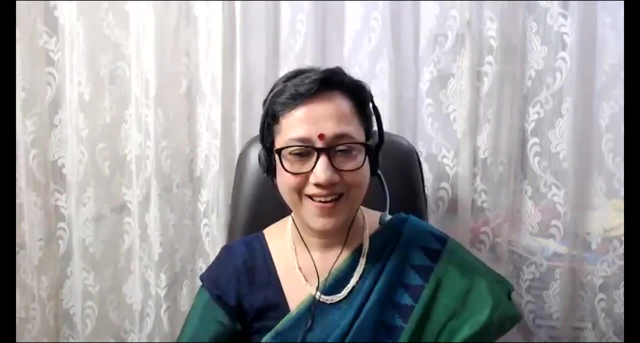 Then only you can do it. You have to add some interesting thing Into that. You have to add some flesh to it In a different way, Not whatever Like. simply you are writing. It will be same as the problems are there in the book. 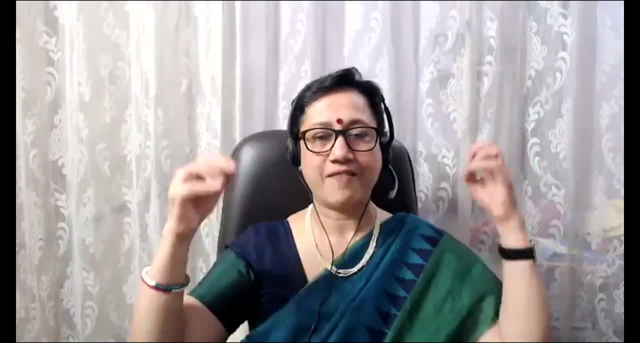 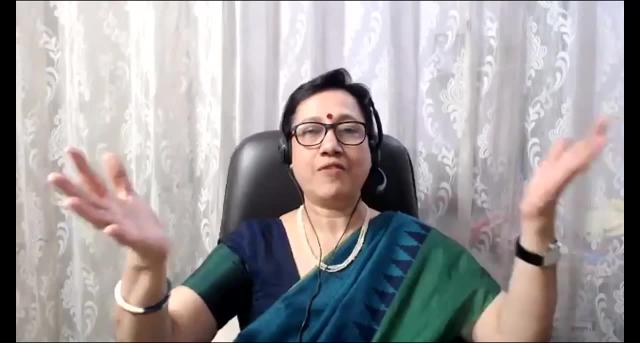 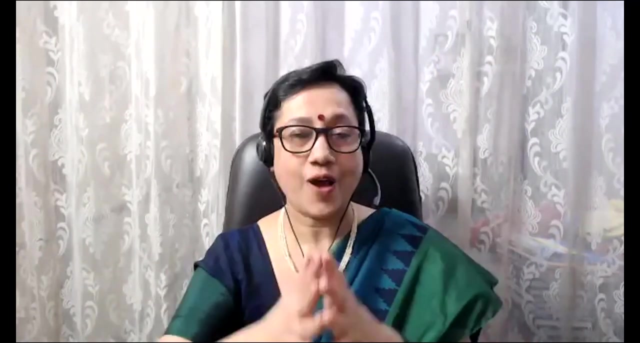 But here what I have done: I have given some environment, I have added some flesh, like this. So see I I am a storyteller. I have picked a few To make you understand How to pick up, How to make your story. 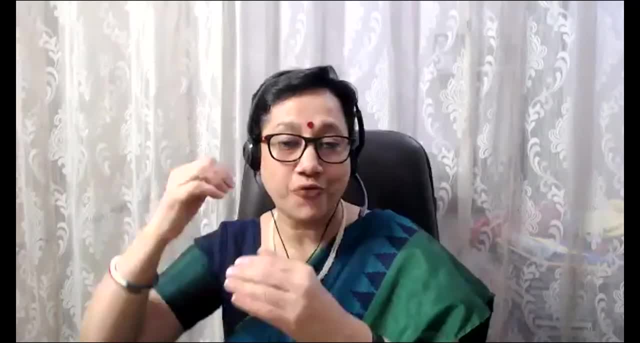 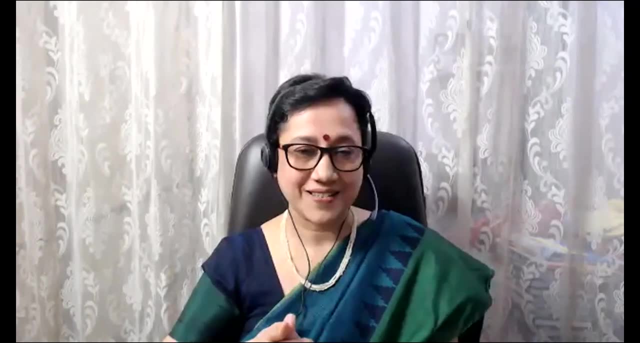 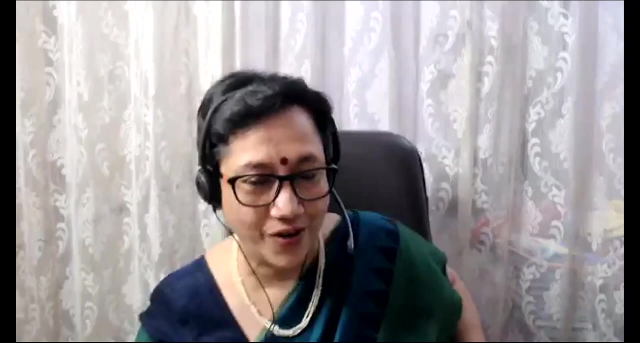 Now the concepts are yours. You have to fit in Your stories into that concept. Then only Children will enjoy the classes. It is up to you now How to get the story And then what I can. Now you are able to identify yourself. 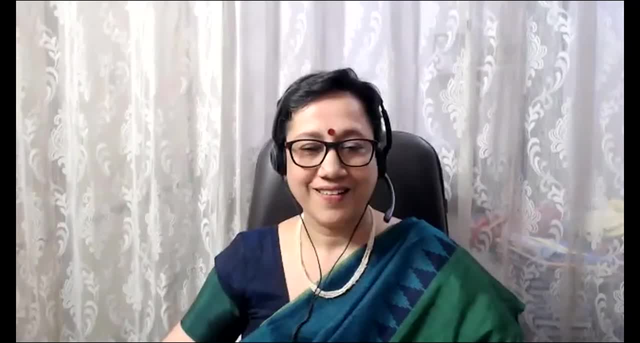 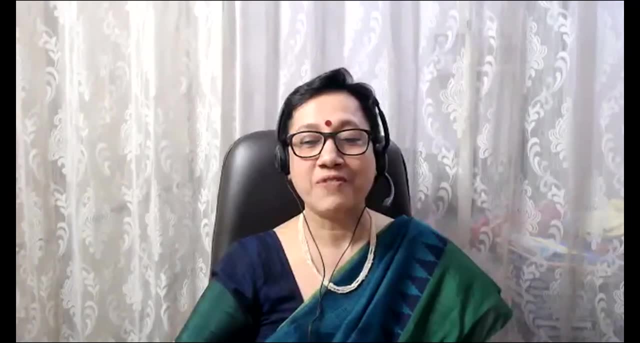 Only I didn't even ask And you had already written those things, So I hope you all enjoyed. Yes, I am getting your remarks. I am looking at them. Thank you everyone That you have enjoyed the session. You are understanding what I wanted. 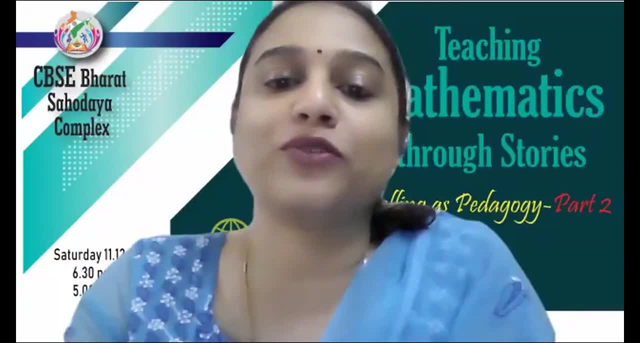 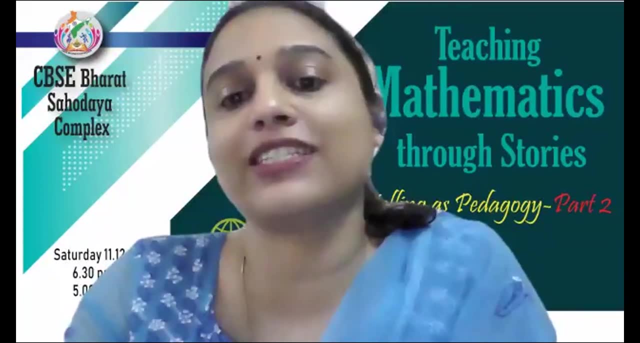 So I have tried my best. Thank you, Usha ma'am. Thank you, Usha ma'am, for such a wonderful session. You know, what I like the most Is the energy and the zest that you have. It is contagious And that is something. 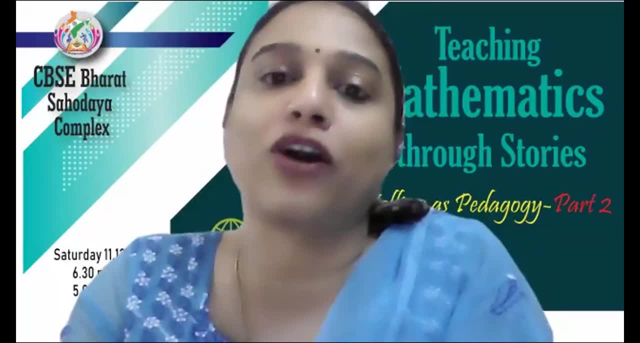 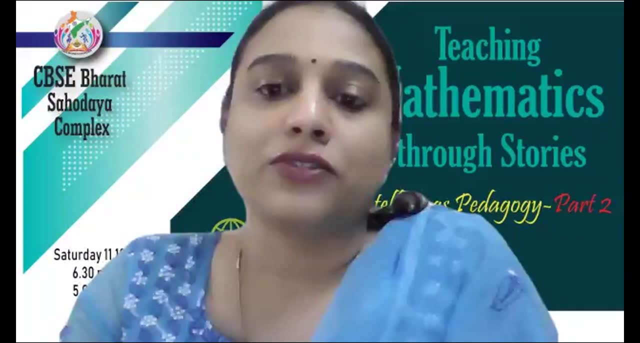 Which is so motivating for all of us Children, I believe They pick on our energy, They respond And they reciprocate in the same way. So I am sure all participants Will agree with me when I say That this session has provided us. 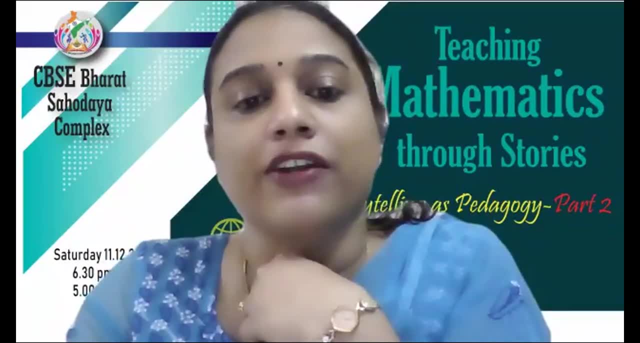 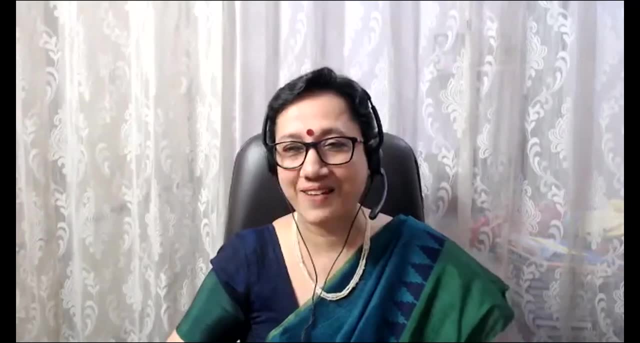 With a new perspective and enlightened us. Ma'am, I have a few questions That were raised by our participants During the registration process. May I go ahead with those? Let me see how far I can help them. Let me see One of the constant number of questions. 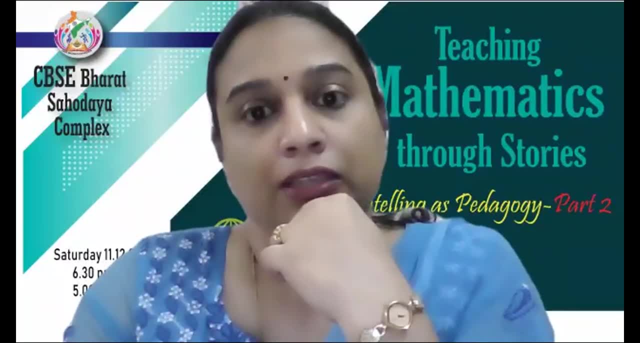 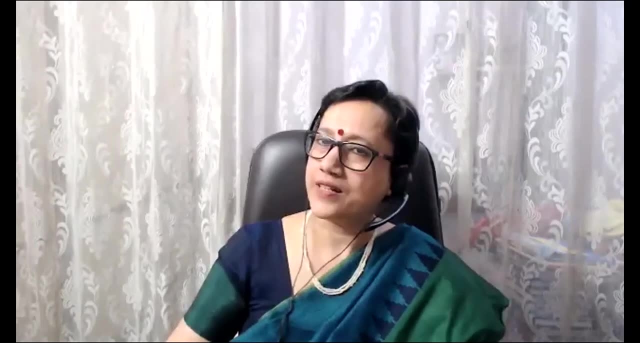 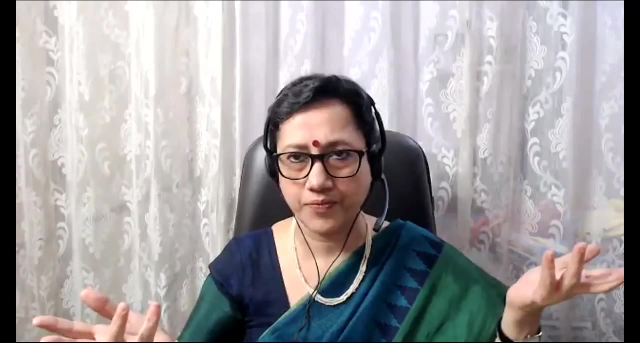 That I came across was In the senior classes. See, I told you the process. The process is same Whether it is junior, Whether it is senior. You have to understand the concept, What you want to do, And look out for some stories. 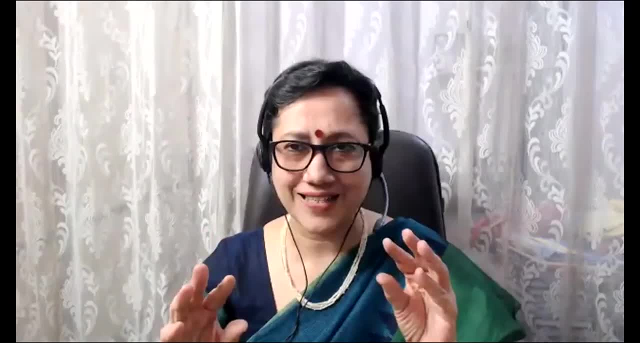 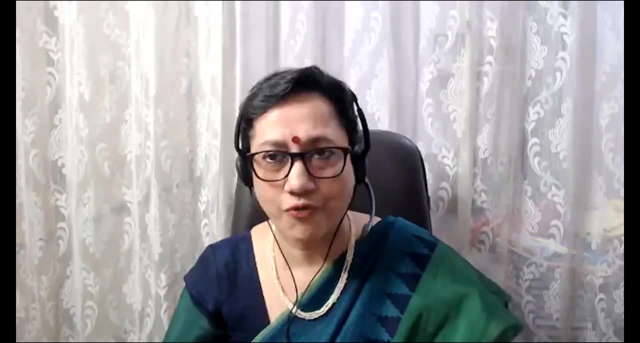 Or you make your stories, What you can do. Even you can do one simple story in the class And let children come out with the story. Then you will understand how they are, Because they are far, far ahead of us. So when you are picking any 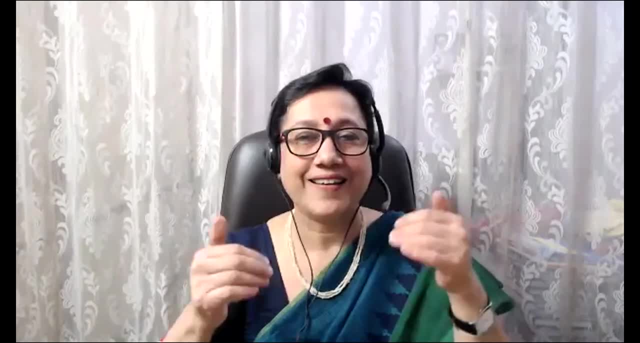 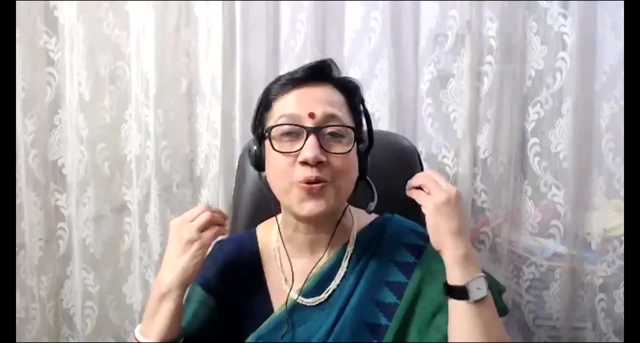 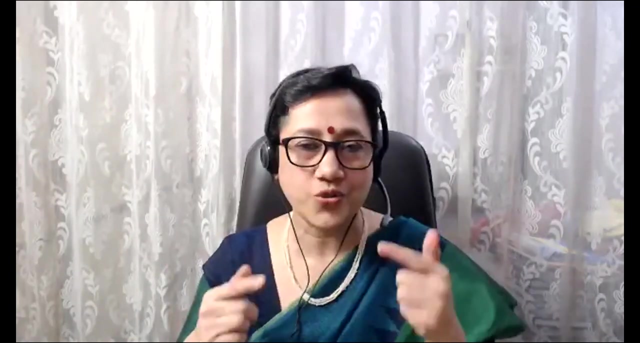 You try out first And then give it to children, Then you will see How they are doing it. They immediately take it Because they are playing so many games these days, You know, And in games so many characters, So many things they are learning. 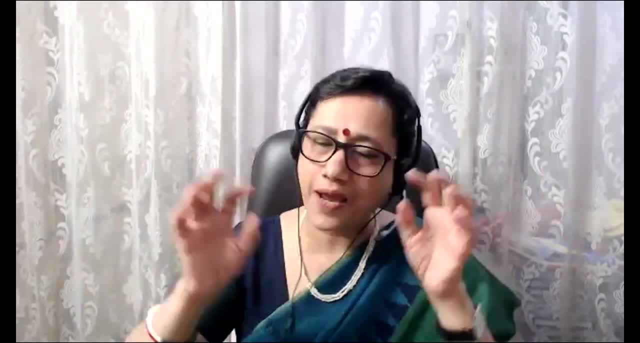 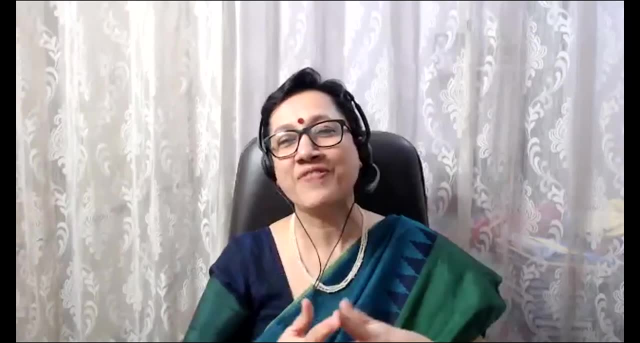 So once you have understood my process, How I am doing with it, Then you will be able to incorporate your things. Story telling: Mostly people think that it is for junior classes, But I feel It is for all the classes. It is up to you. 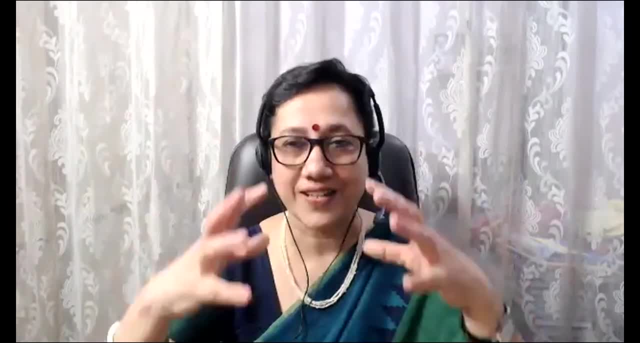 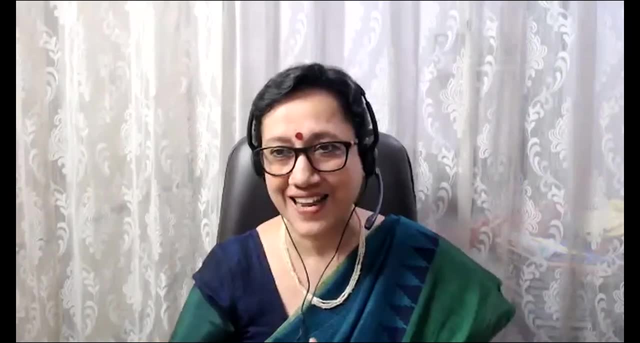 See, I am a story teller. I can tell you how to make your story interesting, But you have to find out, As I have shown. Maybe I have done, I think, four or five stories I have done today, I don't know. 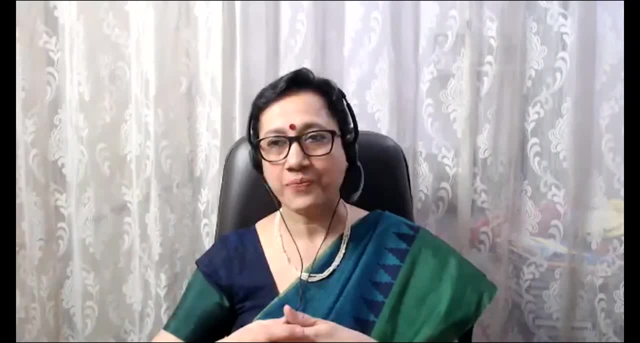 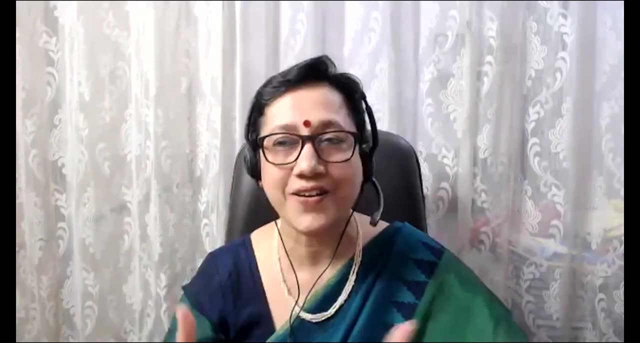 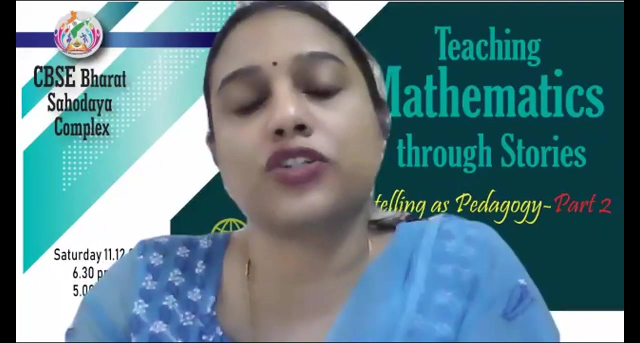 Right, And so many stories. through different stories, I have told you how to weave that. Weaving is my area. Your area is to find out the story. Bone structure. Okay, ma'am, This is quite an interesting question Someone has asked. 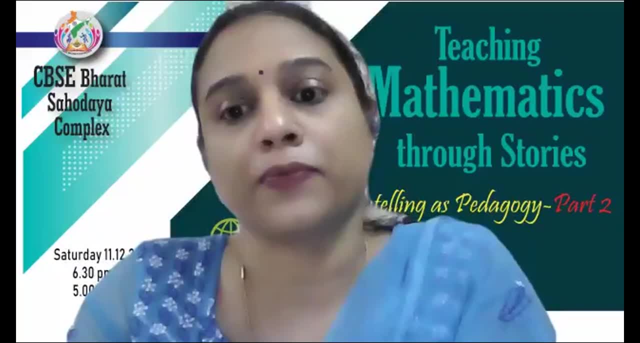 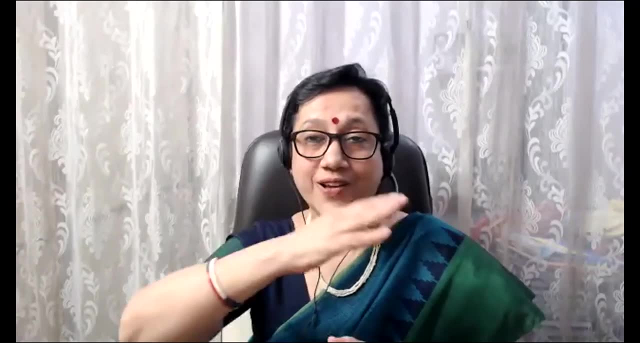 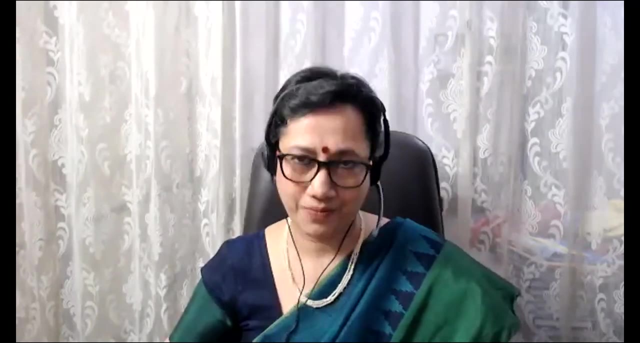 How can storytelling be implemented for students Who are on the autism spectrum? See, Yeah, Autism Is also actually a big spectrum, Right, Different types of autism. So I think special educators And the parents And the teacher, They all have to be at the same page. 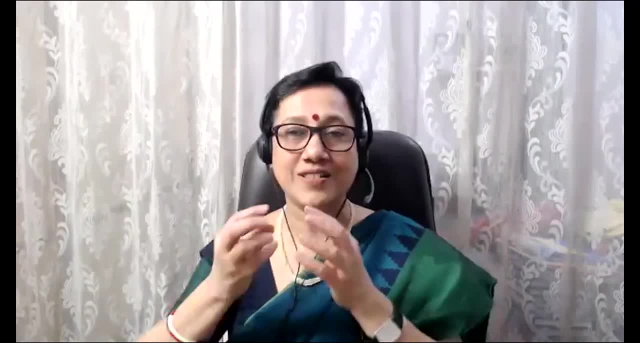 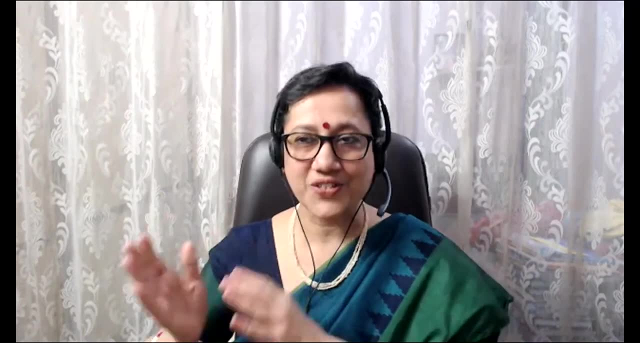 They have to invite them. All three of them should sit together, Because whatever the teacher is trying to impart Should be told to the parent And the special educator also, Because these children are taken care of By special educator also. So whatever methodology, 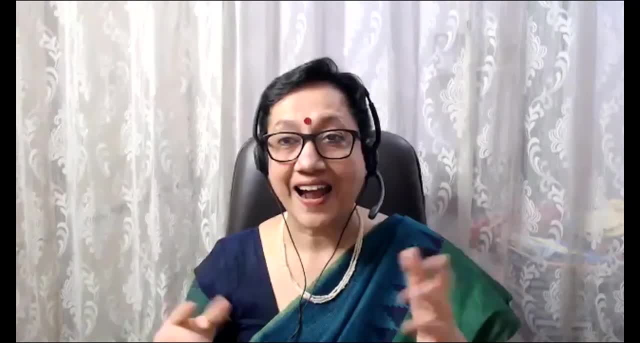 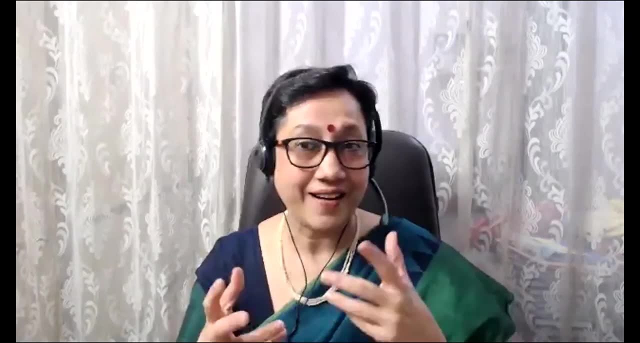 The story she is doing with that child. It has to be repeated And these children pick up very fast. I tell you This I have seen, Because, yeah, Maybe you feel that they are understanding. So if you tell them through stories, 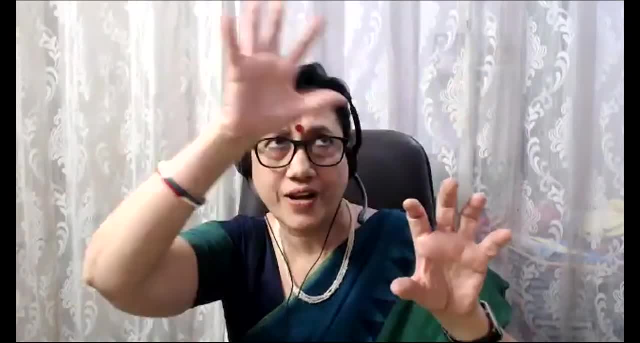 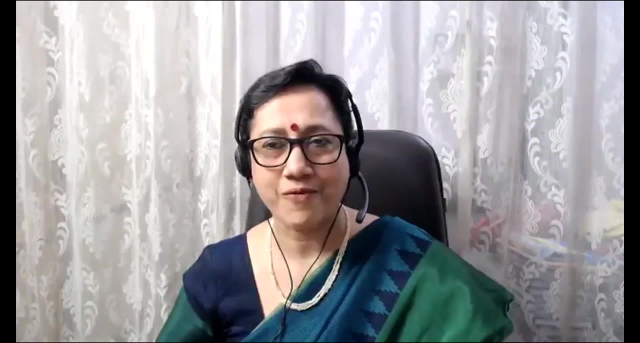 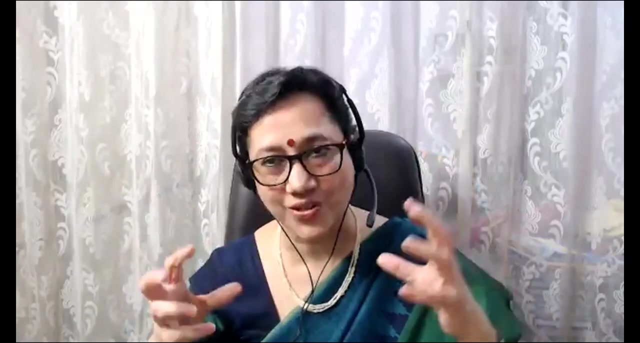 Or pictures. You can make pictures Like a story in the form of pictures And show it to them, Because I have also seen- I have got a few children When I was teaching in that school. So, yes, They learn fast. 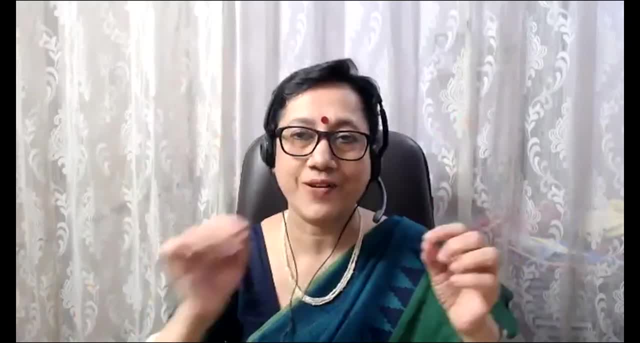 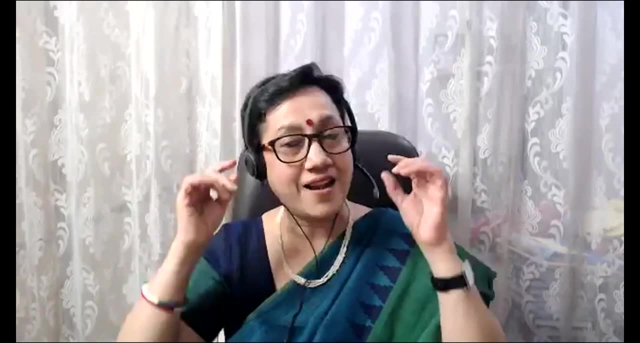 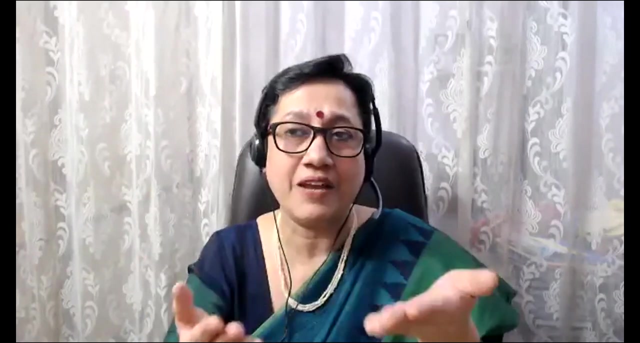 Pictures also, Colors also, So maybe you have to use different colors For different characters And they draw also And they understand very fast the concepts. So once you tell them, Make a story, You just give some idea. Maybe you can give a book to them. 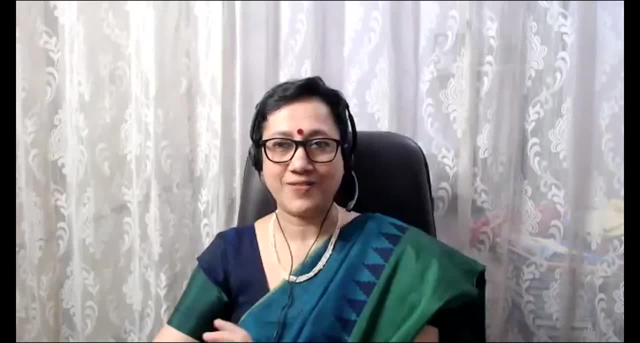 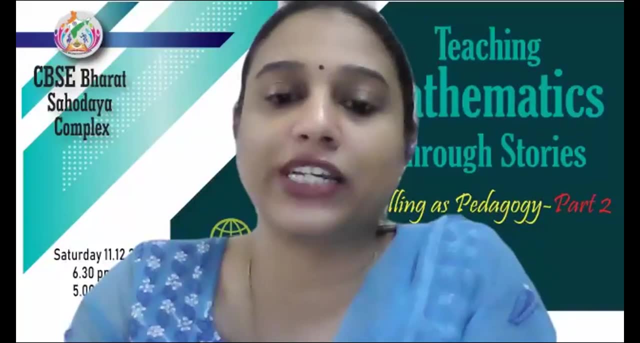 See, this story is there And then they do it wonderfully. I have actually seen myself, So I can say it. Thank you, ma'am. One more question. I am sure this has come from one of the teachers. I could relate to it to a large extent. 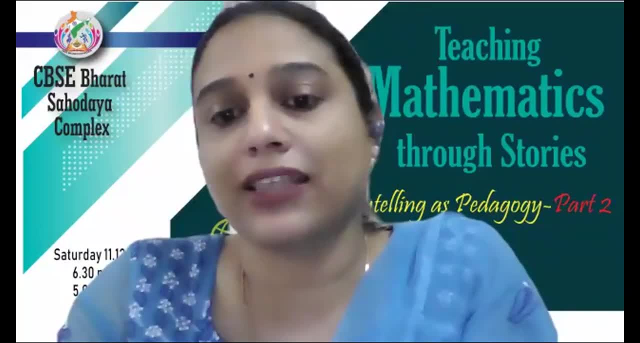 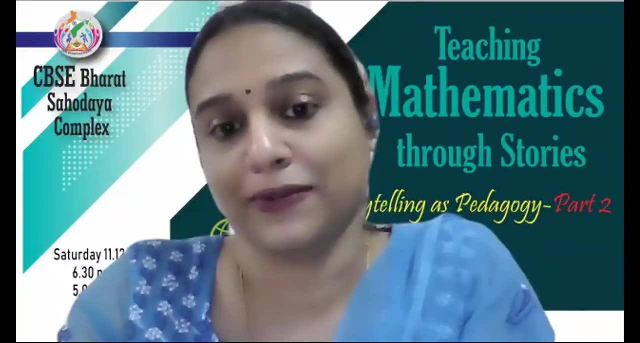 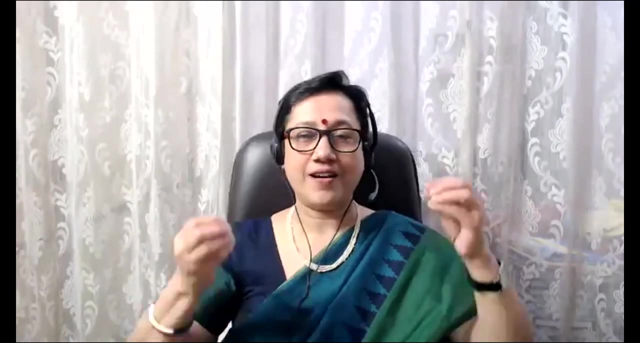 So ma'am says Art, integration and storytelling in math is fun, But shouldn't teachers Spend more time on solving more problems? Since math is all about practice Here, I will just Immediately, I will just stop you here In between. Listen carefully. 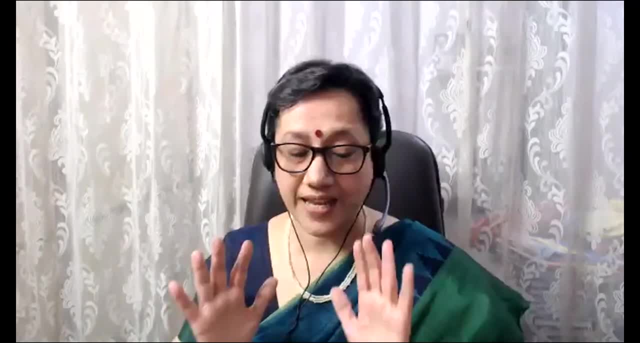 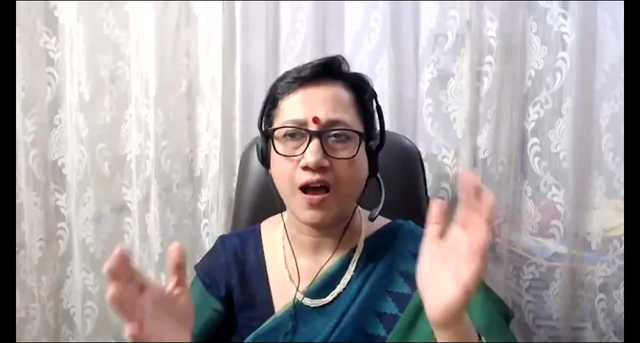 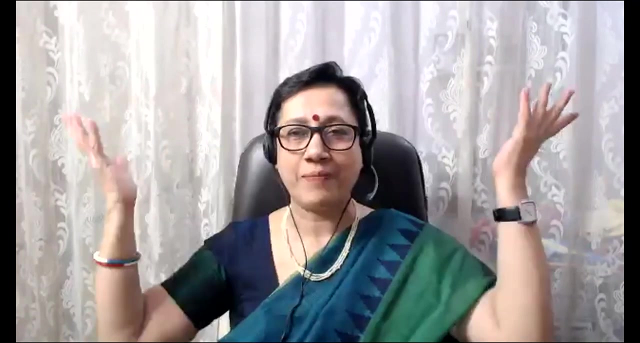 When we are introducing a topic. See, I have done five stories In front of you And explaining the whole process Also within an hour. One story will hardly take Five minutes, That's all. But your class will become From here, it will jump to that. 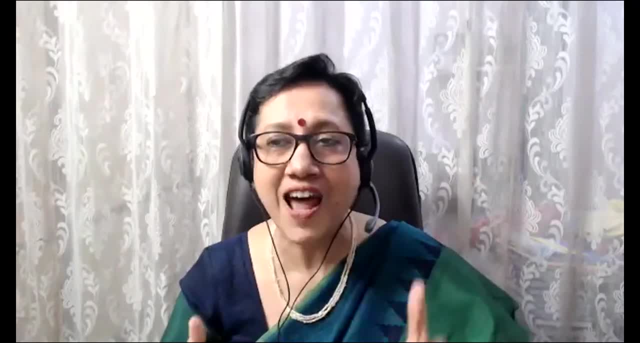 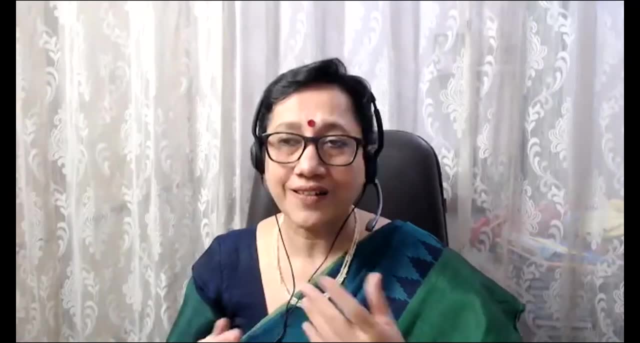 And you have seen yourself When teachers were giving the feedback, How many children in the class Love math: 50%, 40%, 30%. Even someone said Out of 40, only 5 to 7 children Because they are not getting hooked. 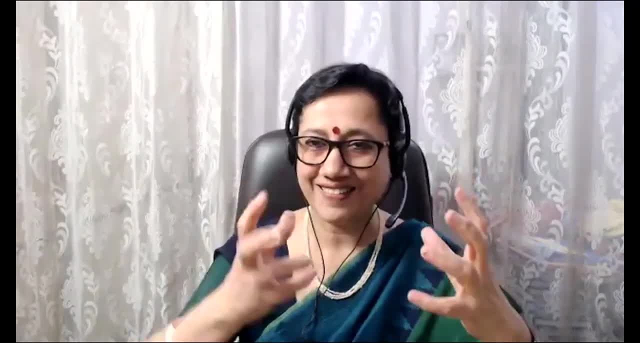 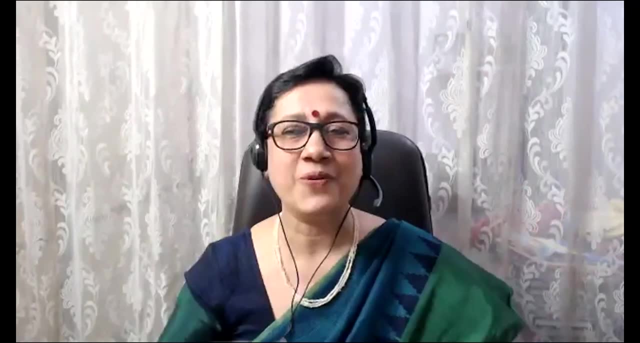 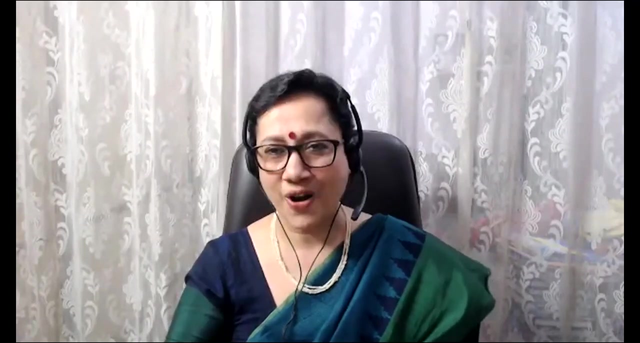 So this storytelling is the best tool For hooking a child For a topic. You can give one period to them Make your own stories. Give them one period You can borrow from someone. Okay, you have finished your course, So all this can be done in revision also. 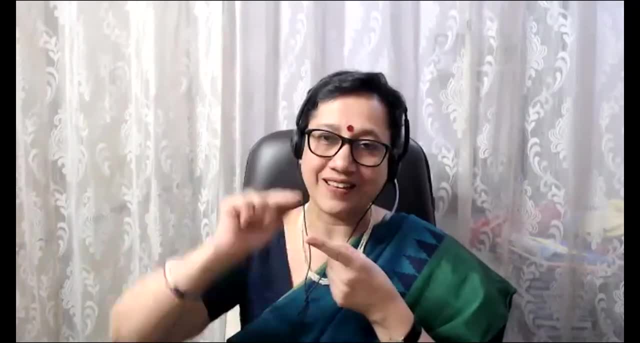 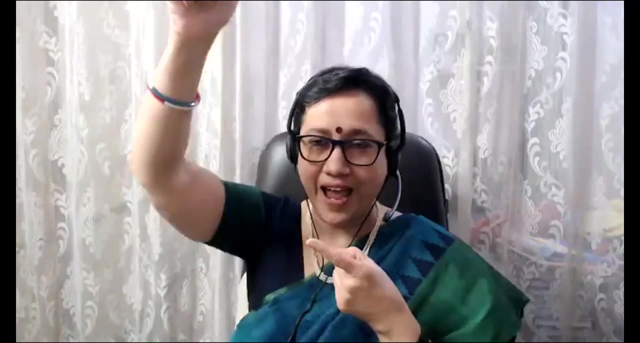 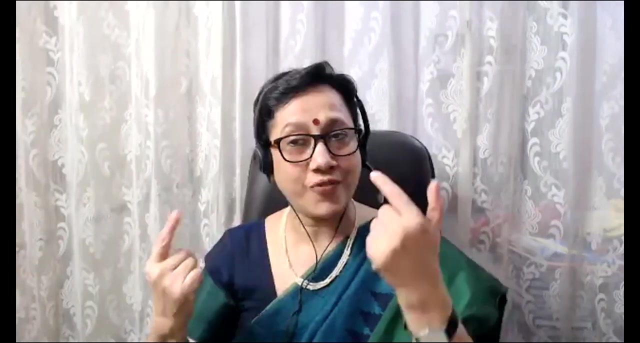 So what I feel Our aim is to improve The understanding, Make them interested in our subject. Okay, So when we have the higher aim, Then all these things will vanish. at that time, Hardly five minutes For a story Introducing the concept. 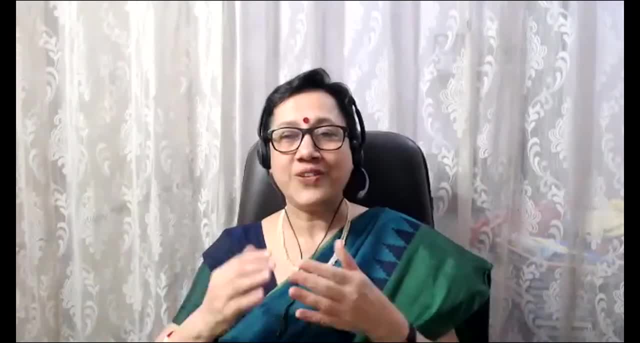 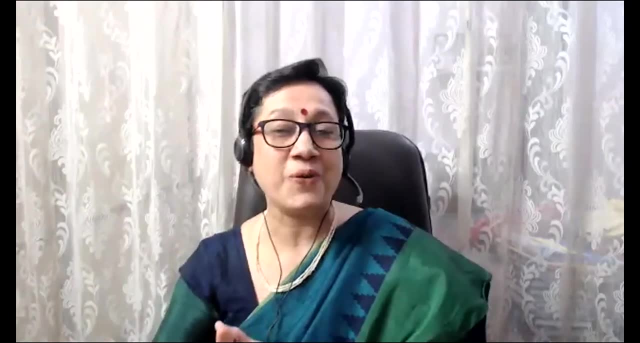 And giving them one period To make your own stories, I feel that your class results Will improve from here to here. They will be just looking out from the classroom Waiting for you. What do you want? You want to solve more problems. 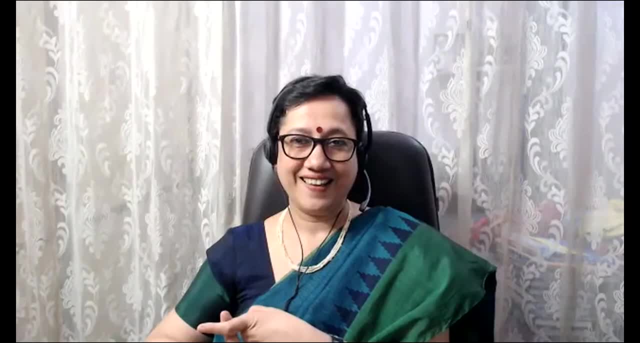 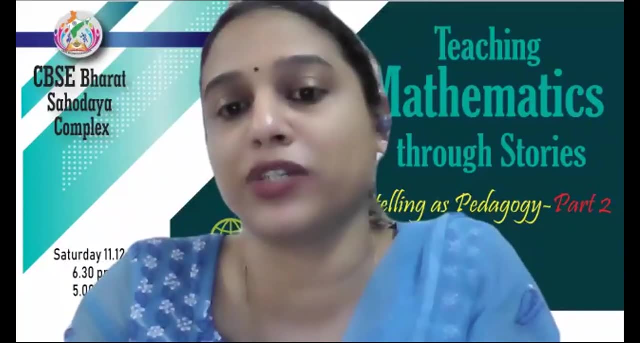 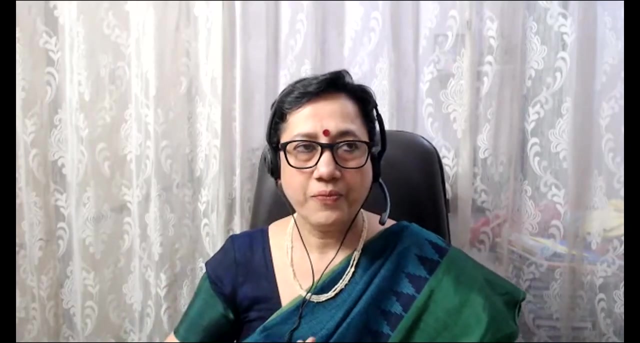 No, they can solve their own And they will remember those problems Which they had enacted in the classroom. And I also believe This solves the next question automatically. One more thing is there, Because sometimes I feel Children don't understand What is the importance of this topic. 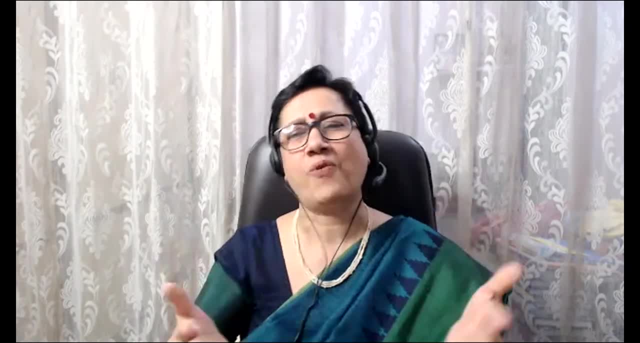 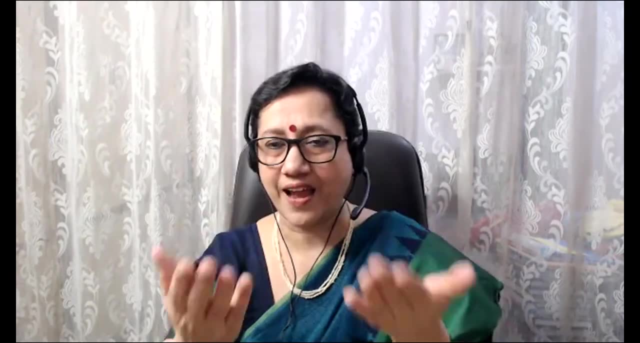 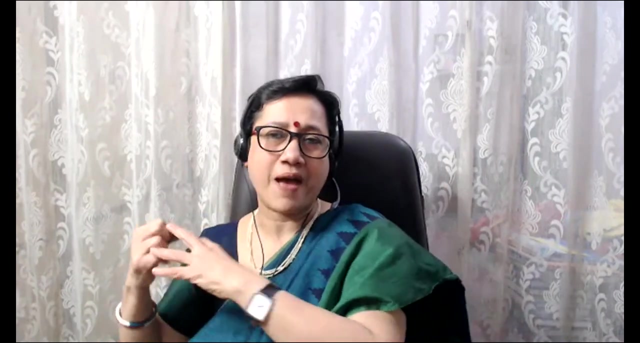 In my life. So if we emphasize on the importance, As I started my whole session, Where do you find maths, Those children Who are just away from maths? They don't like it, There is some phobia- And ask simple questions in the class. 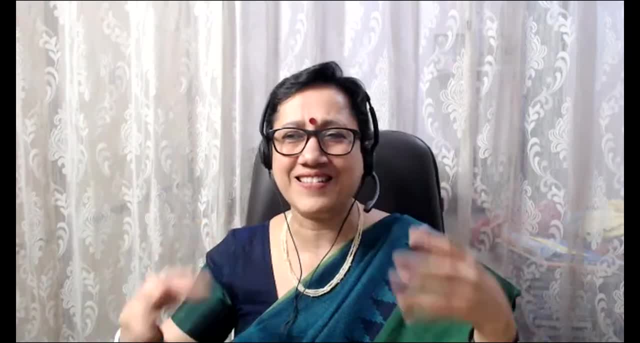 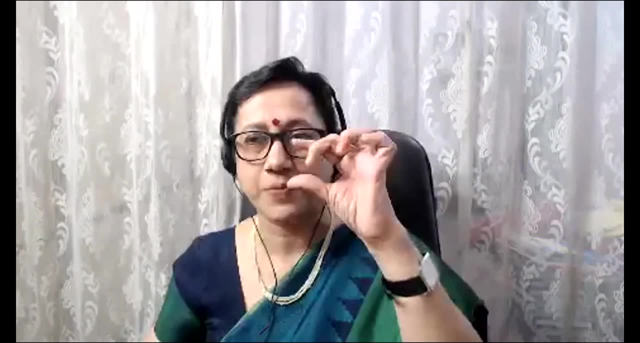 And they will remember And ask simple questions in the class. Don't give high type questions Because, see, Hots are also what we do. Hots question also. we give very less percentage. Mostly we see average, Even give below average questions. 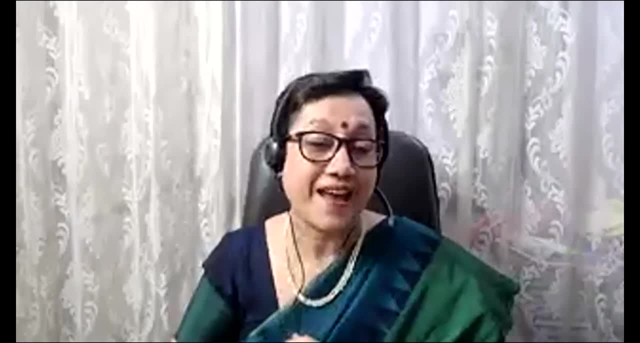 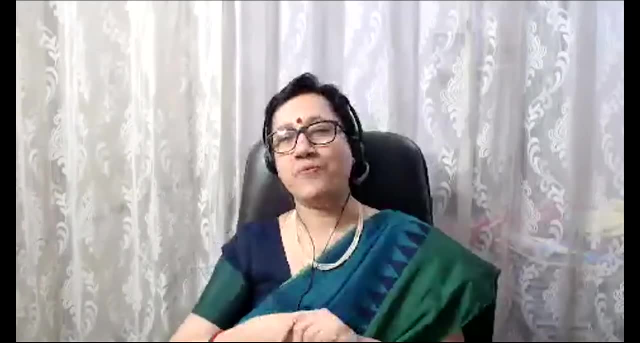 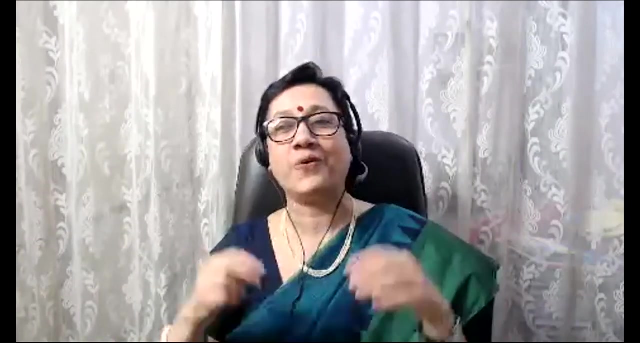 In the beginning, Just to make fun. Okay, these children will feel, Okay, I can do it. First let them have confidence Of I can do it, Then there won't be any phobia. And if phobia is there, Then they will understand. 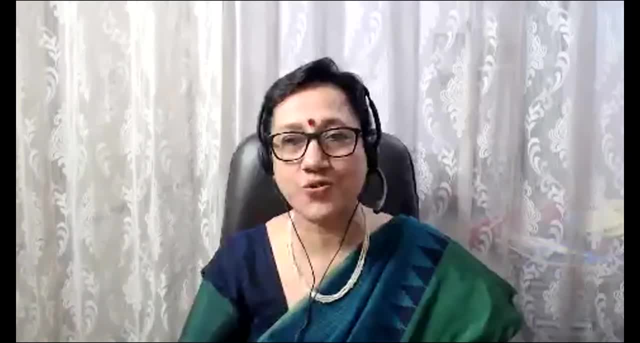 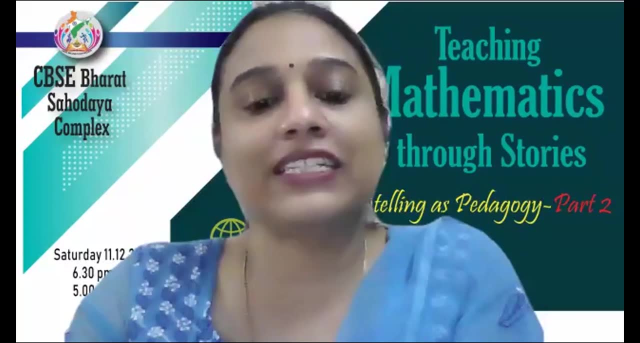 I have seen story telling doing magic, Today also. you have seen Wonderfully. you all have understood, And I am not a maths teacher. I am telling you, I have done story telling. This is a very practical question. Could you please suggest websites on apps? 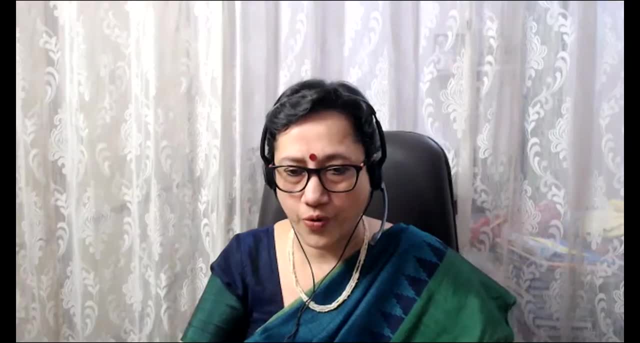 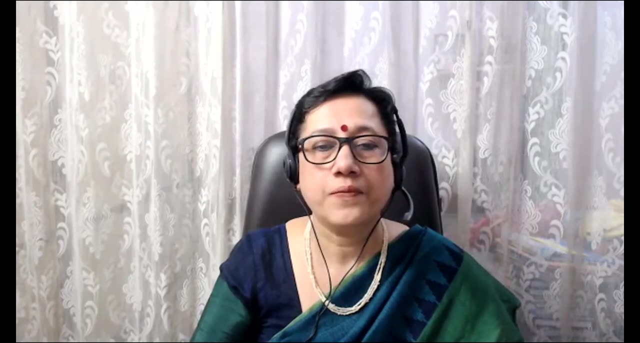 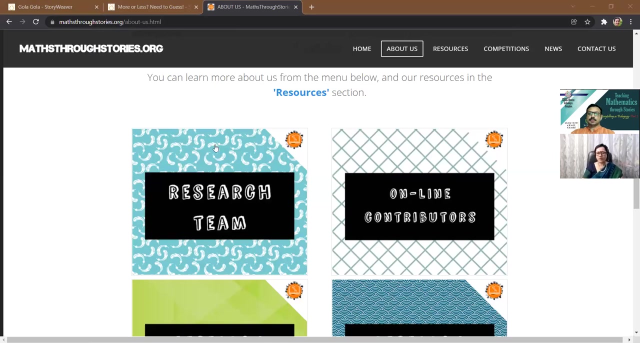 That can strengthen story telling. See websites, I am telling you. I will show you some of the things. Very, very important websites. Yeah, I am telling you. Wait, It is very interesting. Maths through stories dot org. You are able to see, I hope. 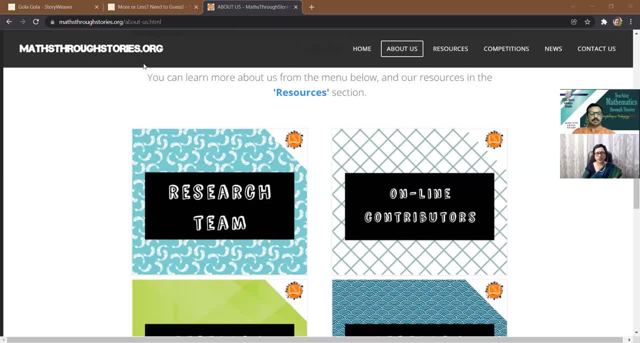 Yes, ma'am. Okay, Maths through stories dot org. This is a good resource Here. they have given many books You have. maybe you can buy books. Or I will suggest you go to your library, Go for story books And try to think. 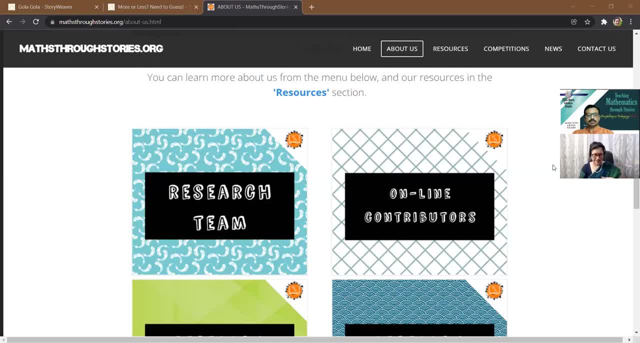 As I have done. I have read story books From those stories The characters somewhere I have added also I have not taken fully the same, So you can also go to children small, Like your junior school library Over there you will get good stories. 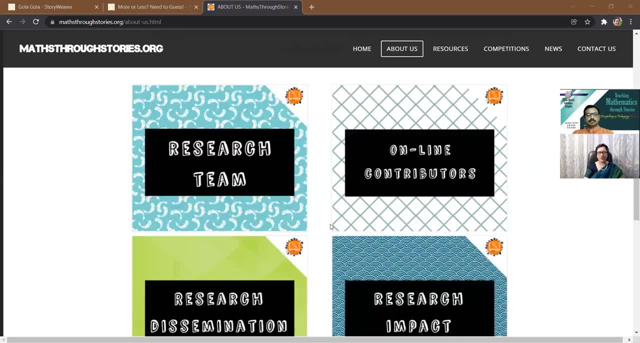 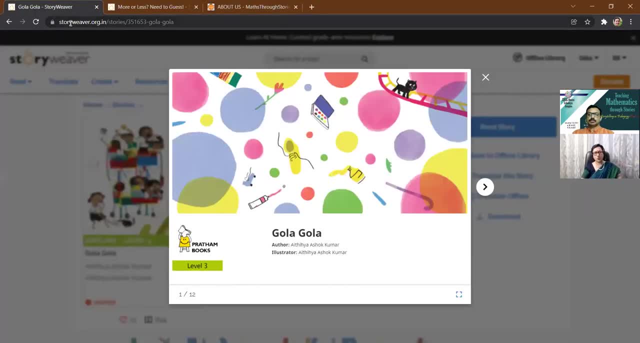 And from there you can, Because here also they have what they are doing. They are using so many books. Now there is one more website I will tell you: Story weaver. Now see here in the story weaver They have given the story. 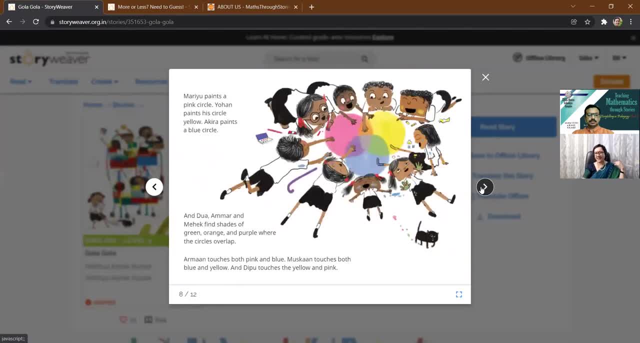 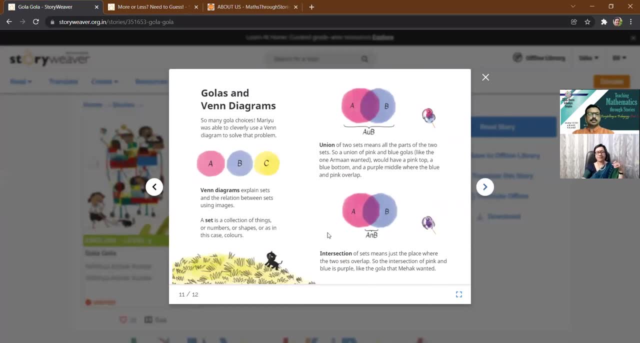 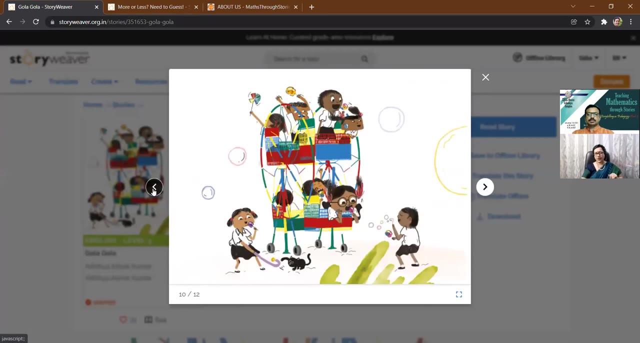 And it is actually going to Tell about Venn diagram. You will see They are talking about Venn diagram, Such a big concept of Venn diagram. What is set? What is union intersection? So easily they have done, With the help of this story. 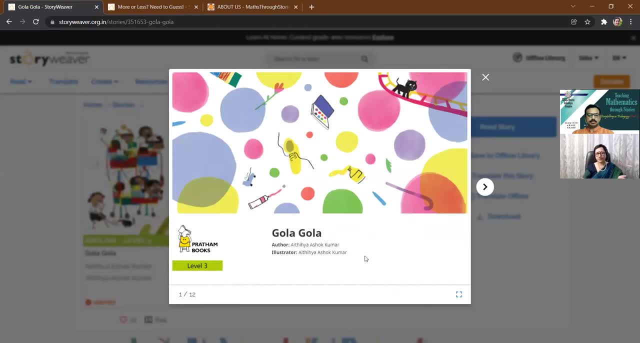 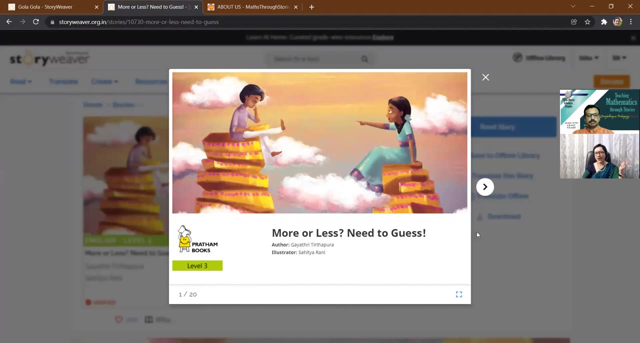 So this is on story weaver, Pratham books, Beautiful story And this is story weaver dot com. Yes, Story weaver dot org. dot in So easily. you will see this story More or less. This is also in Pratham books, story weaver. 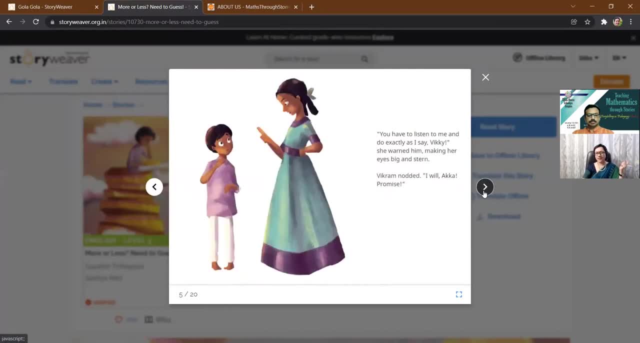 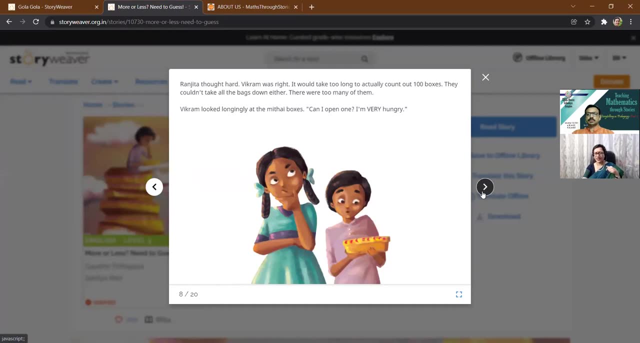 More or less. And then here they have to Pile up these things In hundreds or tens. They have to take the laddu boxes Downstairs. There is a function going on, And then they try how to make sets. 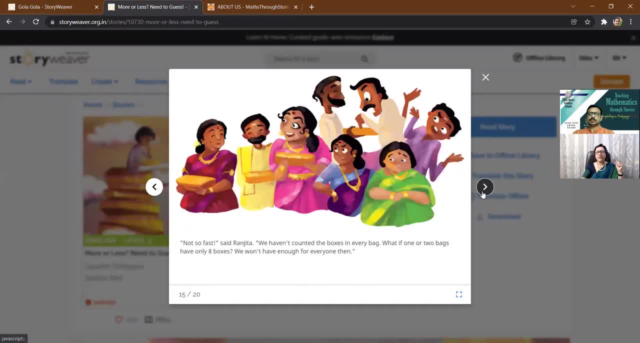 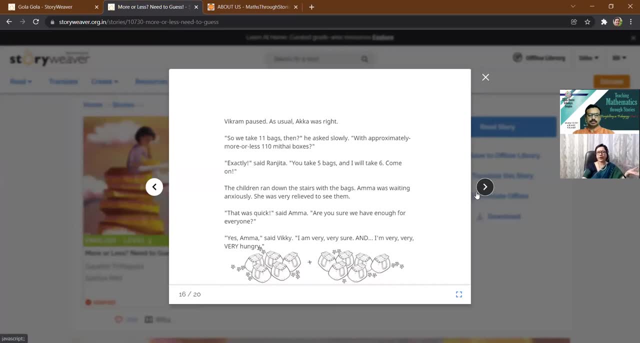 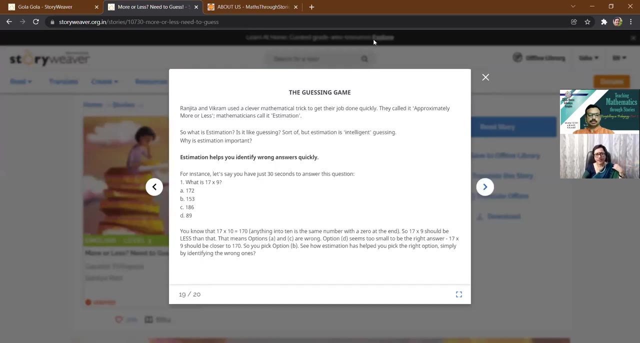 And more or less They have understood. So if you go through the books, You will get some math books And you can put those stories And fit your math into it, As I did today. Okay, Ma'am, another question. One last question. 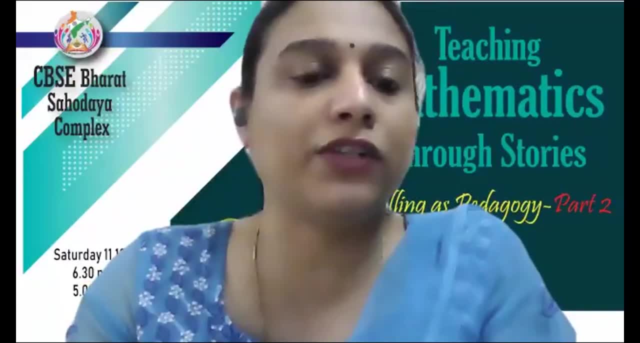 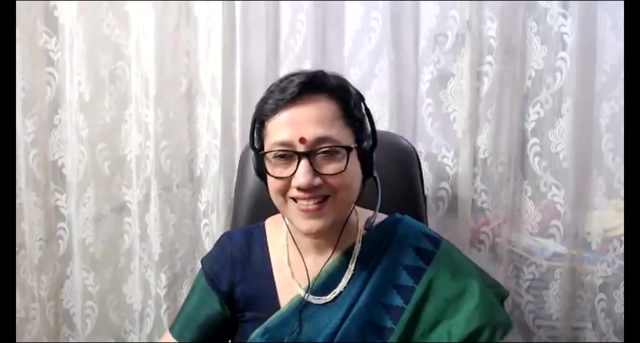 What should be the, The kindergarteners especially. The attention span of the talks Is really small, So one teacher wants you to know What should be the length of story So that we can keep them engaged. Yes, So if you have children, 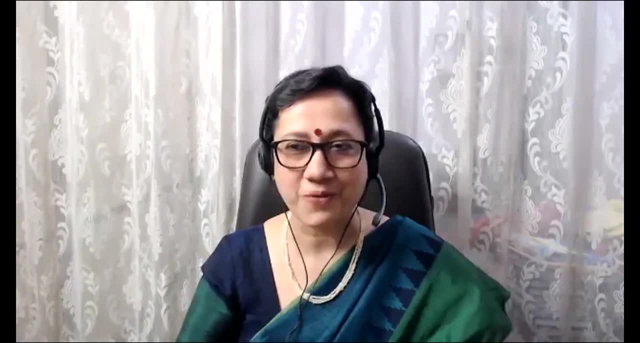 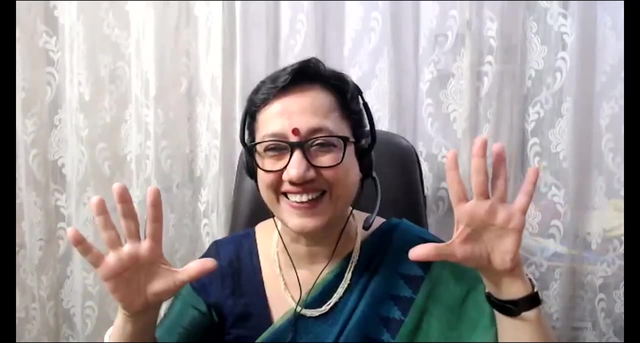 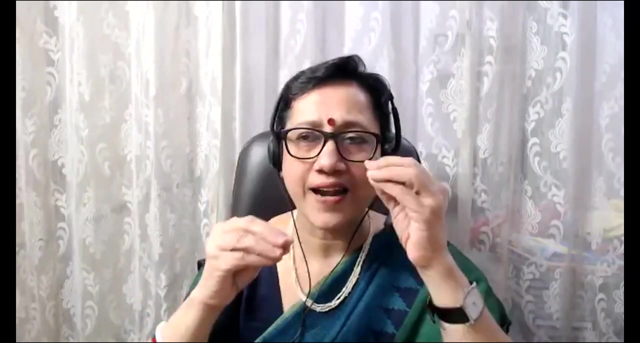 At this age. I have given storytelling sessions to them also. If your story, You make it interesting With your voice, modulation And props and all They will just keep looking at you. The magic is there. It's not in the concept. 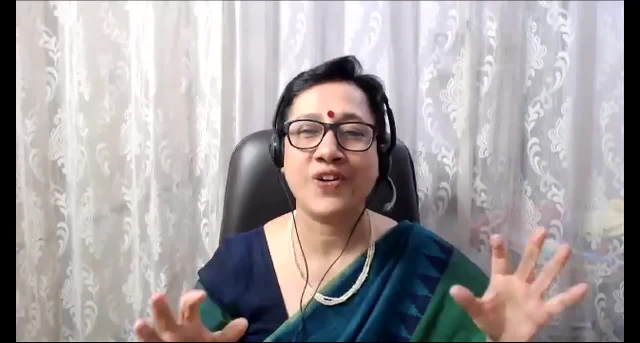 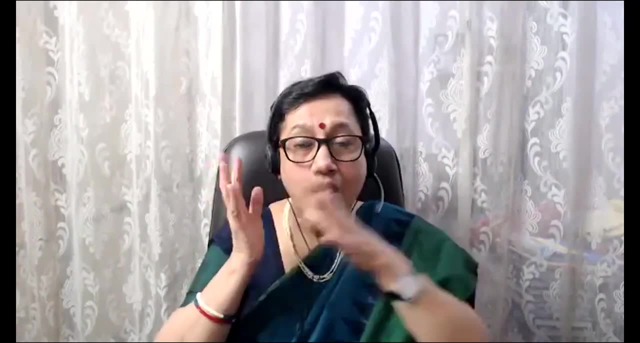 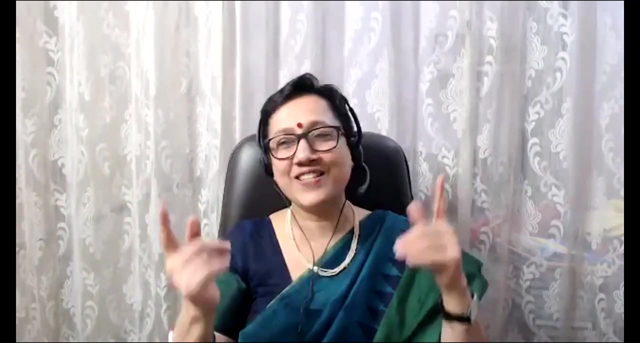 The magic is there. Maybe you can add some songs for them. Otherwise, the magic is your voice modulation And your props. Oh See what he has done. Oh, Now, what will he do? Then they will all answer. So don't give them a chance to get bored. 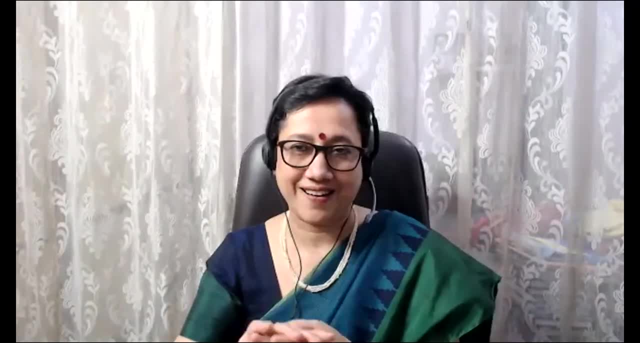 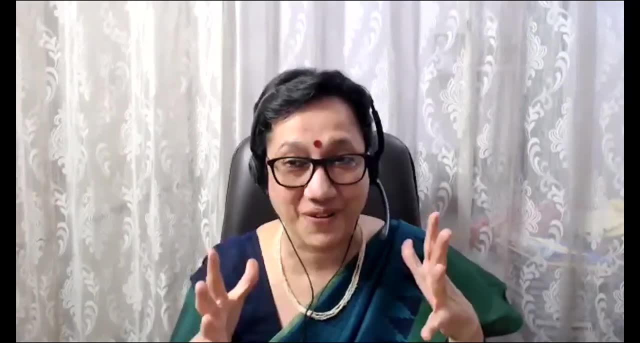 These children Immediately will run away from there. So this is our target over there: Like to make it so interesting, So lively, That children just don't turn away their faces. They will just look at you And the story time should be. 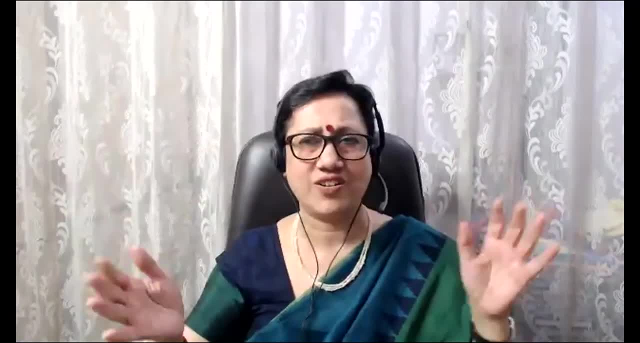 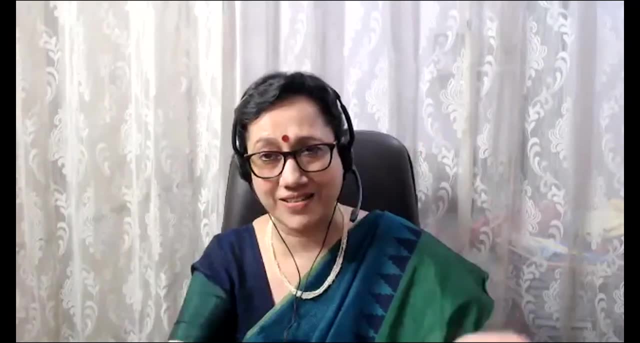 Three, four minutes Enough For higher children also, Even for the smaller ones. Four minute, three minute story will do, And then they will start making. You will see hundreds of stories. They will just will not be able to sit there. 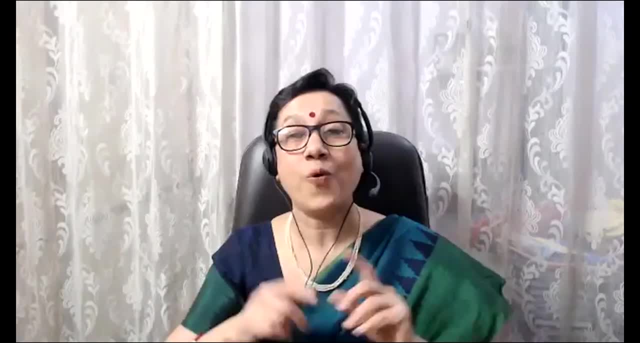 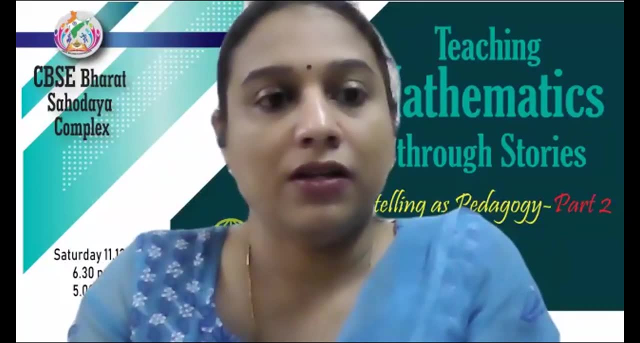 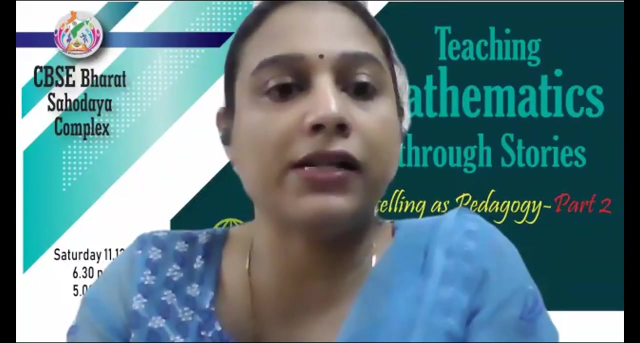 Ma'am, I will tell you a story, Ma'am, I, And that's what we want: Children to speak, Children to think And make their own questions. Ma'am, can we take a few questions from the participants now? Yes, Sir, can we unmute the participants? 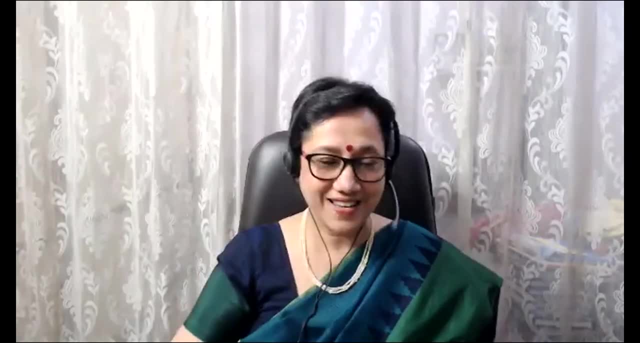 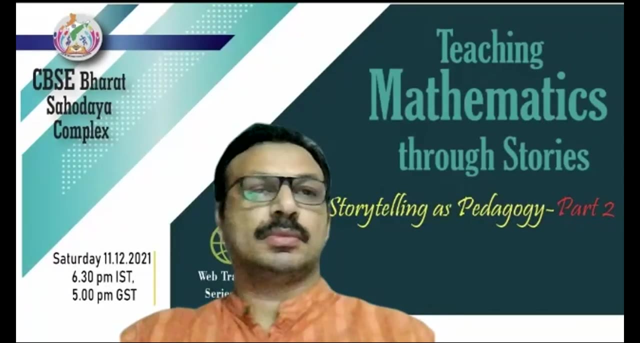 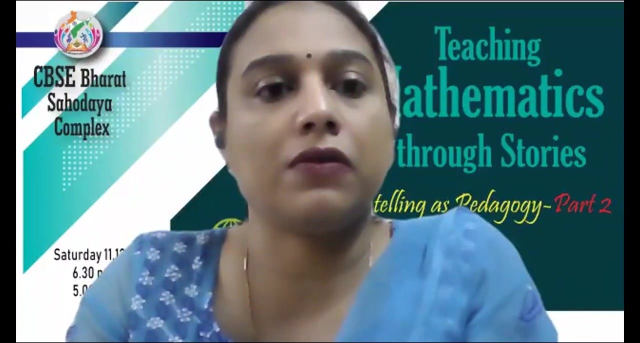 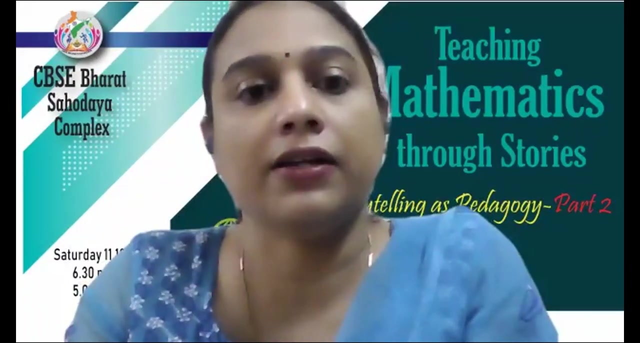 Yeah, let me see, Because, let me see what questions. Yes, yes, Ma'am, Ma'am, are you able to unmute yourself? You go to next one, Sir. Yes, Come on hold on. Very good evening to everyone. Am I audible? 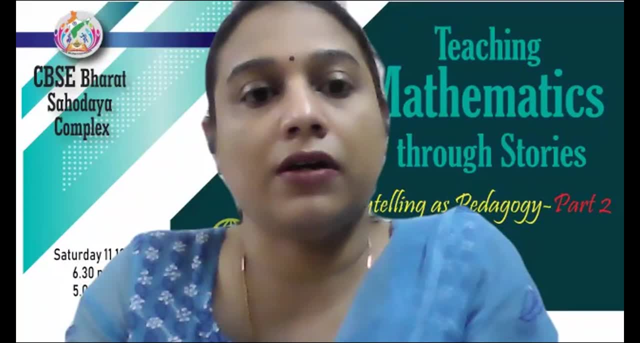 Yes, So, Ma'am, this is not a question. actually, My question has already been answered by Usha ma'am. Usha ma'am, I must tell you this session has been amazing. Why I endorsed that is: I just left from school after the examination work. 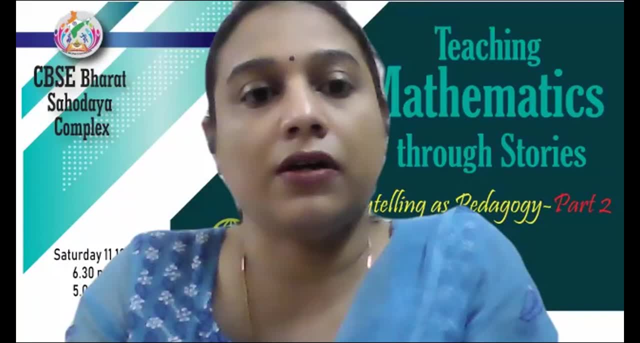 And I was on my way, When I was just listening to you, I didn't have access to the, access to the- uh, you know the ppts and all. but let me tell you, ma'am, the entire duration i've been stuck to your voice and i think this, this has done the wonders, that, the magic that you're. 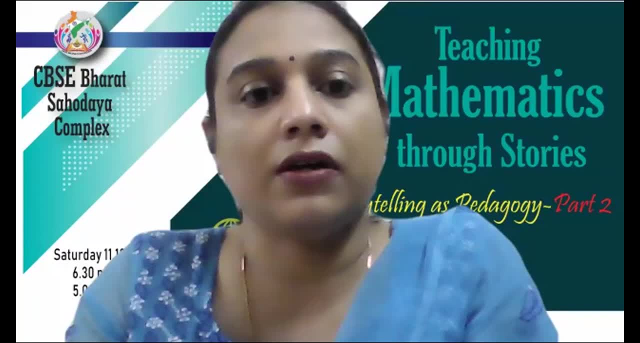 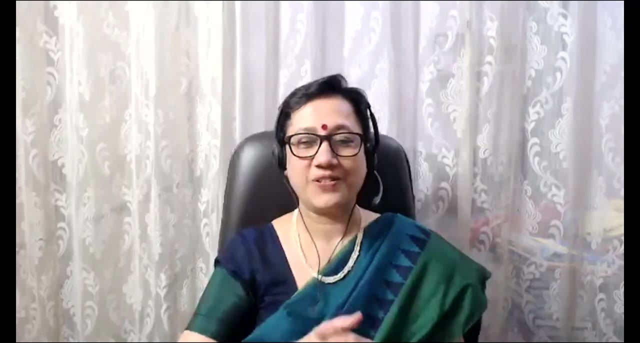 talking about. we have to create that interest in the students and practice will follow automatically. i absolutely resonate with that and thank you so much for this session. uh, uh, that's it, ma'am. there was no question from my end. thank you so much. thank you so much that you enjoyed and. 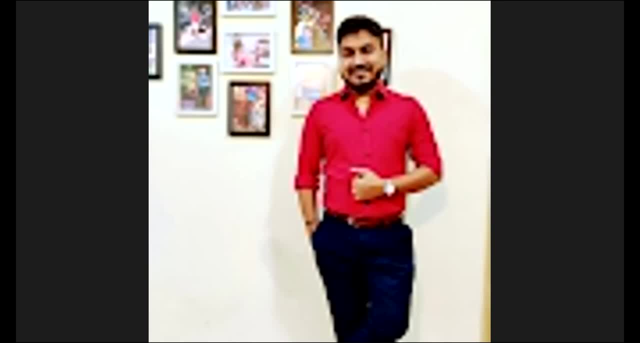 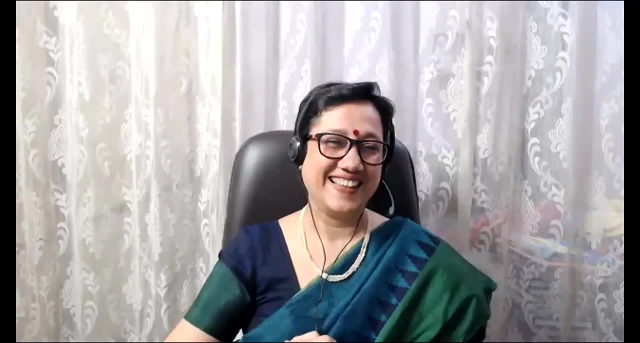 you were stuck with that. thank you. my last one hour i've been like i'm reaching home, i'm yet to reach home, and this entire duration has been amazing, as if i'm listening to radio and i'm just learning mathematics in a new format. yeah, thank you. so much on me, thank you. 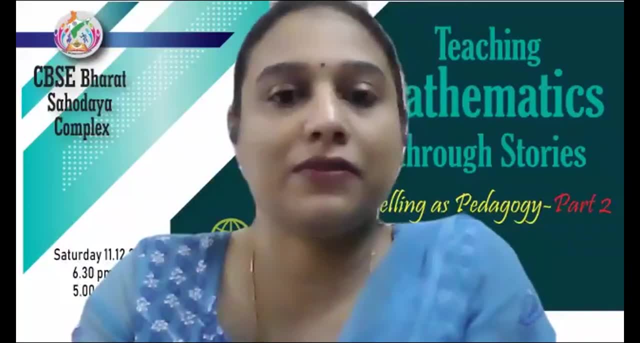 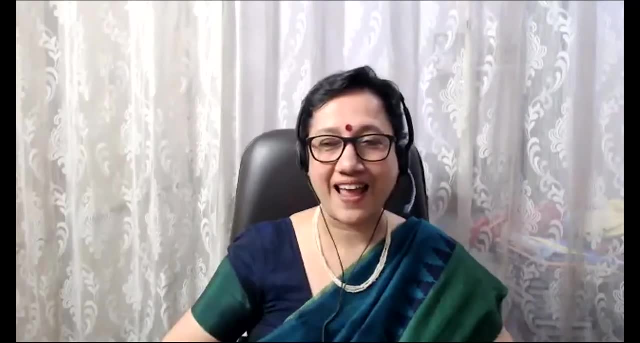 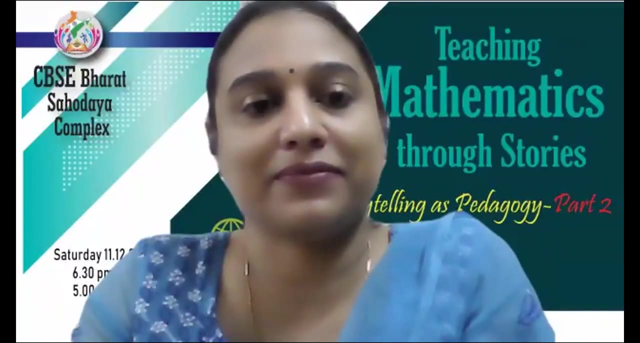 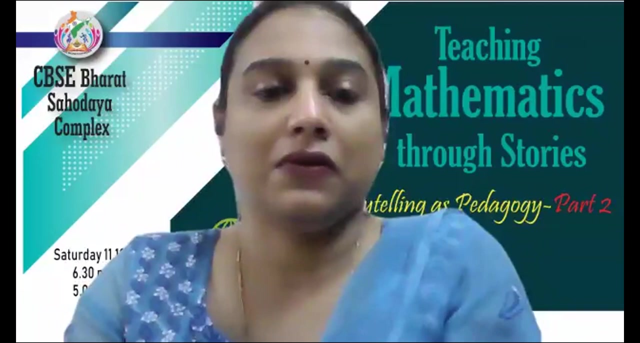 actually miss tomo. mr tomo had, uh, you know, a lot of questions in the beginning. i could, okay, but i hope i have answered all because he didn't have any. i yes, good evening ma'am. a very interesting session i have had, and i am an english teacher. 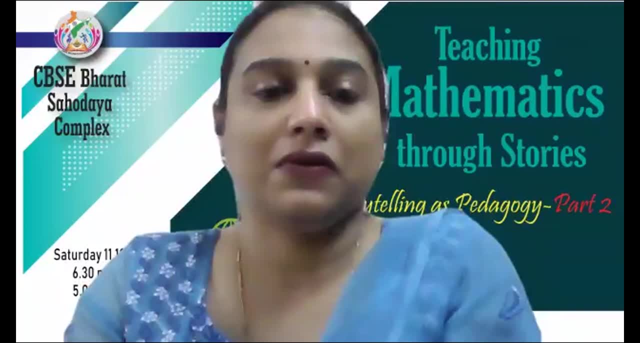 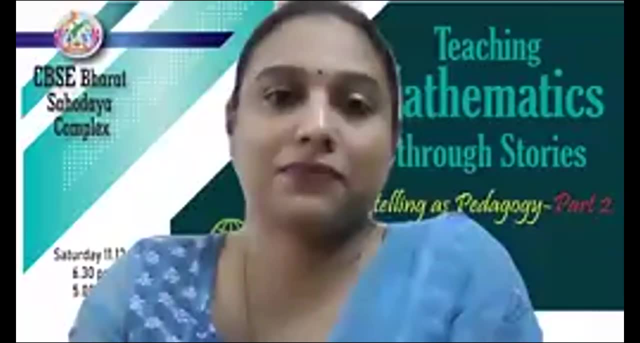 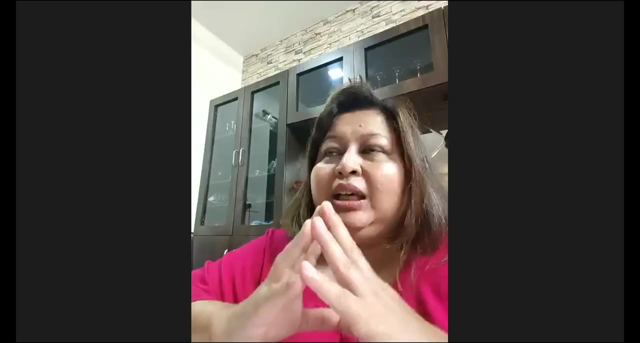 okay, and i'm working as an academic coordinator for grade 9 to 12. okay, i had a fantastic session and myself into voice modulation and dramatics and all these things, so i really enjoyed up me, you, you and i want to add one tip, uh to uh, i'm i'm sorry to barge in like this. it's your 40, but 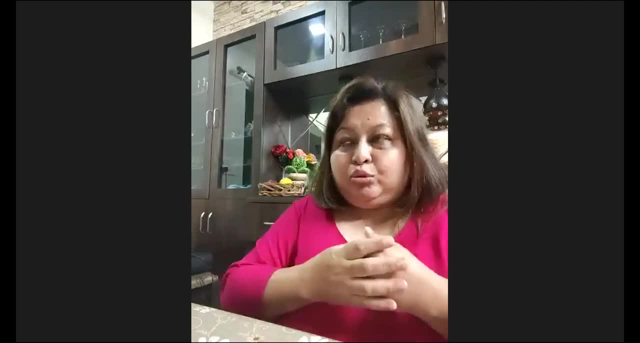 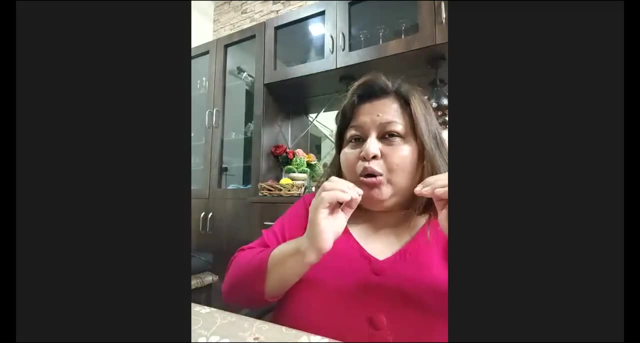 i want to add one tip, if at all you want to train your students on voice modulation? uh, i'm just showing one small exercise so maybe you know they can see, see and listen and see, uh, understand. what is it like if i say this: howling wind makes me shout. 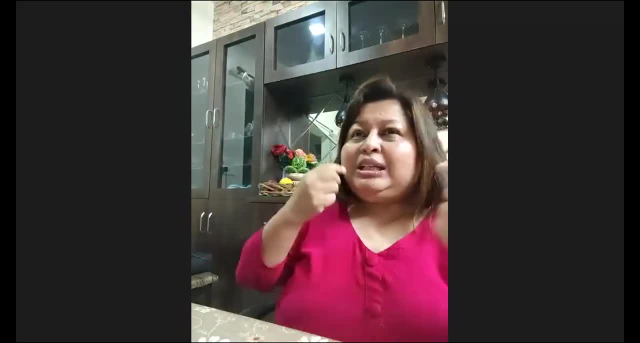 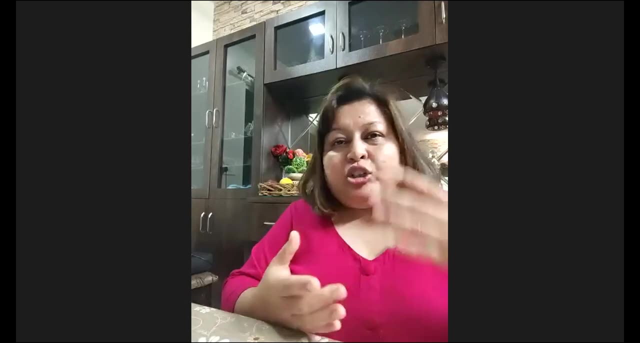 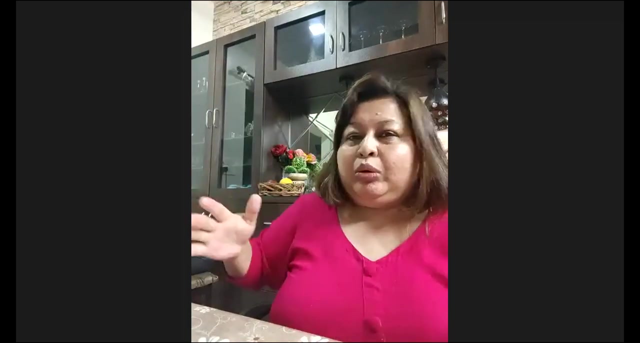 now my umbrella is inside out, so these are the small exercises and tongue twisters which will help. now, with our expertise, we can show. but what is the technique? so we can ask the children that you imagine that your uncle has come to pick you up in a railway station or an airport. so when you spot, 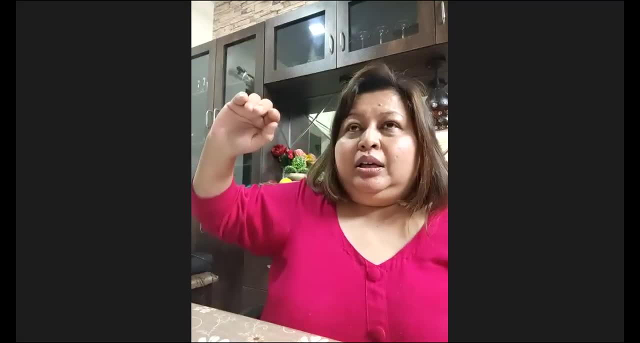 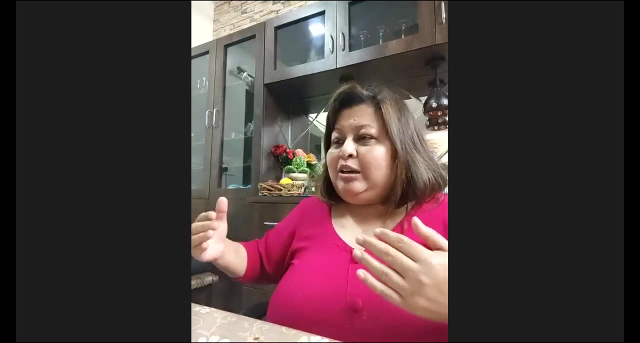 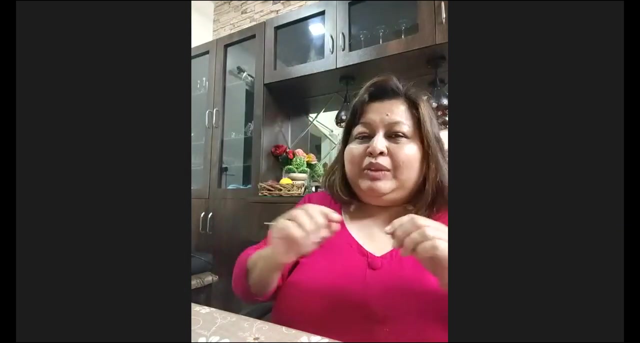 your uncle. you know how you will say cha-cha. and the moment you find him you're coming little close. cha-cha, namaste, and the moment he comes literally close. so these are some techniques we can show them, like what you did: auntie, auntie, would you like to buy some salt? 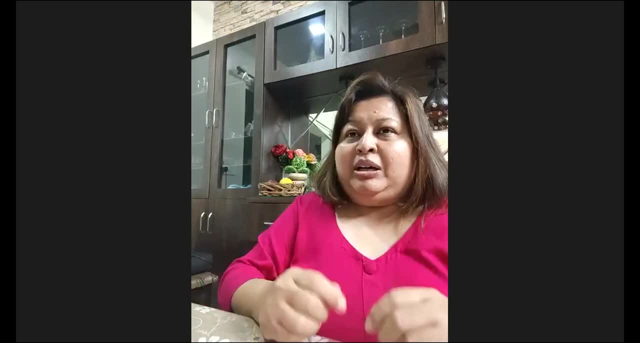 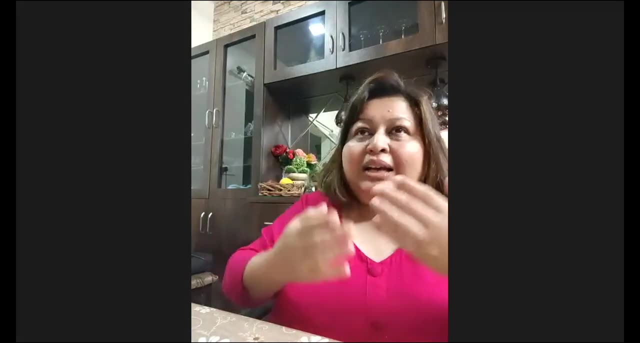 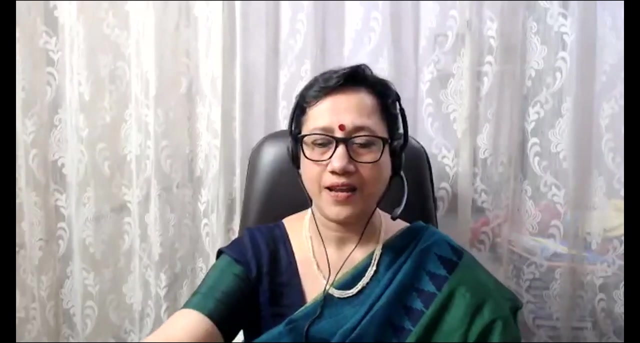 and then mama's voice: what have you got? why did you get the salt? and the papa's voice? so all these things we can learn with these techniques, there's someone. so we yeah what we have to do, that we have to keep it like one mark, one number here, two, three, four, five. 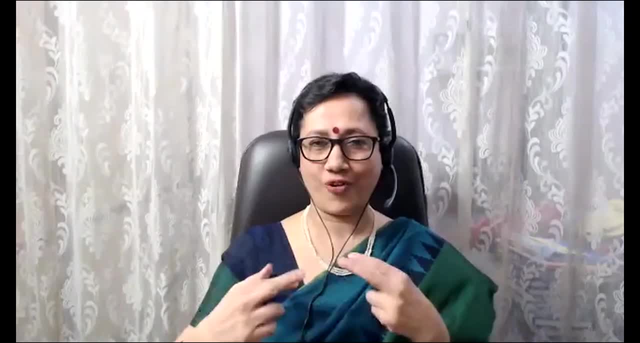 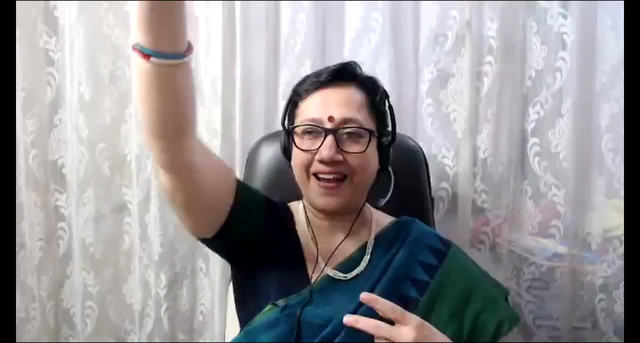 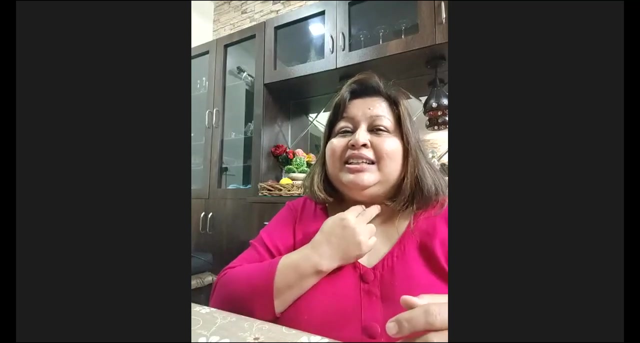 six, ten, ten. then what we do, like when i train, then what i do, the same way if one is sitting near in this front and then five is in the middle and ten is at the end. so if i am going to address my audience who is sitting at the tenth row, then i'll shout like this: these are the toolbox we have. a. 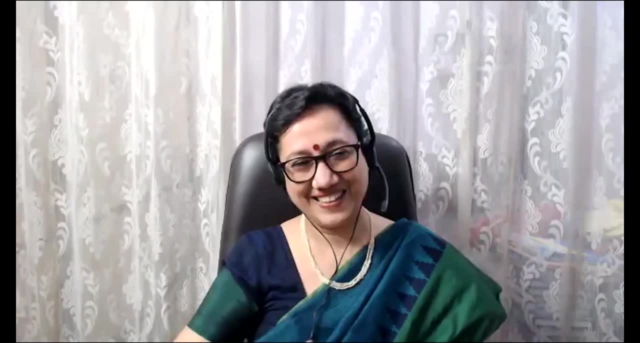 toolbox by god. yeah, it's a gift that is inside our mind and we have to find the right tool to do this. we have a tool box by god. it's a gift that is inside our mind and we have to keep it, and we have to keep it. 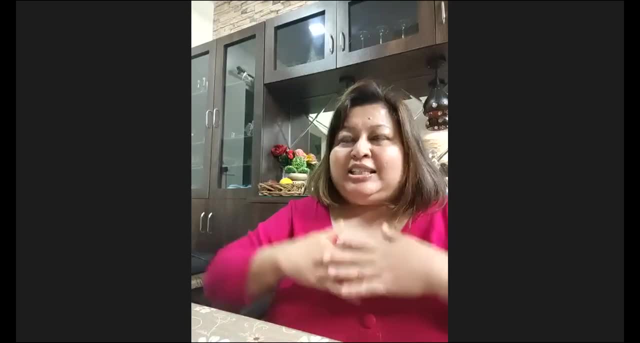 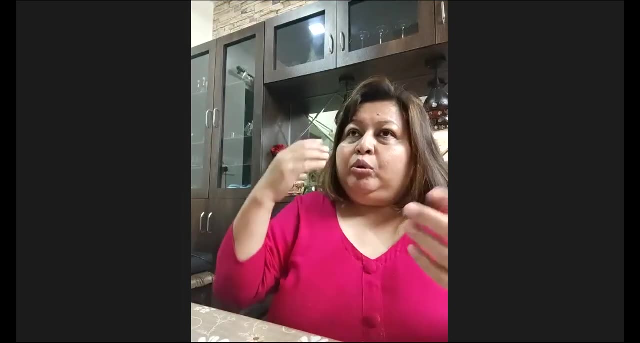 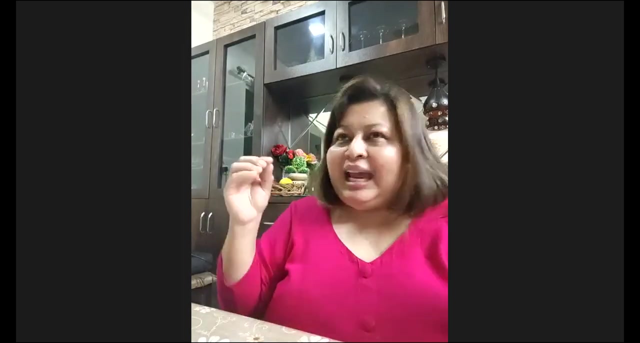 uh throat, so we can use the base. so these are the techniques. the teachers must know that, how to modulate and very interesting storytelling. but then you have expertise and framing. from mathematics point of view, i would only understand english point of view. hats off to you and the entire team. thank you, i have nothing to do with. 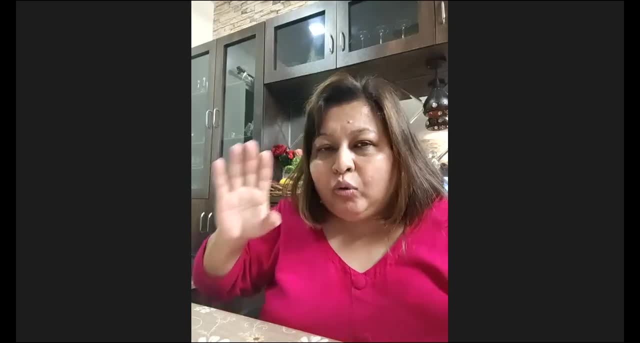 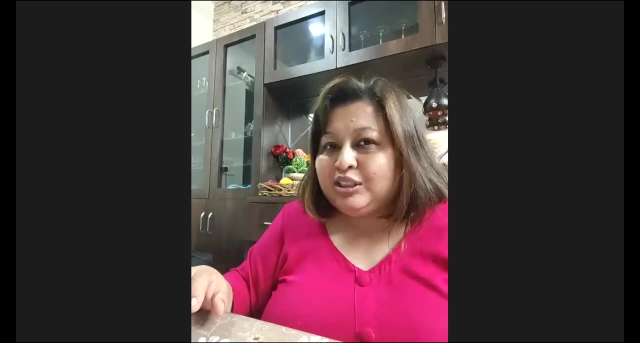 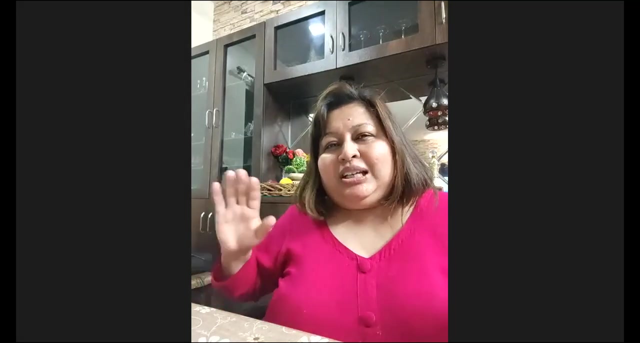 mathematics, but i said let me log in and the moment i heard your voice it was music. it was like any rj, as someone just said, listening to a radio session. very interesting, thank you. interesting, i think i put glue on my seats and i was sitting, thank you. 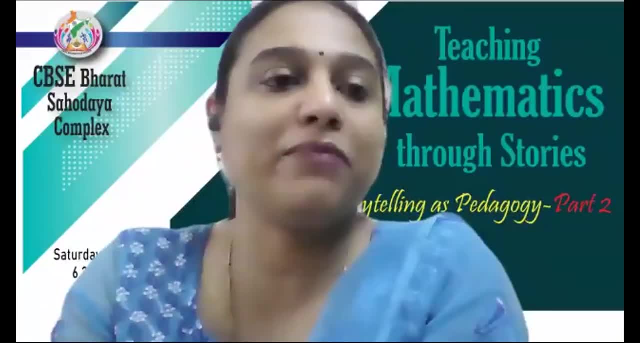 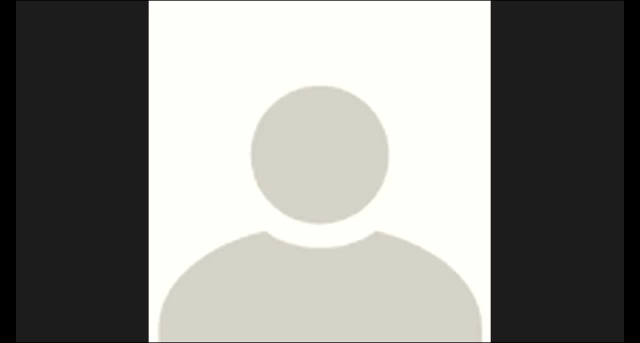 thank you so much, ma'am, yes, ma'am, yes, ma'am, yeah, ma'am. very wonderful section and actually i'm handling lower classes, but but the voice modulation, fantastic, ma'am. really i'm very happy with your section and i'm very excited i'm at the from monday. i at that moment only. i wanted to start with my explanation very. 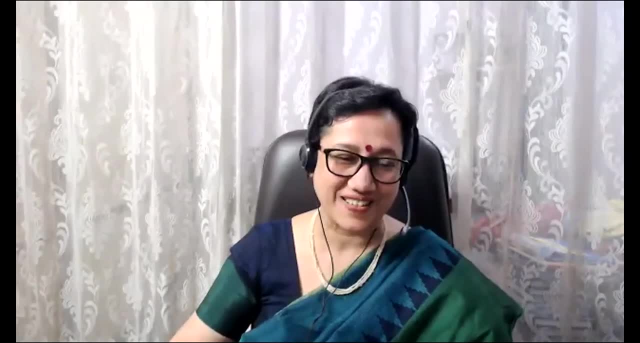 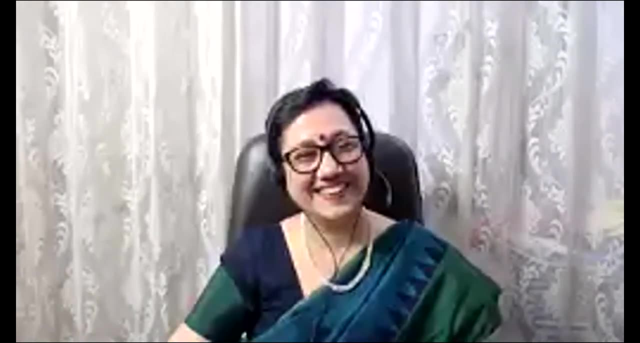 very, very, very happy. ma'am. oh, my god, thank you so much, especially for the lower classes. what we needed is the storytelling. yes, storytelling is not so easy, but when, when i attended your section, i couldn't express my thing. ma'am, wonderful, wonderful section, thank you very much excited. 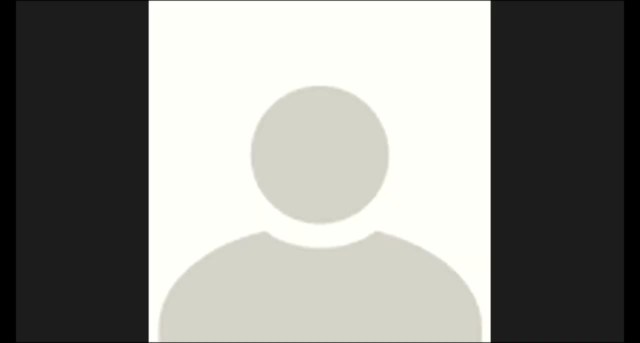 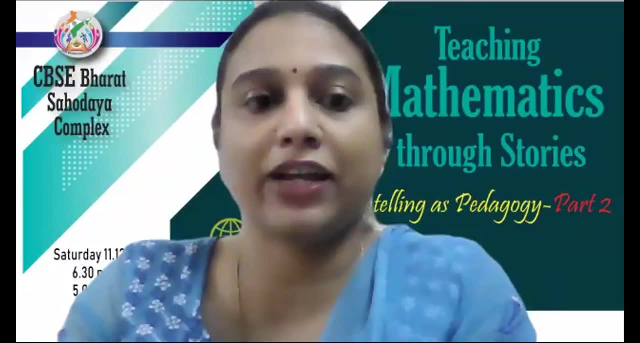 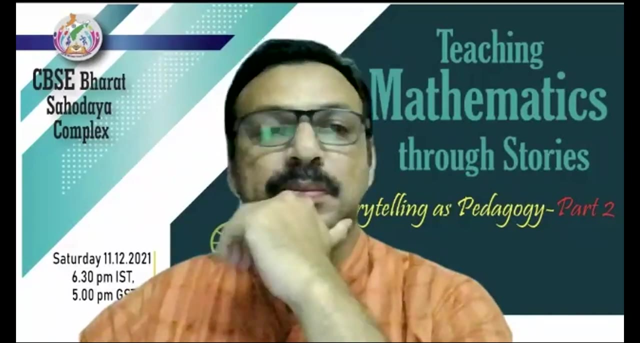 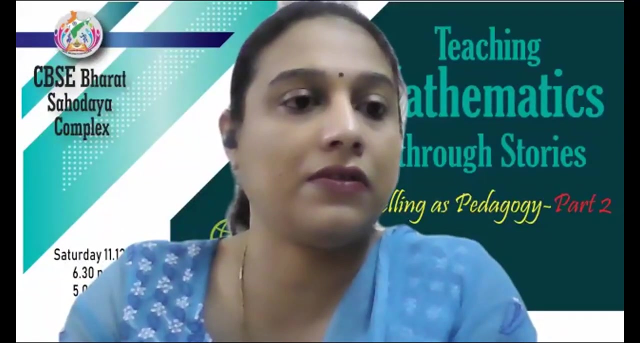 thank you, thank you so much, thank you, thank you so much, thank you. thank you, ma'am. do we have any more questions? sir, i cannot see any more questions. they can raise their hands. if participants in their questions, they can raise your hands. yes, yes, mr sanish. 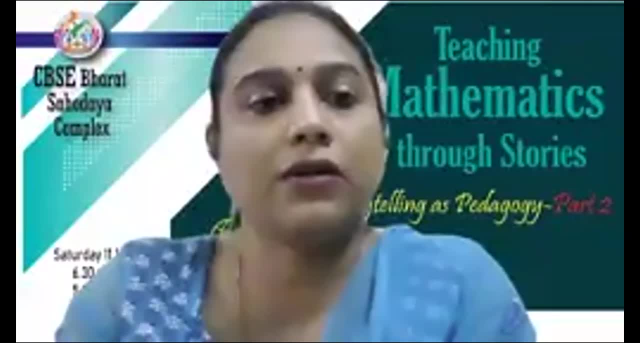 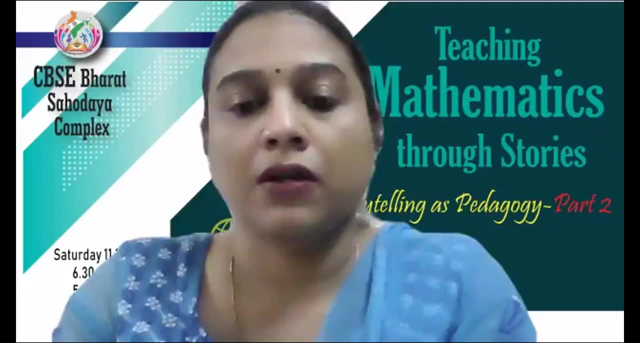 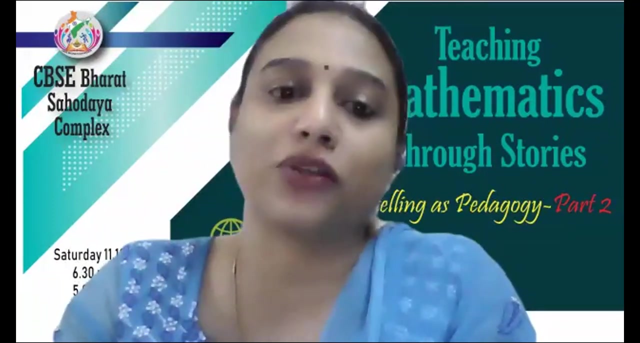 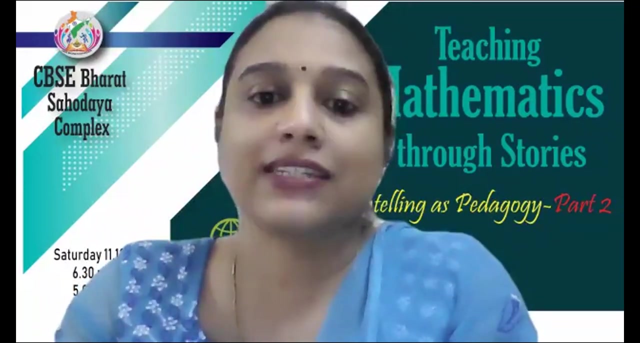 okay, ma'am, okay, compañeros. thank you once again, usha ma'am, for such a wonderful and enriching session. the participants, their expressions and their comments have constructed all. thank you so much. we come to the end of today's session. let we propose the formal vote of thanks. I begin by thanking our extreme resource person for today. 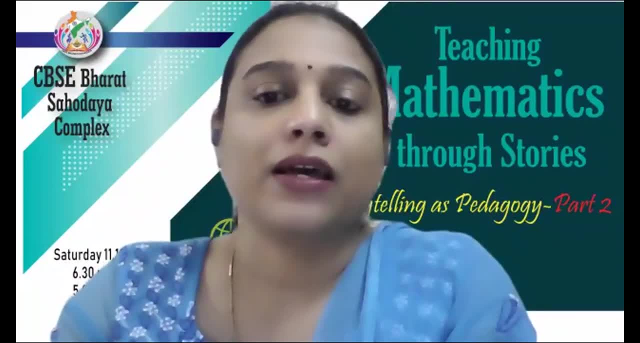 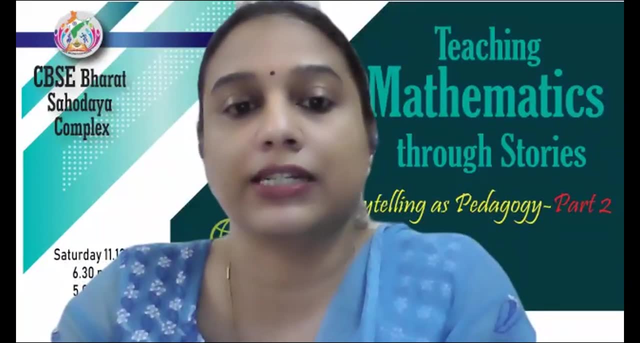 Mr Shah Chhabra for conducting such a wonderful session. We have all gained such a lot more knowledge and tips and tricks to make mathematics more appealing and attractive to our learners. Your exuberance and zest are contagious, as I said before, and all of us are motivated. 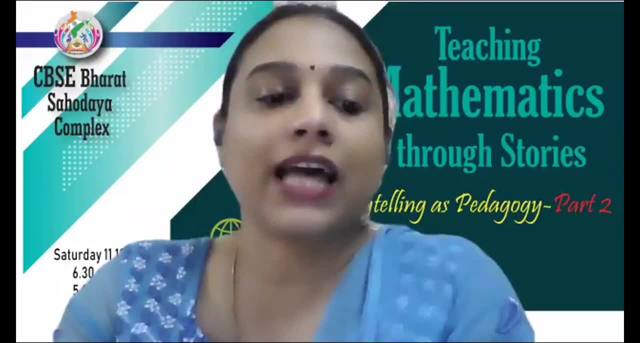 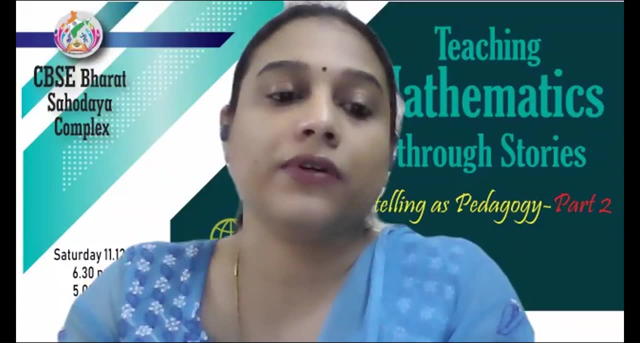 to try teaching math through storytelling. My humble thanks and gratitude to our program director, Dr Abdul Salam, for giving me yet another opportunity to work for Bharat Pahodia and for his unflinching support. Thank you, sir. A special thanks to our program collaborator. 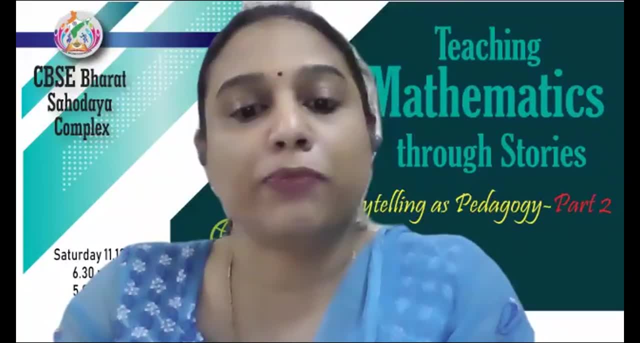 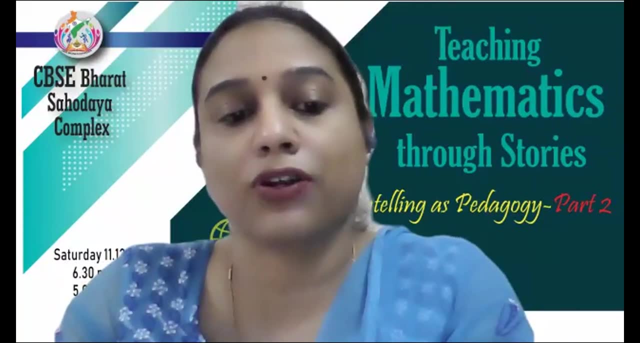 Mr Shibu for supporting us in every way. A big round of applause for our technical team today: Mr Arun Mohan and Mr Arafat. Both of them worked tirelessly behind the scenes for all our sessions. Last but not the least, a very big thank you to each and every participant who 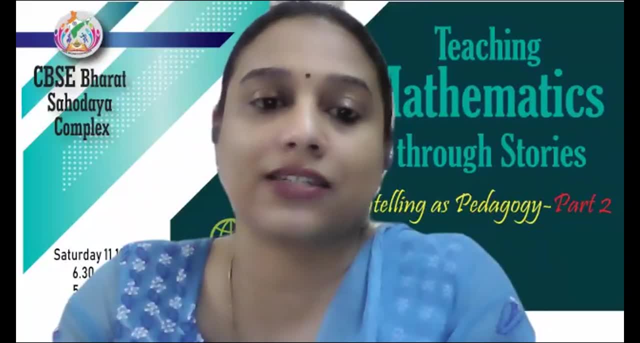 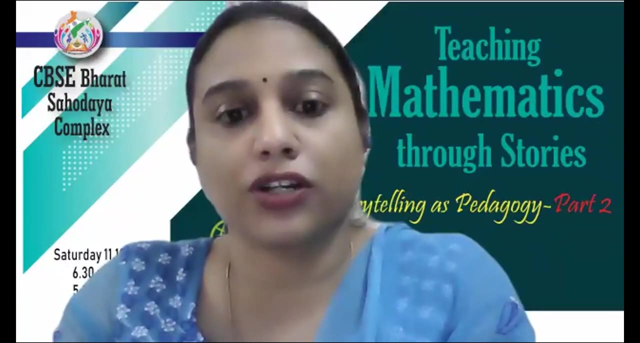 was present for today's session. Our children are truly blessed to have educators who are so very eager to learn and empower themselves. Before we wind up participants, please note that the feedback on certificate link, which is permanent for all our sessions, has already been posted on the chat box. 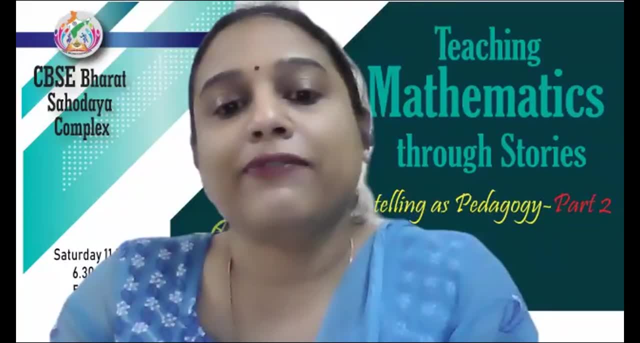 Please ensure that you all fill up the form. I believe that's it from my side, wishing you all a happy and healthy evening. We shall meet yet again for other equally wonderful sessions in the future. Stay healthy, stay happy and stay safe. 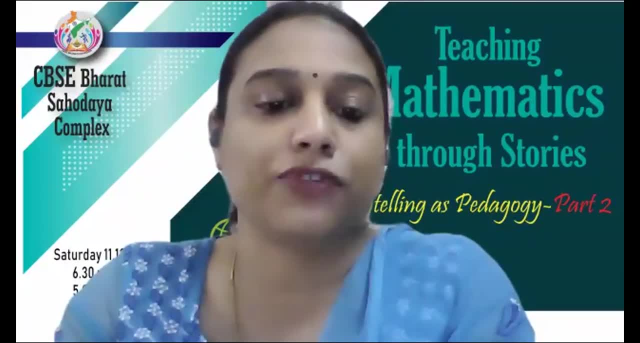 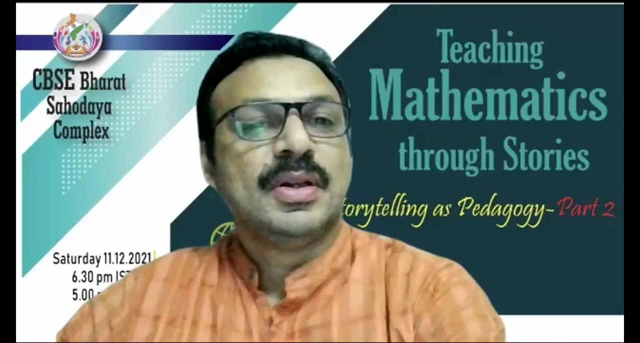 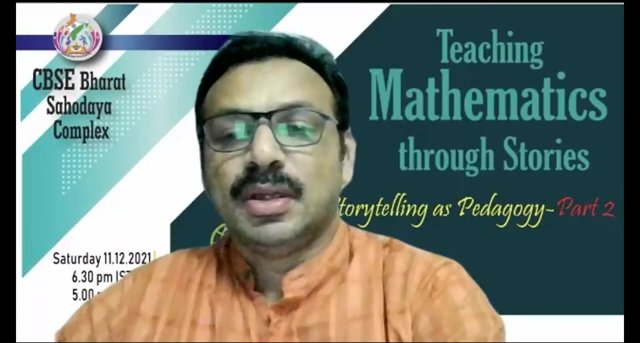 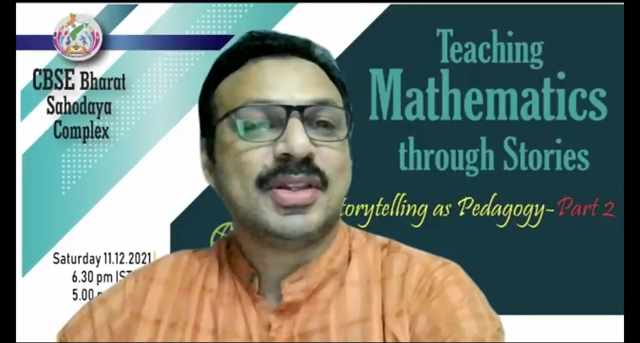 I now request Dr Abdel Salam to please wind up the session for today. Thank you, sir. Thank you, Sritamma, for the nice moderation you have done. You were helping us a lot. and participants: I would apologize for, you know, deactivating the chat box because I don't want you. 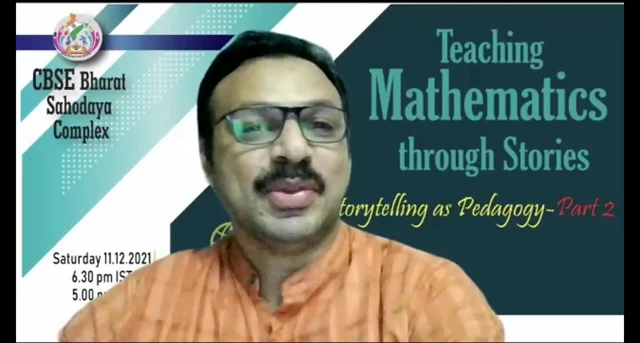 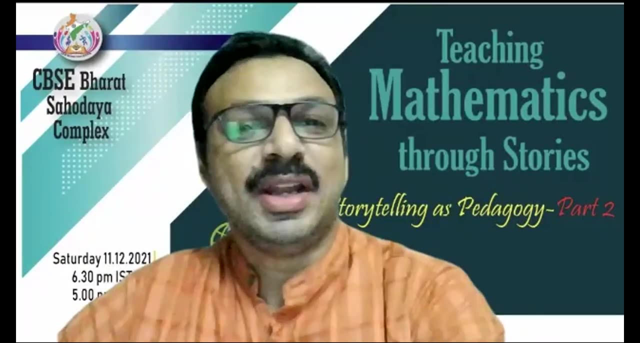 to miss uh, usha, madam's session. i mean the segments. we had a different segments, four or five segments from stories. so if you keep on, you know uh giving- yeah, i mean uh typing in the chat box- your attention may be, you know, diverted and uh, we don't. we won't get to usha ma'am every time. 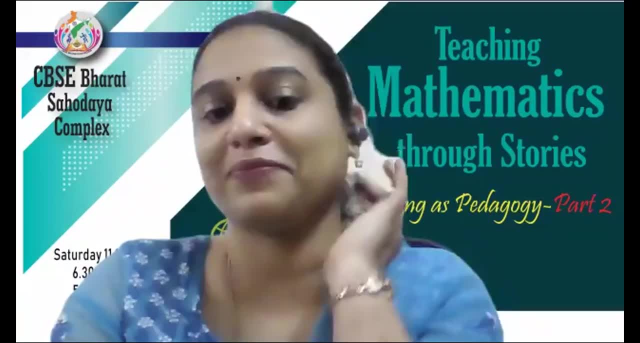 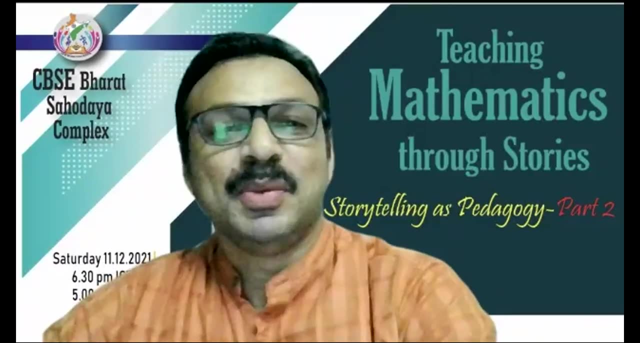 on board. uh, you know, we should not miss this chance opportunity. that's why so that's the very reason now, i think, the chat box is full of appreciation, as usual, with usha ma'am- rightly, madam has, you know, portrayed, she has shown how, uh, you know, children, especially the younger ones, can. 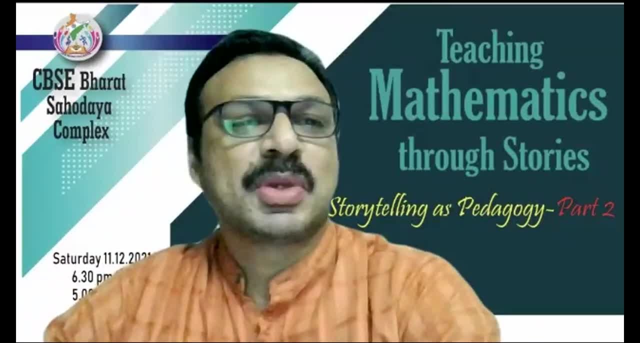 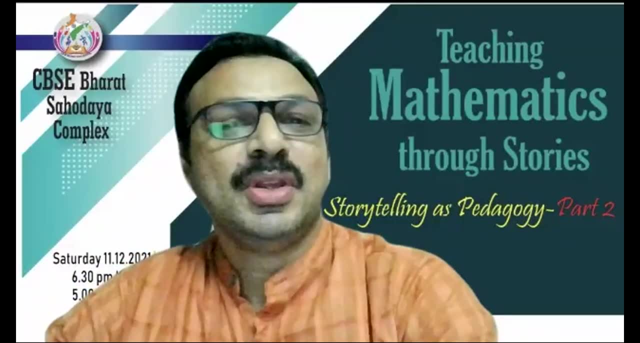 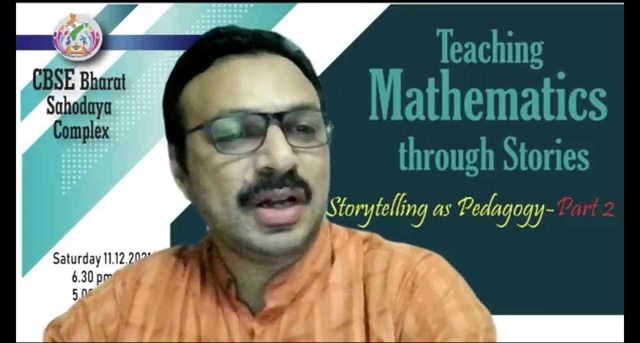 be made to sit and listen to you. especially when you have classes online, it's very difficult to catch their attention, so this is one of the best ways you know through expressions. that is very important. you have to dramatize the situation, as madam has. you know, she has worked hard and she, you know. 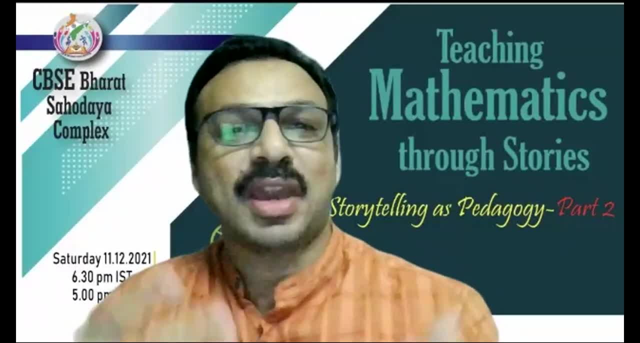 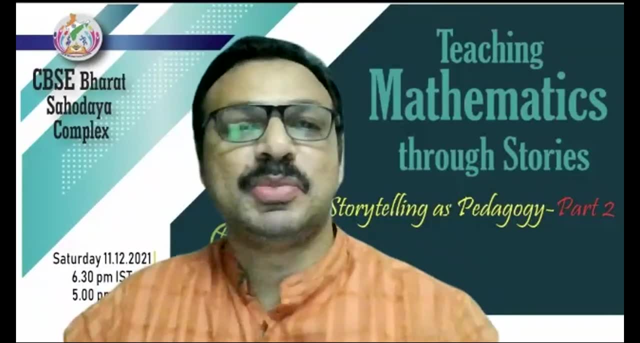 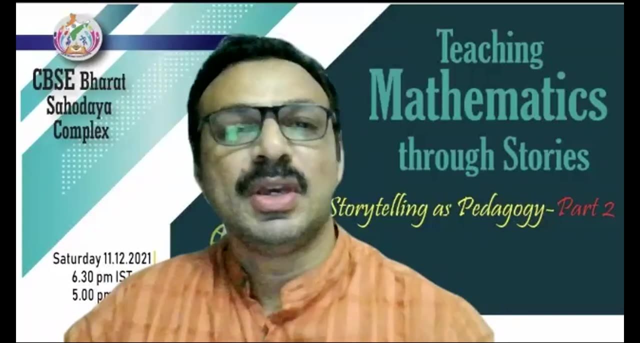 brought away, made plots, different plots and different characters, and you know she uh incorporated and uh related with the different subjects. that is wonderful. you know, as required by nep, that should be the mode of teaching these days. you have to relate to your teaching in with uh different subjects and also i like the way you know. 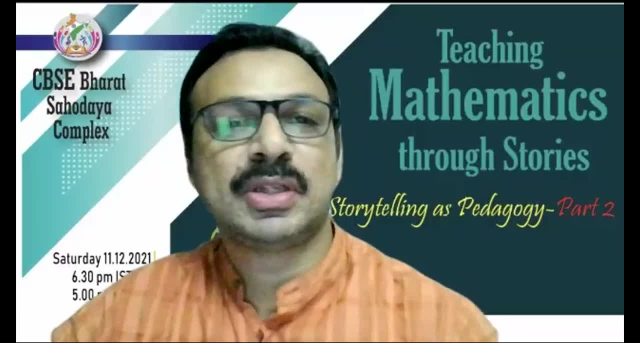 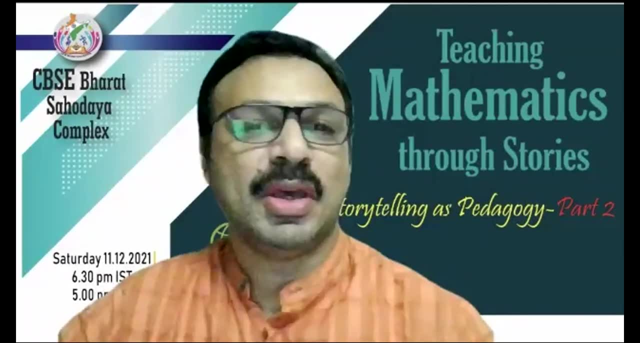 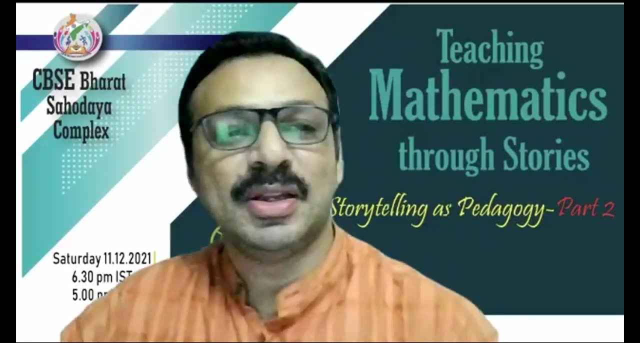 when children were asked to find out the measure of the tail and all it's, it's project-based learning. they go and they do research, they uh explore. so this is what we have to do. uh, please, uh, implement it in the classroom. uh, we are. we are pretty sure that some of you will be, you know. 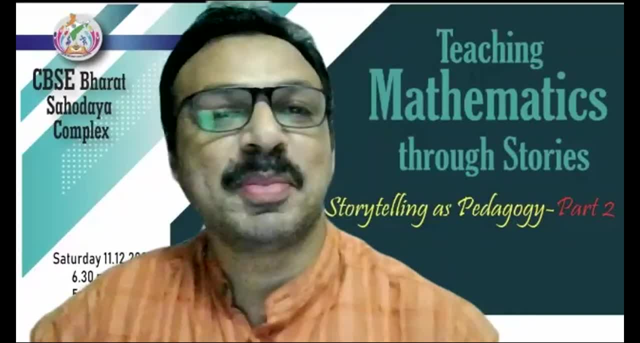 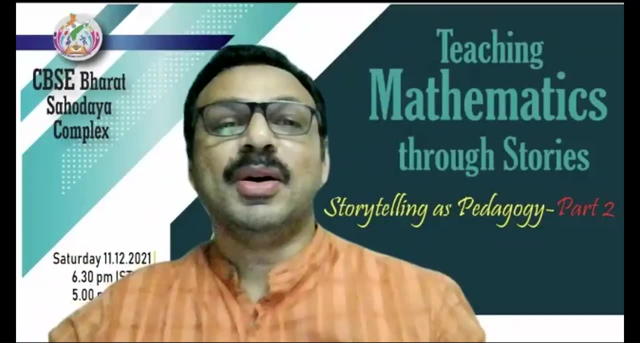 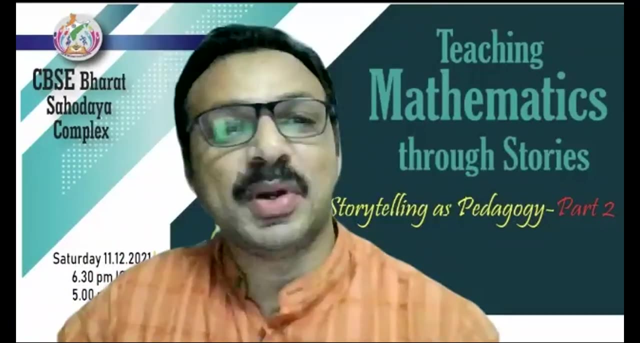 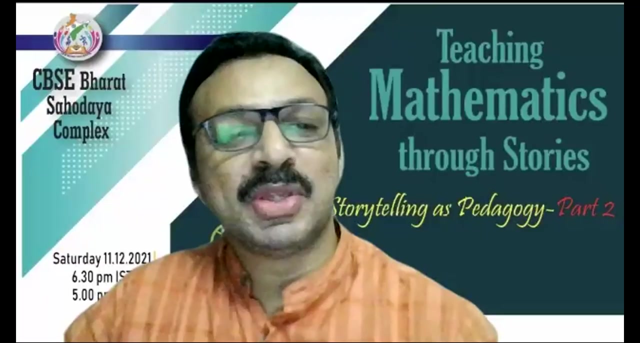 implementing into the next day itself, as uh one of the participants, as uh rightly said. so we are very happy, uh, for the second day we have with you. you know, here i hope you are a proven- we have no doubt that you are a proven storyteller. thank you so much. a master or mistress of all traits. 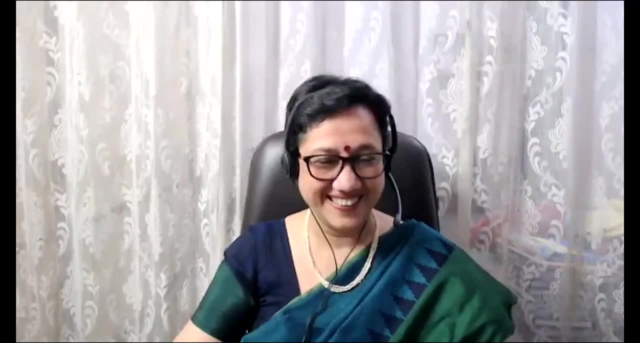 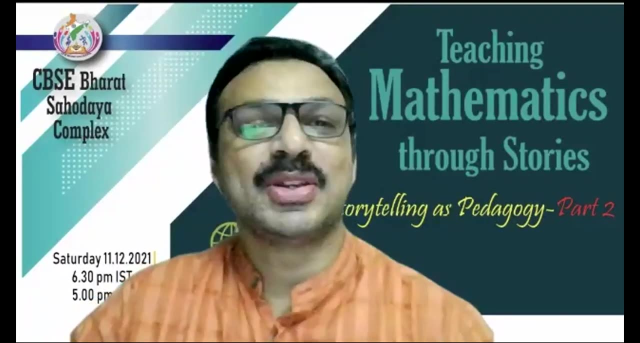 thank you so much for being with us and it's a pleasure listening to you, especially the voice modulation which we have to learn, and we are very happy to be here with you and we are very happy to be here with you and we are very happy to be here with you and we are very happy to see both of you. 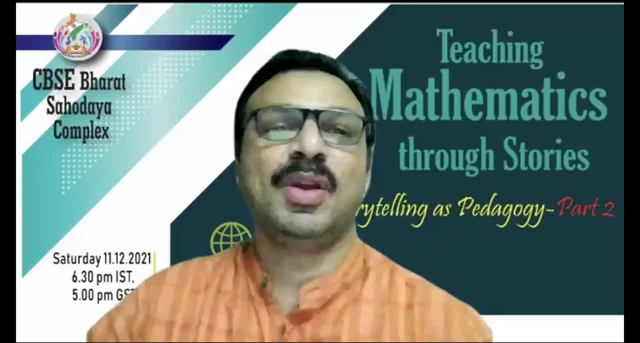 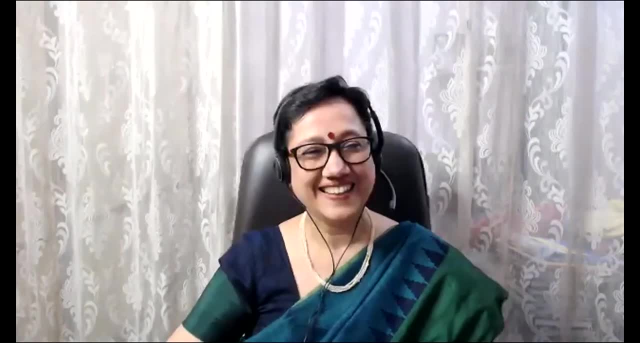 it's a gift. actually, you are gifted. so thank you so much, uh, each and everyone for listening to her and we we hope to have usha once again with a different topic, but nobody telling us. yes, thank you so much, sir, for your nice words and for this platform providing with this platform. 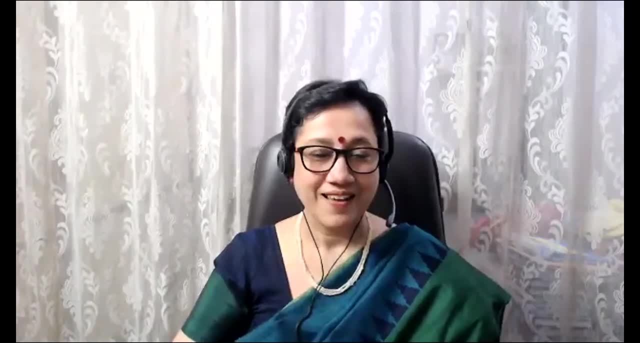 sarita, ma'am and all the participants who are here. uh, i must say that i was worried that, because it's a math thing, see, i had my in my bs. i have done my bse, but i think teacher have made me feel much better. i am like a teacher and i am a social scholar and i have been studying for all these years. 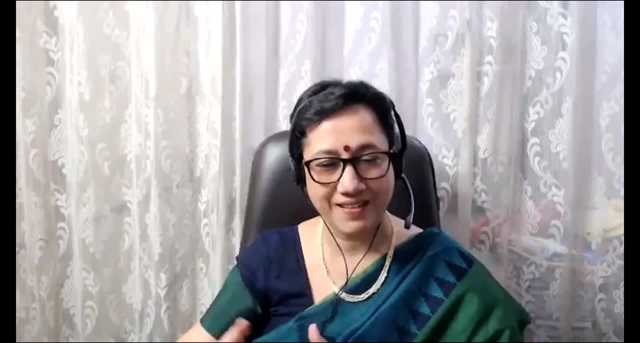 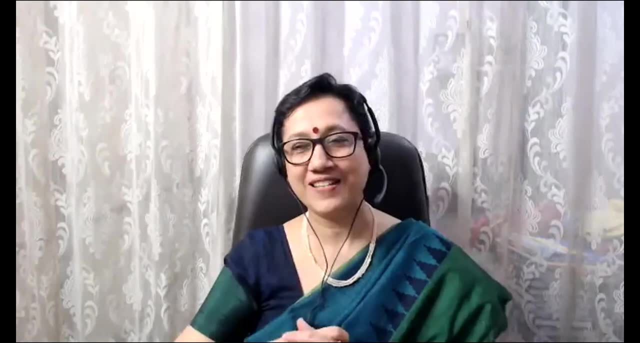 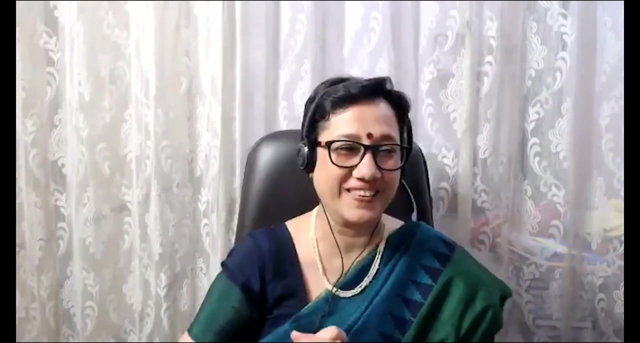 honest physiology. and later on I have shifted to Hindi and then English also. I done so, but a long time gap. you can say enough with the maths. so I was just worried whether I will be able to do justice or not. but yes, as when storytelling comes, then no problem, I feel. so I can manage, so I have.